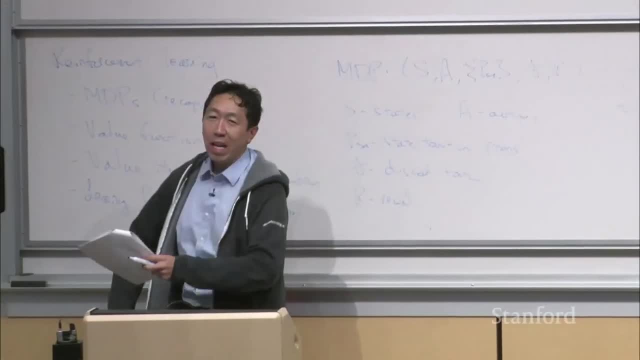 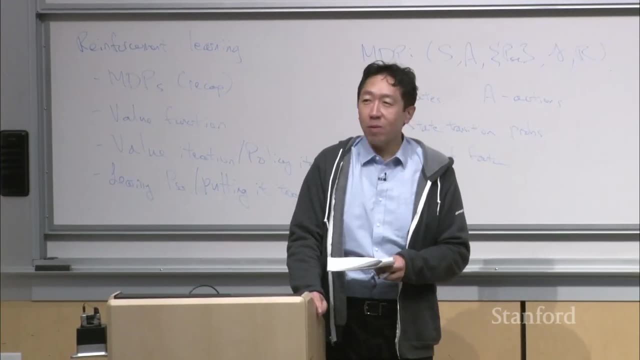 Not sure if you guys are following the news, but in- in reinforcement learning, we chat a lot about robotics, right, And one of the- you know uh cluster problem a lot of people use reinforcement learning to solve is robotics. And um, I think uh, uh back in May, um, 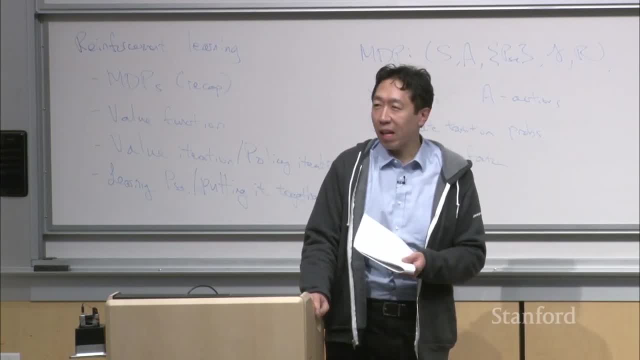 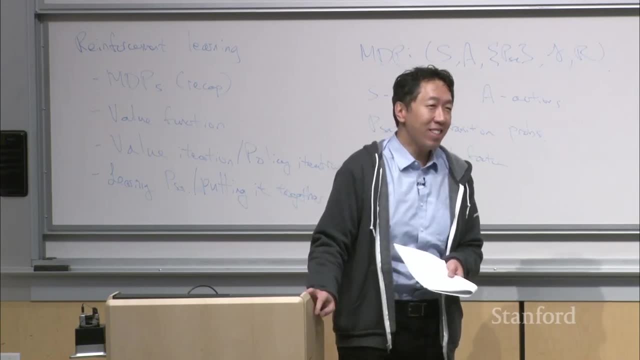 the InSight Mars Lander had launched from uh here in California and is about to make an attempt at landing on the planet Mars in the next two and a half hours or so. So excited about that, Uh, I think it's actually one of the grandest. 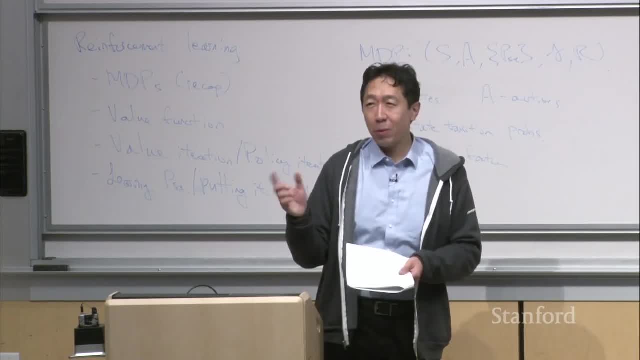 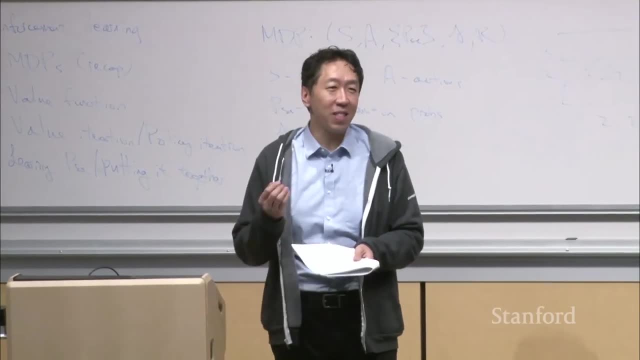 um applications of robotics, because you know with a what 20-minute light speed from Earth to Mars. you know, once it starts its landing, there's nothing anyone on Earth can do, And so I think it's actually one of the most exciting applications. 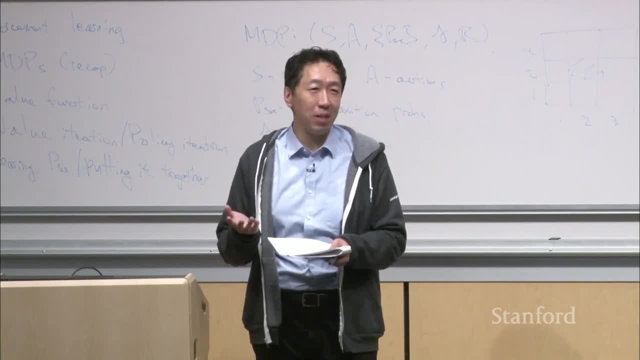 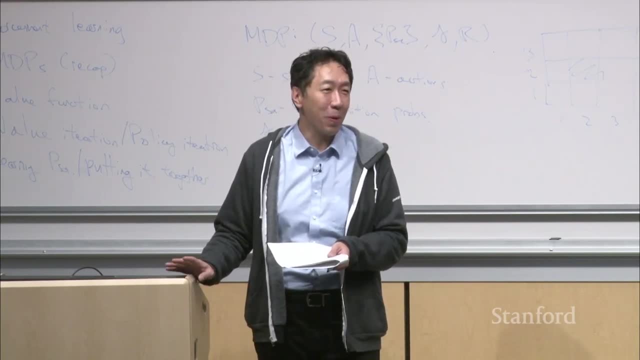 of autonomous robotics where you launch this thing is now about 20-- 20 light minutes away from planet Earth, So you actually can't control it in real time, uh, and you just have to hope like crazy that your software works well enough. 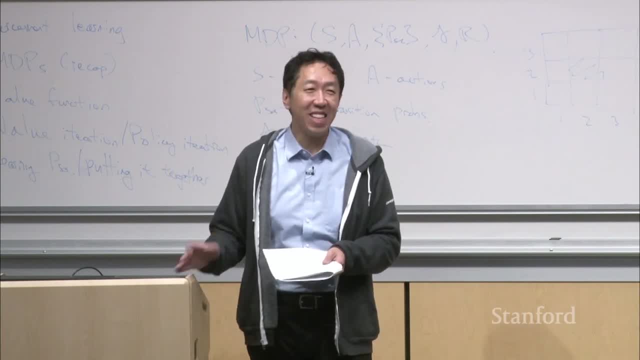 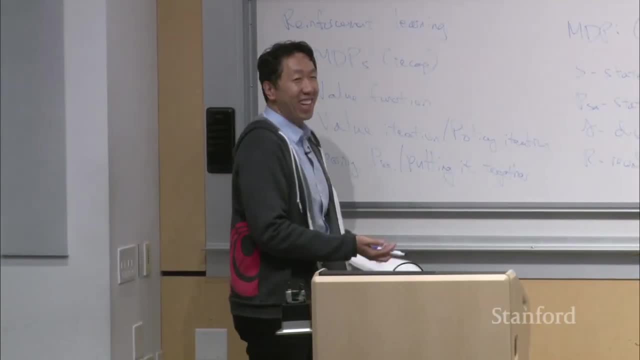 for it to land on this planet. you know, uh, uh, And- and so we'll- we'll find out a little bit after noon if the landing happened successfully or not. I think- I don't know. I- I think, um sorry. 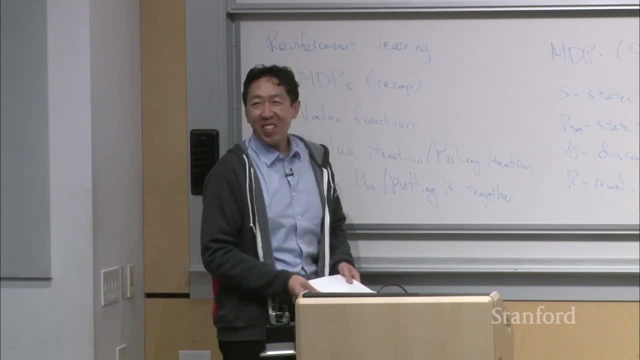 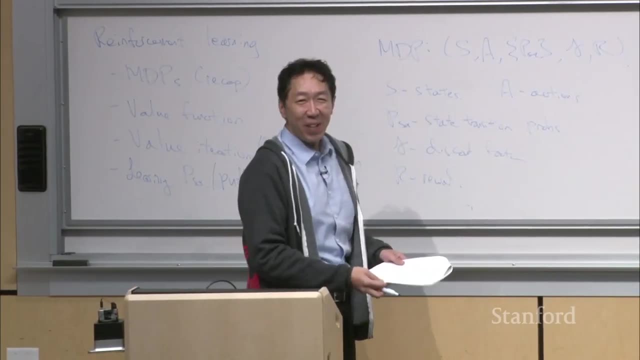 I- I just get excited about stuff like this. I- I hope you guys do too. And for those of you that are from California, I mean: take some pride that it launched from a home state of California and- and is now nearing its uh- landing on Mars. 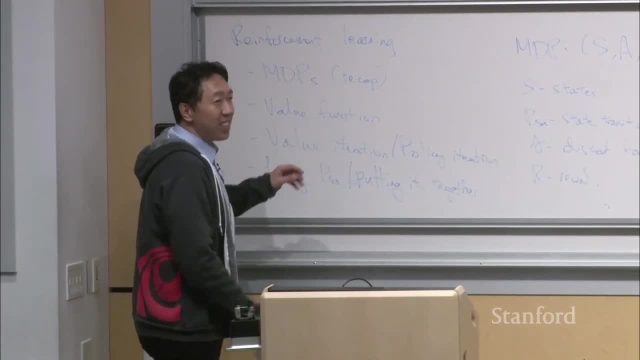 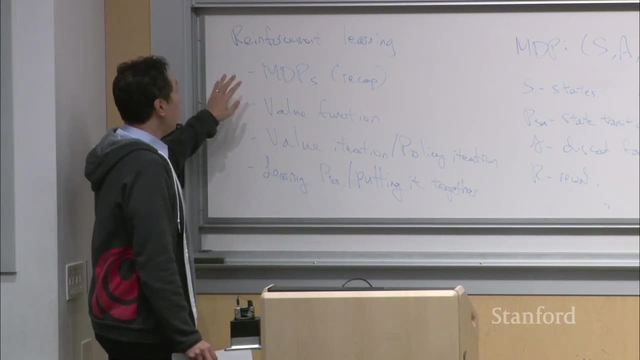 Okay, Um, all right. So, um, what I want to do today is, uh, continue our discussion on reinforcement learning. Uh, do a quick recap of the MDP, or the Markov Decision Process Framework, Um, and then we'll start to talk about algorithms for solving MDPs. 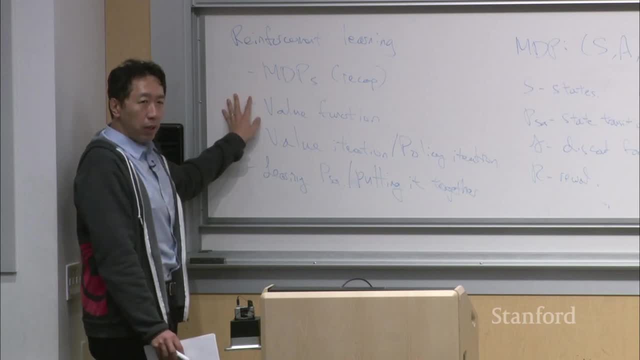 In particular, need to define, uh, something called the value function, which tells you how good it is to be in different states of the MDP. And then, um, we'll define the value function and then talk about an algorithm called value iteration for computing the value function. 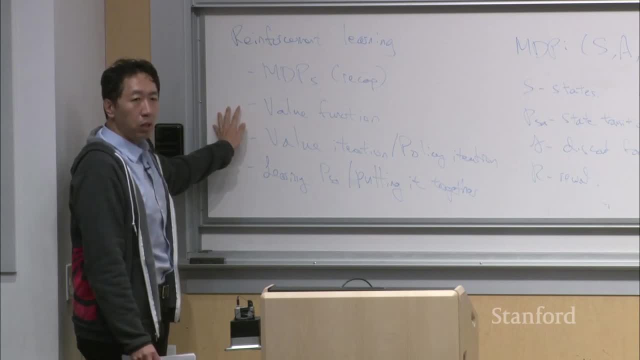 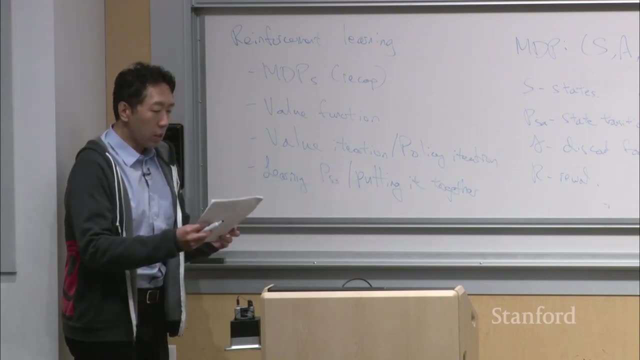 And this will help us figure out how to actually find a good controller or find a good policy for an MDP. And then we'll wrap up with uh learning, state-transition probabilities and how to put all this together into an actual reinforcement learning algorithm that you can implement. 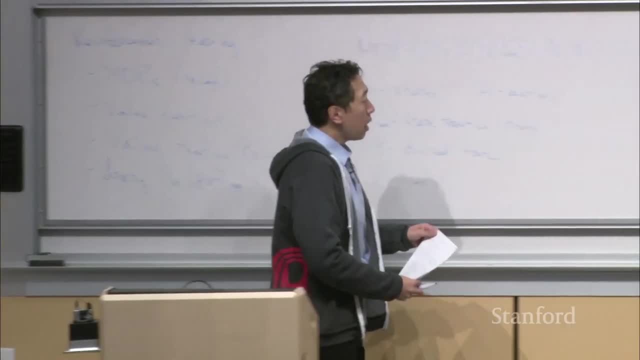 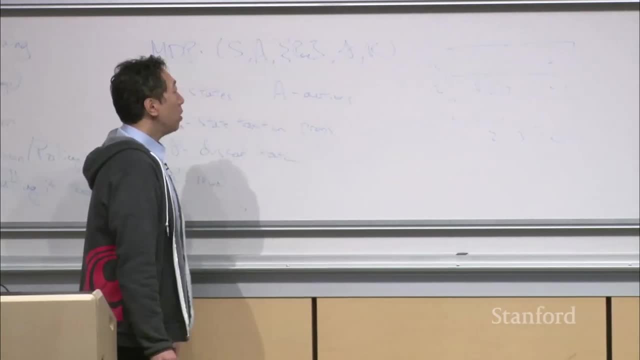 Um, to recap, um, a motivating example, a running example from the last time, from before Thanksgiving, was uh, this 11-state MDP, And we said that an MDP comprises a five-tuple, a list of five things with uh states. 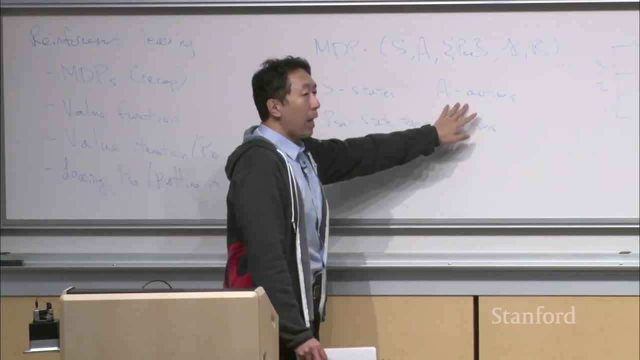 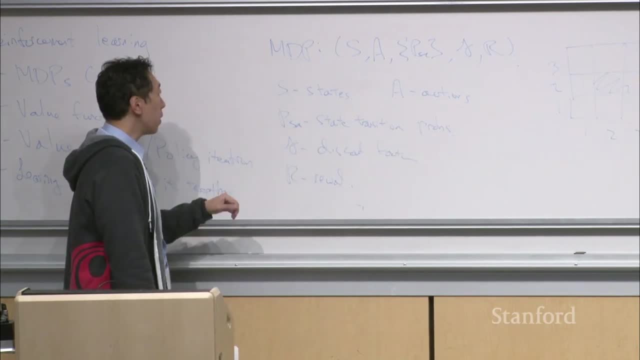 So that example had 11 states um actions And in this example the actions were the compass direction north, south, east and west. You can try to go in each of the four compass directions, The state-transition probabilities and in the example, 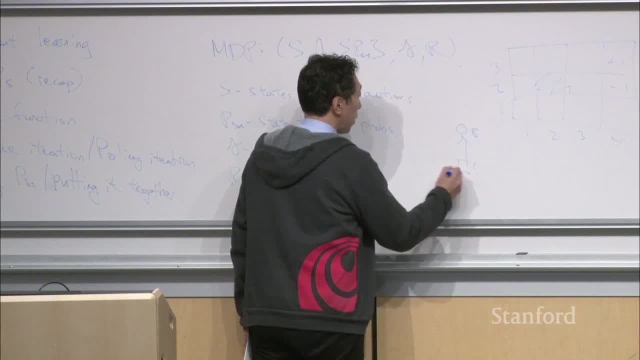 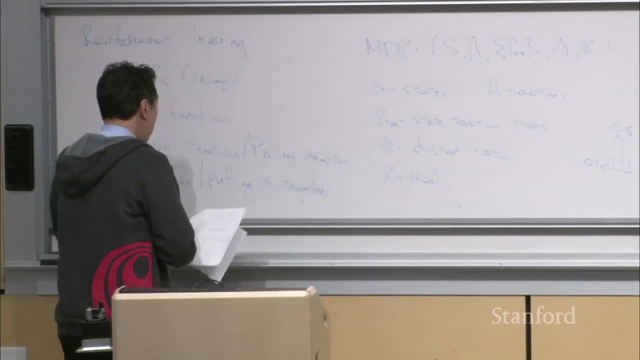 if the robot attempts to go north, it has a 80% chance of heading north and a 0.1% chance of veering off to the left and a 0.1% chance of veering off to the right. 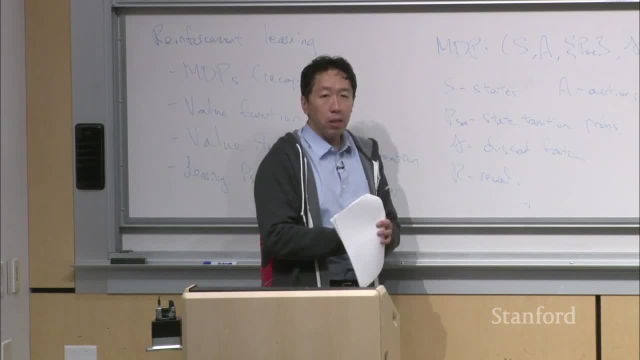 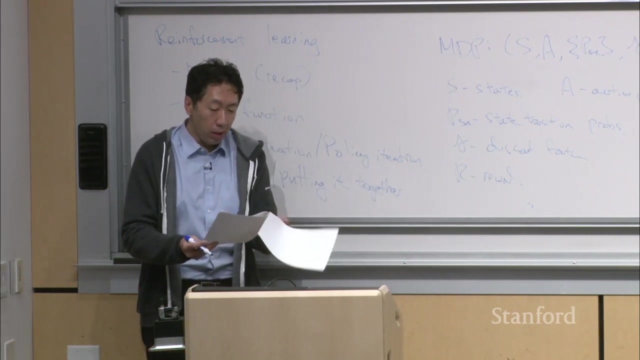 Um. gamma is a number slightly less than one. Um usually slightly less than one. There's a discount factor. Think of this: as you know, 0.99.. Um and r is the reward function that helps us specify where we want the robot to end up. 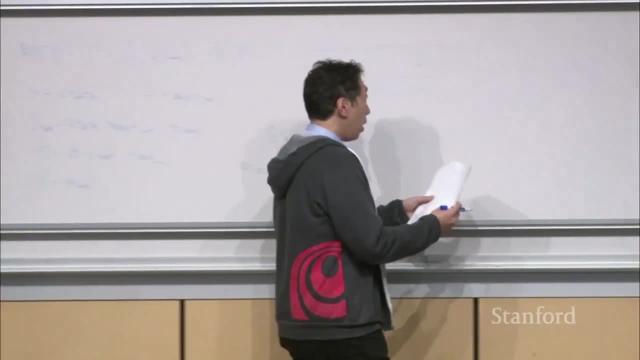 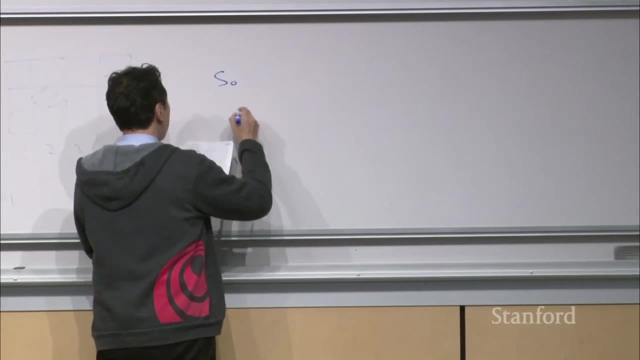 Um, and so what we said I said last time, was that, um, the way an MDP works is you start off in some state s zero. Um, well, it's much better. You choose an action, uh, A zero. 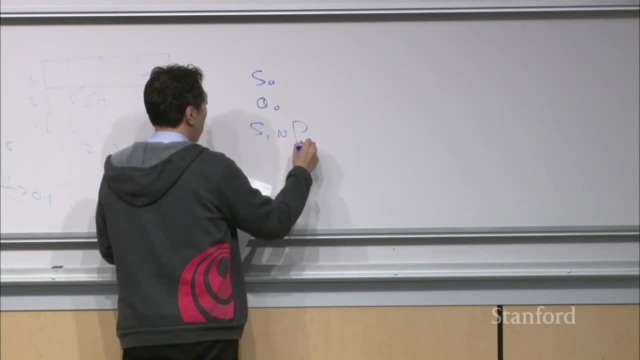 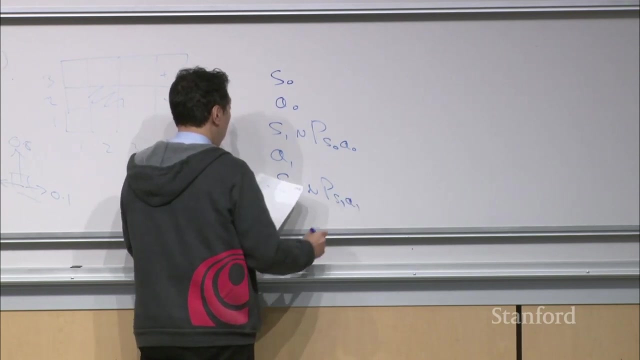 And, as a result of that, it transitions to a new state- S one- which is drawn according to P of s- zero, A zero. And then you choose a new action- A one- And as a result, the MDP transitions to some new state P of s one, A one um. 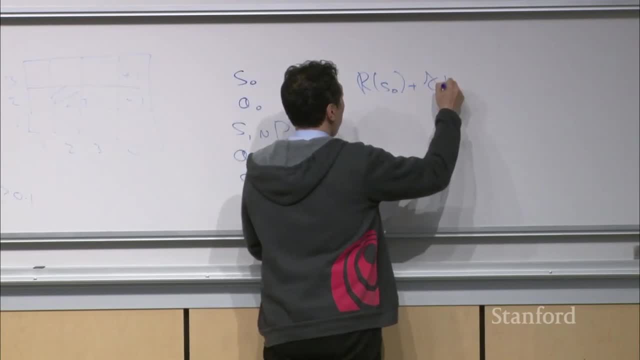 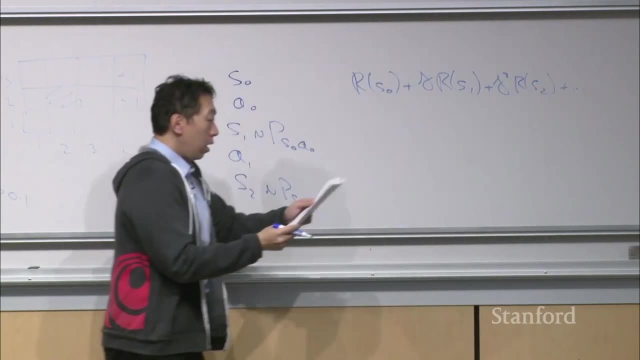 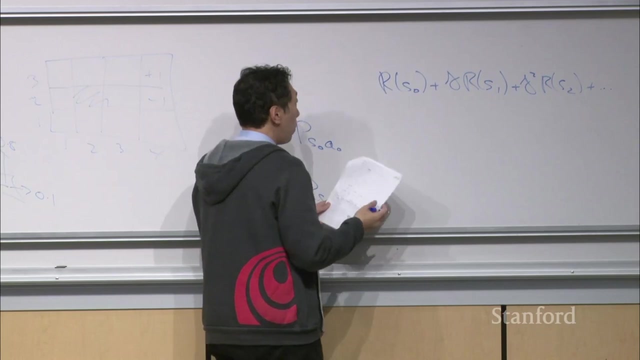 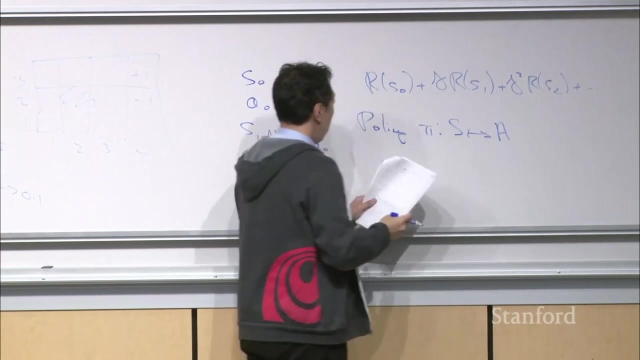 and the total payoff is the sum of rewards, right, Um, and the goal is to come up with a way, um, and formally, the goal is to come up with a policy, pi, which is a mapping from the states to the actions. 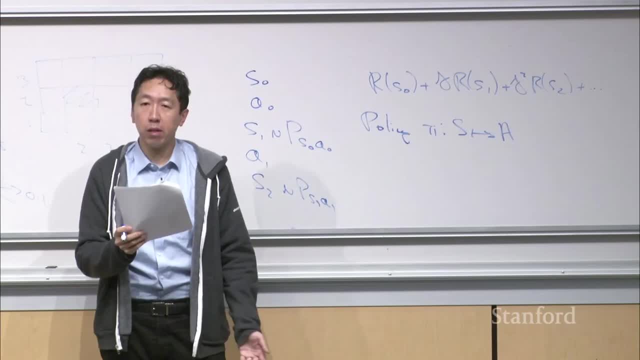 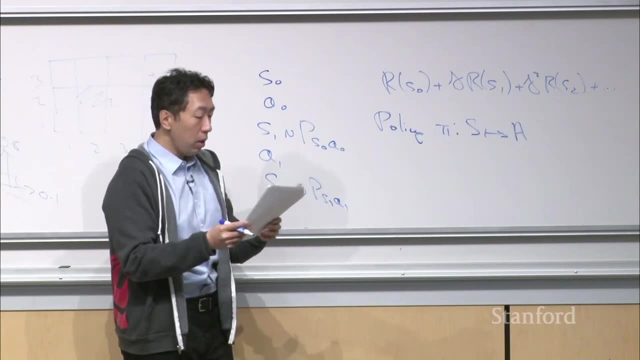 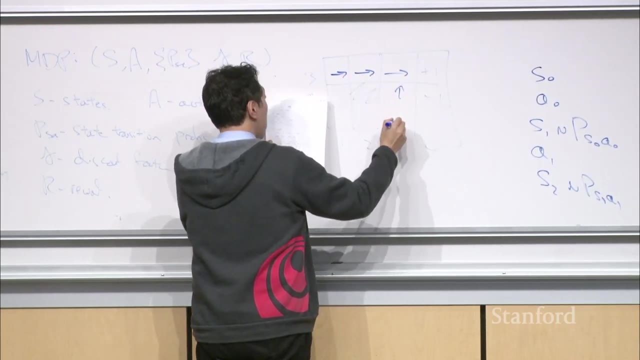 uh, that will tell you how to choose actions from whatever state you're in, so that the policy maximizes the expected value of the total payoff. okay, Um, and so I think last time I- I kind of claimed that this is the optimal policy for this MDP right. 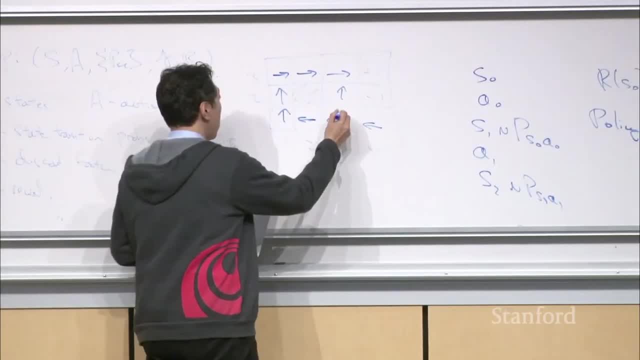 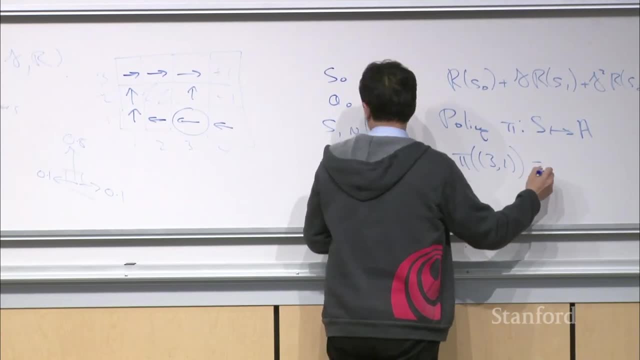 Um, and what this means, for example, is, if you look at this state, um, this policy is telling you that pi of 3 comma 1 equals uh, west, I guess. Or you can write west or left, or whatever you call that left arrow right. 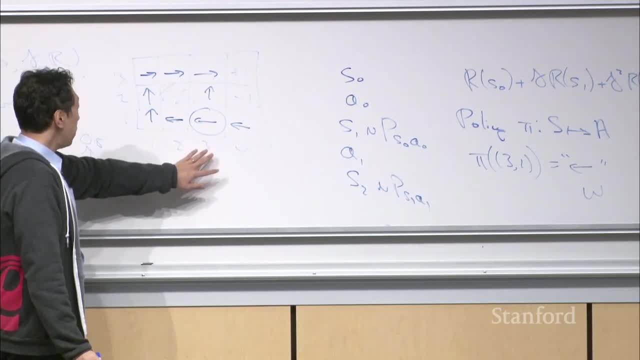 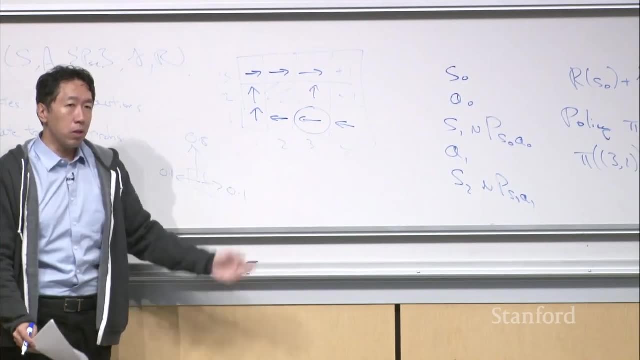 Where? from the state um, from the uh state 3, 1,. you know, the best action to take is to go left, is to go west, And so, if you're executing this policy, what that means is that um. 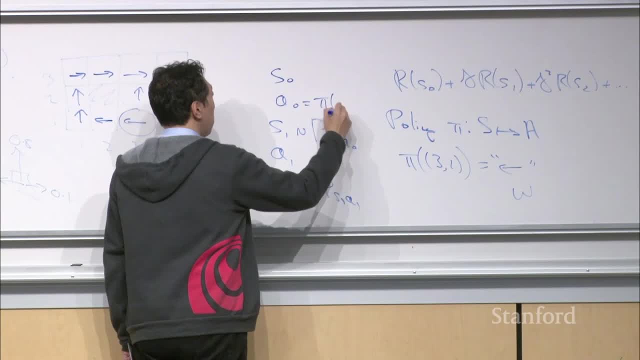 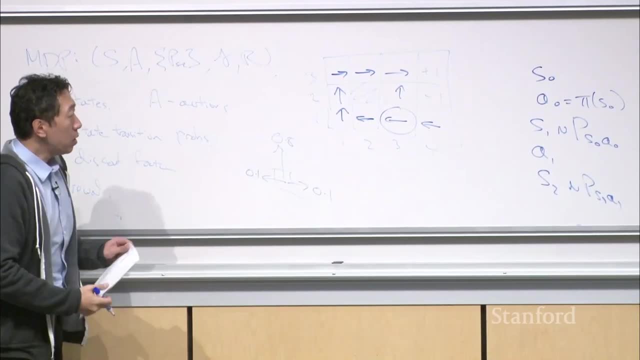 on every step, the action you choose would be, you know, pi right of the- of the state that you're in. okay, So, um, what I'd like to do is now, uh, define the value function. 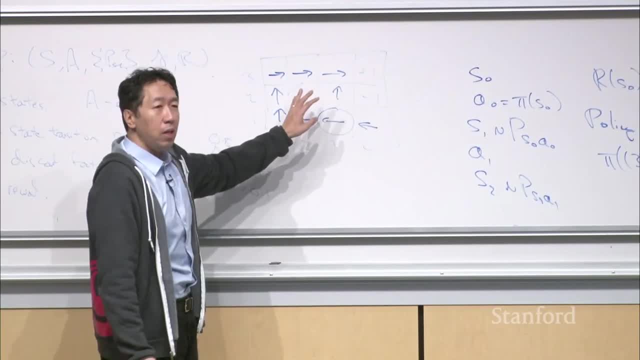 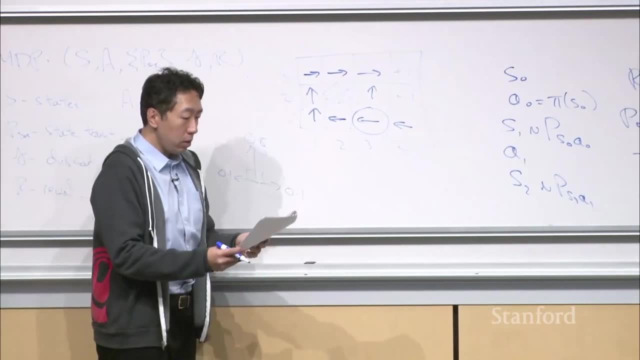 Uh, so how-, how-, how- how- how did I come up with this right? What I'd like to do is have you um learn. given an MDP, given this 5-tuple, how do you compute the optimal policy right? 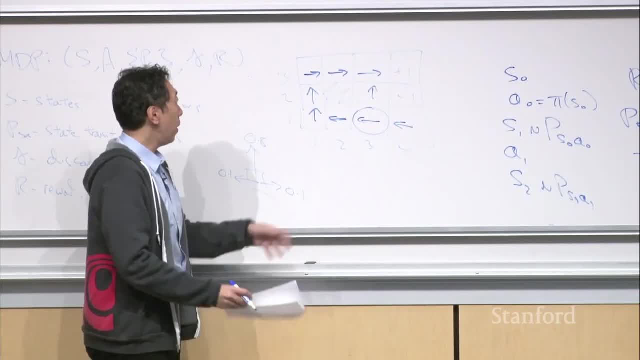 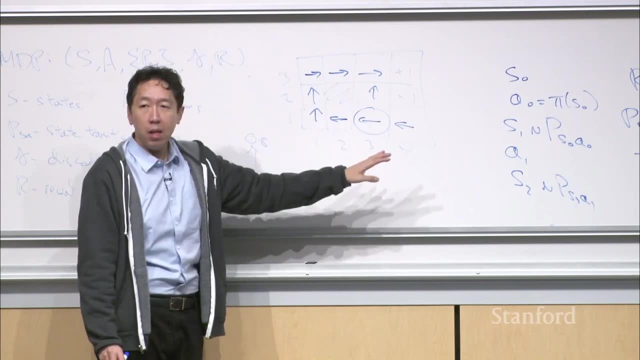 And one of the challenges with um- finding the optimal policy- is that you know there's a- there's an exponentially large number of possible policies, right? If you have 11 states and four actions per state, the number of possible policies is. 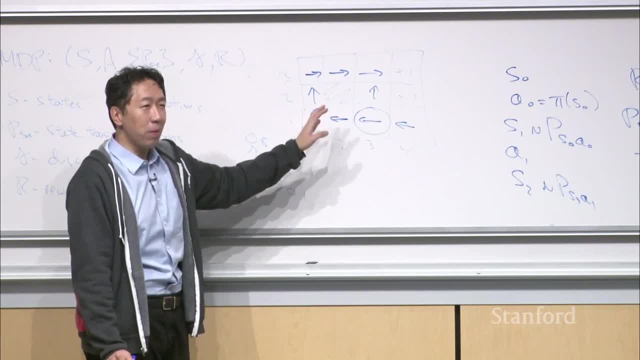 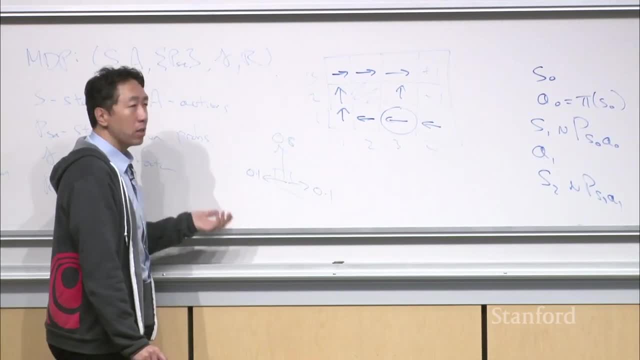 uh four to the power of 11, which is not that big because 11 is a small MDP. right, There's a number of uh policies- possible policies for- for an MDP is combinatorially large. There's a number of actions to the power of a number of states. 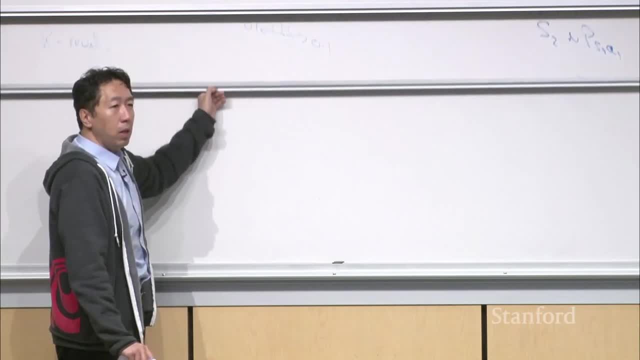 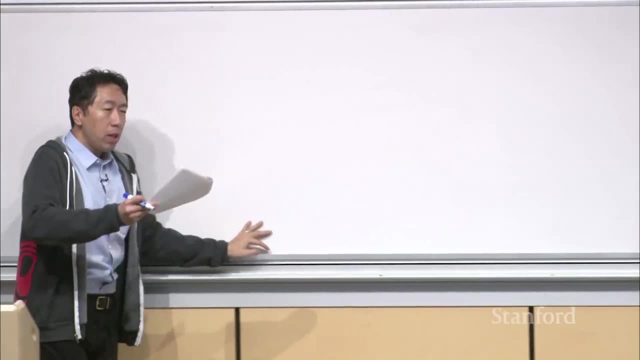 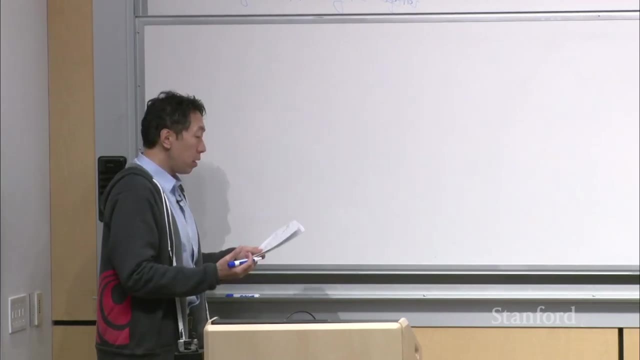 So how do you find the best policy? okay, So what you learn today is, um, how to compute the optimal policy. Now, in order to develop an algorithm for computing an optimal policy, um, we'll need to define, define three things. 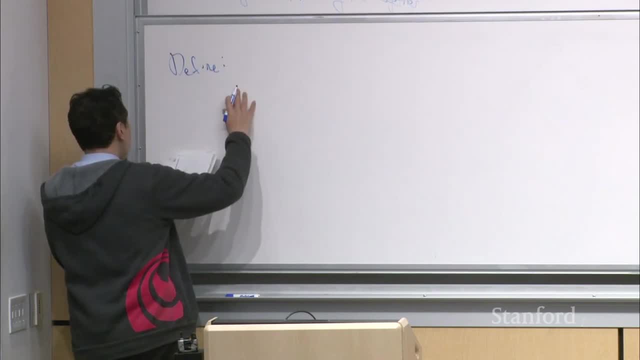 So, just as a road map, um, what I'm about to do is define V, pi, V star and pi star. okay, Um, and based on these definitions, we'll see that we'll- we'll- we'll come to a definition. 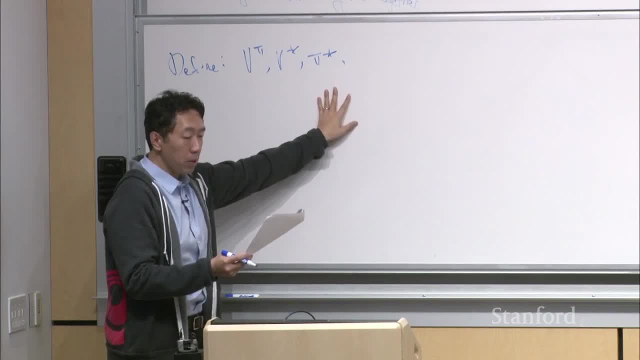 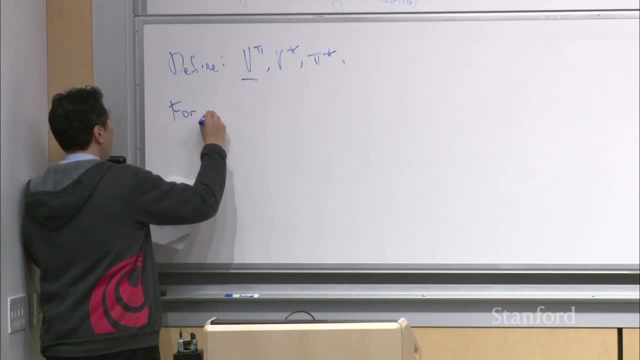 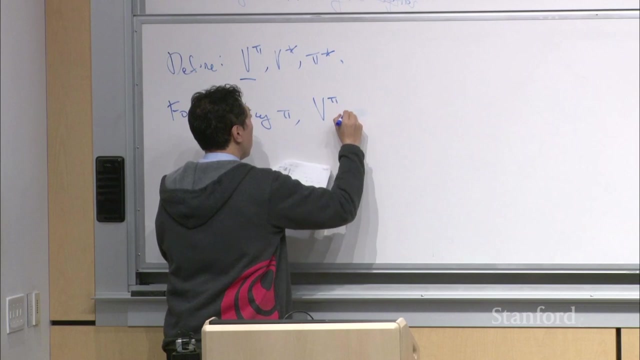 we'll, uh, derive that pi star is the optimal policy. okay, But so let's- let's go through these few definitions Um first, V pi. So for a policy, pi V pi is a function mapping from states to the rules. 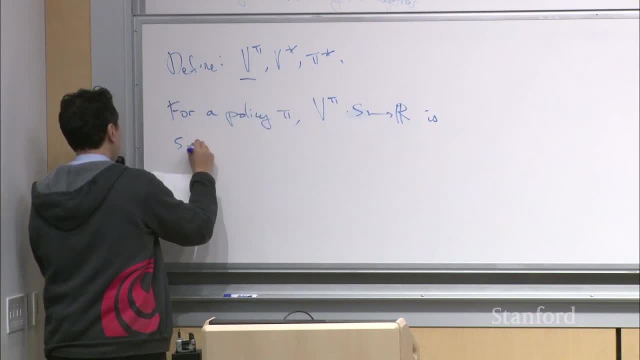 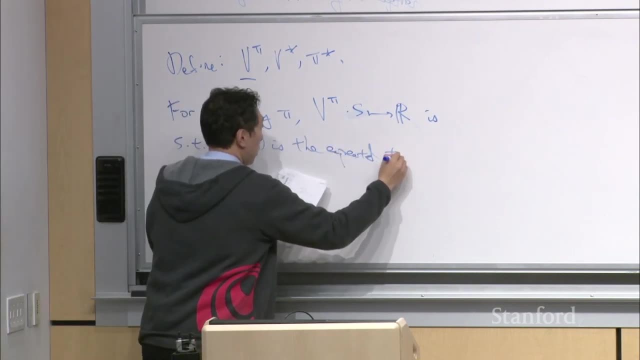 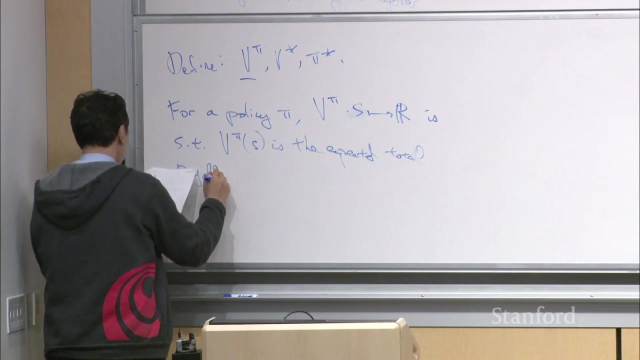 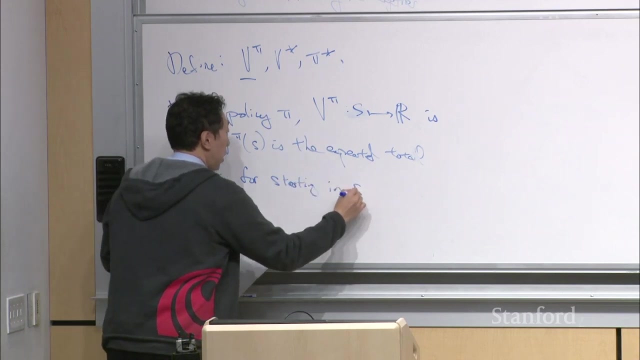 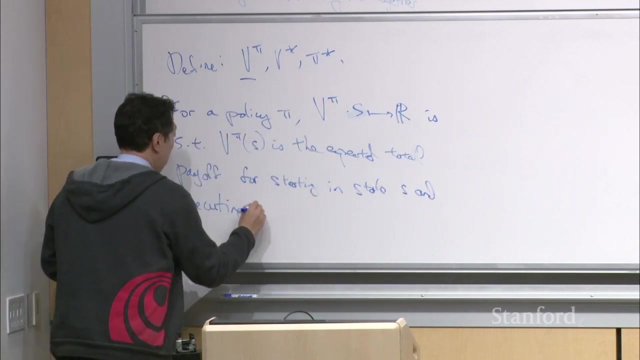 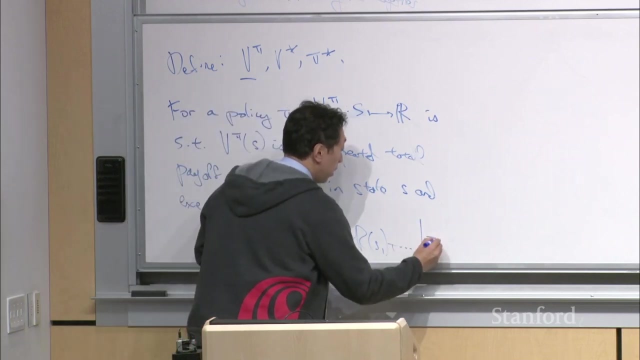 um is such that V pi of S is the expected total payoff um um for starting in state S and executing pi, And so sometimes you write this as V pi of S is the expected well total payoff, given that you execute. 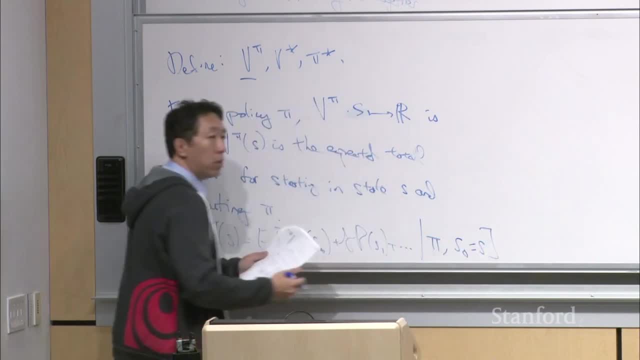 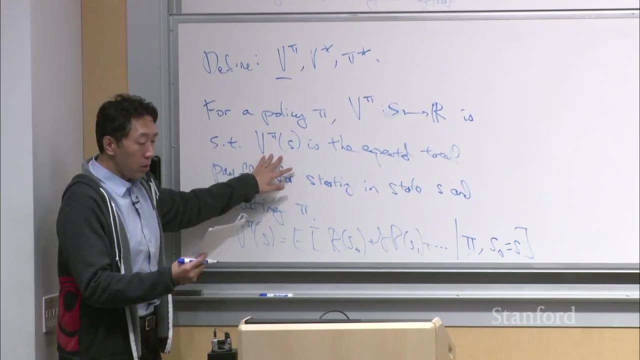 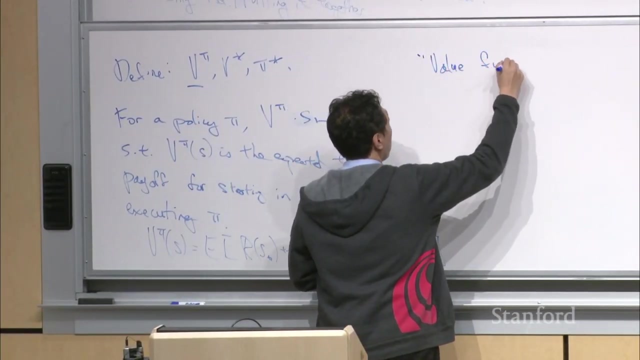 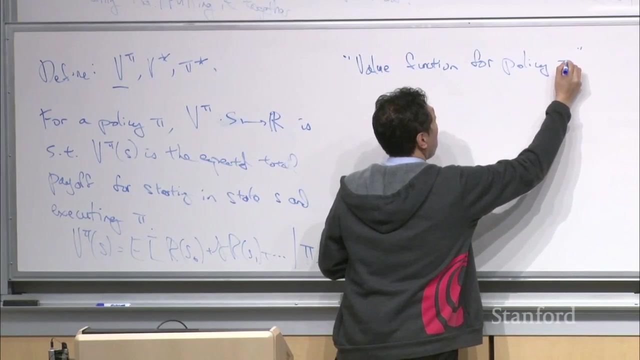 the policy pi and the initial state as zero. As zero is equal to S. okay, So the definition of V pi. this is called the um value function for a policy right. This is called the value function for the policy pi. okay, 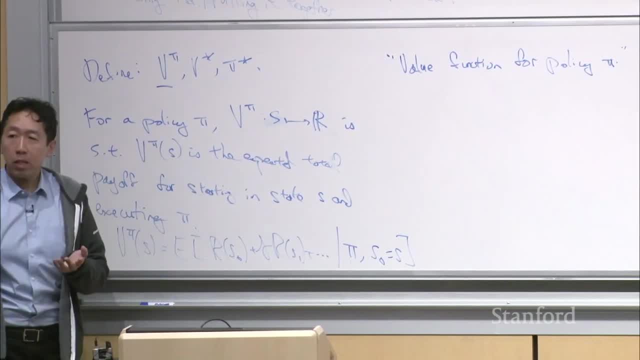 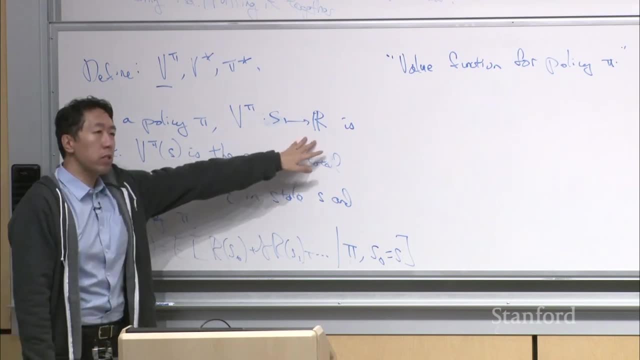 Um and so what the value function for a policy pi, denoted V pi- is is. it tells you um for any state you might start in. there's a function mapping of states to rewards right For any state you might start in. 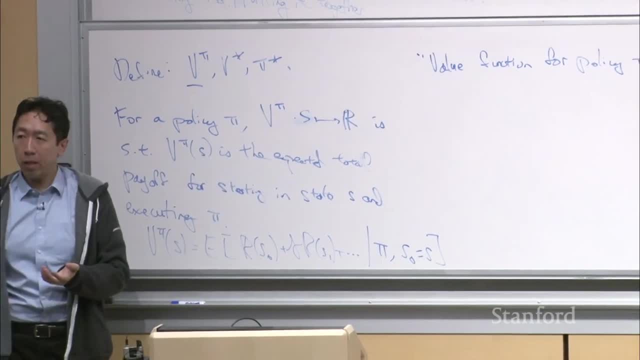 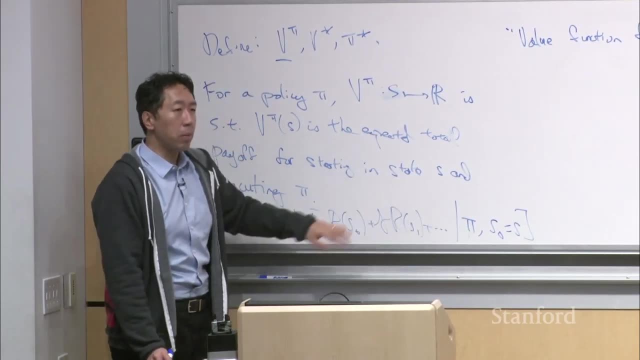 what's your expected total payoff if you start off your robot in that state and if you execute the policy pi? And execute the policy pi means take actions according to the policy pi, right? So here's a- here's a specific example. 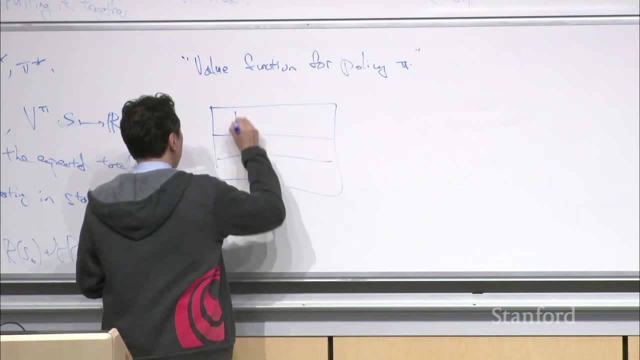 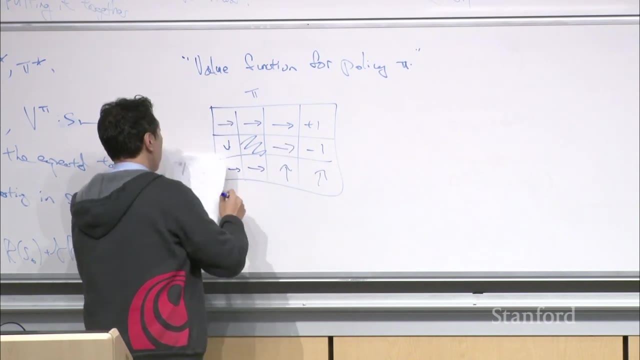 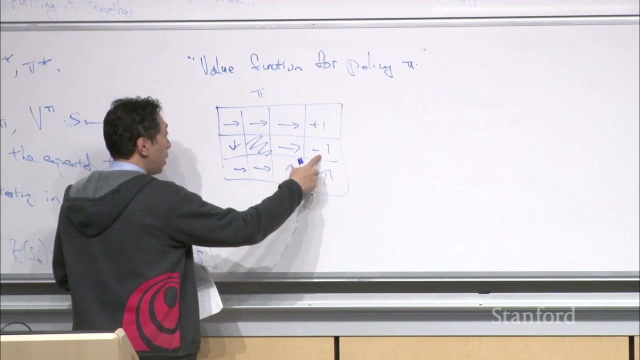 Um this policy, so let's consider following policy pi, right Um? so this is not a great policy, right Um? you know, from some of these states it looks like it's heading to the minus one reward. Oh, sorry. So remember the reward was plus one that we get here. 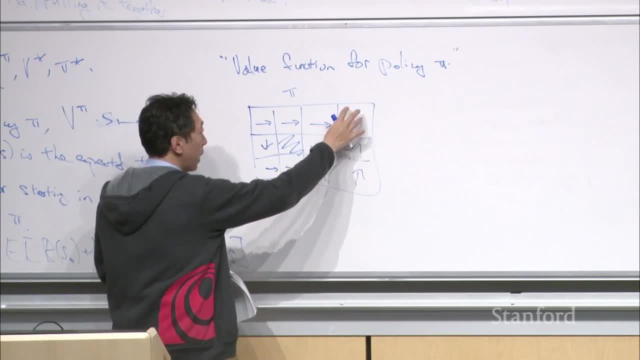 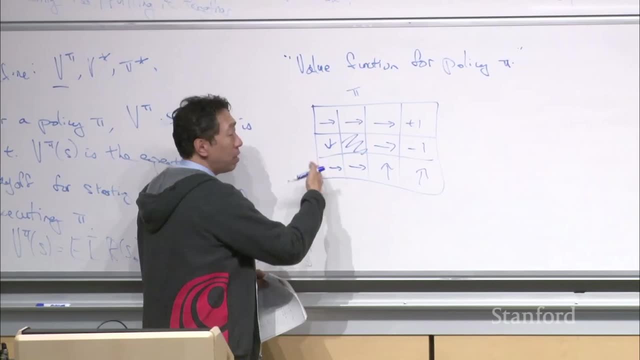 And um, technically this is called an absorbing state, meaning that if you ever get to the plus one, to the minus one, then the world ends and there are no more rewards or penalties after that. right, So-. but so this is actually not a very good policy. 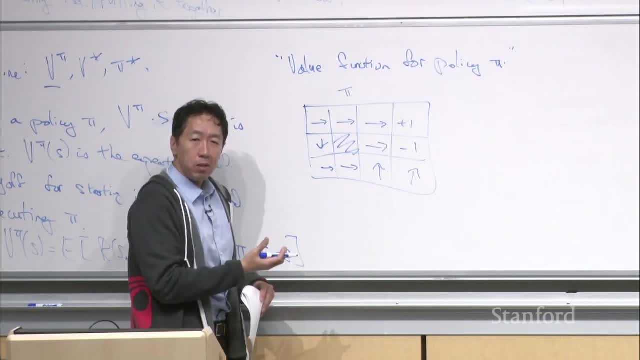 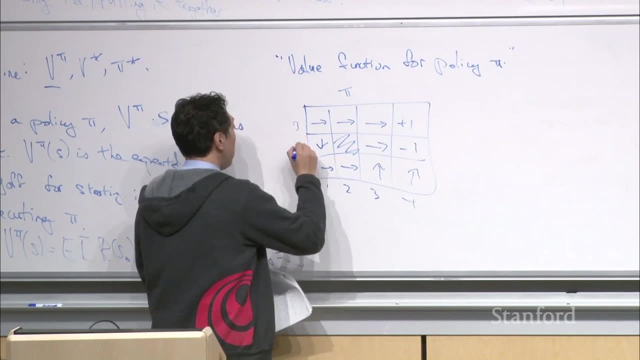 So a policy is any function mapping from the states to the actions. So this is one policy that says, uh, in this state, you know, this policy tells you, in this state, for one go null, which is actually a pretty bad thing to do, right, 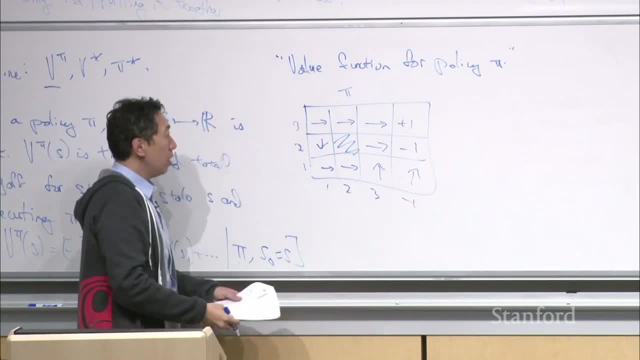 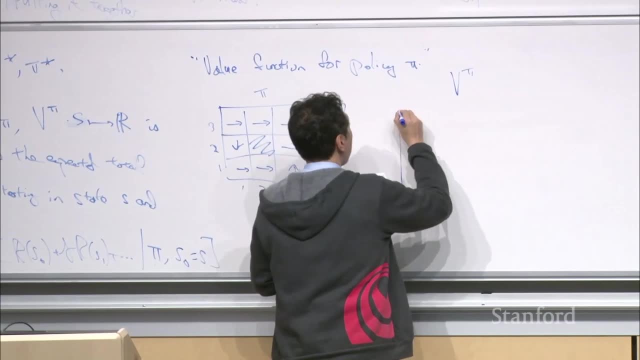 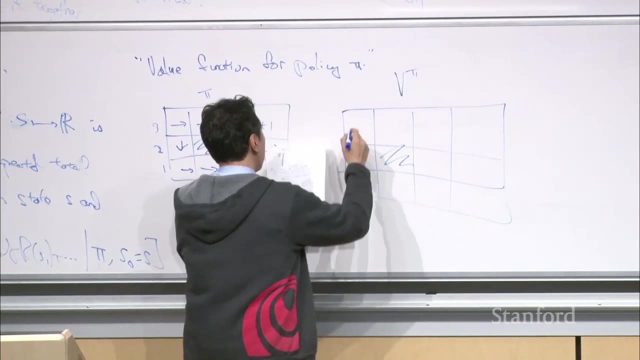 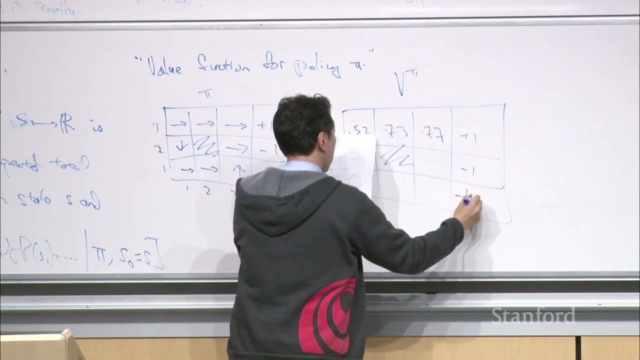 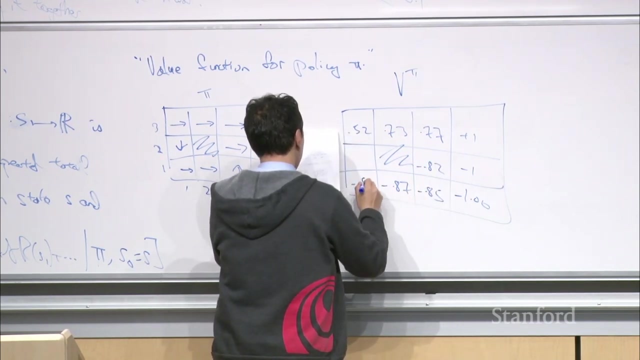 It's taking you to the minus one reward. So this is not a great policy. Um, but- but- but this is just a policy And v? pi for this policy. um looks like this, right? Um? don't worry too much about the specific numbers. 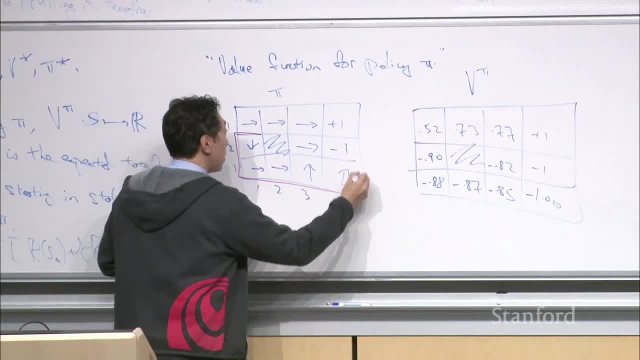 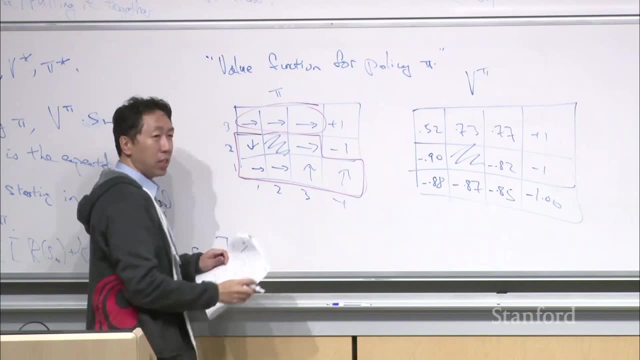 But you know, if you look at this policy, you see that from this set of states it's pretty efficient at getting you to the really bad uh reward, And from this set of states it's pretty efficient at getting you to the good reward right. 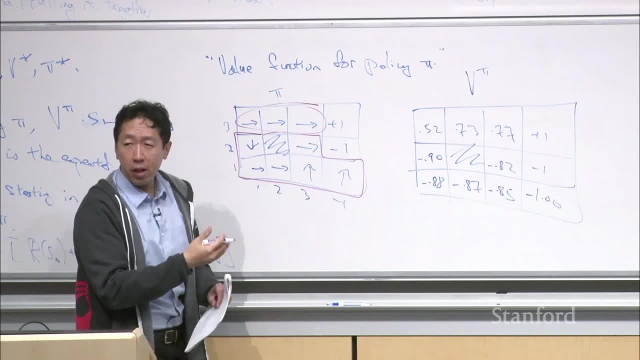 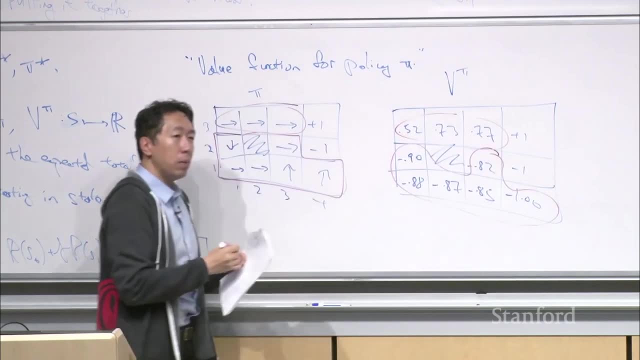 With some mixing because of the noise in the robot veering off to the side. And so you know, these numbers are all negative and those numbers are at least somewhat positive, right So-. but so v pi is just um if you start from say: 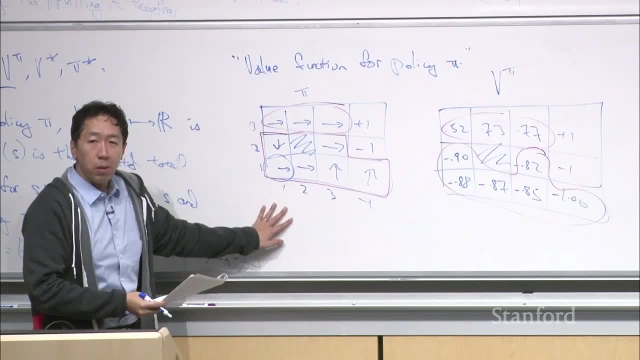 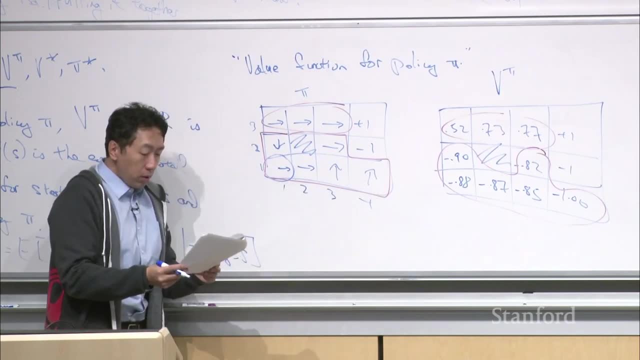 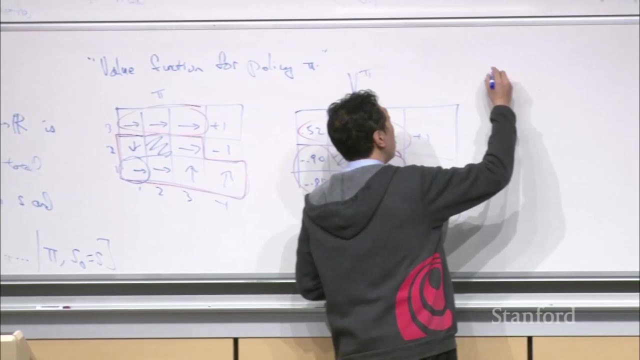 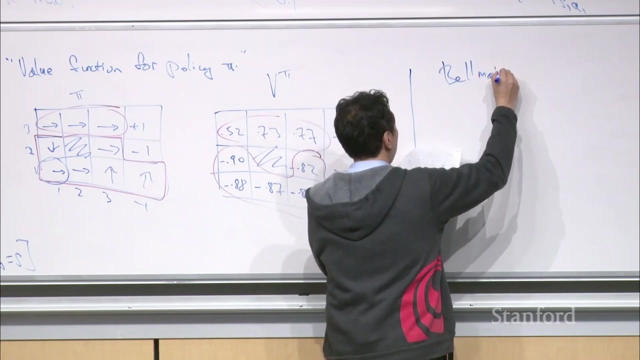 this state from the state 1, 1, on expectation, you're expected some of this. counter rewards will be negative. point 8, 8.. Okay, Um, so that's what v pi is right Now, um. 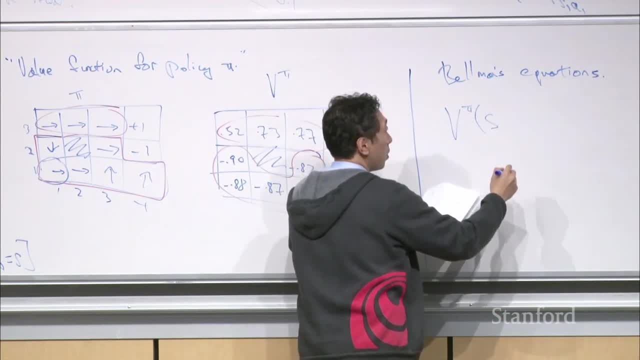 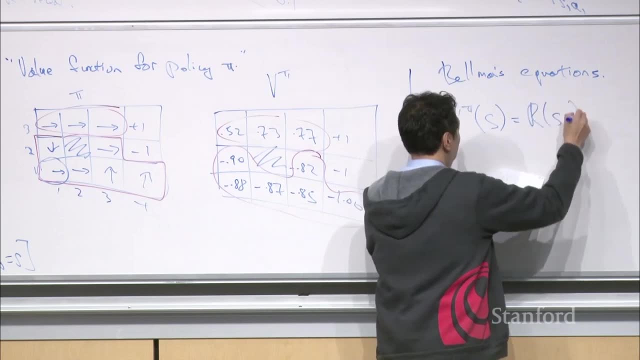 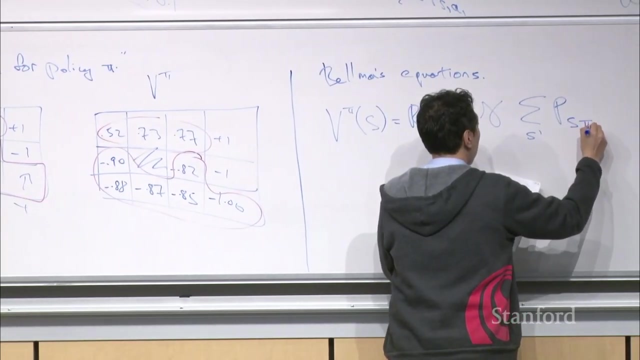 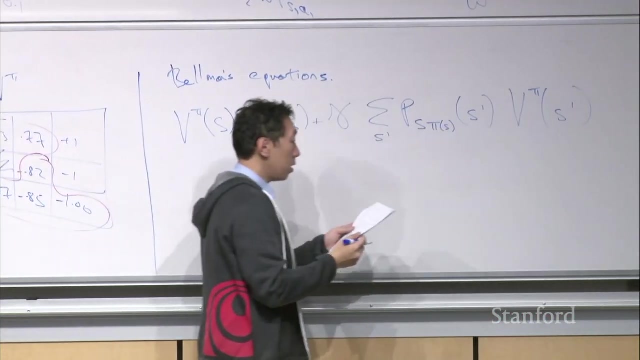 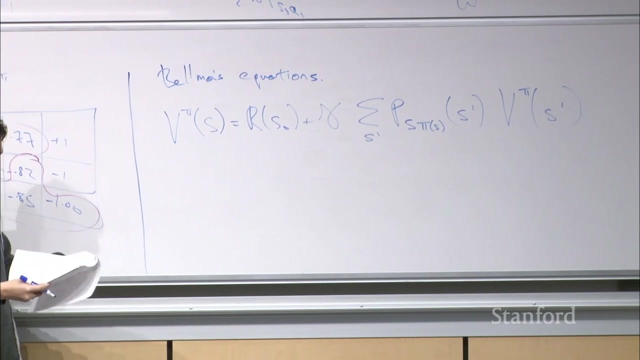 the following equation: let me think uh governs um the value function. right, It's called uh. it's called uh. Bellman's equation Um, and this says that your expected payoff at a given state is. 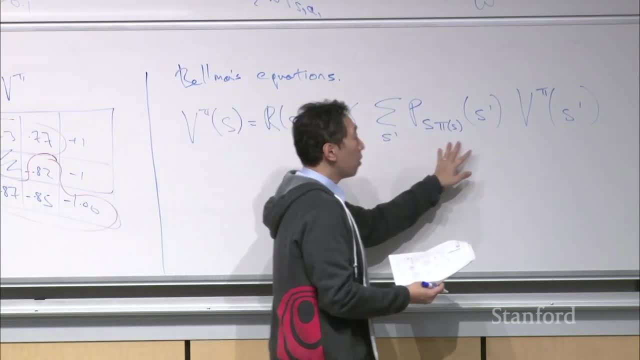 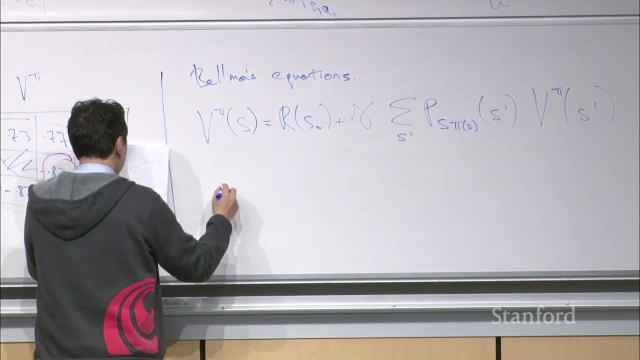 the reward that you receive, plus the discount factor times the future reward. So let me- let me actually explain um the intuition behind this right, Which is that, um let's say, you start off at some state s0, right. 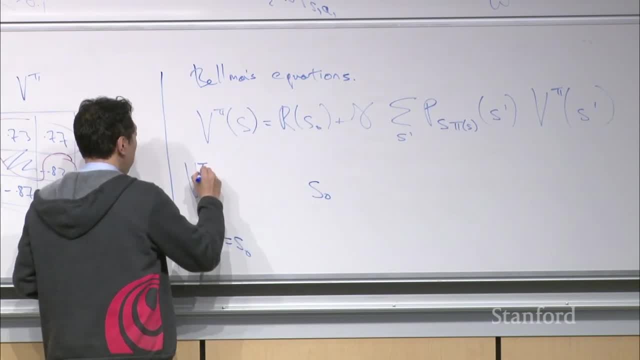 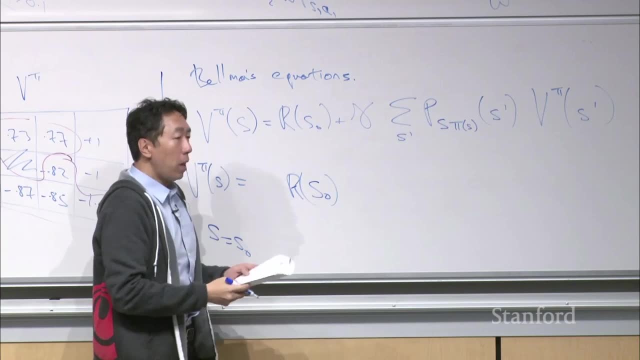 So- oh, and again, let's- let's say s is equal to s0, right? So v pi of s is equal to well, just for your robot waking up in that- I'm- I'm gonna add it in a second, okay. 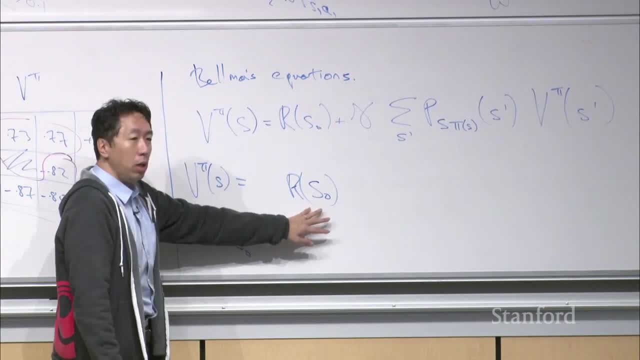 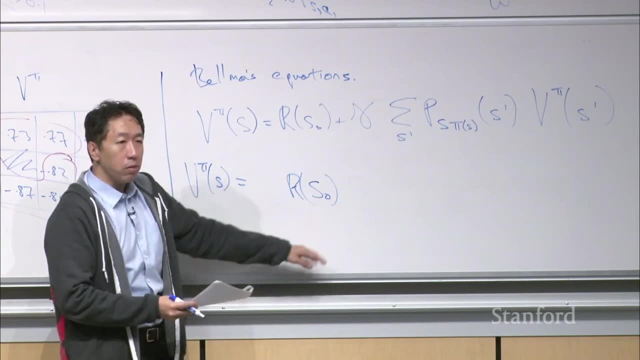 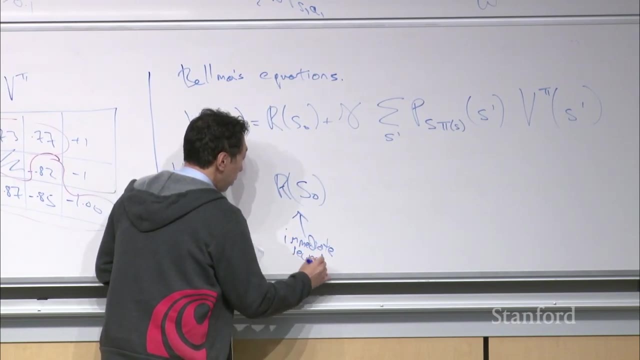 But just for the sake of you know, take- just for this- for the fact that your robot woke up, um, in this state S you get the immediate- you get the reward R of S zero right away. Uh, this is something that's called- this is also called the immediate reward, right. 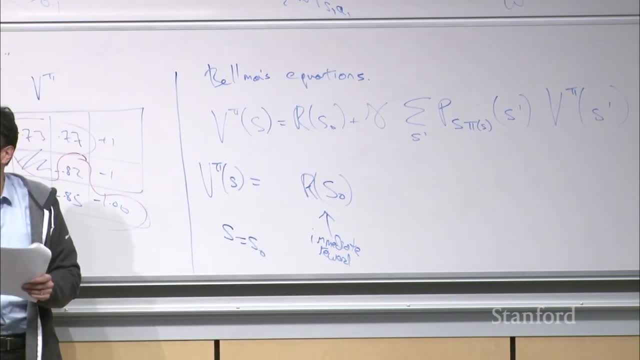 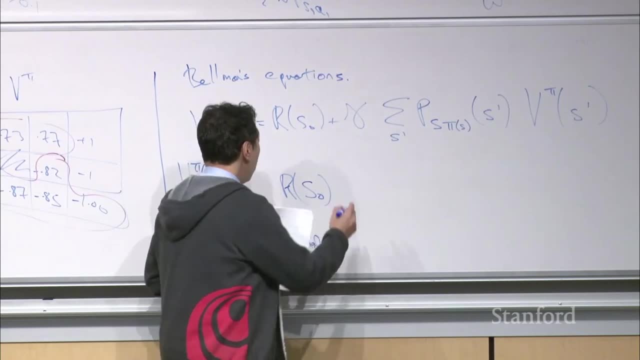 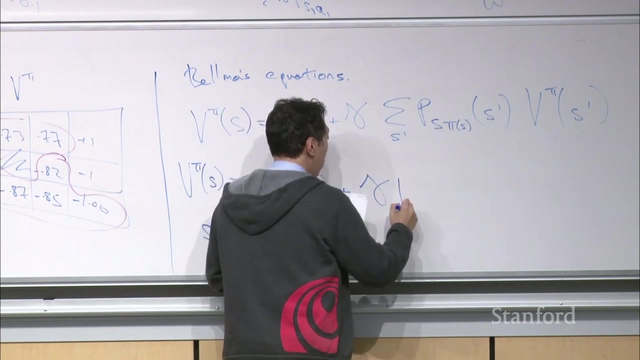 Uh, because you know, just for the- for the uh good fortune or bad fortune of starting off in this state, the robot gets a reward right away- This is called the immediate reward- And then it will take some action and get to some new state S1,. 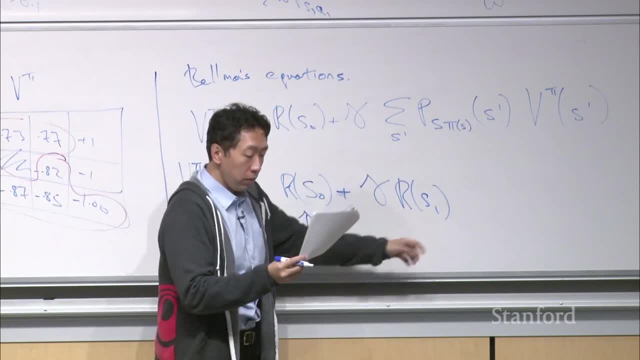 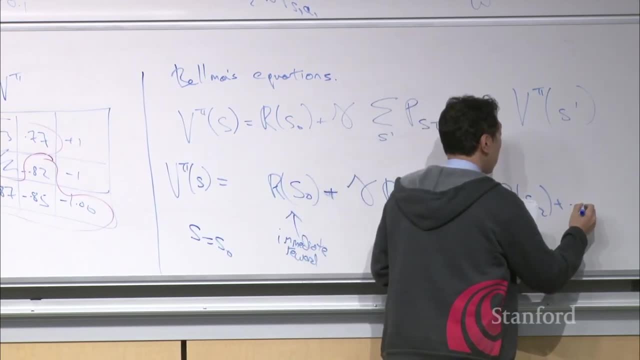 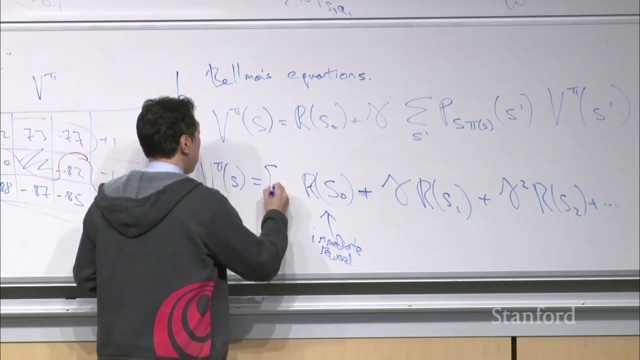 where I'll receive, you know, Gamma times- the reward of S1. And then- right, And then I'll get some future reward at the next step, and so on. Um, and just to flesh out the definition, the value function V, pi is really. 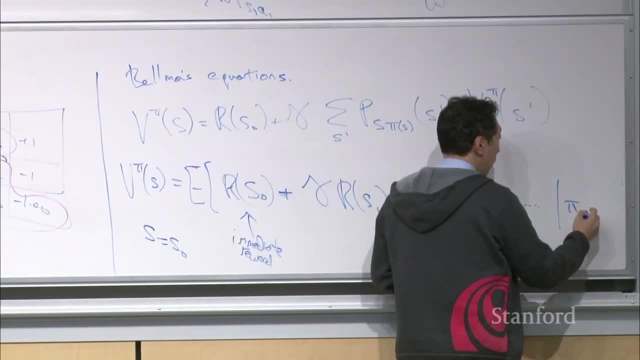 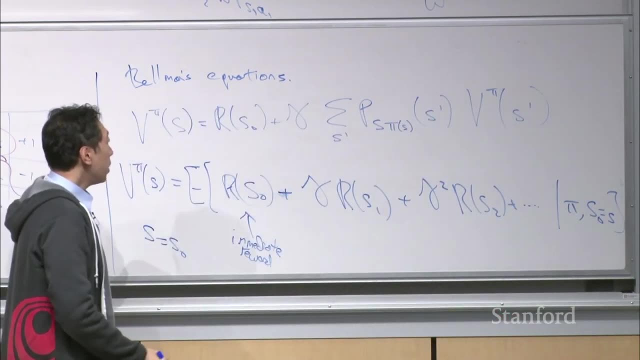 this: given that you execute the policy, pi and uh S uh. zero equals S right, And you start off in the state S zero. Now what I'm going to do is rewrite this part of the equation a little bit. 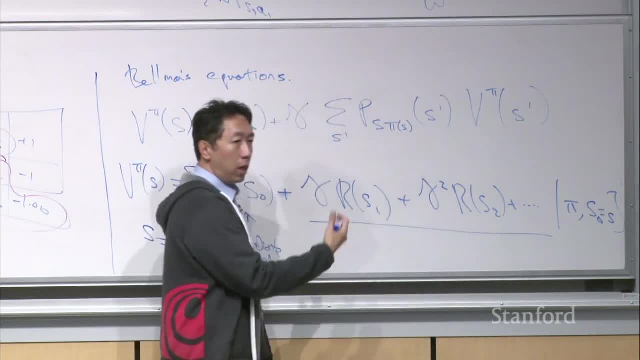 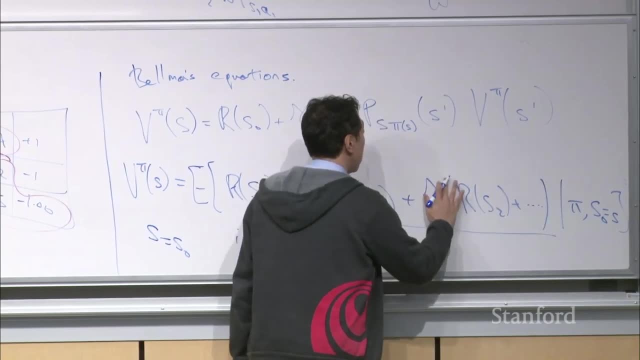 I'm going to factor out- I'm just gonna take the rest of this and factor out one factor of Gamma. So let me put parentheses around this, right, And just check out Gamma there. okay, So I'm just, you know, taking this previously. this was. 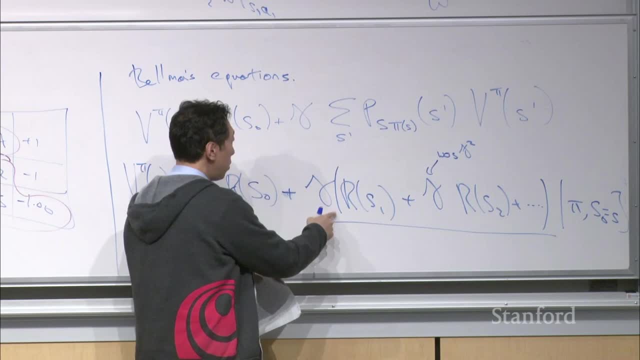 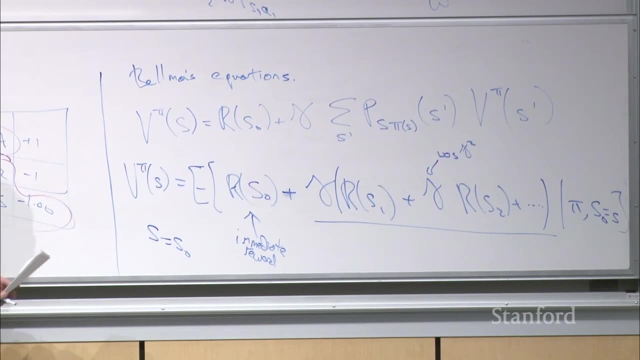 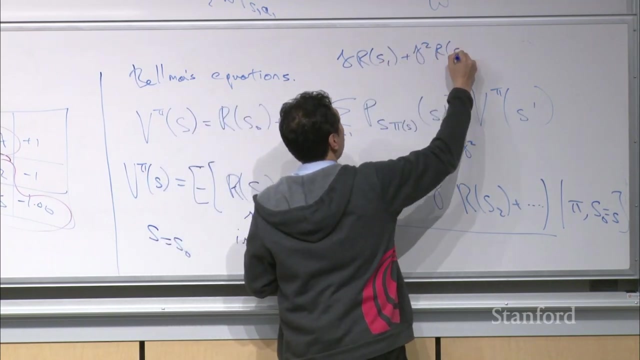 uh, Gamma squared right, But adding the parentheses here. I'm just taking out one factor of Gamma. uh, uh, that multiplies in the rest of that equation. okay, Does that make sense? No, So as in Gamma R of S1 plus Gamma squared R of S2 plus dot. 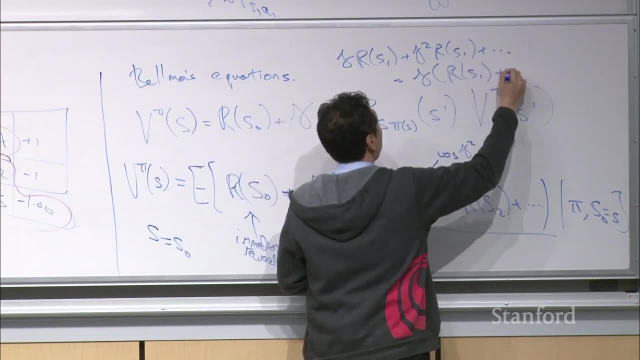 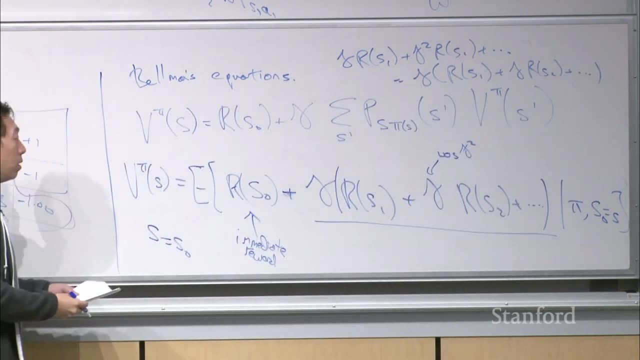 dot dot equals Gamma times R of S1 plus. okay, So that's- that's what I did down there, right, Just factor out one- one factor of Gamma, And so, um, this is the- the value of state S is: 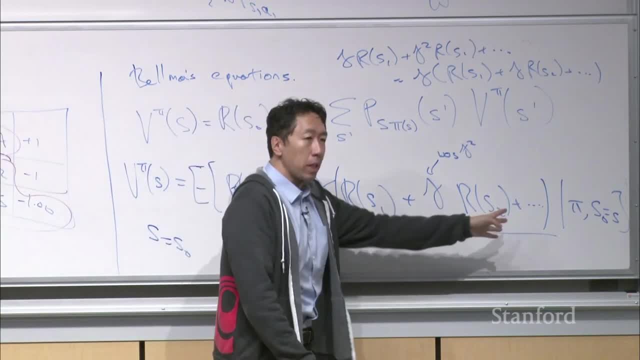 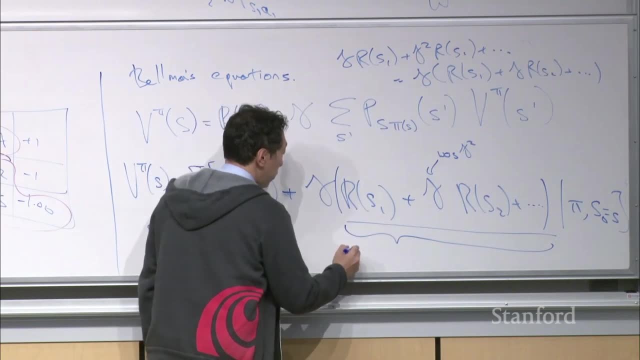 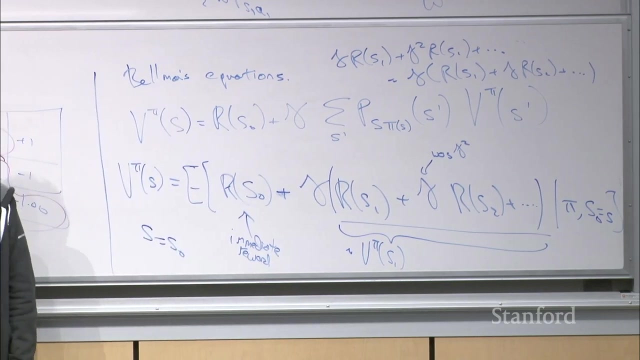 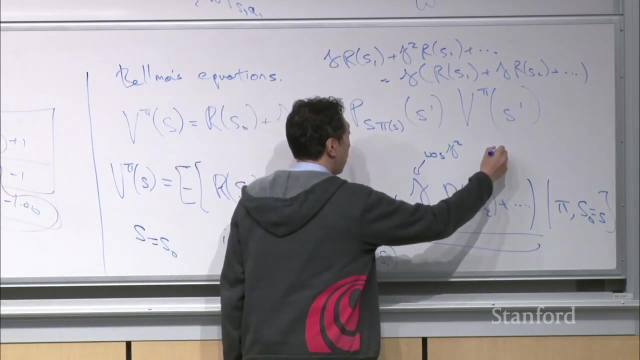 the immediate reward plus Gamma times the expected future rewards. right, So this. the expected value of this is really V Pi of S1, right, Um, so this- and- and so the second term here, this- this is the uh. 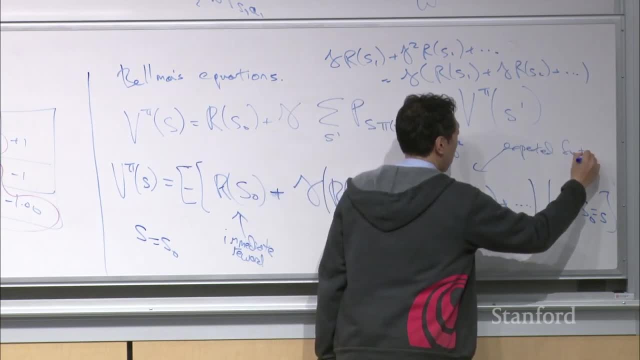 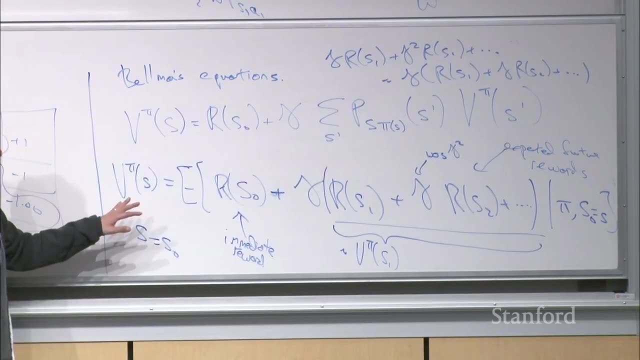 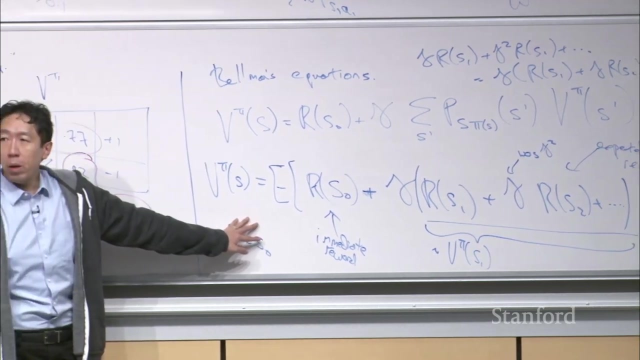 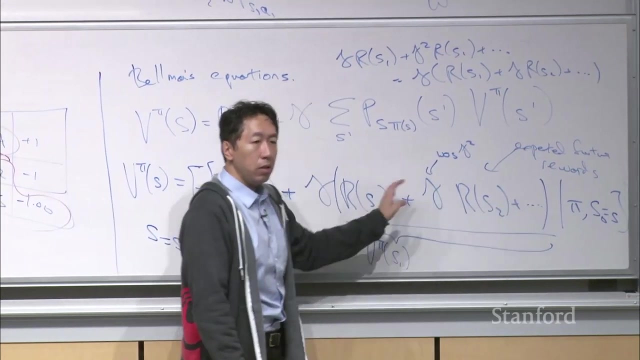 expected future rewards right. So Bellman's equation says that, um the value of a state, the value, the expected total payoff you get if your robot wakes up in the state S is the immediate reward plus Gamma times the expected future rewards. okay, 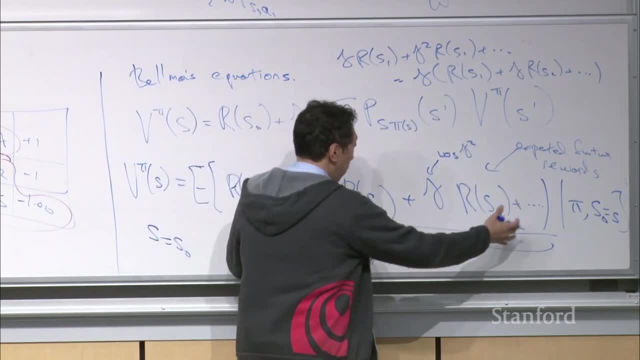 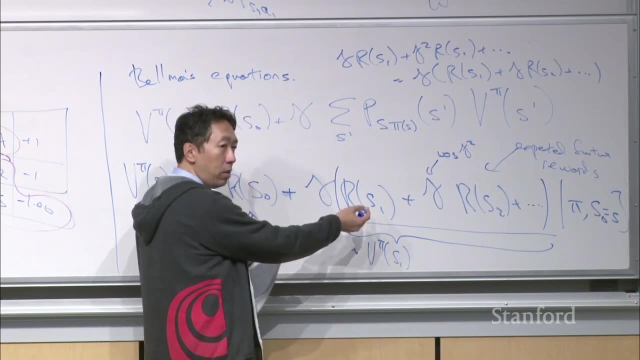 Right, And-. and This thing under, you know, above the curly braces, is really, um, uh, asking: if your robot wakes up at the state S1 and executes pi, what is the expected total payoff? right, Uh, and this- what if your robot wakes up in the state S1,? 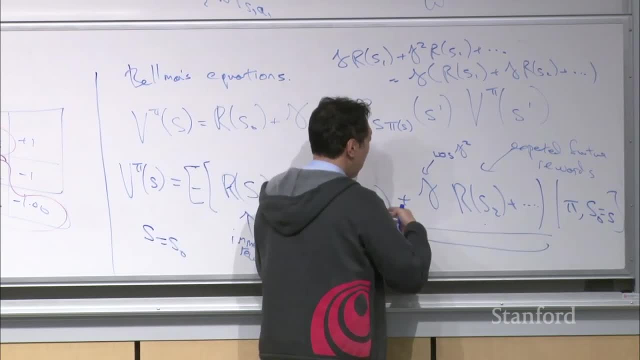 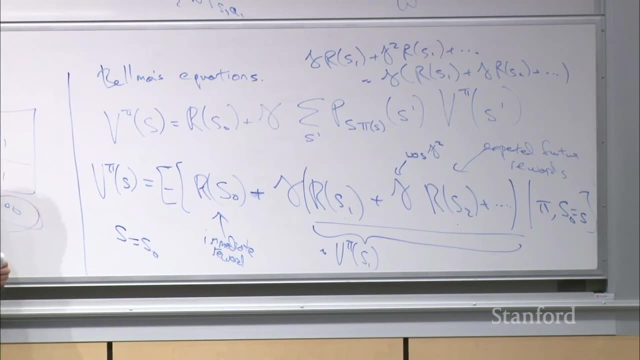 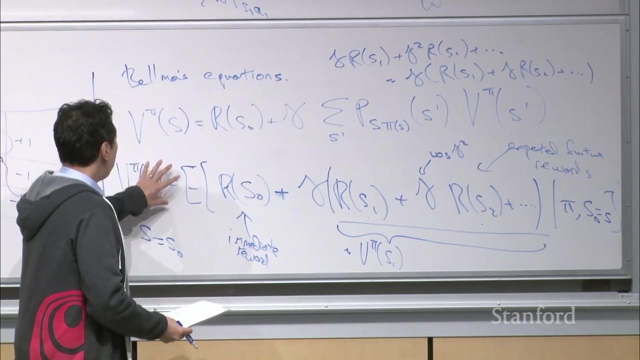 then it'll take an action, gets S2,. take an action, get to S3, and this- this is the sum of this- counter awards where it starts off in the state: S1.. Okay, Make sense. So, um, uh, this. 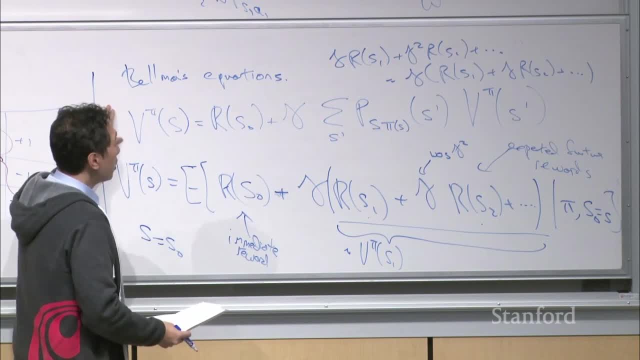 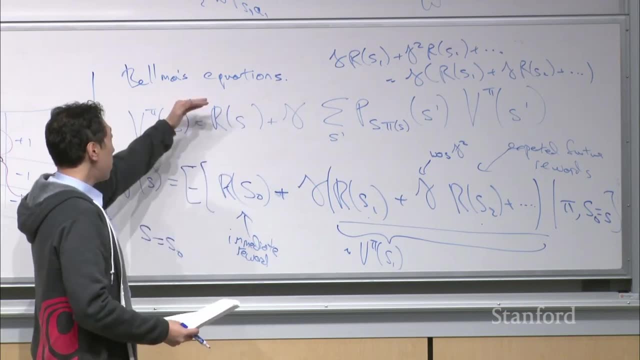 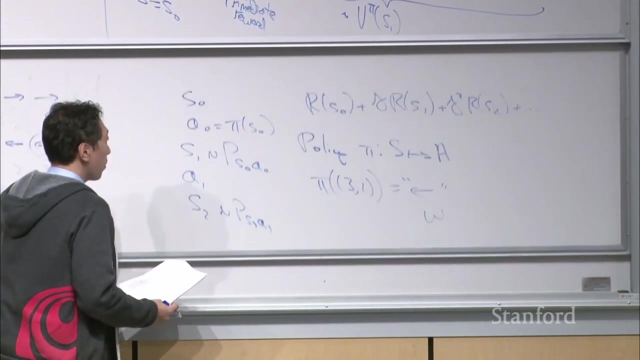 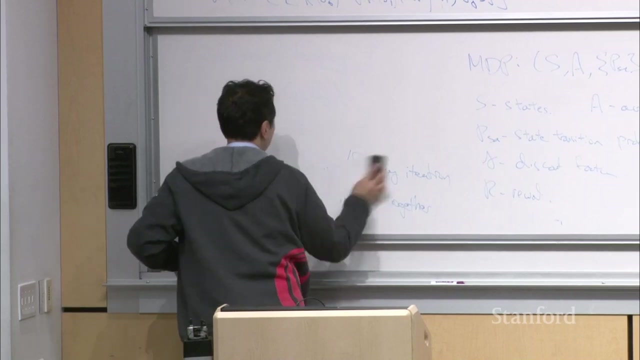 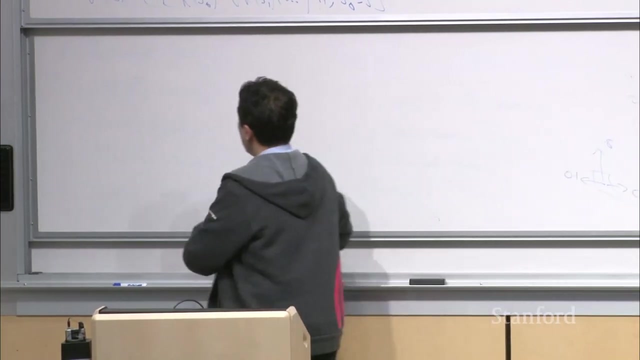 based on this, you can write out: well, let's justify Bellman's equations, which is: um, oh and uh, excuse me, and the mapping from this equation to this equation. All right, Yeah, The mapping from the equation on top to the equation at the bottom is: 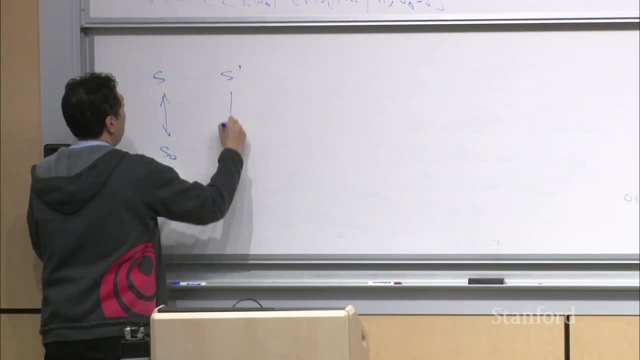 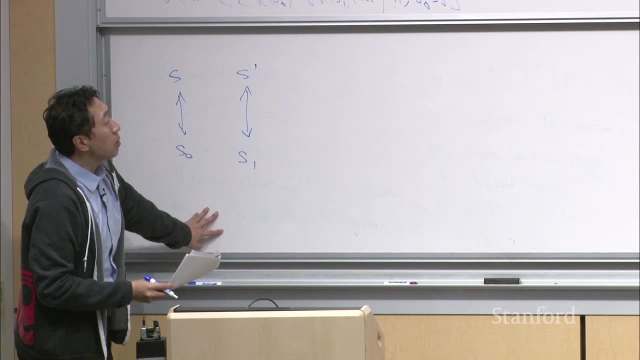 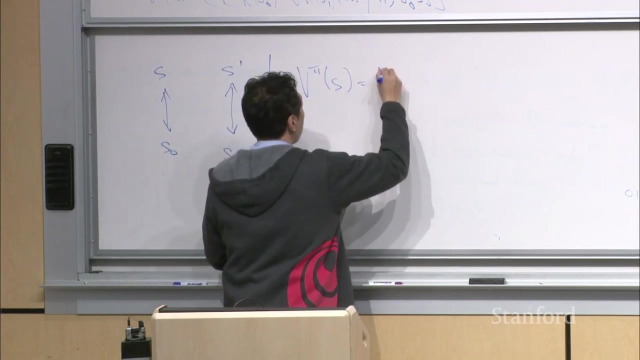 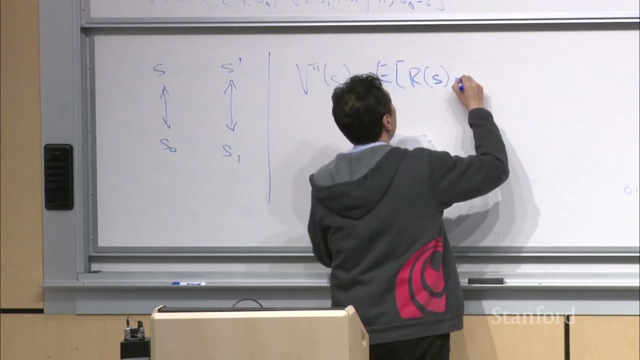 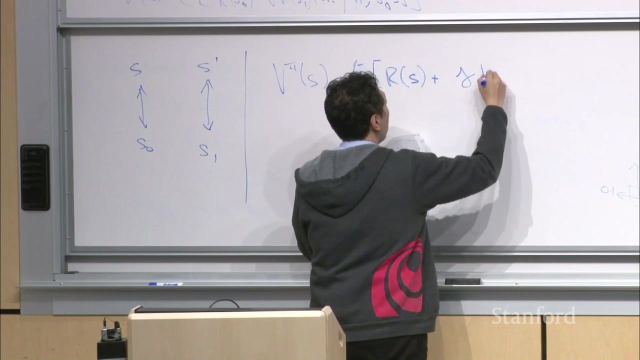 that S maps to S0 and S prime maps to S1, right, Um, and uh, um, right, And so if we have that V pi of S equals right, Okay, Okay, Okay, Okay, Okay, Um, does that make sense? 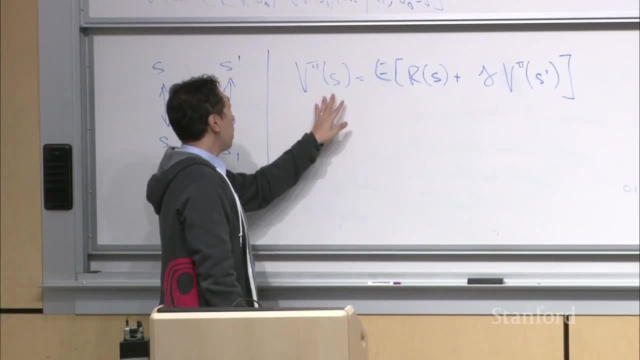 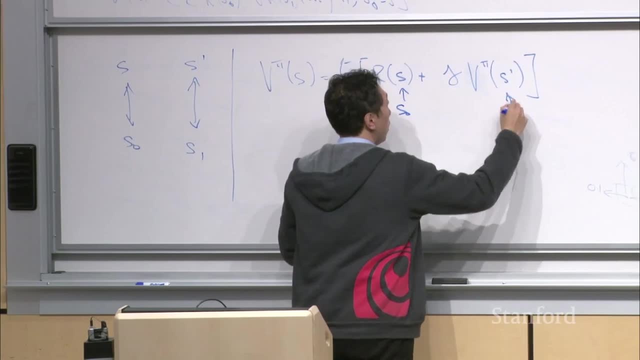 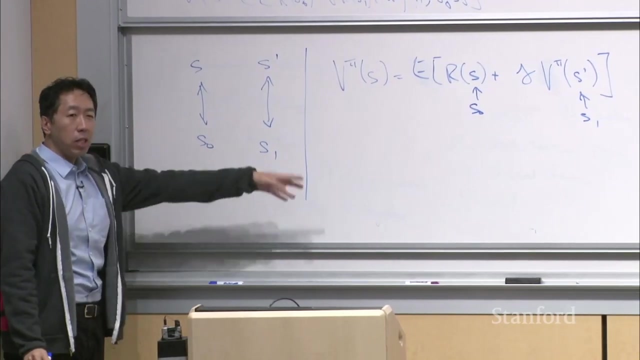 All right. So the value of um state S is uh R of S plus V pi of S prime, where this is really S zero, And this is S1.. Um and- and in the notation for MDP, if you want to write a long sequence of states. 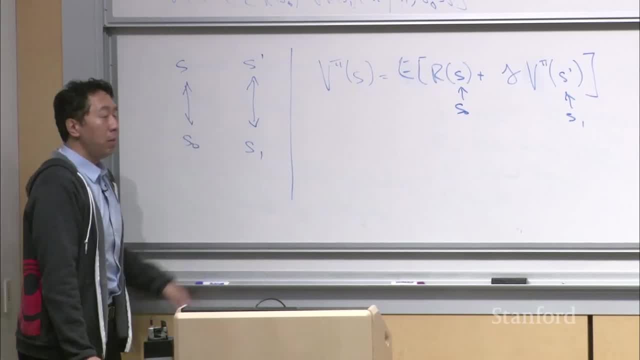 we tend to use S zero, S1,, S2, S3, and S4, and so on. But if you have- want to look at just the current state and the state you get to after one time step, we tend to use S and S prime for that. 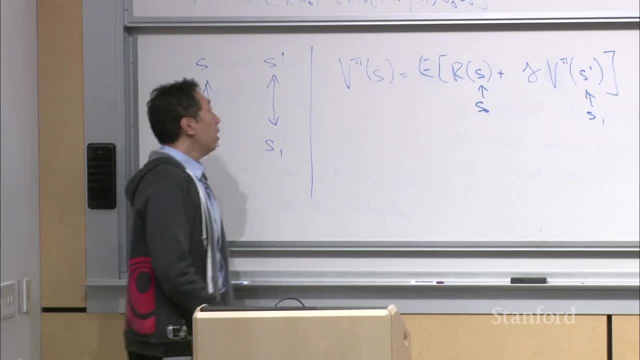 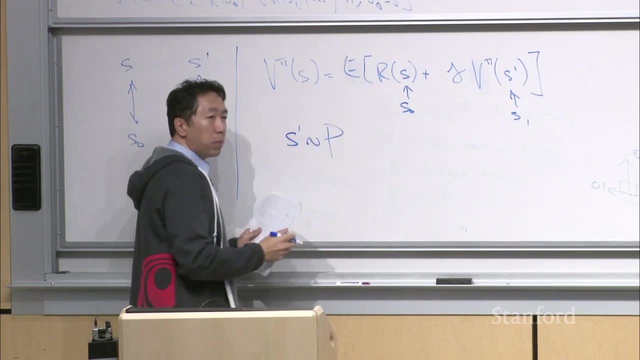 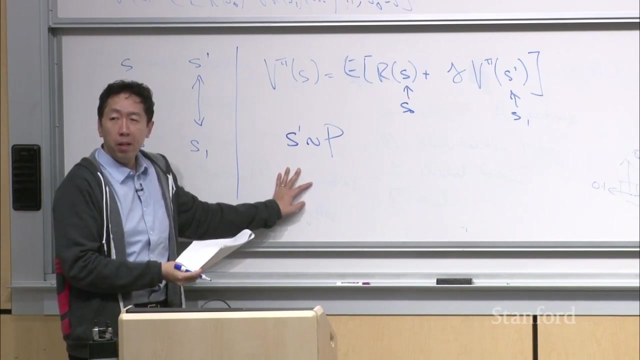 So that's why there's this mapping between these two pieces of notation. Uh, so if S prime is, say, you get to after one step, well, let's see what is S prime drawn from right. This- so the-, the- the- the state S prime or S1 is the state you get to after one time step. 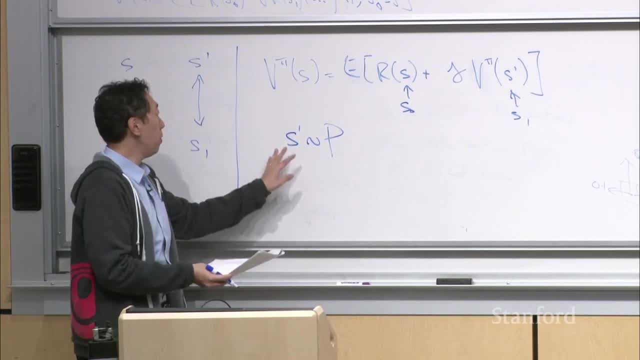 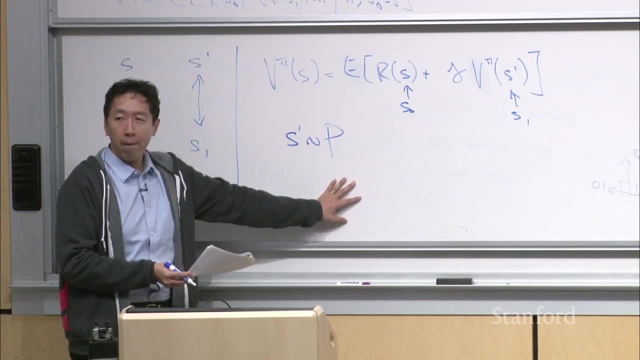 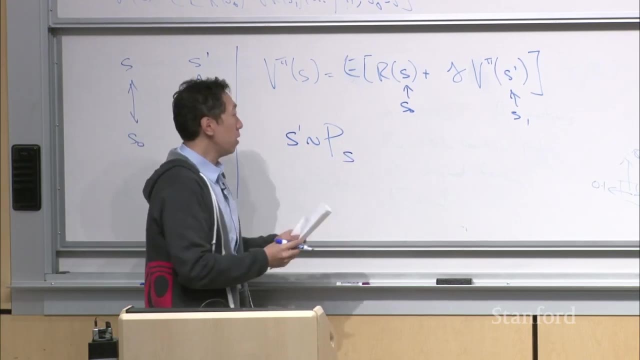 So what is- what is the distribution that S prime is drawn from? S prime is drawn from P of what? Yep, Okay, P of S and then pi of S. right Cool, Does that make sense? Because, um, in state S. 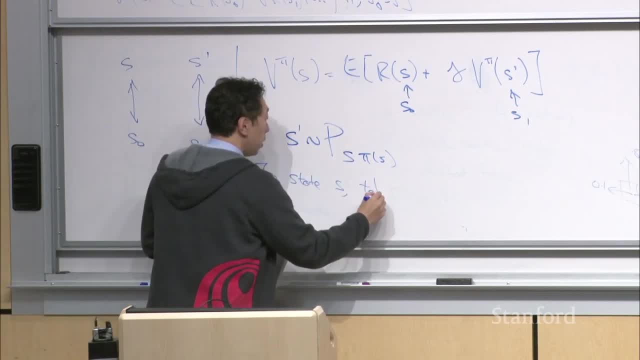 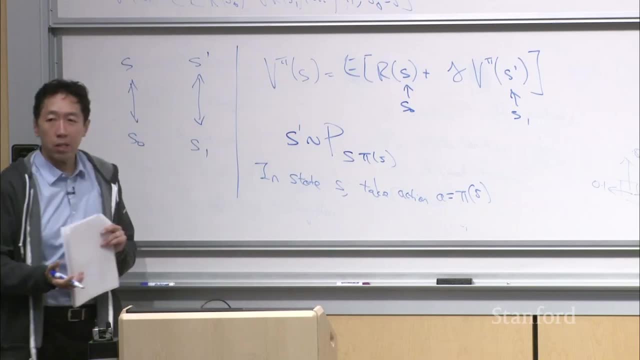 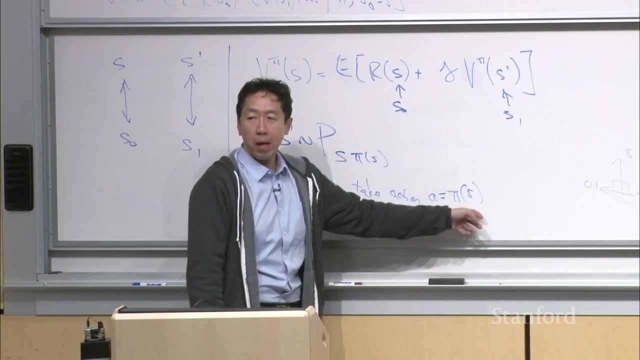 you will take action A equals pi of S, right, So we're executing the policy pi. So that means that when you're in a state S, you're gonna take the action A given by pi of S, because pi- pi of S tells you: please take this action A when you're in state S. 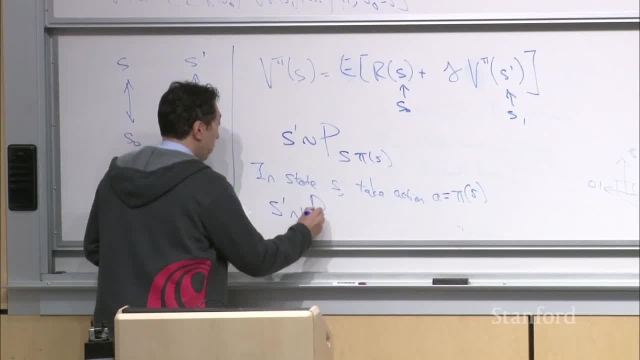 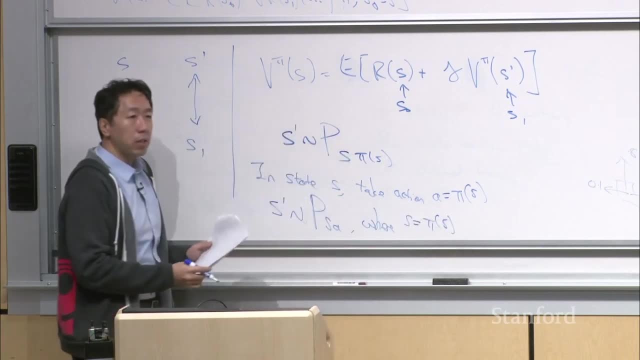 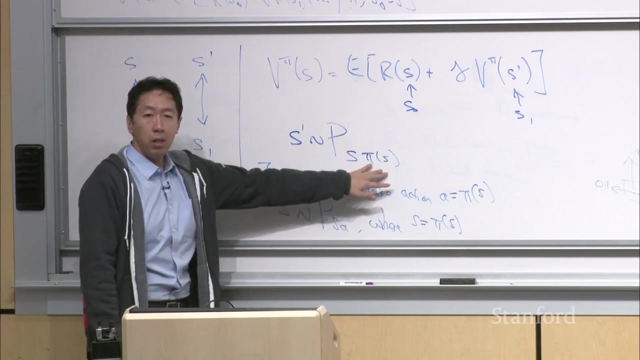 And so um S prime is drawn from P of S A, where A is equal to pi of S Right. Because- because that's the action you took, which is why S prime- the state you get to after one time step- is drawn from the distribution S pi of S. Okay. 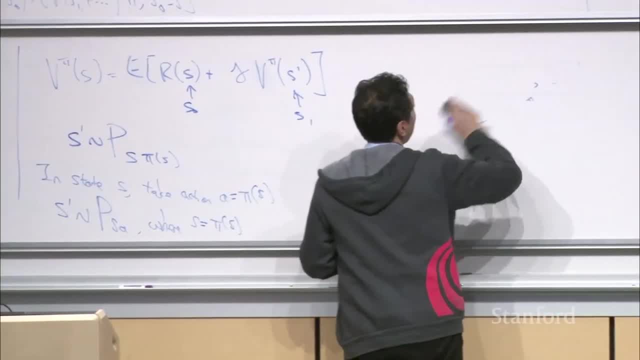 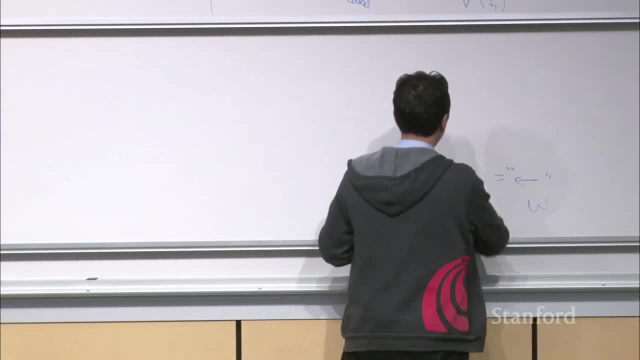 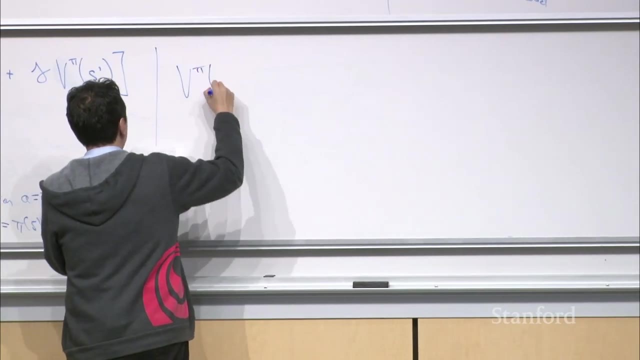 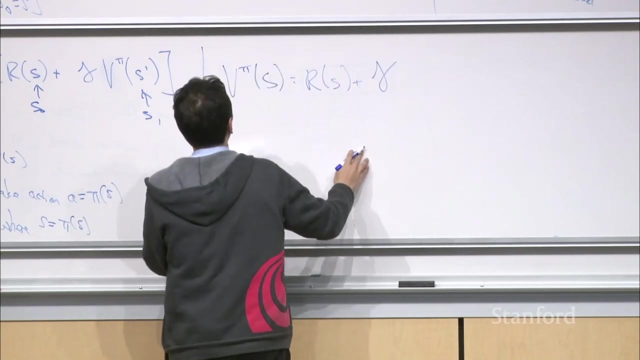 Wow, that pen really left a mark. So putting all that together, that's why- well, I'll just write that again. where Bellman's equations, which is um v- pi of S equals R of S plus the discount factor times the expected value of v-pi of S prime. 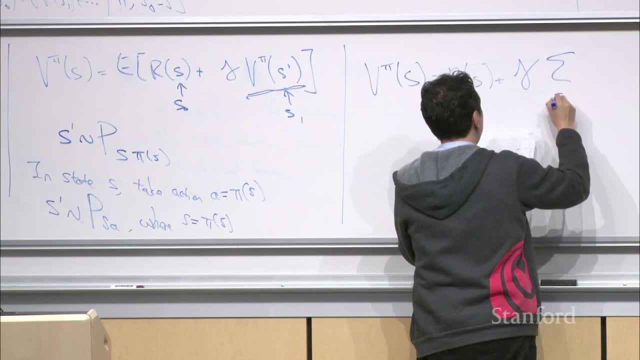 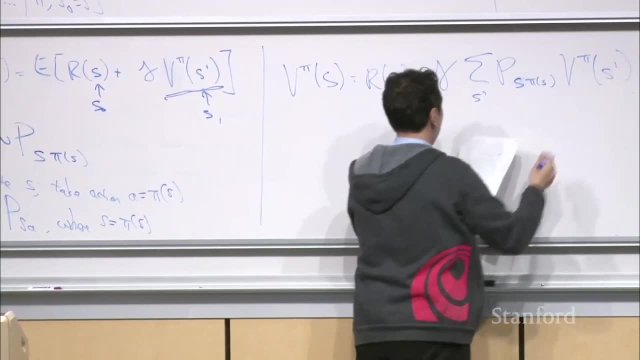 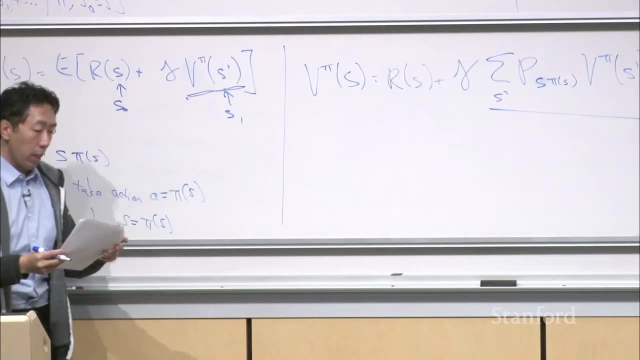 and so this term here is just sum over S prime, V S pi of S, v- pi of S prime. Okay, So that underlying term I guess is- is this underlying term here? Okay, Um, now-. now. now I was just, I was just thinking about one more thing on- okay. 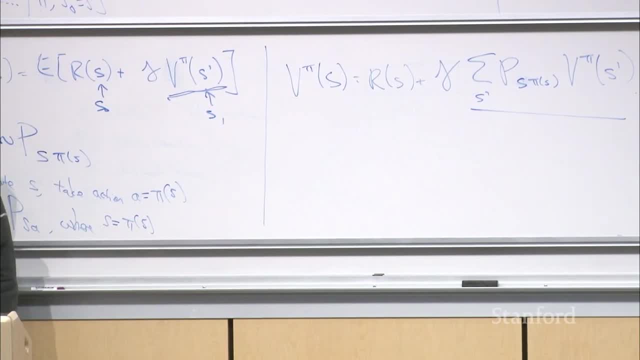 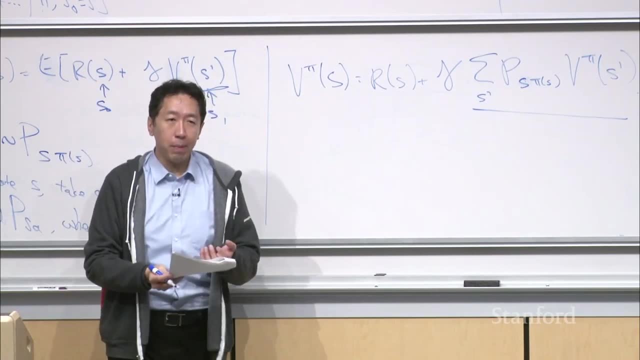 Now notice that this gives you a linear system of equations for actually solving for the value function. Um. so let's say I give you a policy, right, It could be a good policy, it could be a bad policy. and you want to solve for v, pi of s? 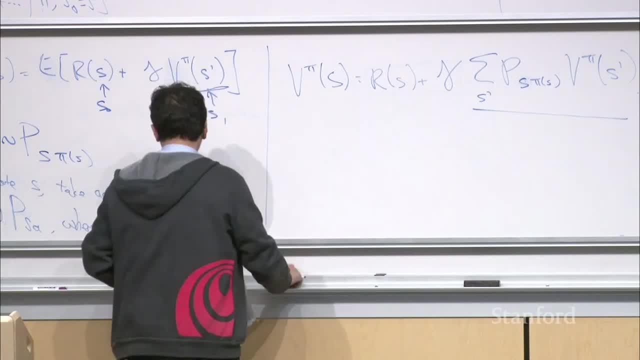 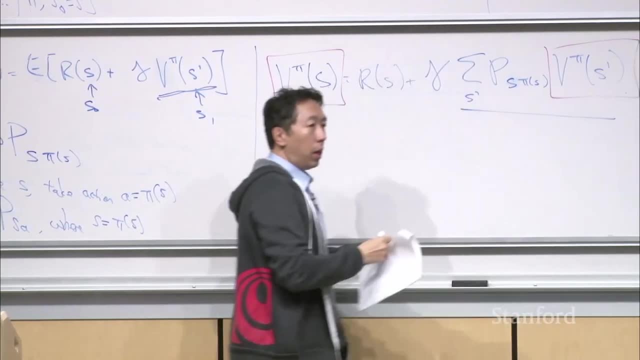 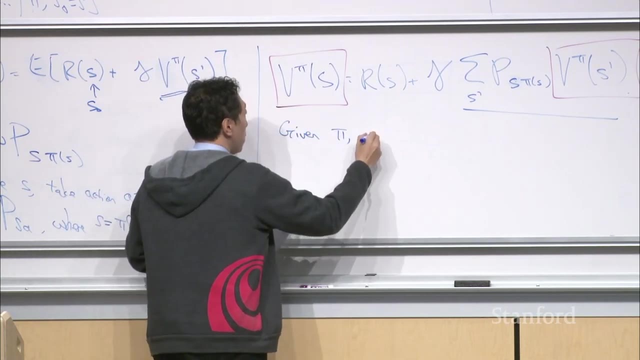 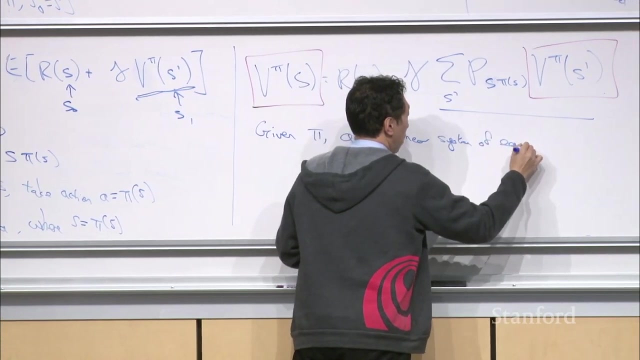 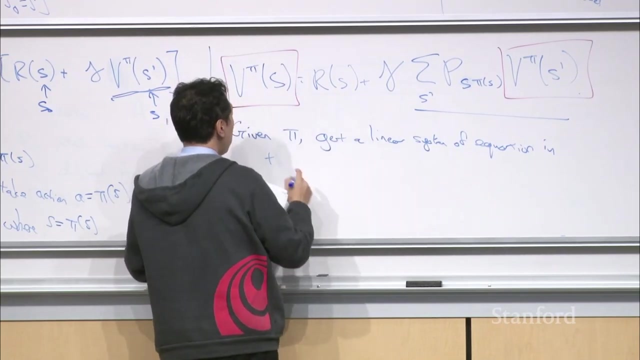 What this um does is, if you think of v, pi of s as the unknowns you're trying to solve for um given pi right, These equations, um, these equa- Bellman's equations, defines a linear system of equations. 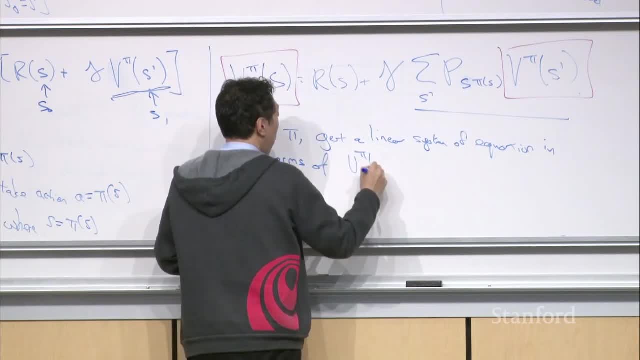 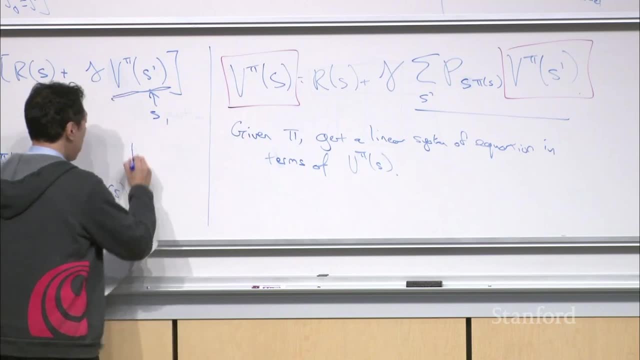 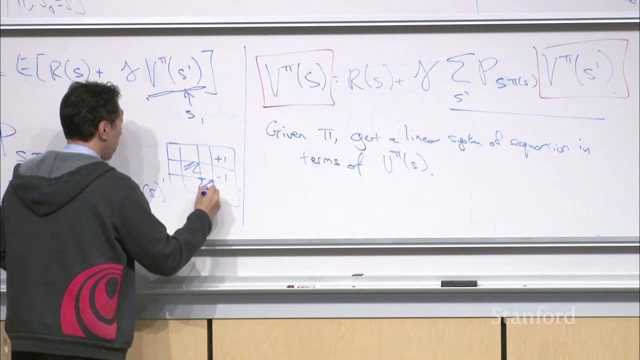 uh, in terms of v pi of s as the value function of the equation, Uh, values to be solved for. So maybe here's a- here's a specific example. Um, let's take the state v1, right? So this is the state v1, okay. 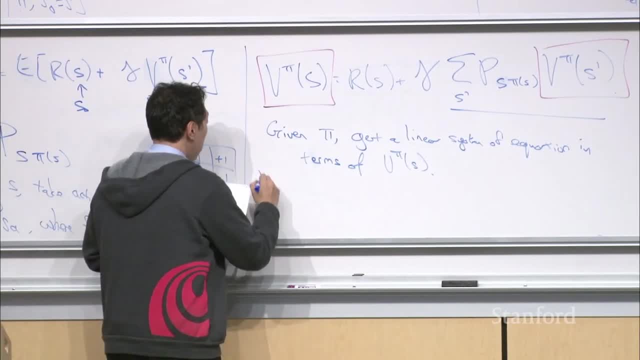 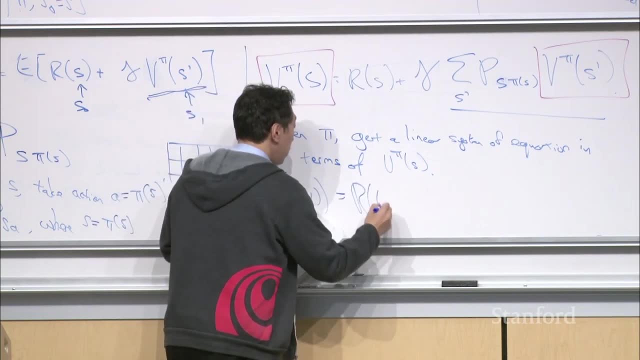 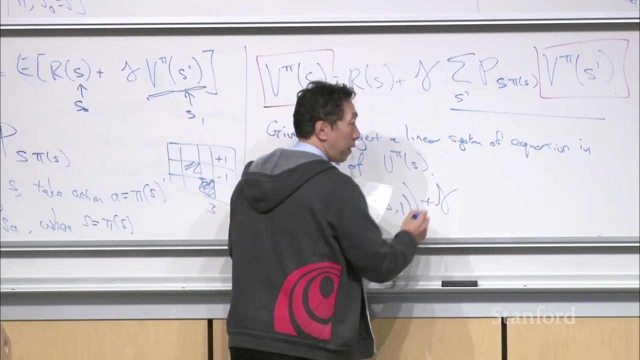 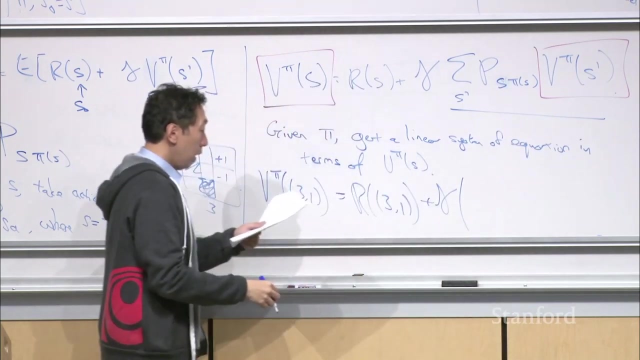 What this- what Bellman's equation tells us, is: v? pi of the state 3,1 is equal to the immediate reward you get at the state 3,1, plus the discount factor times. well, sum of s prime p s pi of s v? pi of s prime right. 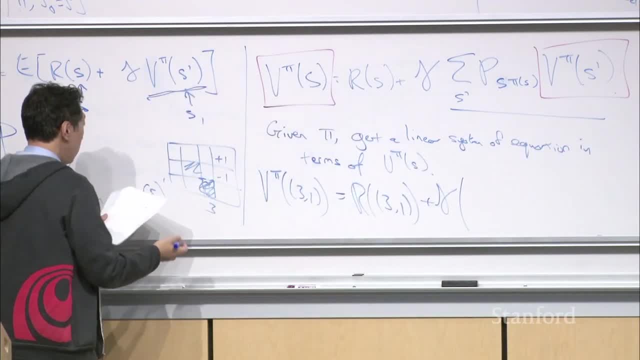 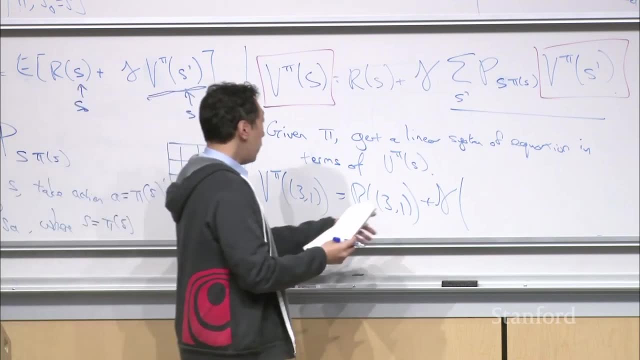 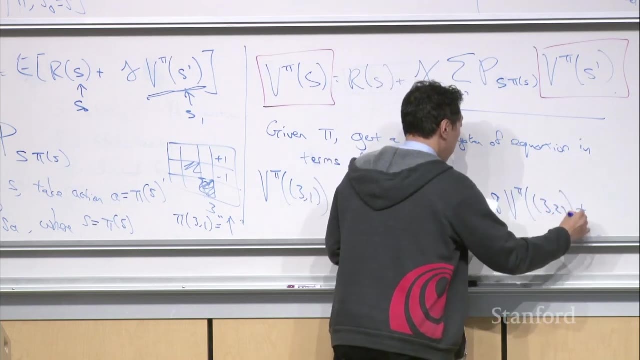 So um, oh and let's see. Uh, let's say that pi of 3,1 is north, right. So let's say you try to go north. If you try to go north from this state, then you have a 0.8 chance of getting to 3,2, plus a 0.1 chance of. 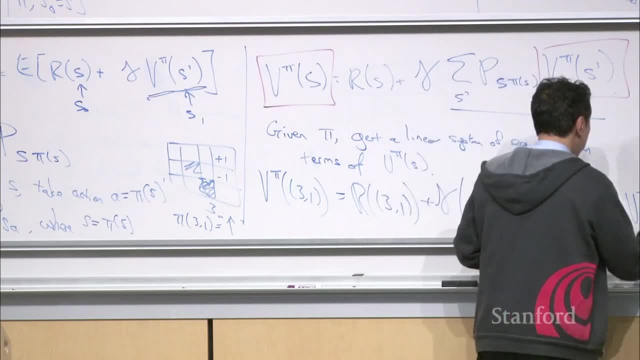 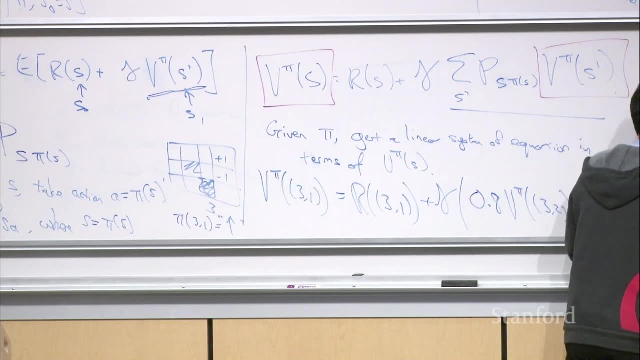 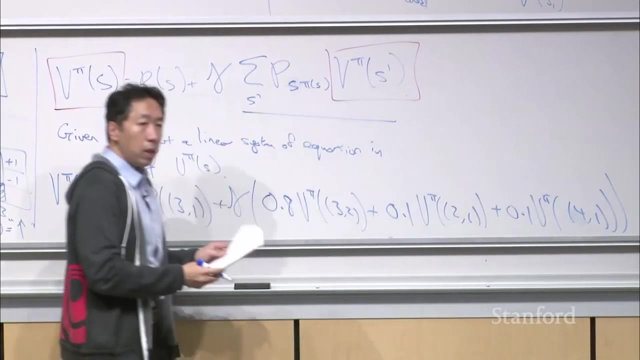 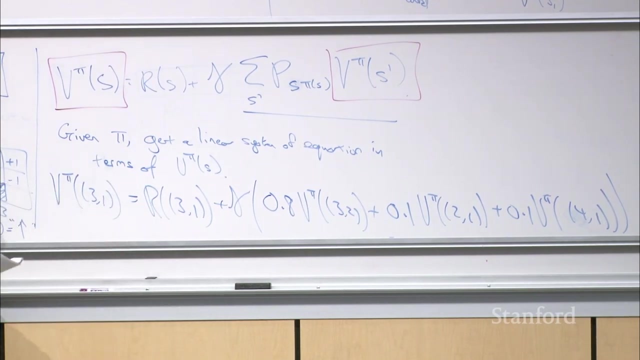 uh, uh, veering uh left, plus a 0.1 chance of veering right. Um, let me just close out that parenthesis. okay, So that's what Bellman's equation says about these values, right? And if your goal is to solve for this, 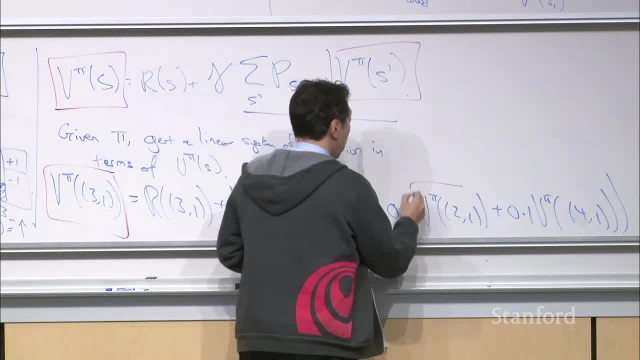 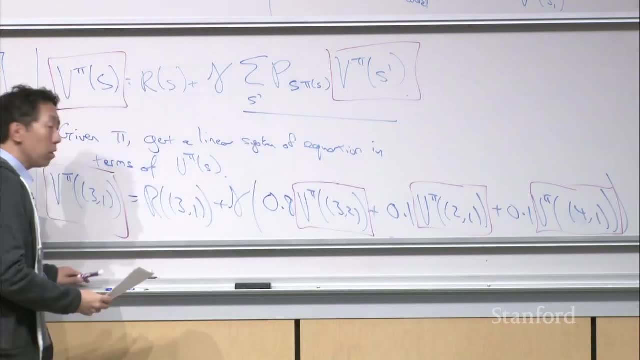 to solve for the value function, then these things I'm just circling in purple are the unknown variables, right And um. if you have 11 states, uh like in our MDP, then this gives you a system of 11 linear equations with 11 unknowns. 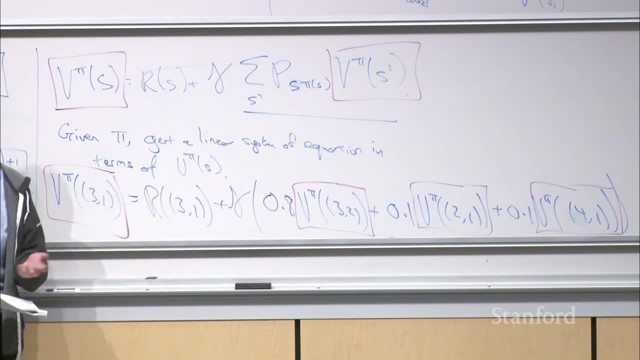 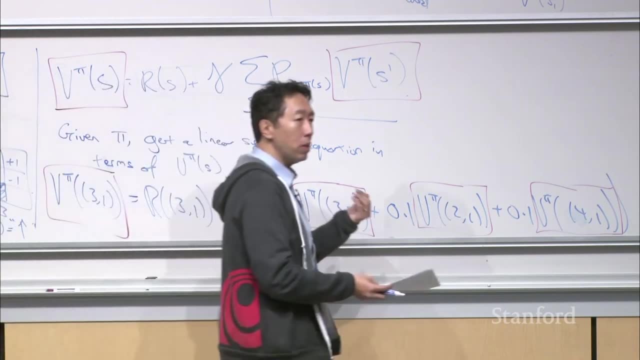 Um, uh, and so using sort of a linear algebra solver, you could solve explicitly for the value of these 11 unknowns. Does that make sense, right? So- so the way you would- so let's say, I give you a policy Pi. 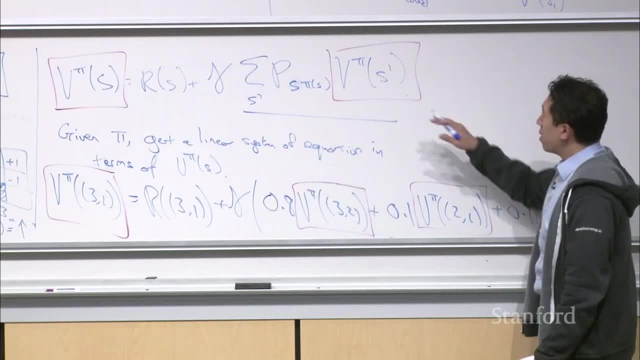 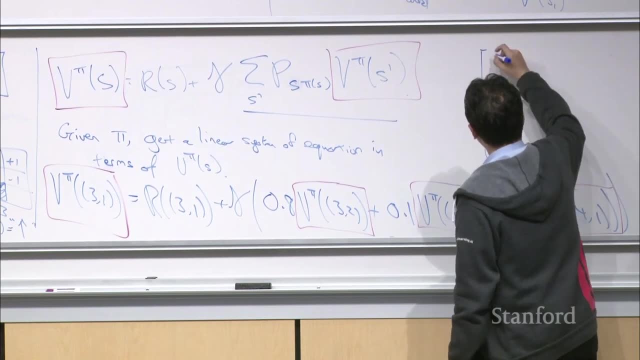 you know any policy Pi Um. the way you can solve for the value function is create an 11-dimensional vector um with V? Pi of, you know, 1, 1, V Pi of 1, 2, and so on down to V? Pi of whatever is the last state. 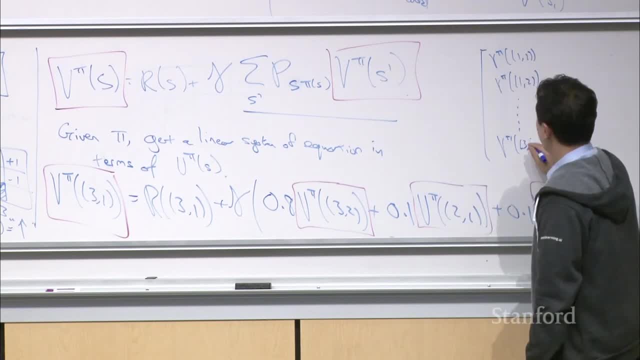 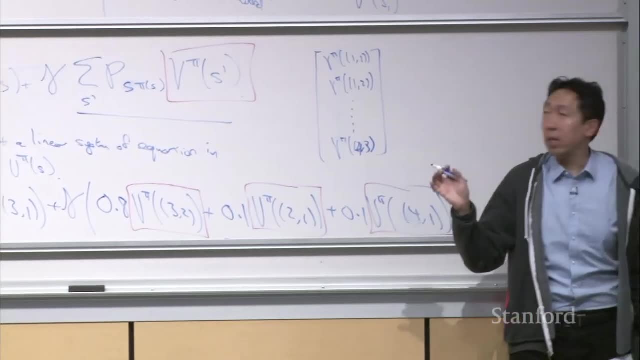 You have 11 states. so V Pi of 3,, 3 or whatever, uh 4,, 3, right? So if you want to solve for those um 11 numbers, I wrote up just uh in- in terms of defining V Pi. 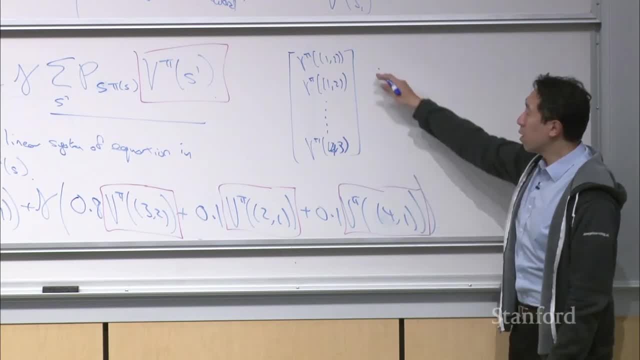 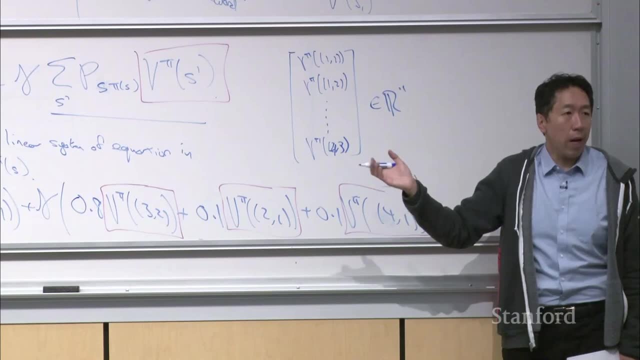 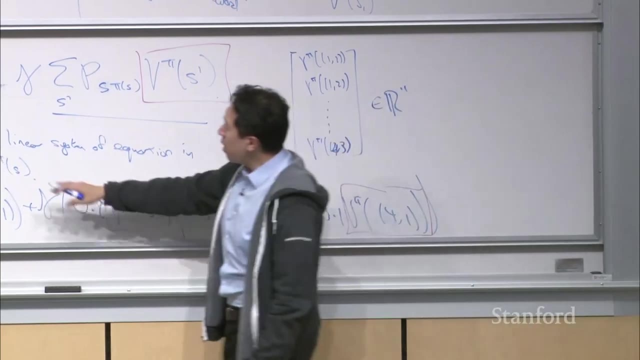 what you can do is I'll give you a policy Pi. You can then construct an 11-dimensional vector, you know, 11-dimensional vector of unknown values that you want to solve for, And Bellman's equations for each of the 11 states. um for each of the 11 states. 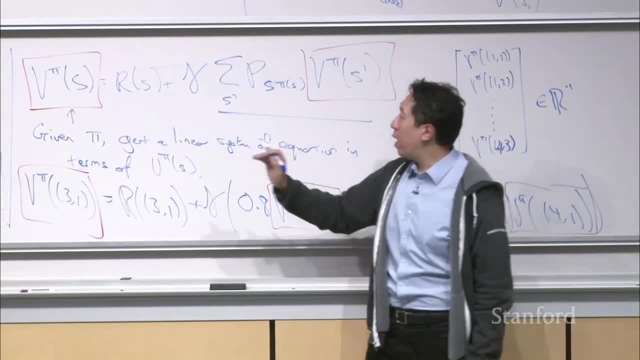 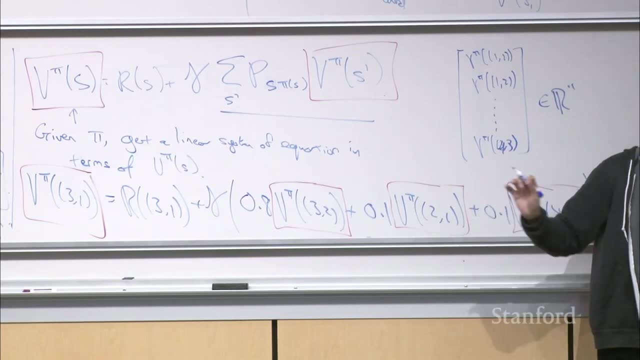 you could plug in on the left-hand side. This gives you one equation for how one of the values is determined as a linear function of a few other of the values in this vector. okay, And so, um, what this does is it sets up. 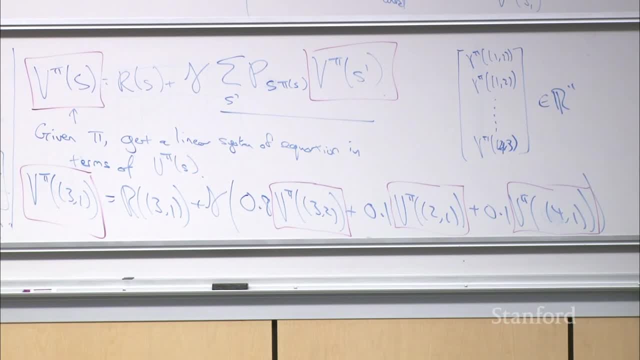 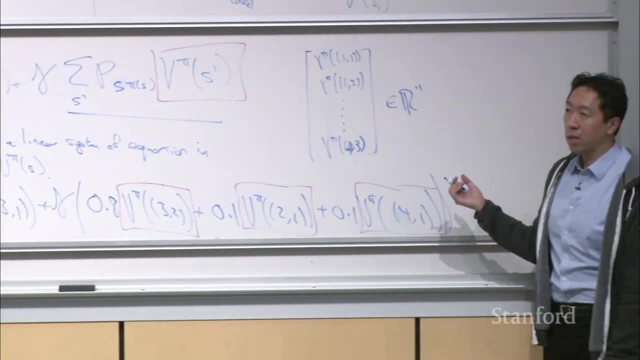 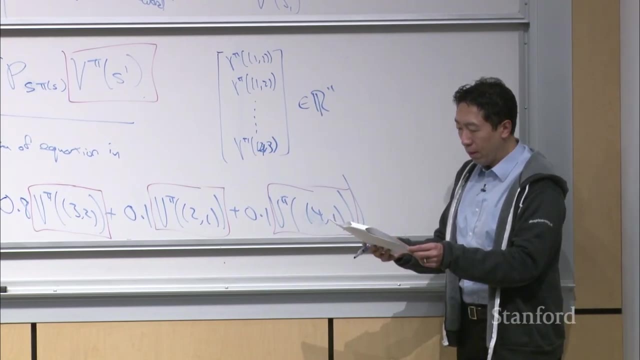 a linear system of equations with 11 variables in 11 unknowns right, And using a linear algebra solver, you- you will be able to solve this linear system of equations. Does this make sense? Okay, Um, all right, And so this works. as long as you're with this piece. 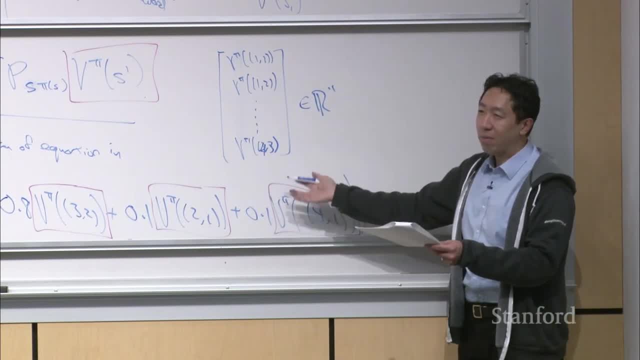 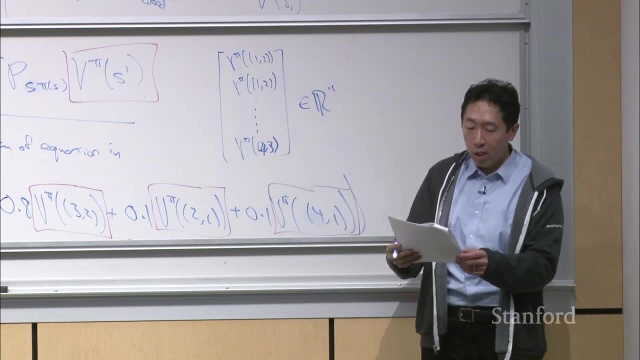 Yeah, If you have 11 states, you know it takes like a, it takes almost a, takes almost no time right In a computer to solve a linear system of 11 equations. So that's how you would actually get those values if you ever called on to solve for V Pi. 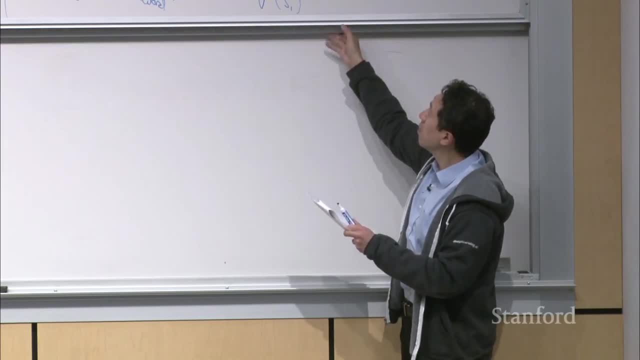 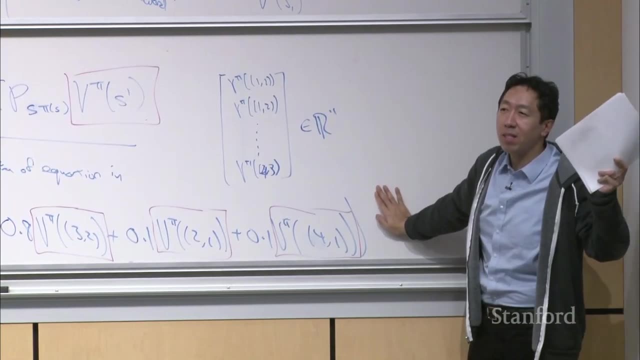 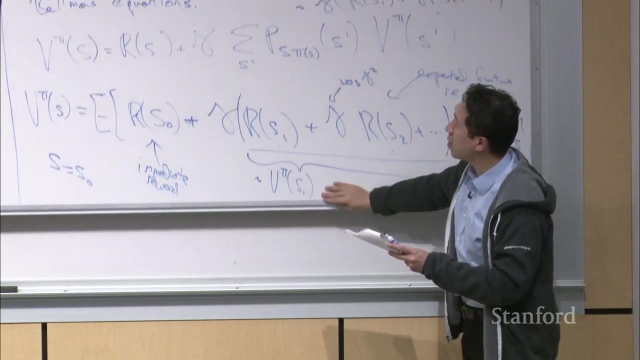 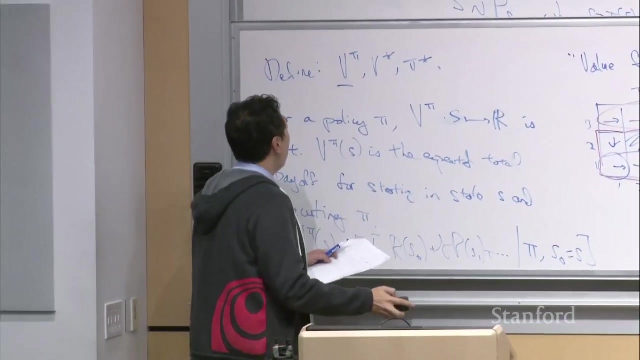 Okay, Actually, the-, the-, the. if what I just say makes sense, Raise your hand. if what I just explained made sense, Okay, cool, Awesome, Great, All right, Good. So, moving on our roadmap, um, we'll define v pi. 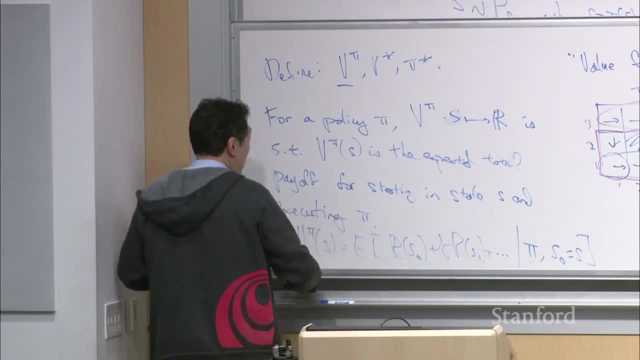 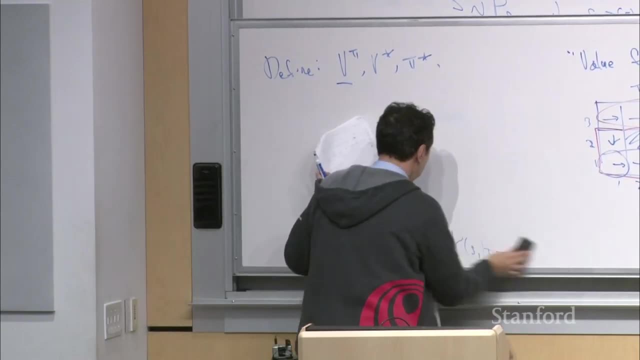 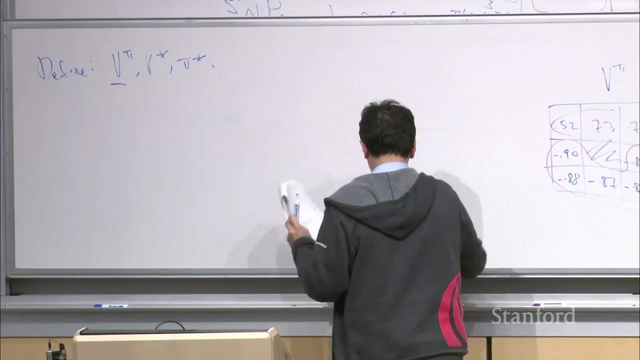 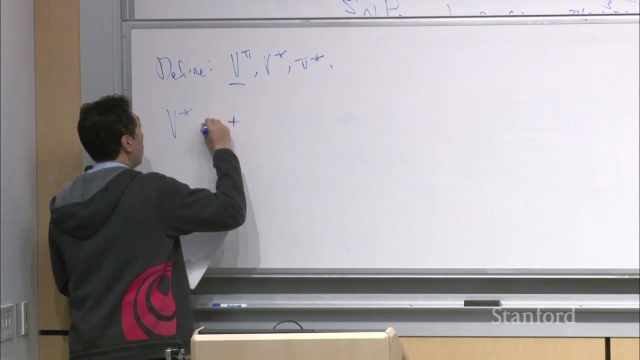 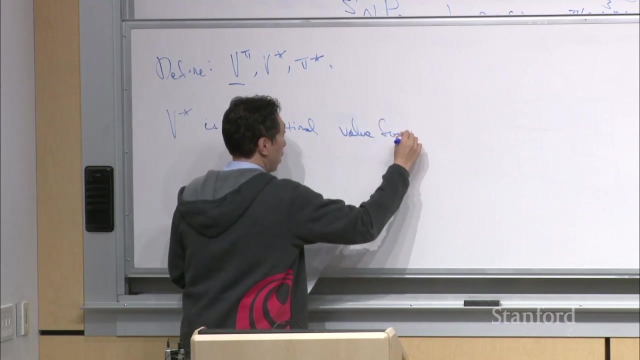 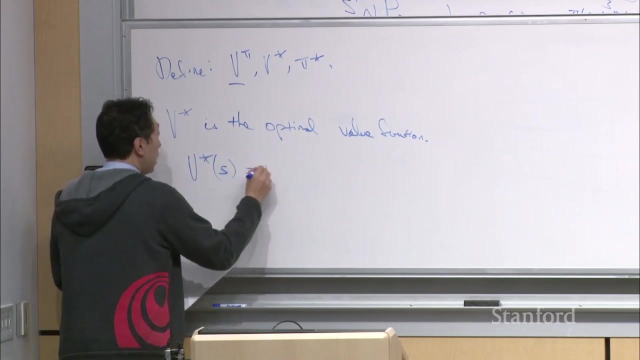 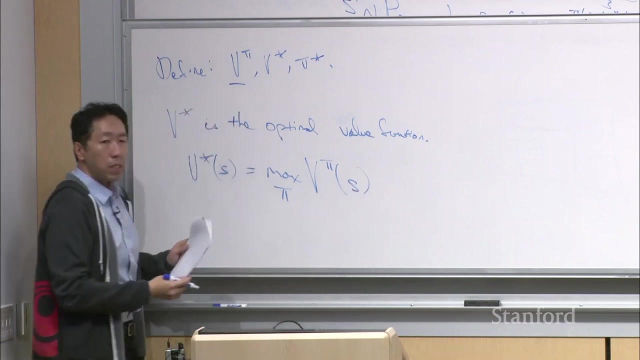 Let's now define v star Um. so. So v star is the optimal value function And we'll define it as v star of s equals max or over all policies. pi of v. pi of s, Okay, Um, one of the, I don't know. 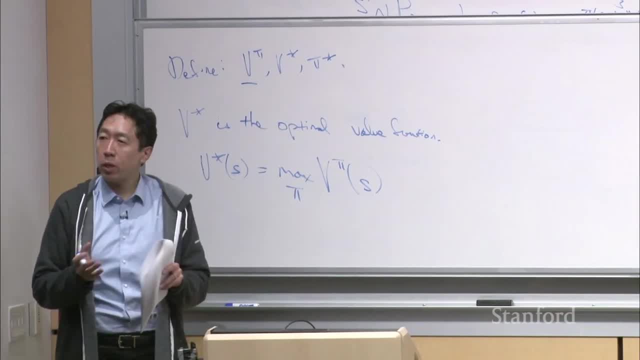 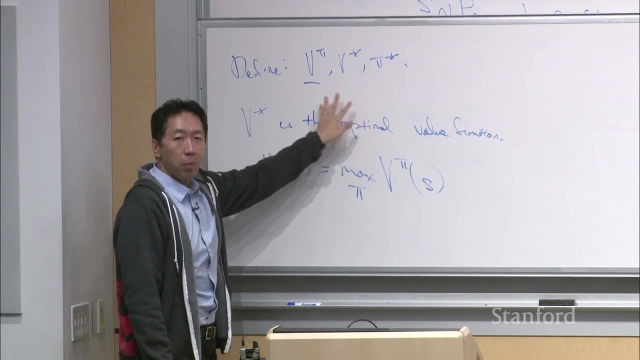 slightly confusing things about reinforcement learning terminology is that there are two types of value function. There's value function for given policy, pi, and that's the optimal value function, v, star. So both of these are called value functions, but one is a value function for a specific policy. 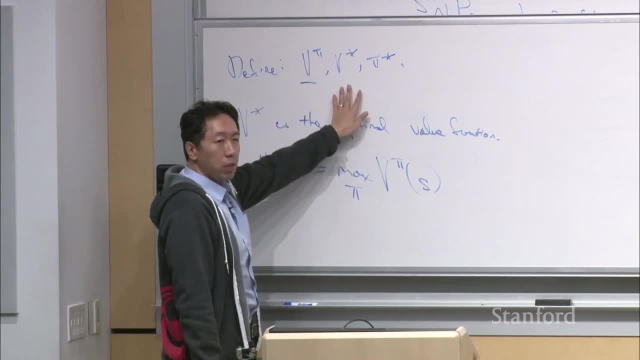 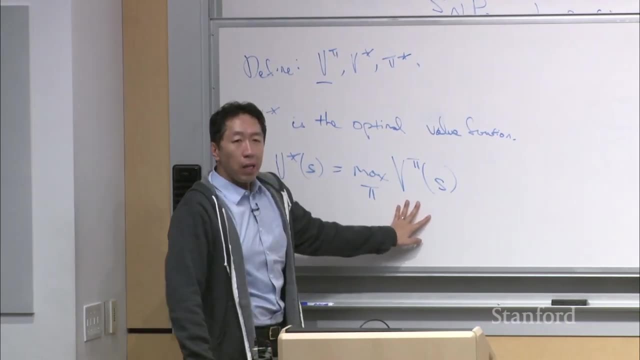 it could be a great policy, it could be a terrible policy, it could be an optimal policy. The other is v star, which is the optimal po- optimal value function. So V-star is defined as um. look at the value, for you know any- look. 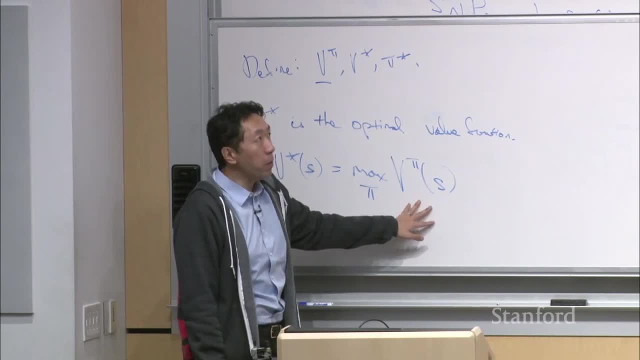 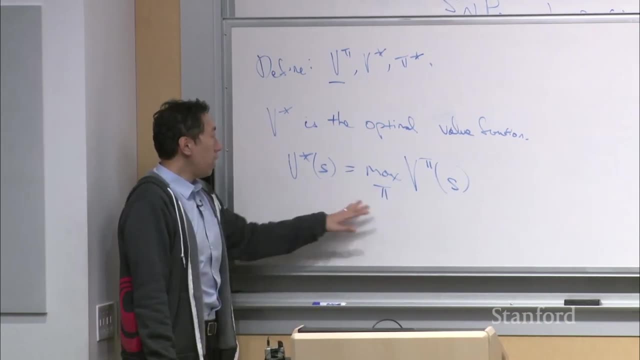 look across all of the possible policies. you could have all um 4 to 11, right. All the combinatorially large number of possible policies for this MDP And V-star of S is well, let's just take the max right. 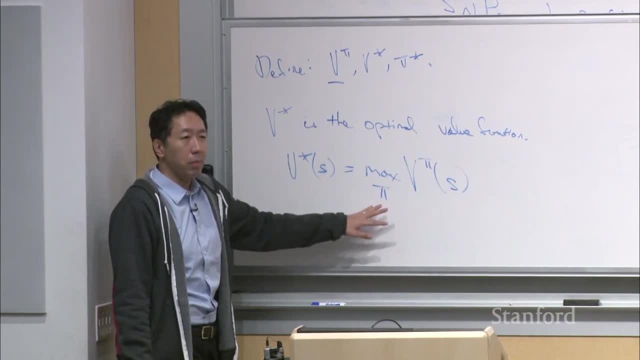 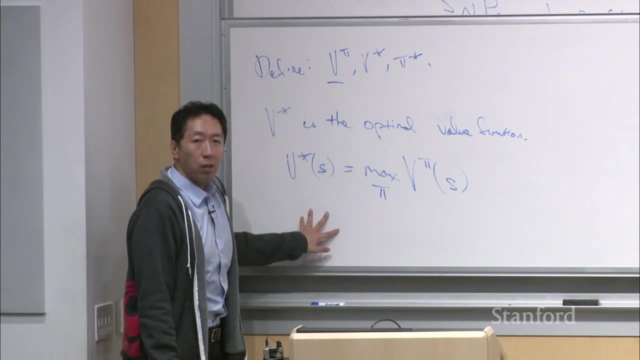 Which is, of all the possible-, of all the policies you know anyone could implement, of all the possible policies, let's take the value of the best possible policy for that state. So that's V-star okay, And that's the optimal um. 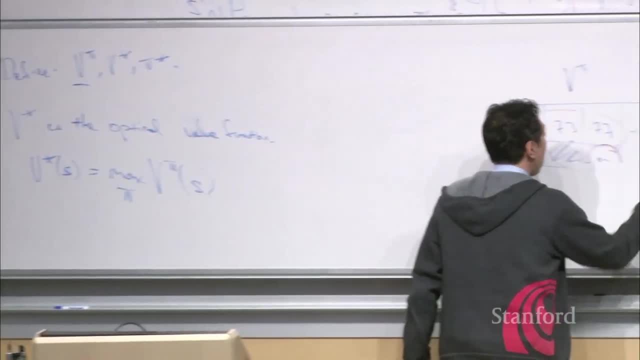 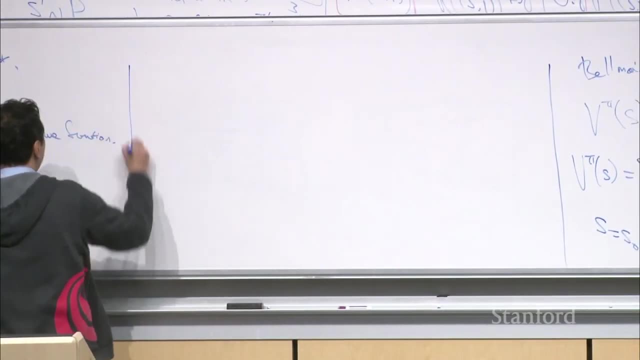 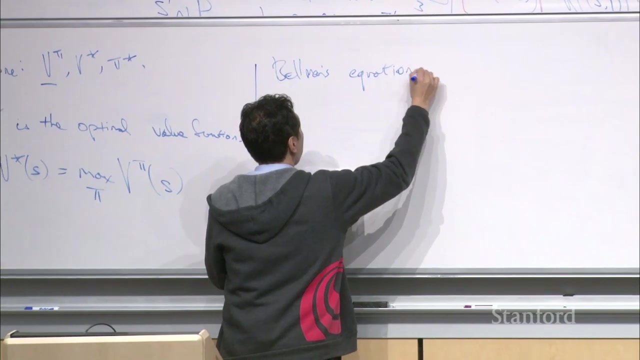 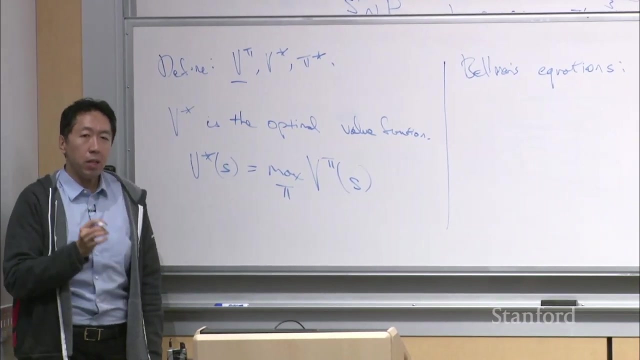 optimal value function. And it turns out that, um, there is a different version of Bellman's equations for this, And again there's a Bellman's equations for V-pi, for value of a policy, and then there's a different version of. 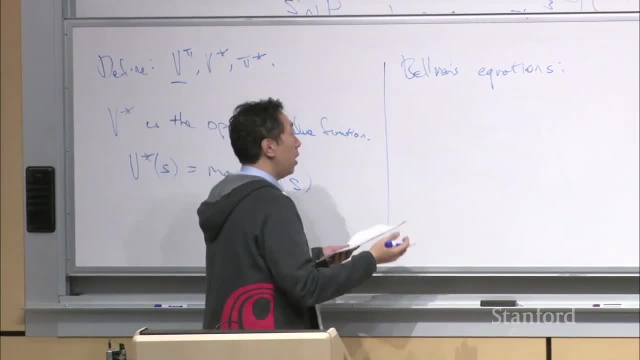 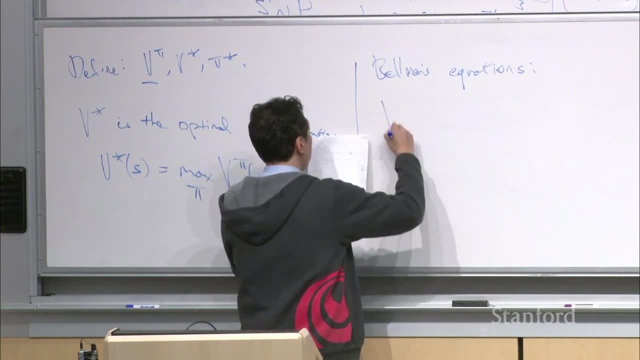 Bellman's equations for the optimal value for even cycle of any value function. right, So just there are two versions of value functions or two versions of Wu-Tang Bellman's equations. But let me just write this out and hopefully this will make sense. 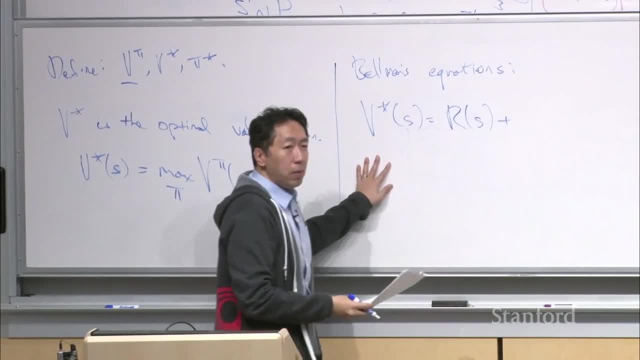 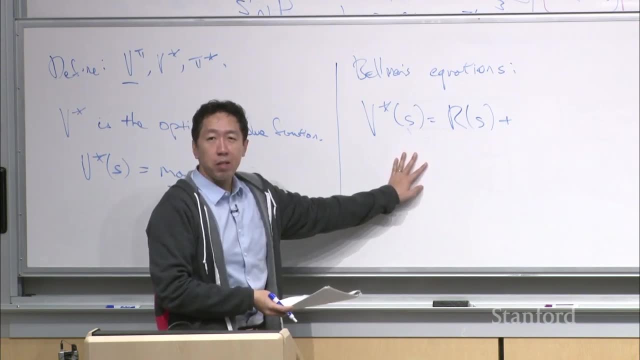 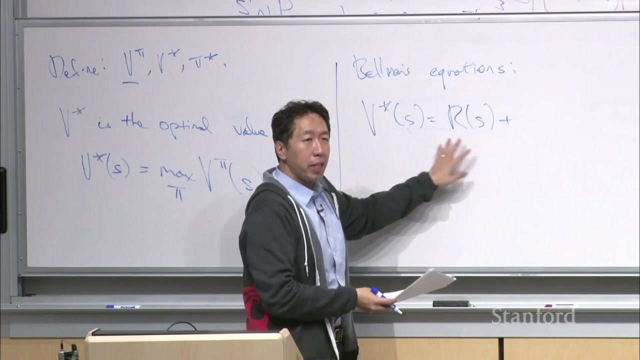 Um, actually, let's think this through. So let's say you start off your robot in a state S. What is the best possible expected sum of discount of rewards? What's the best possible payoff you could get right? Um, just for the privilege of waking up in state S. 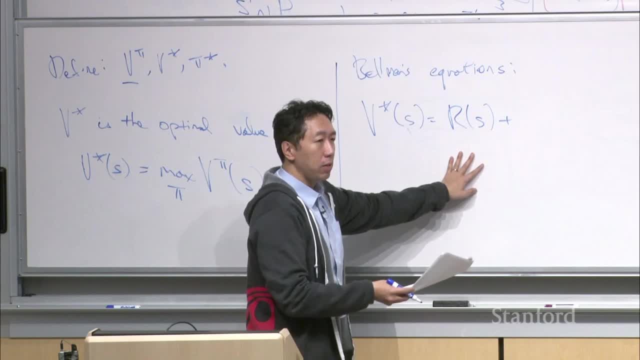 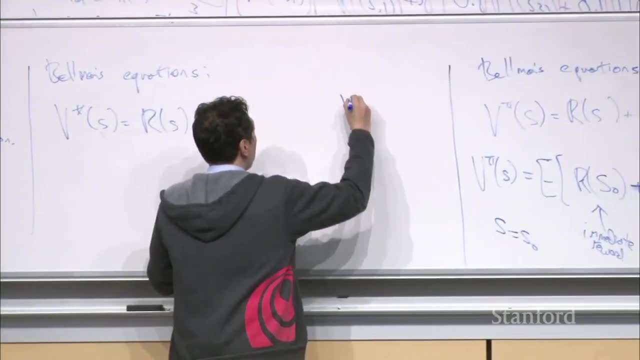 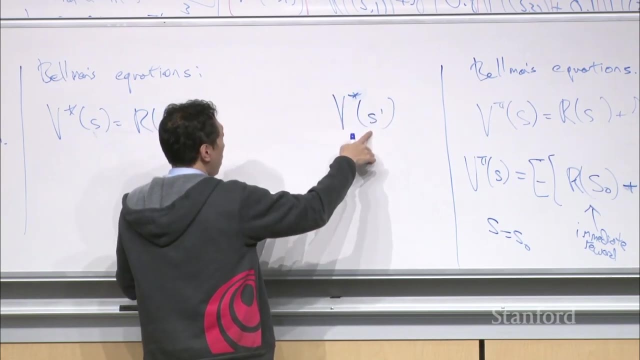 the robot will receive an immediate reward R of S right, And then it has to take some action And after taking some action, it will get to some other state S prime. um, you know, and after some other state S prime. 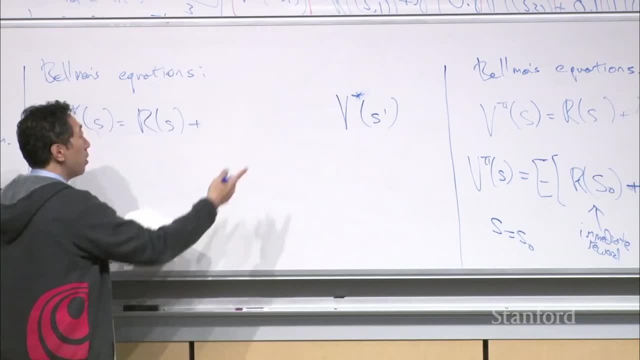 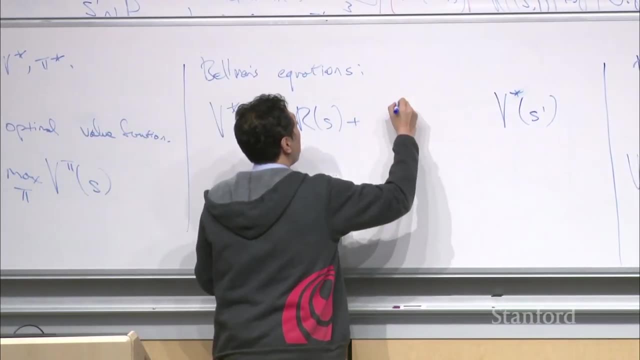 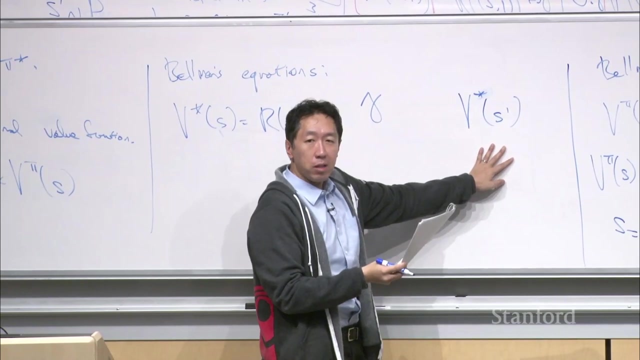 it will receive right future expected rewards: V star of S prime and we have to discount that by Gamma right. So sorry, So well. the state S prime was arrived at by your taking some action. A from the initial state. 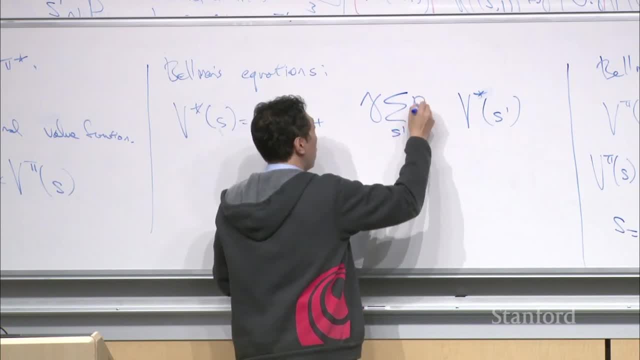 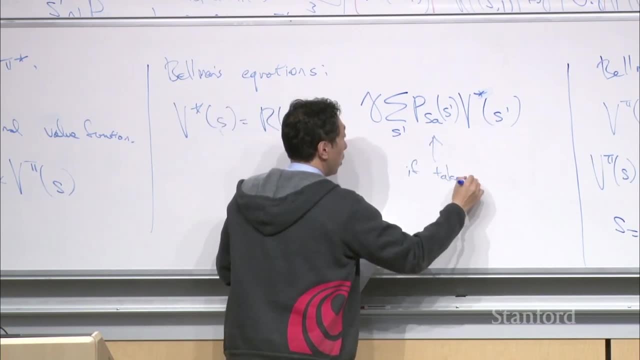 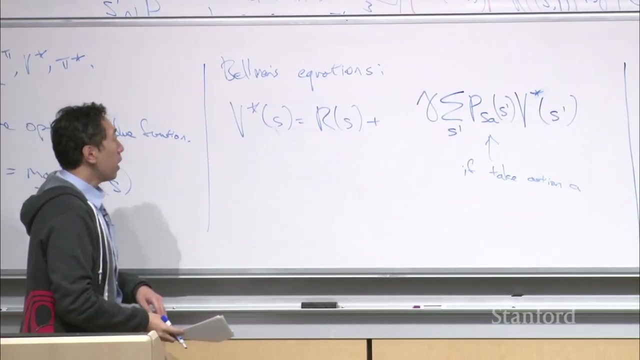 Um. and so one of the action is, you know, for if- if you take action A, right, Okay, Um, so if you take an action A in the state S, then your total payoff will be- expected total payoff will be. 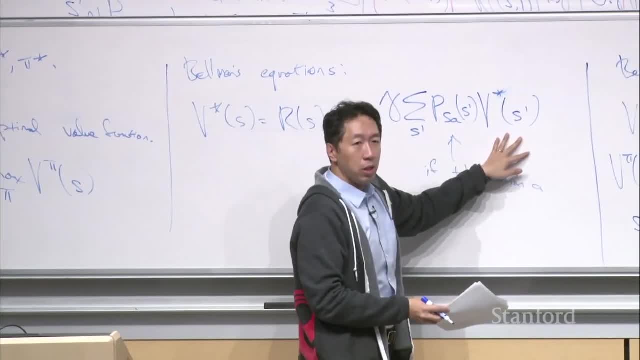 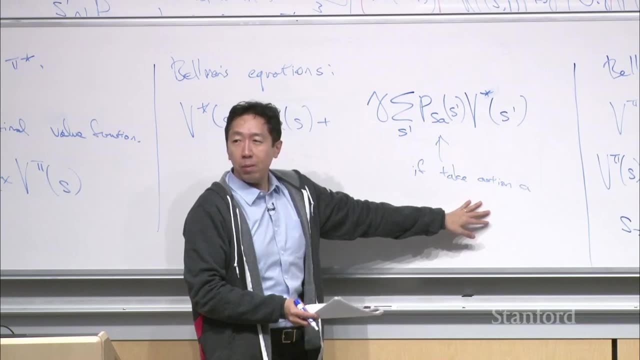 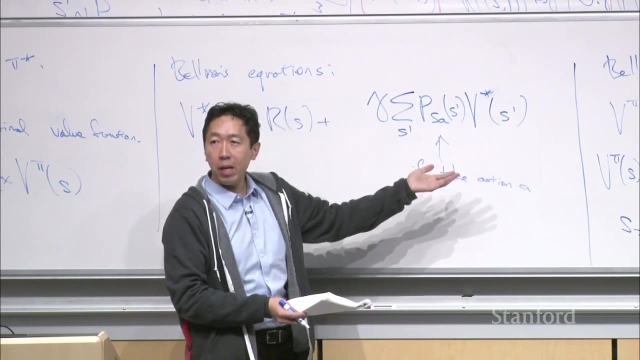 the immediate reward plus Gamma times the expected value of the future payoff. But what is the action A that we should plug in here, right? Well, the optimal action to take in the MDP is whatever action maximizes your expected total payoff, maximizes the expected sum rewards, which is 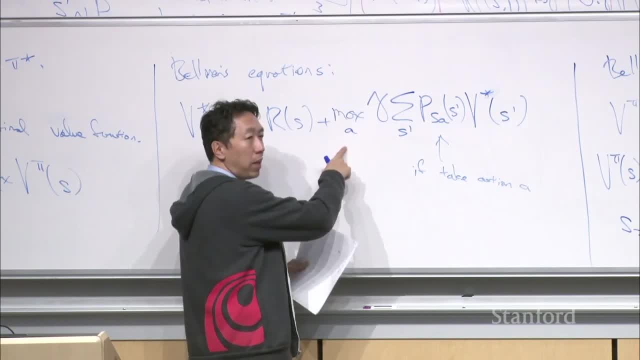 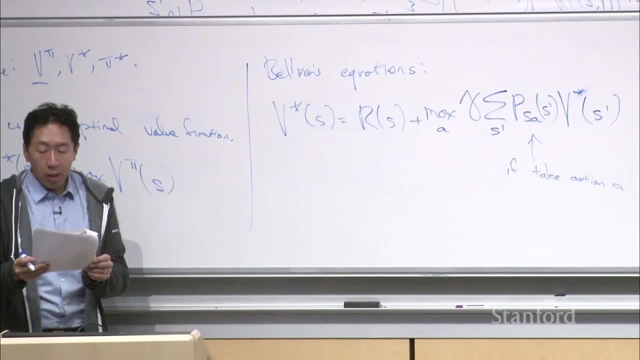 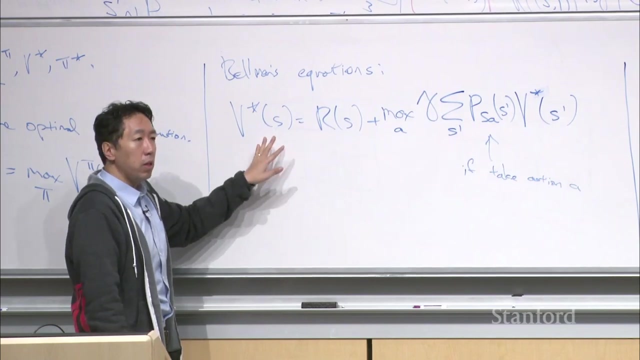 that's why the action you want to plug in is just whatever action A maximizes that. Okay, So this is um Bellman's equations for the optimal value function, which says that, uh, the best possible expected total payoff you could receive, starting from state S, is: 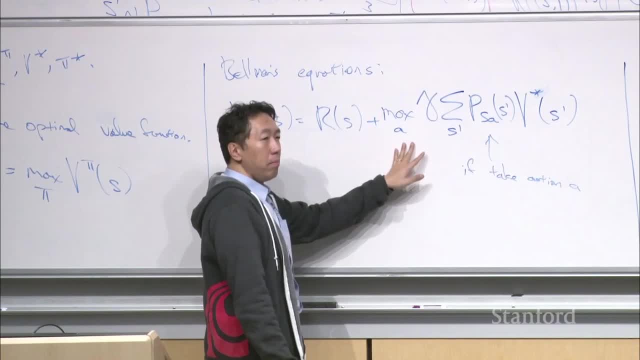 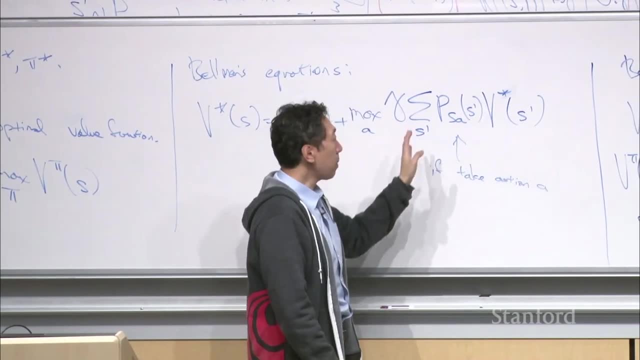 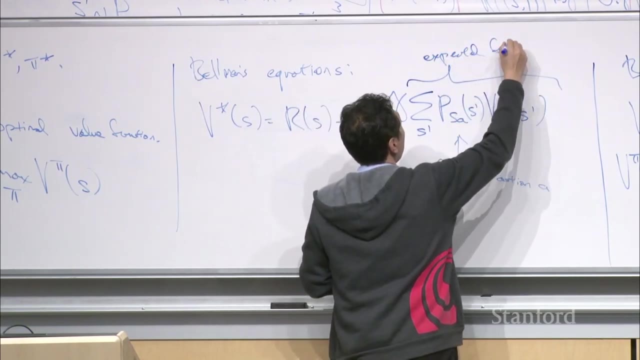 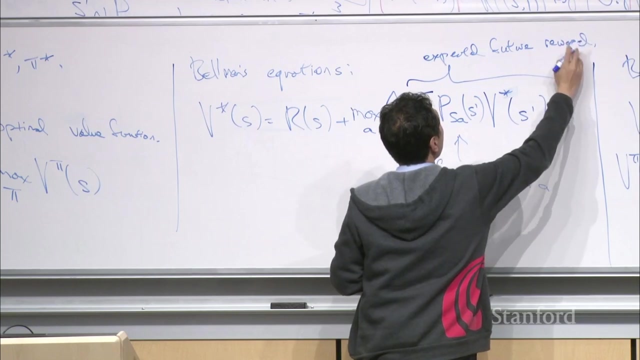 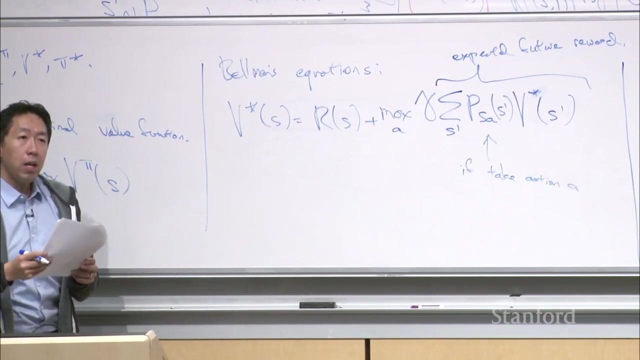 the immediate reward R of S plus max overall possible actions of whatever action allows you to maximize, you know, your expected total payoff. uh, expected future payoff. Okay, So this is the expected future payoff, or expected future reward? Okay, Um, now 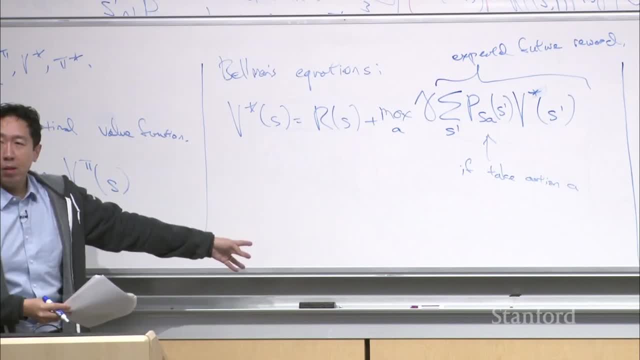 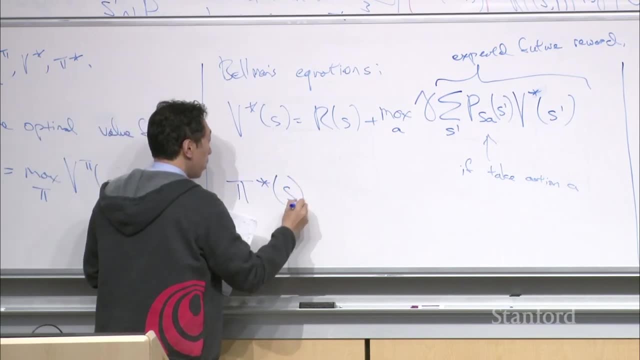 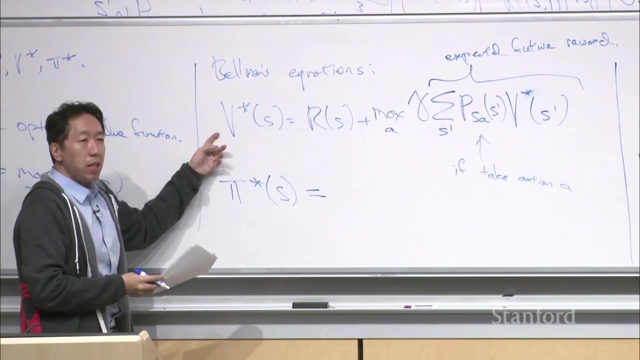 based on the argument we just went through, um. this allows us to figure, to figure out how to compute pi star of S as well, right, Which is um, let's say. let's say, we have a way of computing V star of S, right. 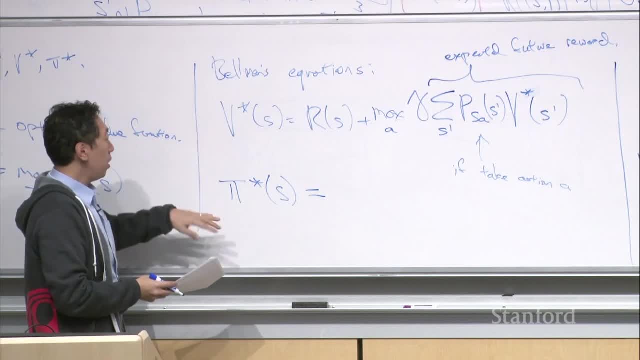 We don't yet. But let's say, I tell you what is V? star of S? Um and then I'll ask you, you know, what is the action you should take in a given state. So remember, pi pi star. 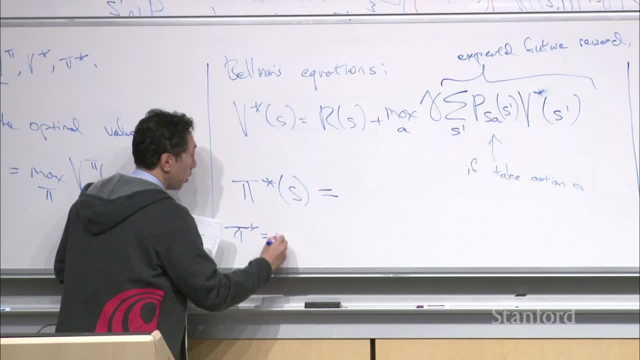 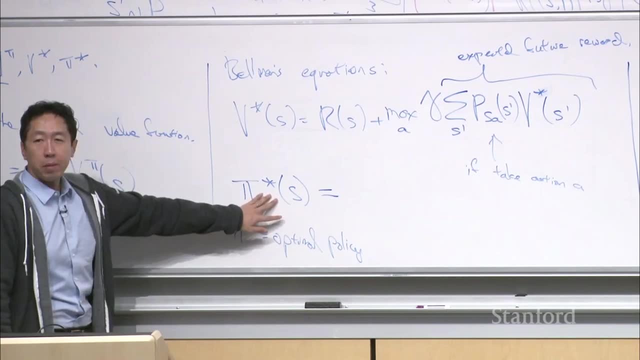 oh, pi star is going to be the optimal policy. Okay, And so, um, what should pi star of S be right, Which is, let's say, let's say we have a way of computing V star? Um, and I now ask you: 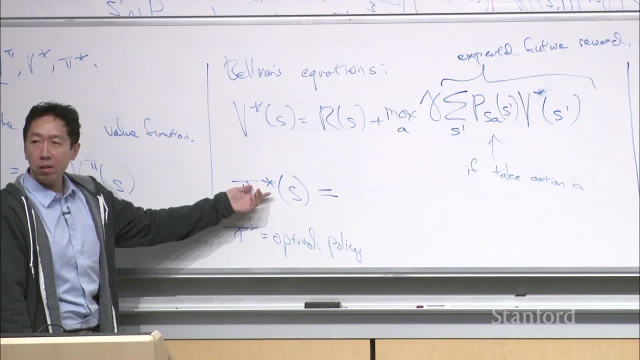 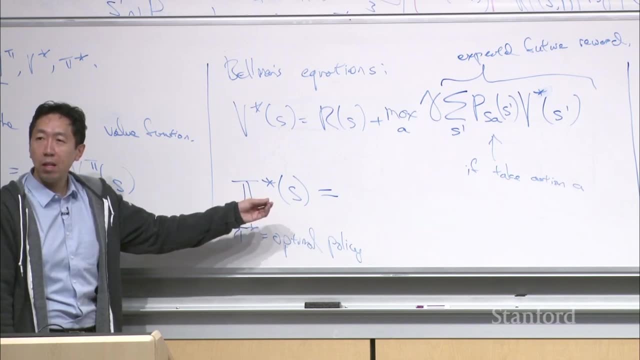 hey, my robot's in state S. what is the best action I should take from the state S? right Then how do I, how do I decide what action to take in the state S? What, what, how, yeah, what. 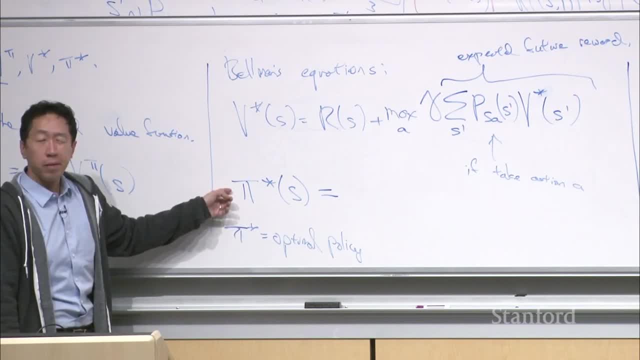 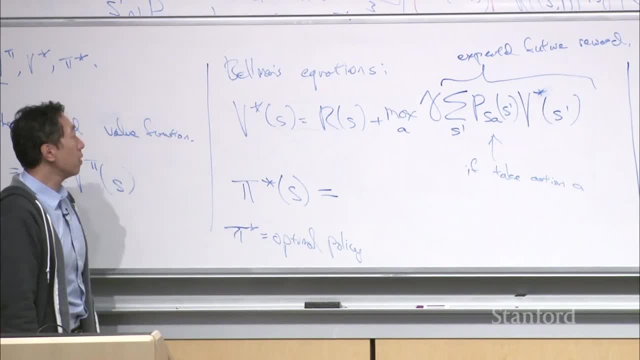 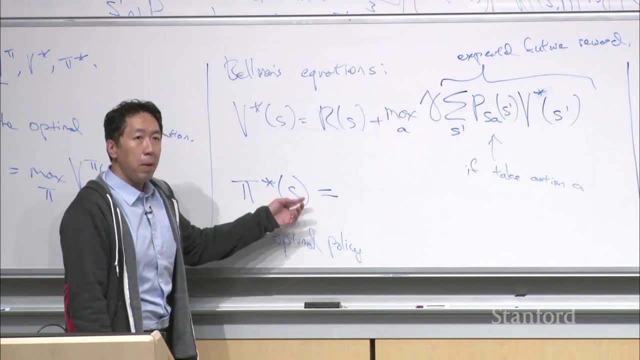 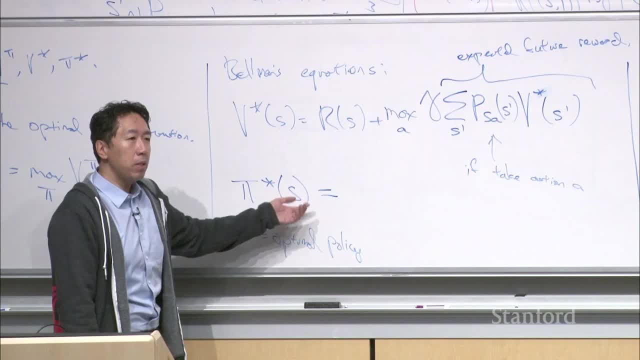 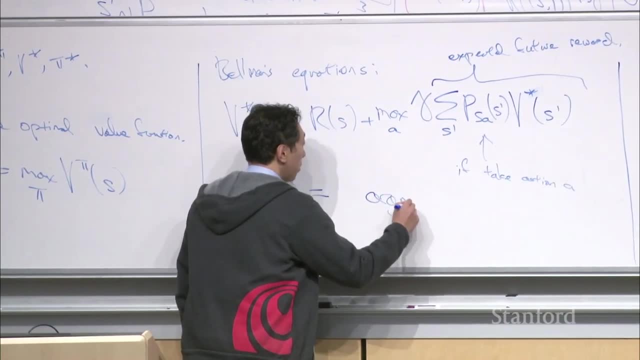 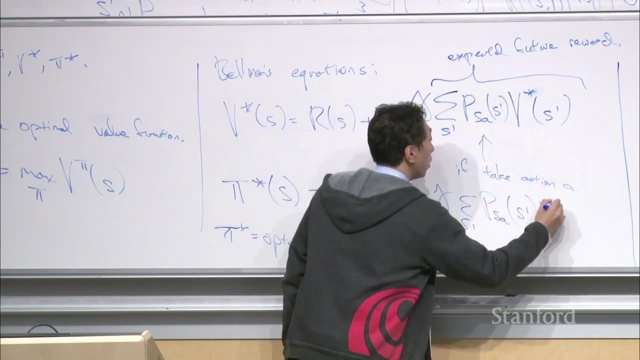 maximizing expected total payoff. But the action that maximizes your expected total payoff is, you know well whatever action we are choosing A up here, And so it's just ongmax over A of uh, that Uh, And because Gamma is just a constant, that doesn't affect the argmax. 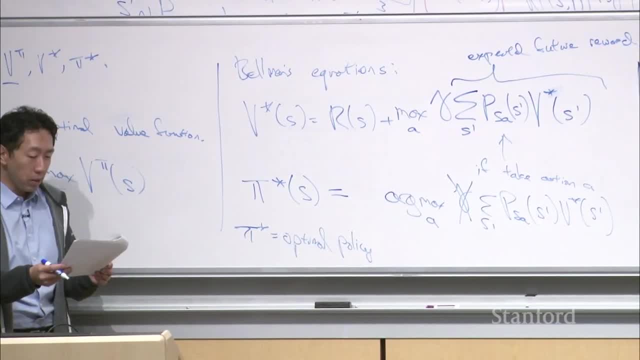 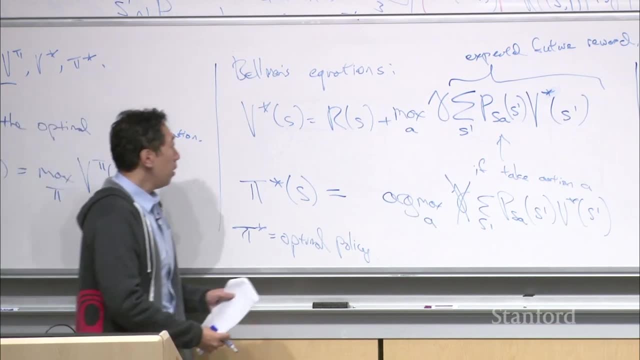 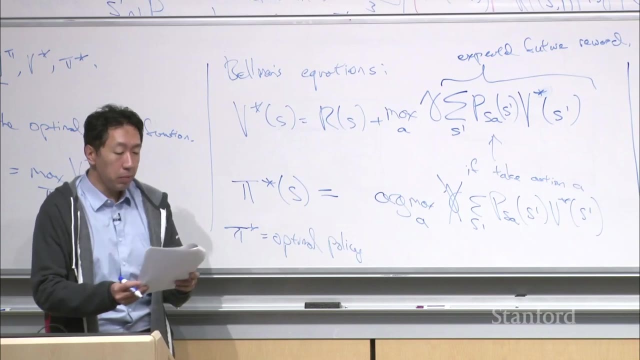 usually we just- we just eliminate that, since it's just a positive number, right. So, um, this gives us the strategy we will use for finding, um the optimal policy for an MDP, which is, um we're going to find a way to compute v. star of s. 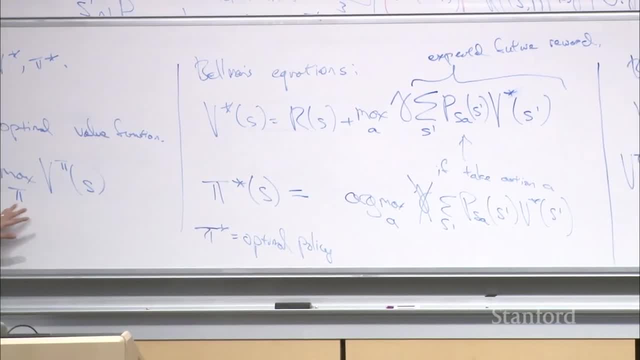 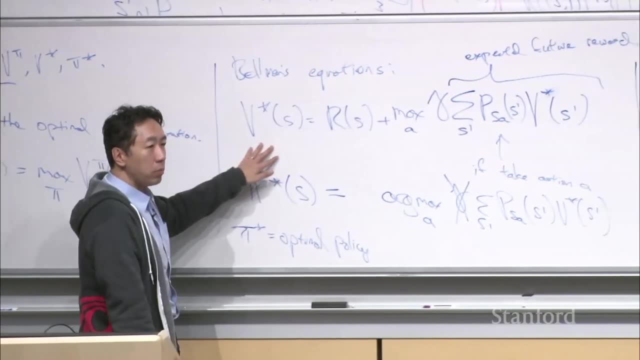 which we don't have a way of doing yet. right V star was defined as uh max over combinatorial or exponentially knowledge number of policies. So we don't have a way of computing v star yet, But if we can find a way to compute v star, 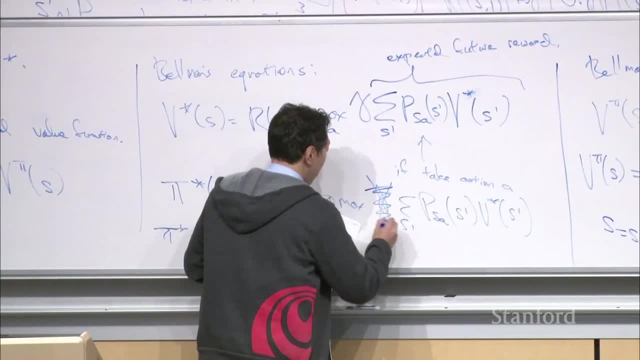 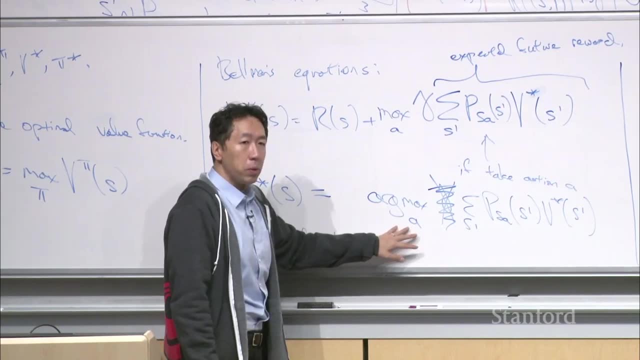 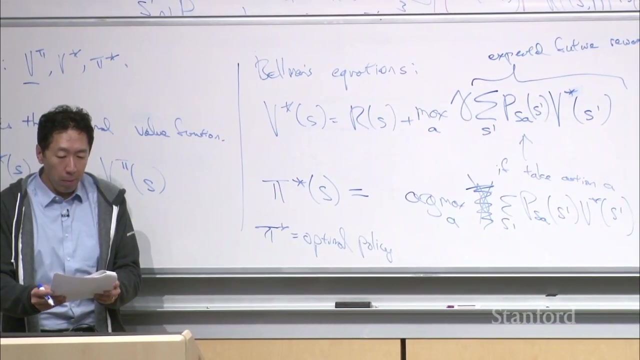 then you know, using this equation- sorry, I just scratched this out- okay, Using this equation gives you a way for every state, for every state s, to pretty efficiently compute this argmax um and therefore figure out what is the optimal action for every state. 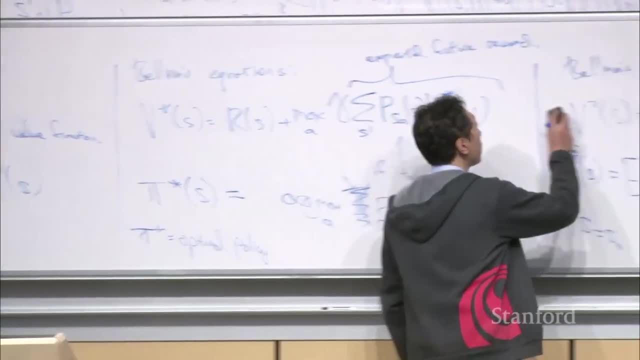 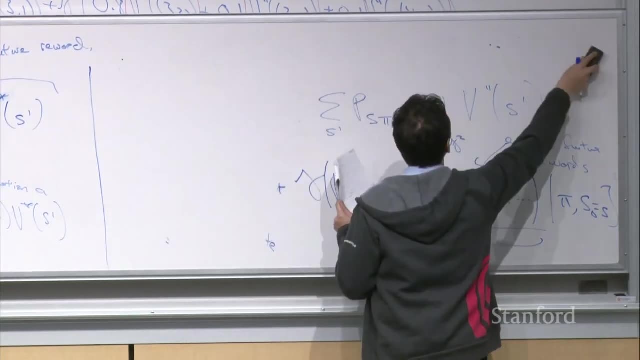 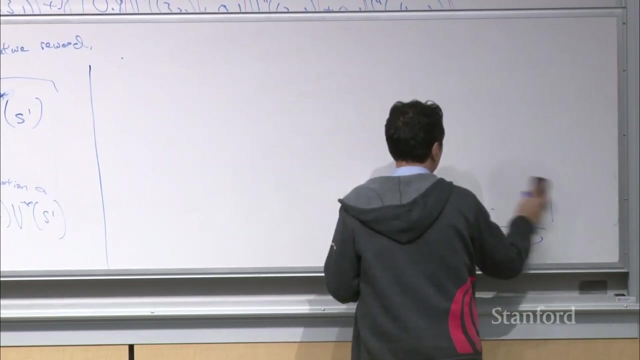 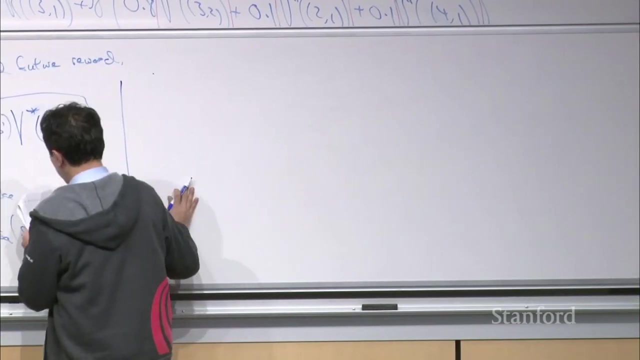 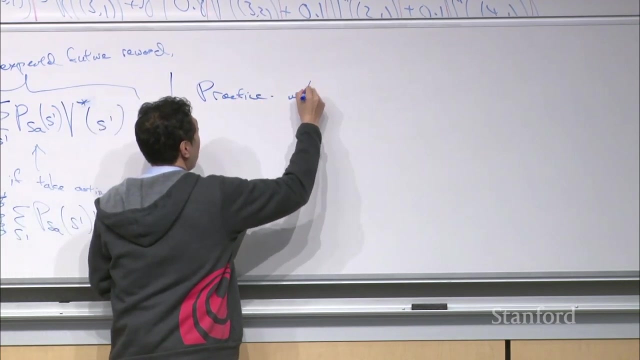 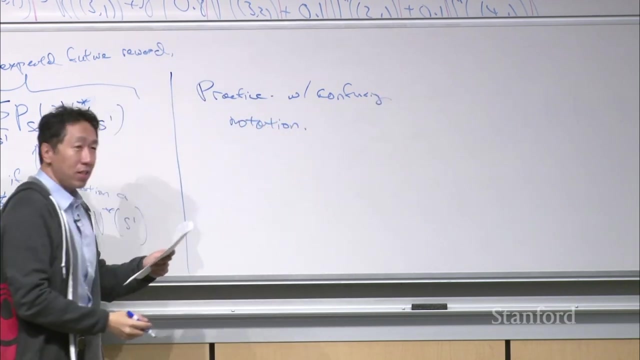 Okay, All right. Um so, all right. So just to practice with confusing notation. All right, let's see if you understand this equation. I'm I'm just claiming this, I'm not proving this, But for every state S. 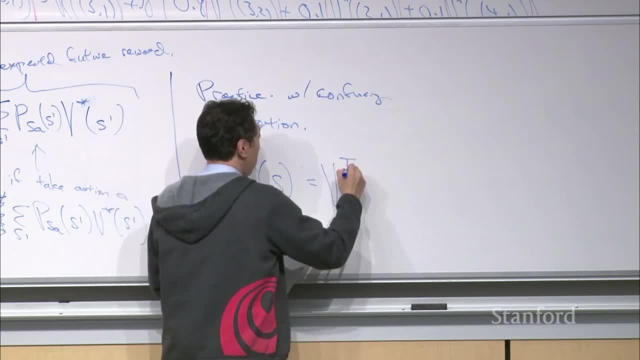 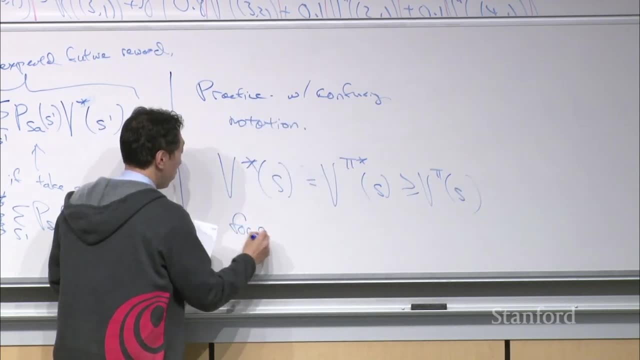 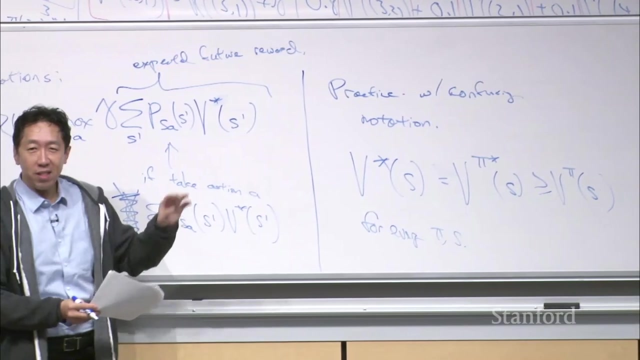 V star of S equals V of pi. star of S is greater than V pi of S. all right, For every positive pi in every state, S okay. So I hope, hope this equation makes sense. Uh, this is what I'm claiming. I didn't prove this. 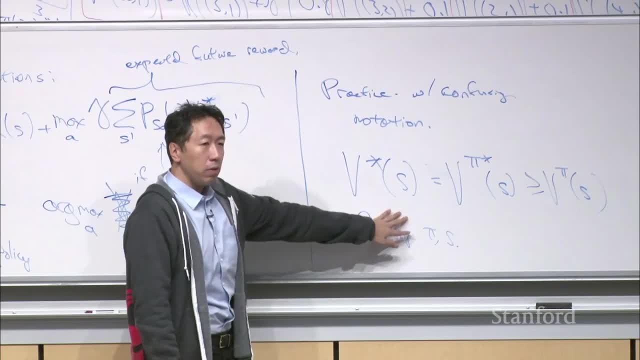 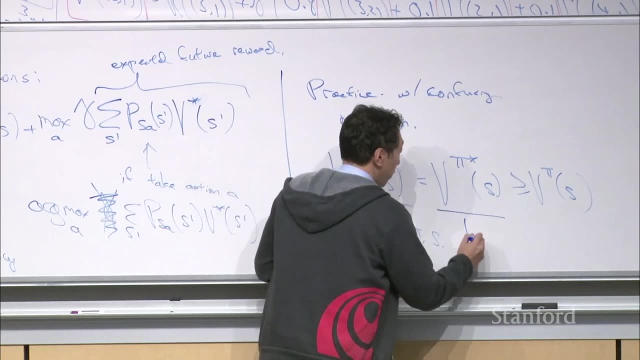 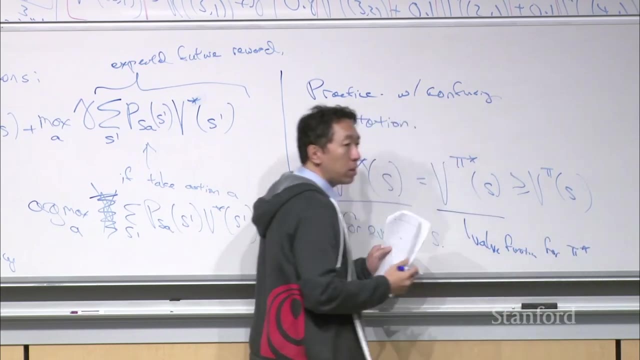 What I'm claiming is that, um, the optimal value for state S is: this is the optimal value function on the left: This is the value function for pi star. So this is: this is the optimal value function. this is the value function for a specific policy: pi. 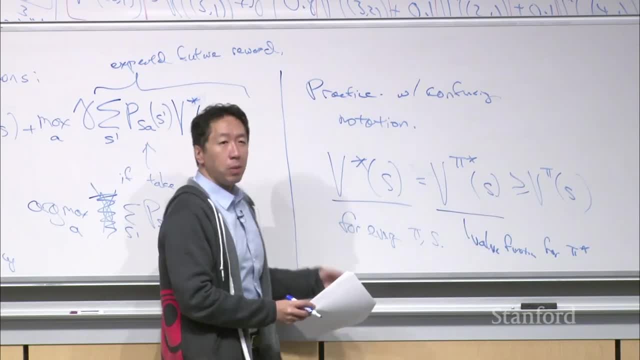 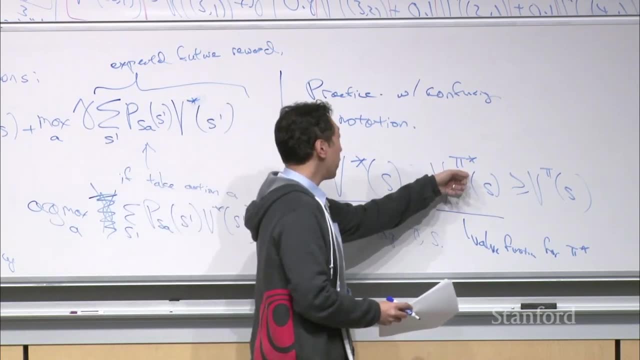 where the policy pi happens to be pi star, And so what I'm claiming here is that um. well, what I'm writing here is that, um, the optimal value for state S is equal to the value function for pi star applied to the state S. 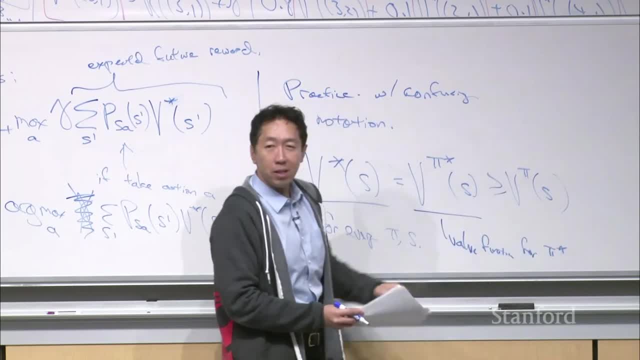 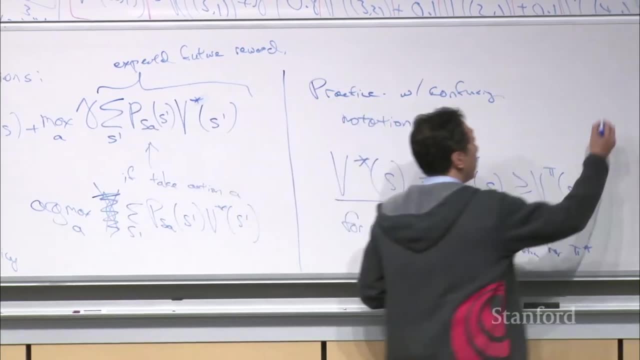 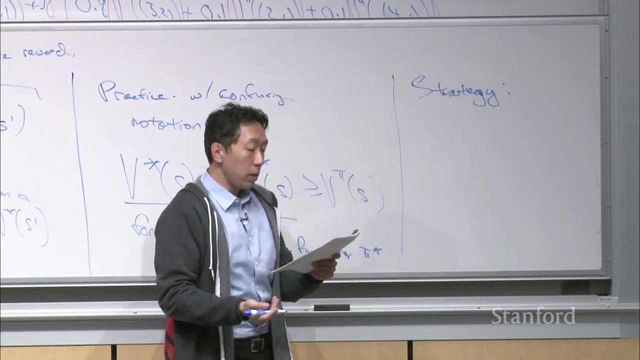 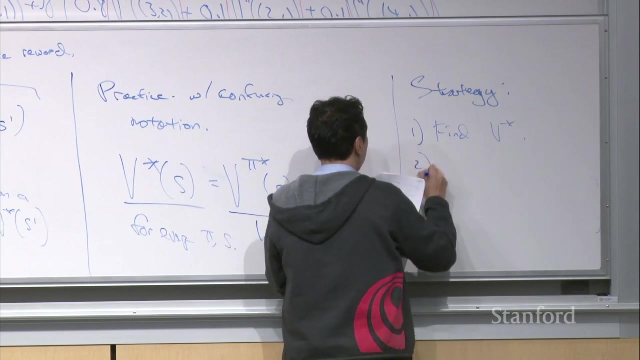 and this is greater than or equal to V pi of S for any other policy, pi. okay, All right, So um, the strategy you can use for finding for optimal policy is: uh, one, um find V star two, you know. 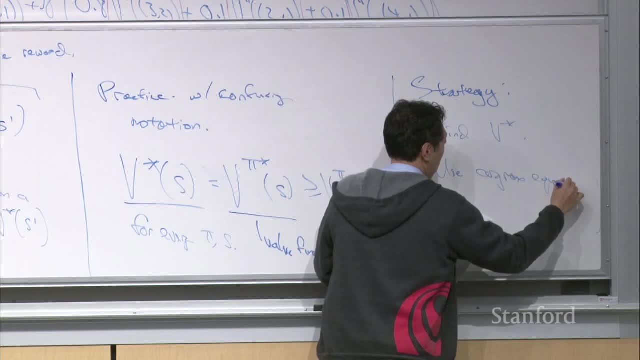 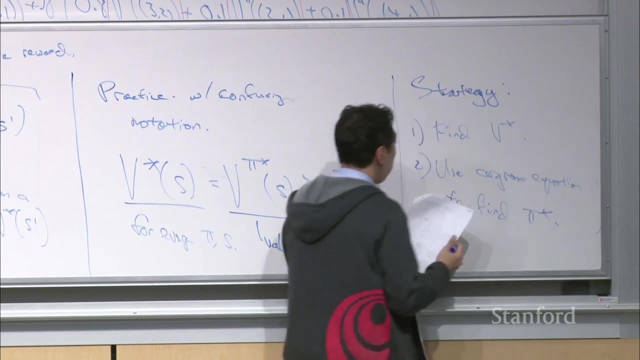 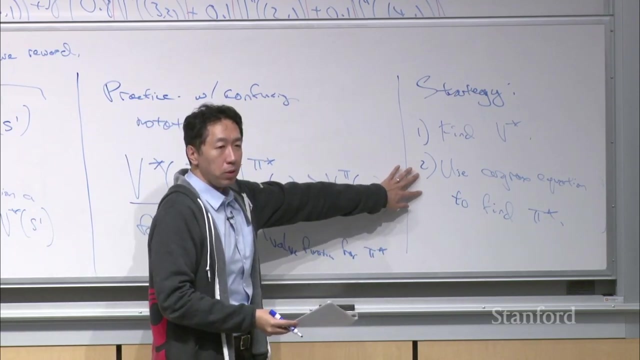 use the argmax equation to find um pi star. okay, And so what we're going to do is, uh well, step two, right, We we know how to do from the argmax equation. So what we're gonna do is talk about an algorithm for actually computing V star, because if you can compute, 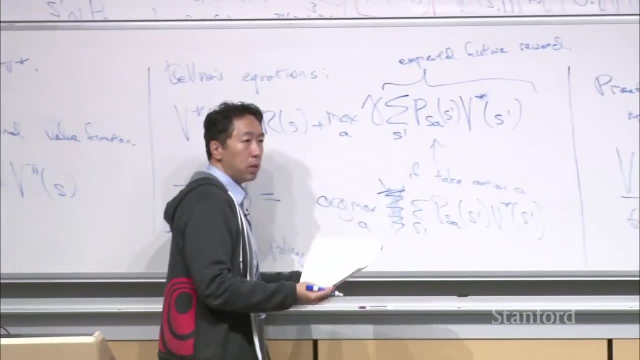 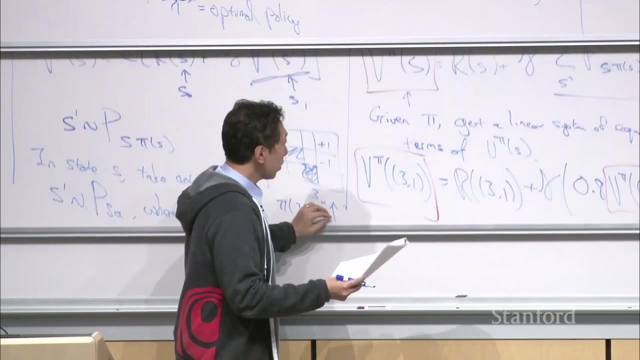 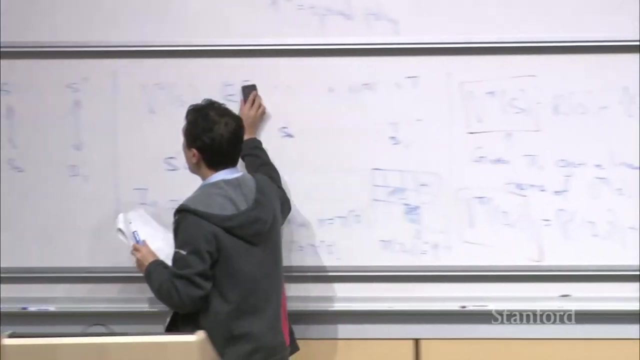 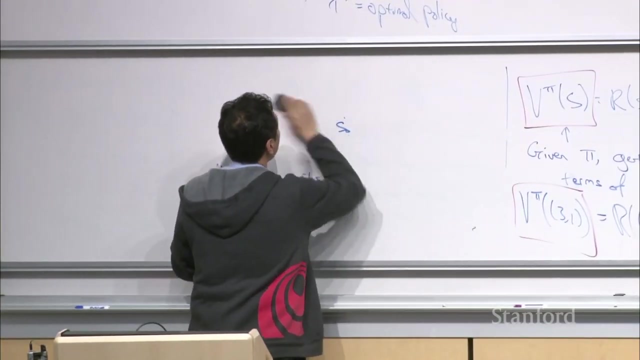 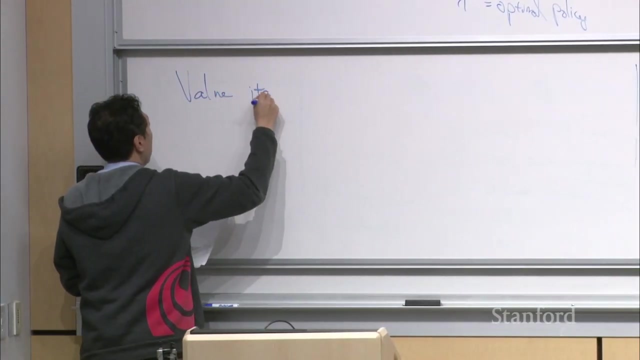 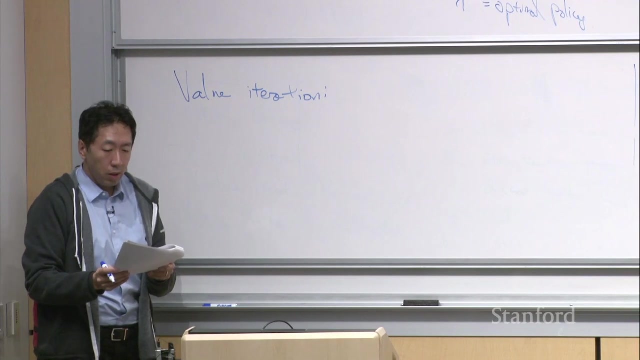 V star, then this equation helps. allows you to pretty quickly find the optimal um action for every state. So um, so value iteration: um is um. uh is an algorithm you can use to um to find V star. 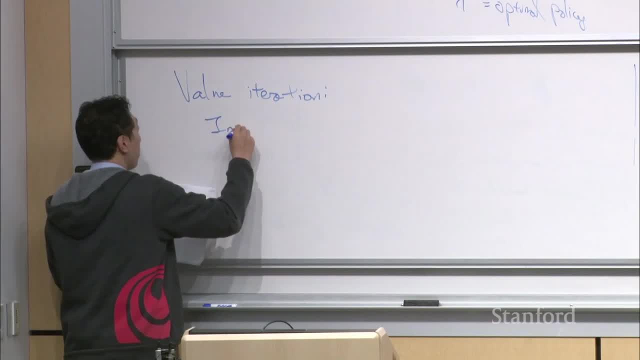 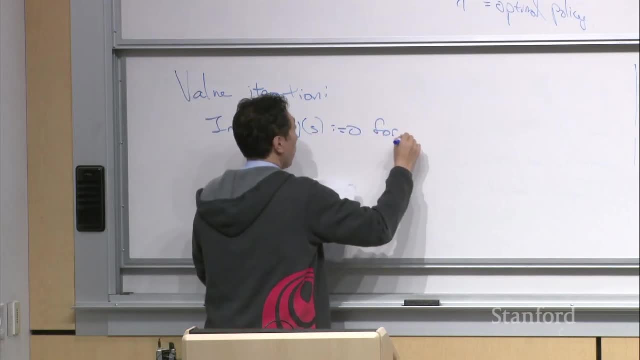 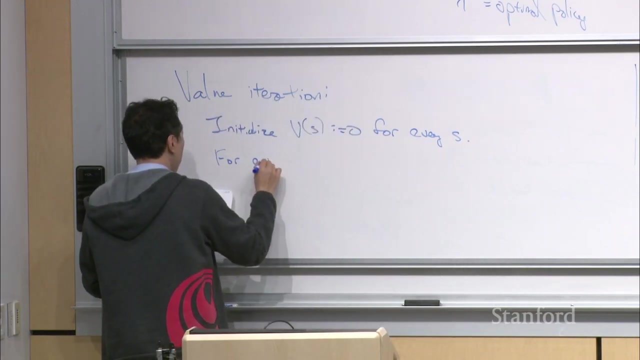 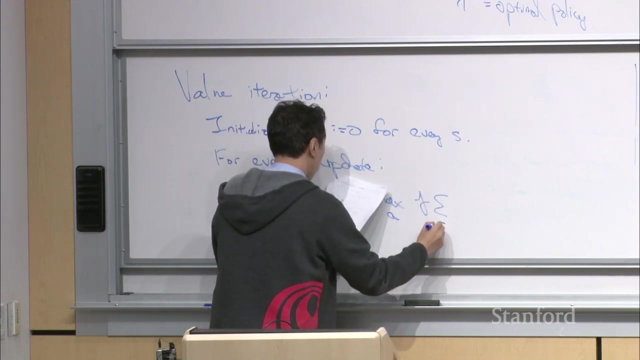 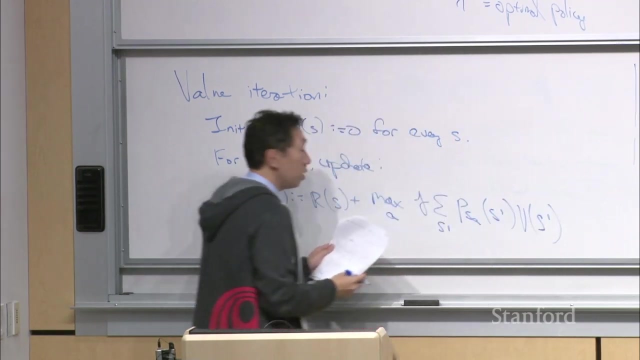 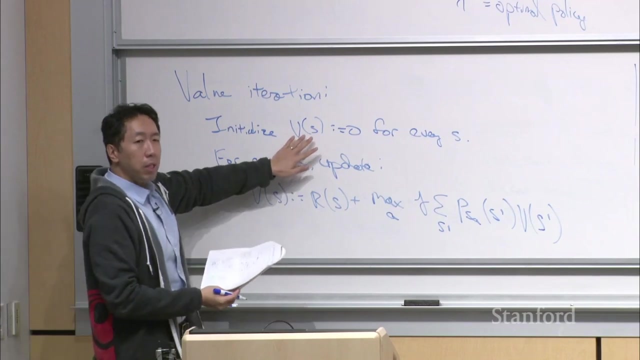 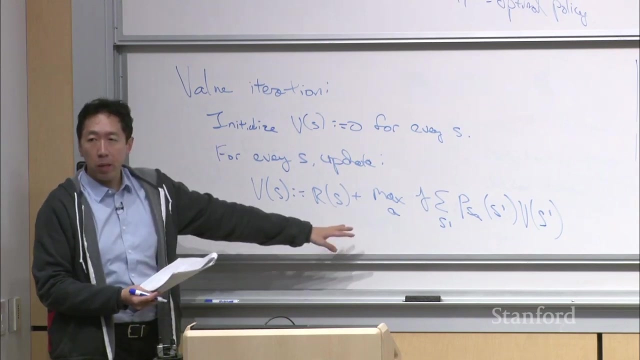 So let me just write out the algorithm: Um, so this is um. Okay, Okay, Okay, Okay, Okay. So in the value iteration algorithm you initialize the estimated value of every state to 0, and then you update these estimated values using Bellman's equations. 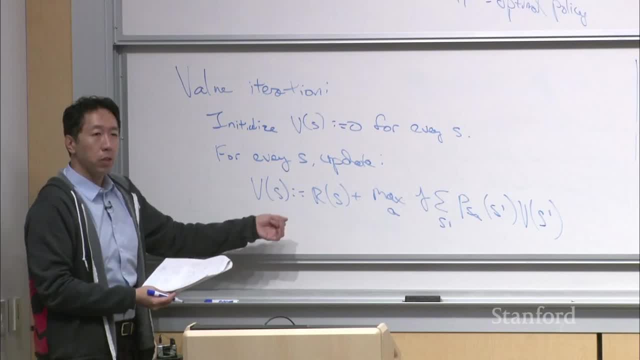 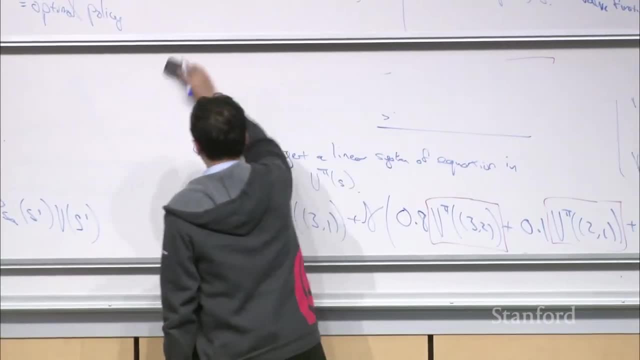 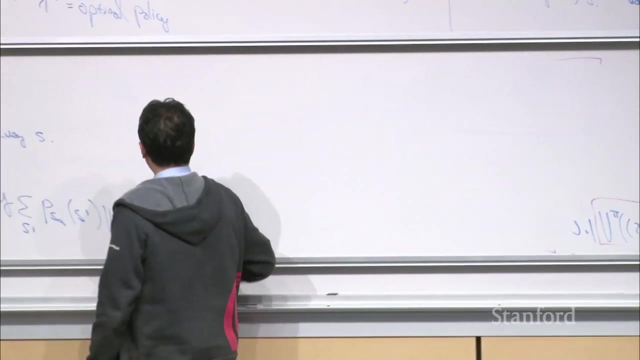 And this is the uh optimal value function, the V star version of Bellman's equations, right And um. so, to be concrete about how you implement this, you know if you're implementing this right, if you're implementing this in Python. 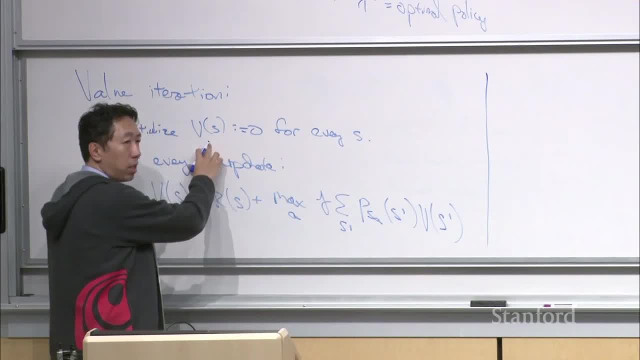 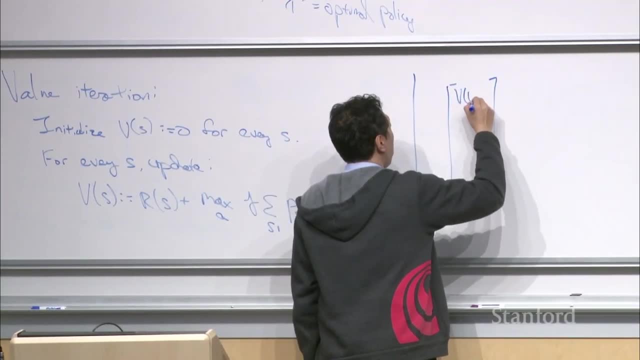 um, what you would do is create a 11-dimensional vector to store all the values of V of s. So you create a, you know, 11-dimensional vector, right that- that uh represent V of 1, 1, V of 1,. 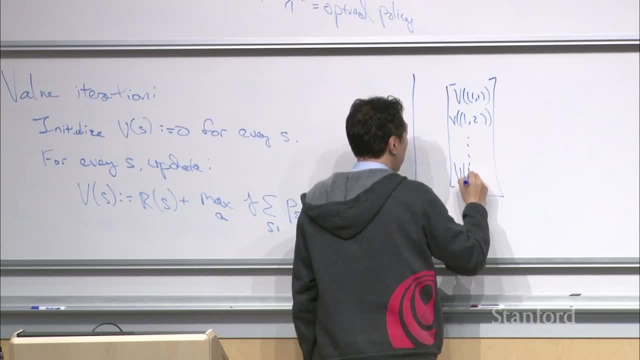 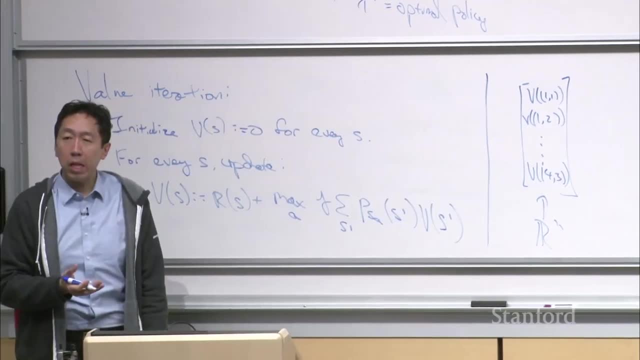 2,, you know, down to V of uh, 4,, 3, right, So this is um 11-dimensional vector corresponding to the 11 states. Um, oh, I'm sorry, I should- wait. did I say 11?? 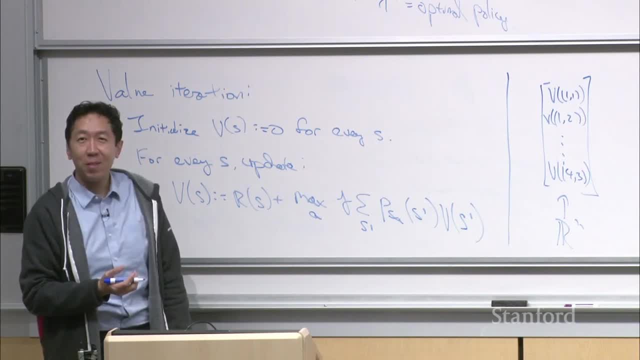 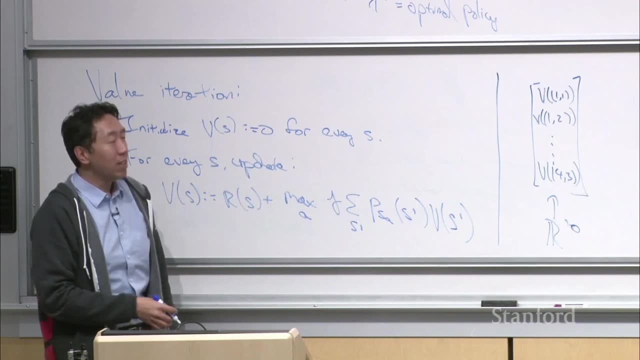 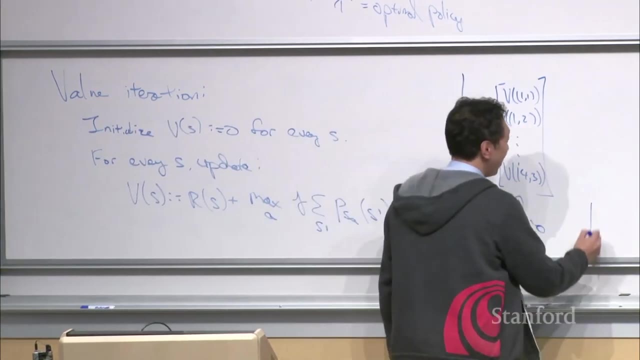 We have 10 states in the MTP, don't we Wait? Yes, we have 10 states. I've been saying 11 all along, Sorry, Okay, 10.. Um, uh, yeah, Uh, wait 11?. 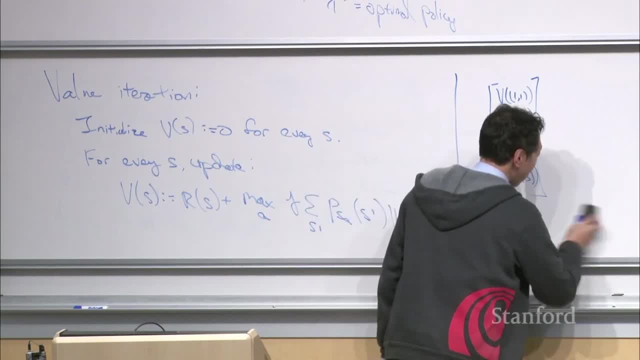 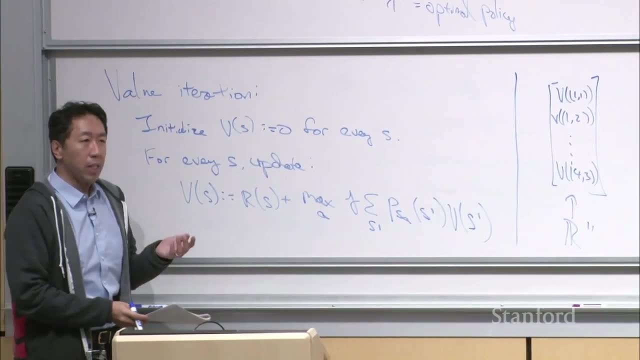 Oh, yes, you're right, Sorry, Yes, 11.. Okay, Sorry, Yes, 11 states. Okay. So, uh, right, So 11 states in MTP. So you create an initial uh, create an 11-dimensional vector um. 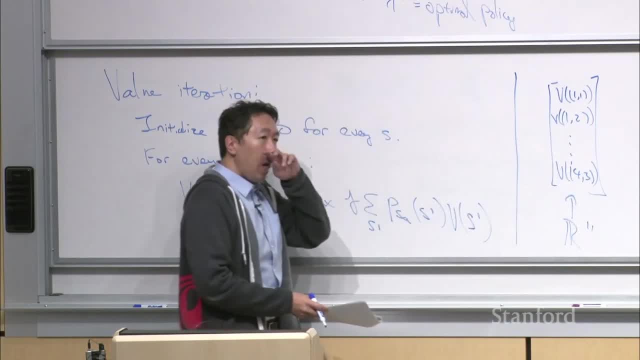 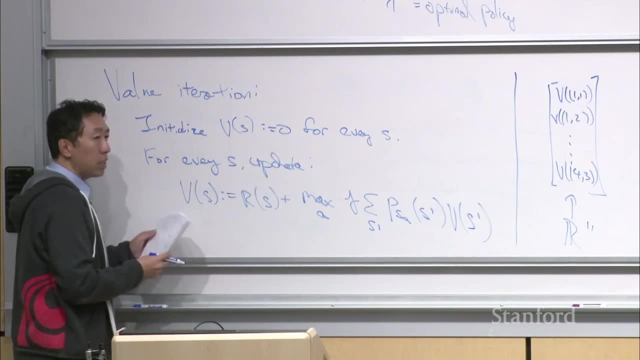 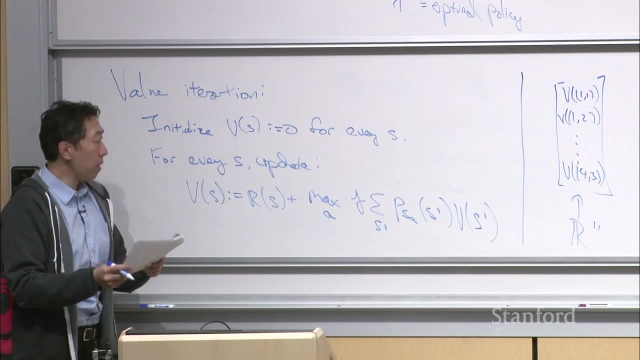 and initialize all of these values to zero, And then you will repeatedly update, um, the estimated value of every state according to Bellman's equations, right, Um, and so, uh, there-, there- there are actually two ways to interpret this. 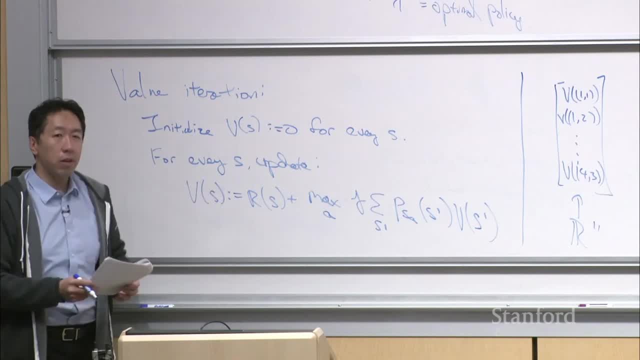 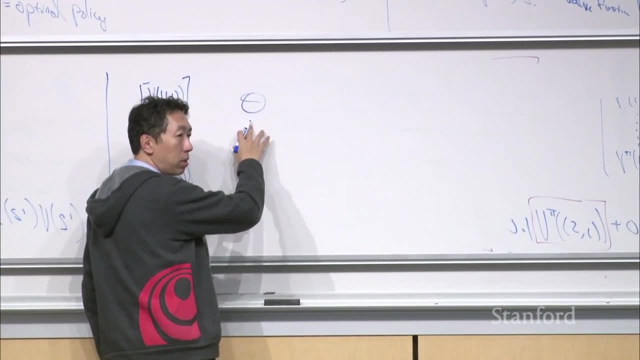 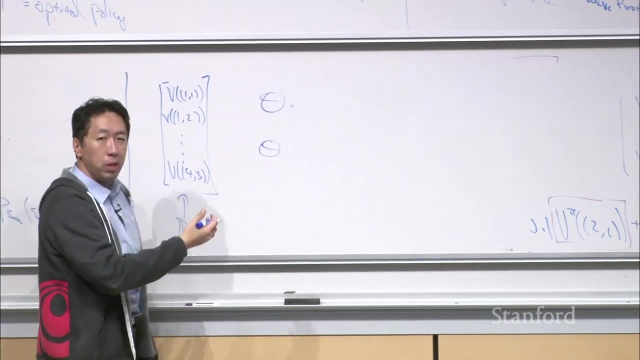 Um and similar to- similar to gradient descent. right, We've written out, you know, a gradient descent rule for updating the theta: uh, the- the vector parameters theta, And what you do is you know and you have um, and what you do is you update all of the components of theta simultaneously, right? 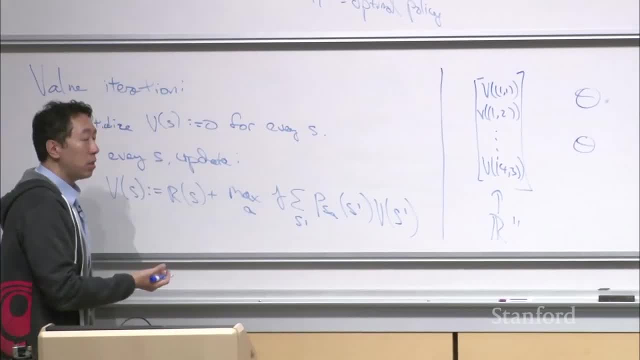 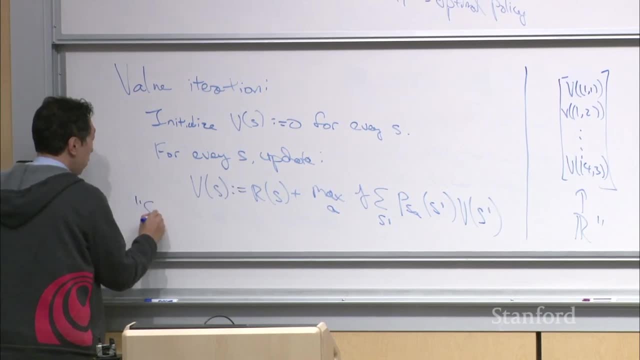 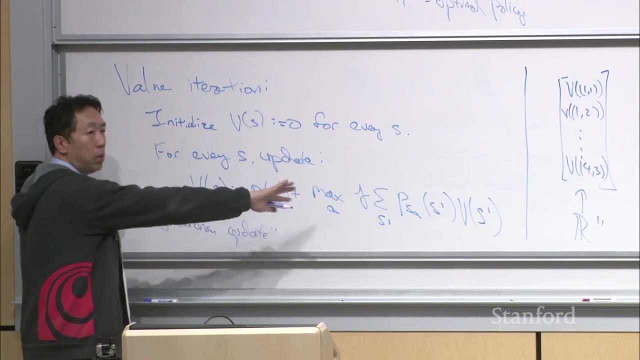 And so that's called a synchronous update. uh, in gradient descent. So one way to- so the way you would um uh update this equation in what's called a synchronous update would be, if you compute the right-hand side, for all 11 states. 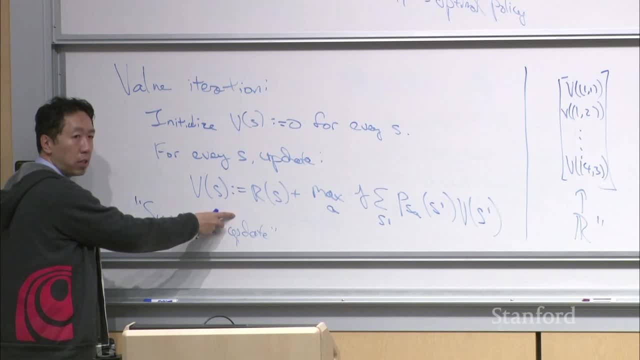 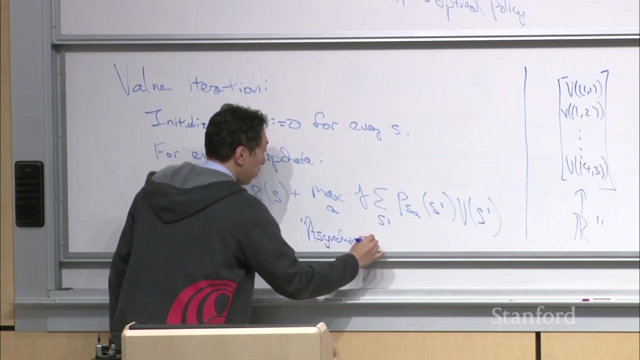 and then you simultaneously overwrite all 11 values at the same time, and then you compute all 11 values for the right-hand side and then you simultaneously update all 11 values. okay, Um, the alternative would be an asynchronous update And an asynchronous update. 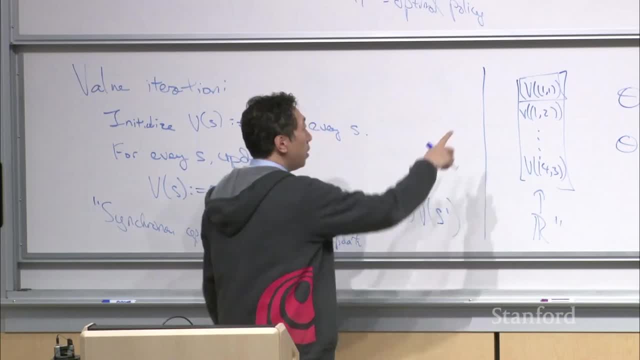 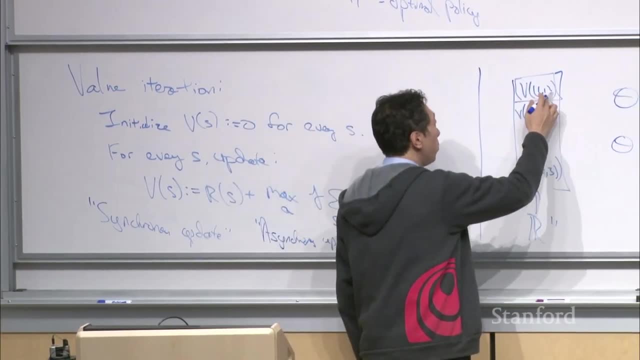 what you do is you compute Vf 1, 1, right, And the value of Vf 1, 1 depends on some of the other values on the right-hand side. Right But the asynchronous update You compute V of 1, 1 and then you would overwrite this value first. 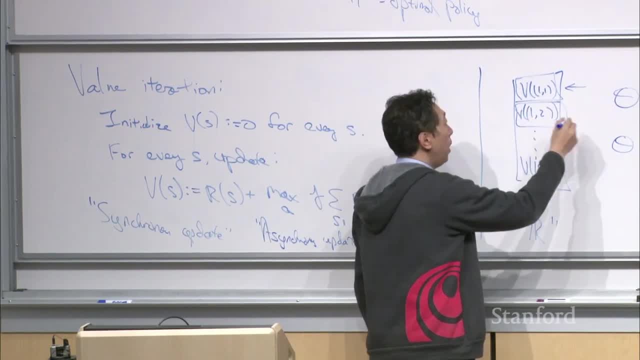 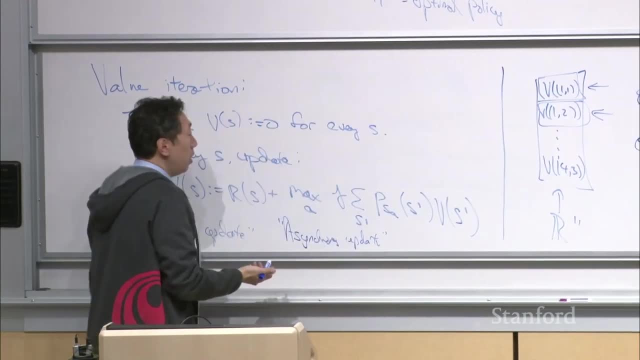 And then you use that equation to compute V of 1, 2, and then you update this, and then you sort of update these one at a time, And the difference between synchronous and asynchronous is, um, you know, if you're using asynchronous update, 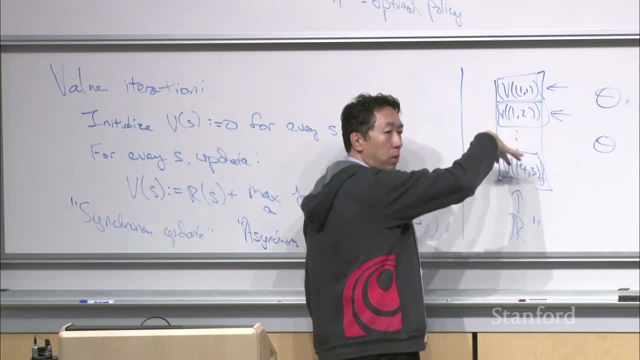 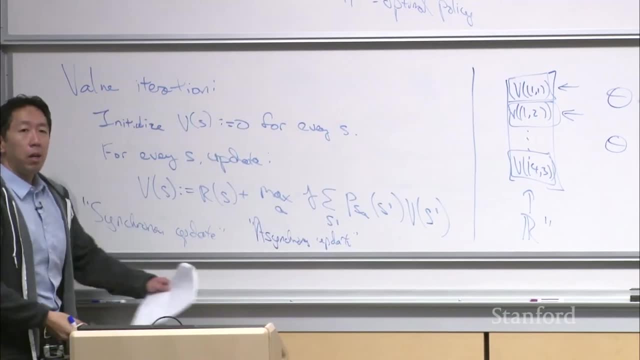 by the time you're using V of 4, 3, which depends on some of the earlier values, you'd be using a new and refreshed value of some of the earlier values on your list. Okay, Um, it turns out that value iteration works fine with either synchronous updates or asynchronous updates. 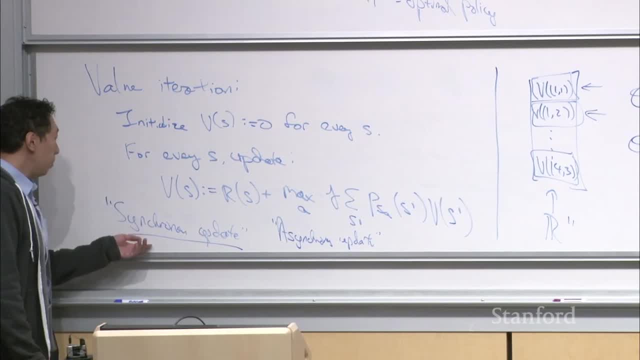 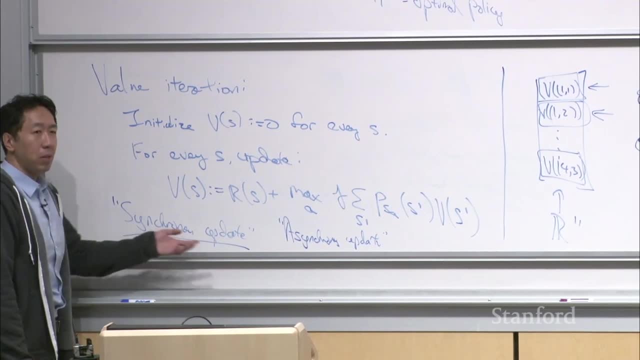 But um for the uh uh, but um uh. because it vectorizes better, because you can use more efficient matrix operations. most people use a synchronous update, But it turns out that the algorithm will work whether you use an asynchronous or an asynchronous update. 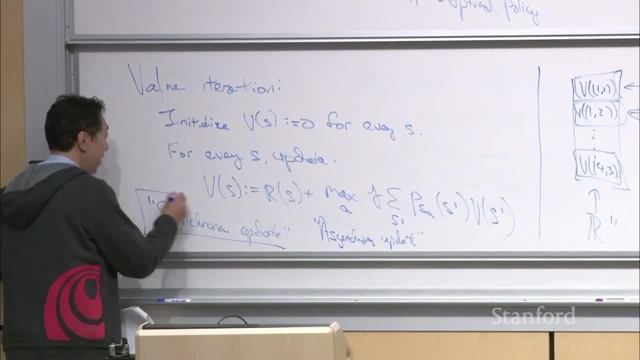 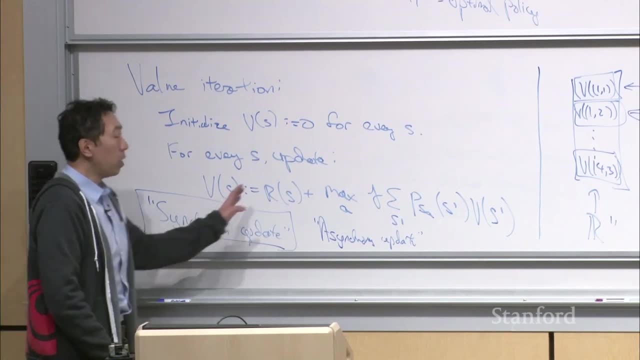 So I- I guess, unless- unless, otherwise, uh, uh, you know- stated. you should usually assume that when I talk about um value iteration, that I'm referring to synchronous update, where you compute all the values- all 11 values- using the- and- and then update all 11 values at the same time. 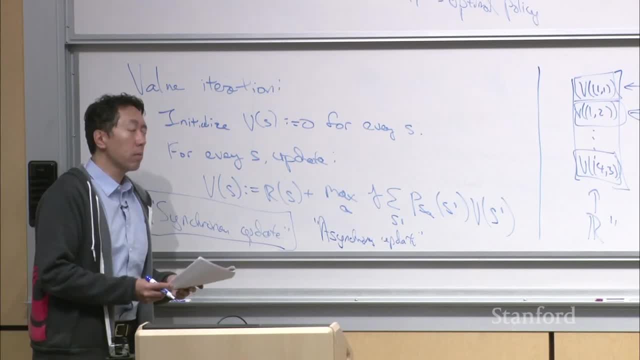 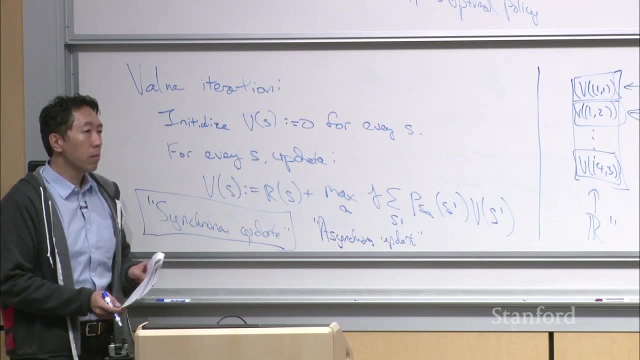 Okay, Is there a question just now Somewhere there? Yeah, So in our specific MVP we also have these two, uh same states where you got there and those simulations ended. Uh, would we represent that by saying that, like, the transition probability from those to any other state is zero? 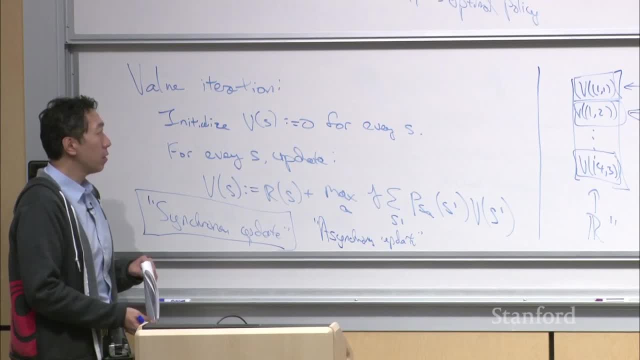 I see, Or is there a way to kind of like, you know hard code, but actually we don't want to, you know, maximize over any subsequent states when we make that? that's true, Yeah, Yes, So I think, uh. 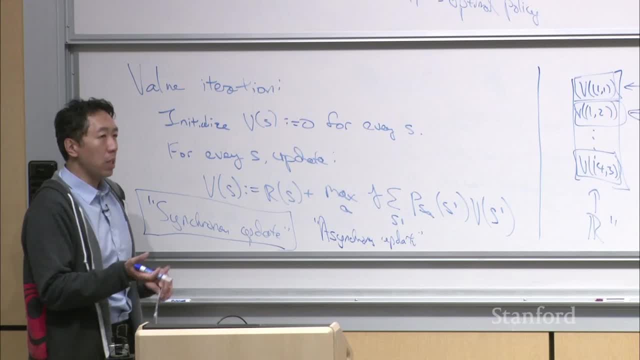 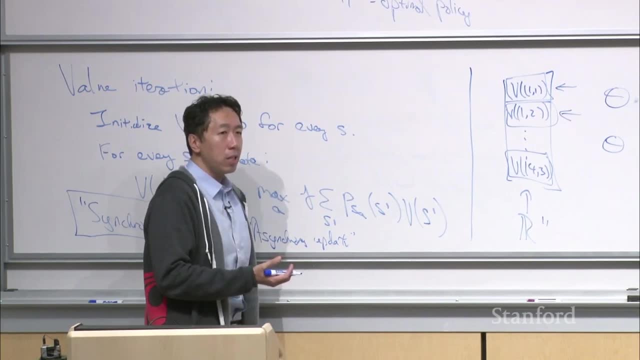 there- there, uh, uh, yes. So how do you represent the absorbing state, the sink state? We get the plus one minus one. then the world ends. Um. in this framework, one way to code that up would be to say that: 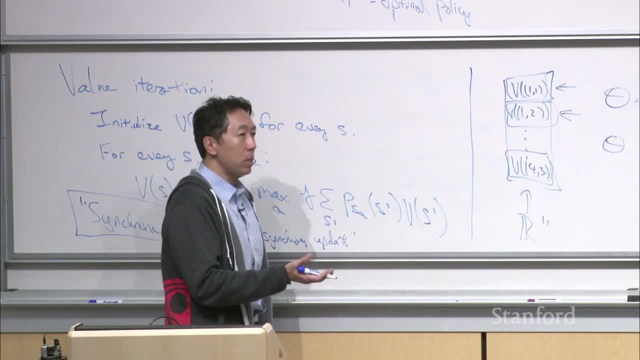 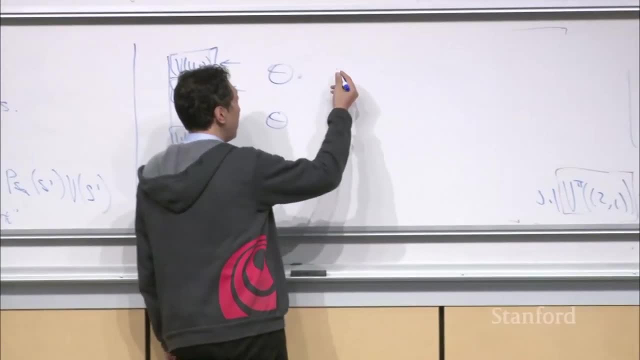 um, the state transfer from that to any other state is zero. That's one way to- to- to- that- that will work. Um, another way would be: um less- done, less often, maybe a little bit cleaner. 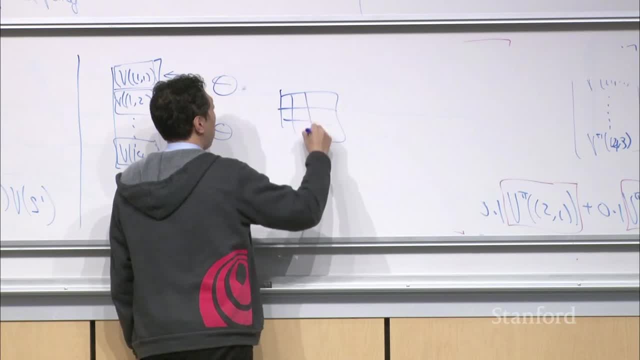 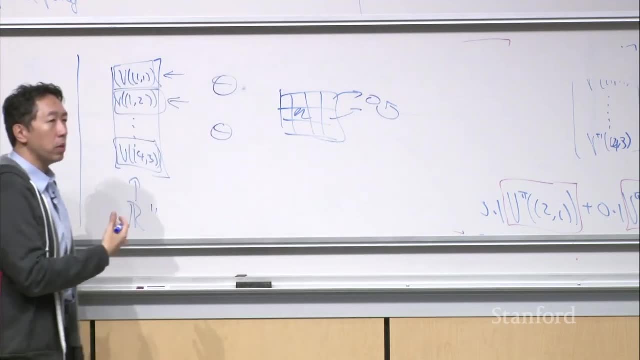 but not how people tend to do. this would be to take your um 11 state MDP and then create a 12 state, and the 12 state always goes back to itself with no further reward. So both- both of these will give you the same result. 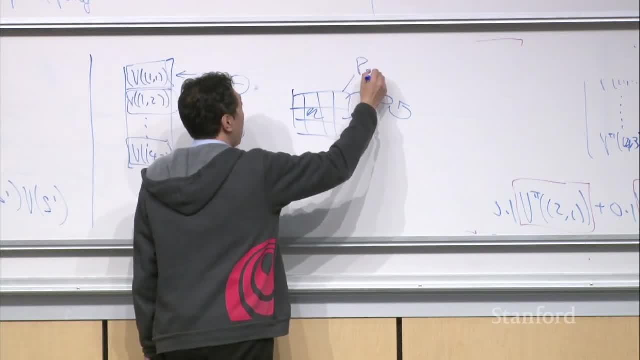 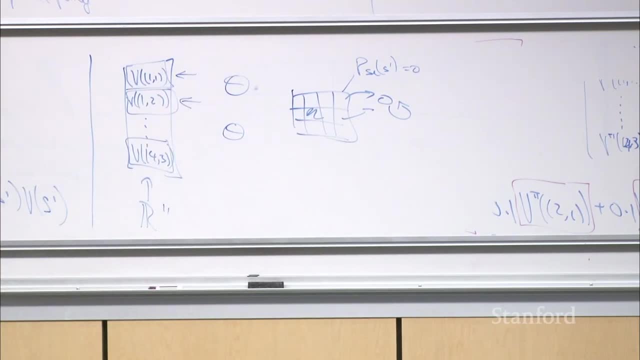 Uh, mathematics is pretty more convenient to just set, you know, PFSA as prime equals zero for all other states. Um, it's not quite a state transfer probability, but that- that will give you the variance as well. Yeah Thanks, All right, Cool. 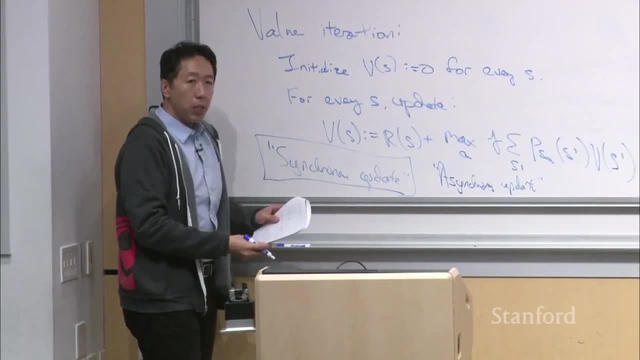 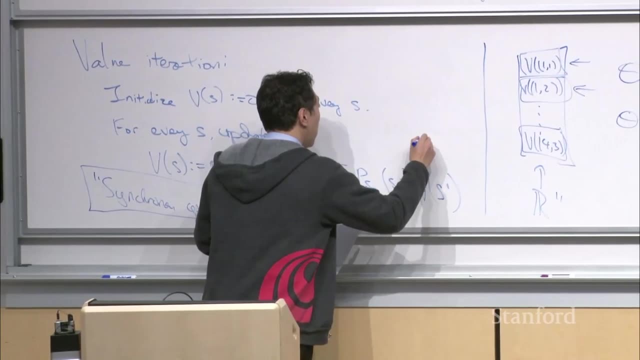 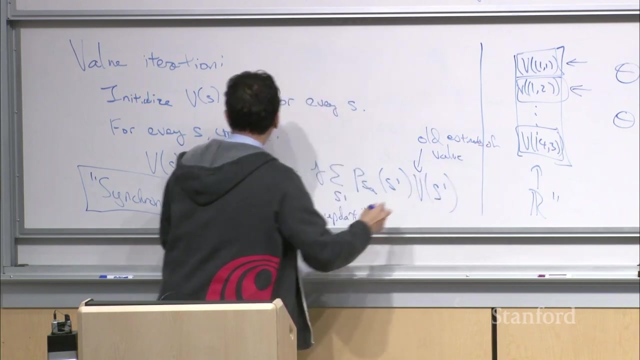 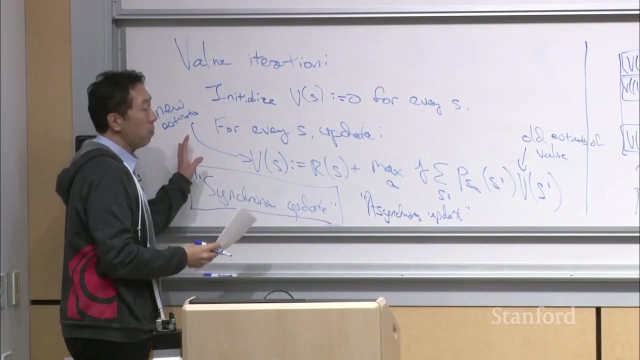 Um, so, just as a point of notation, if you're using synchronous updates, you can think of this as, um, taking the old value function- uh, old estimate right- And using it to compute the new estimates, right. So this- this you know. 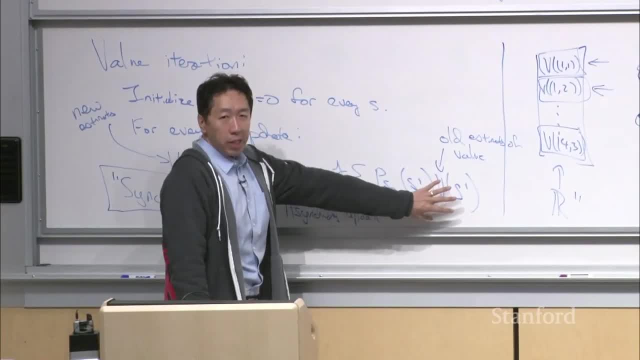 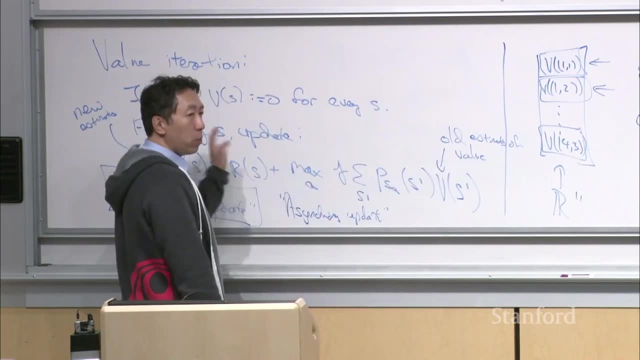 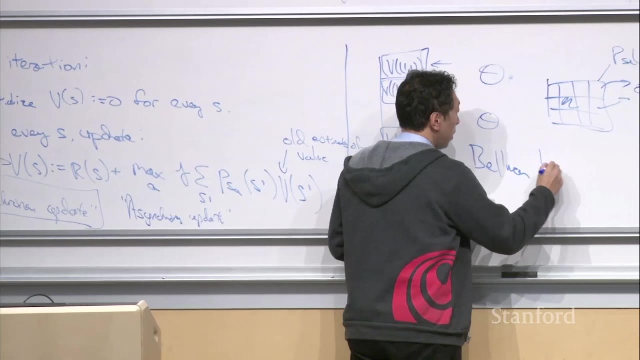 assuming the synchronous update, you have some uh previous 11-dimensional vector with your estimates of the value from the previous iteration And after doing one iteration of this you have a new set of estimates. So one step of this algorithm is sometimes called the Bellman Backup Operator. 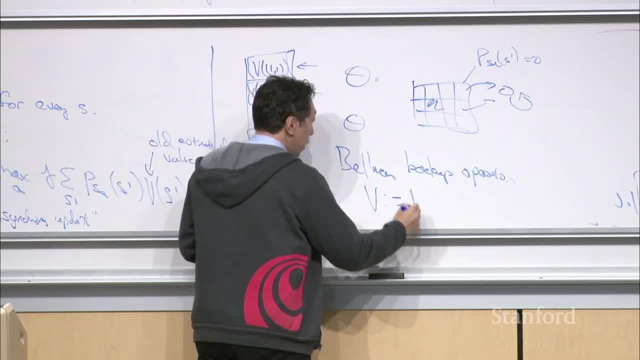 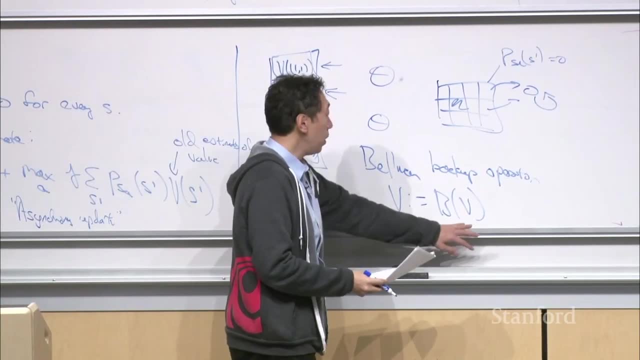 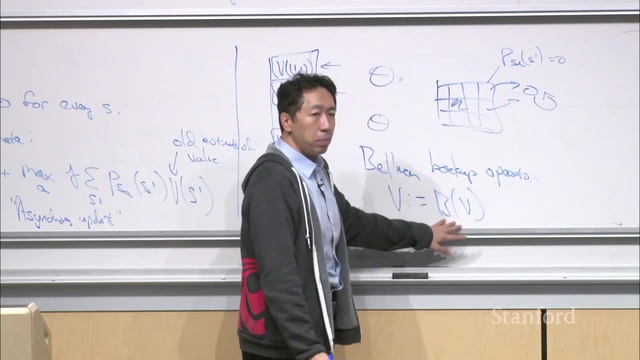 And so where you update v equals b of v, right, Where uh, where now v is a 11-dimensional vector. So you have an old 11-dimensional vector. compute the Bellman Backup Operator with just that equation there and update v according to b of v, Um and so. 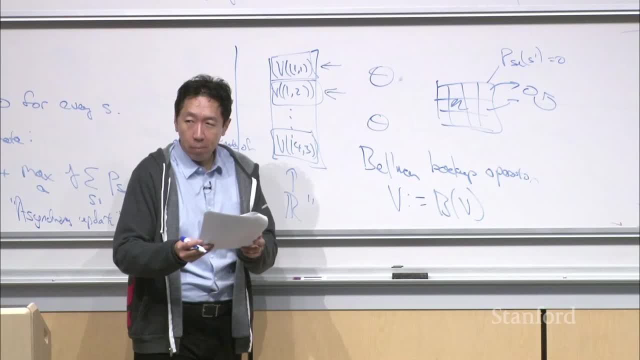 one thing that you see in the um problem set- uh is prove- is uh uh showing that um, this will make a v of s converge to v star. okay, So it turns out that um 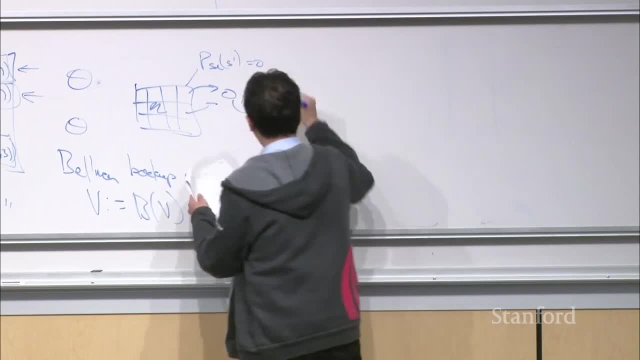 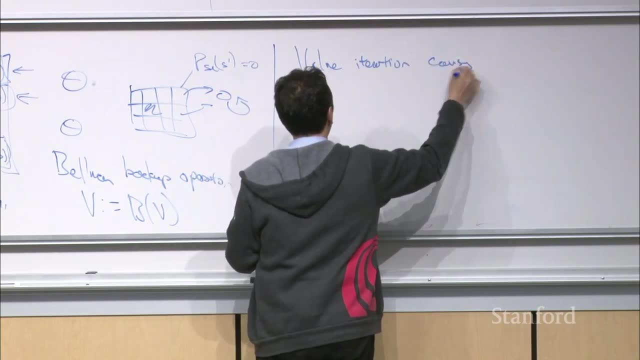 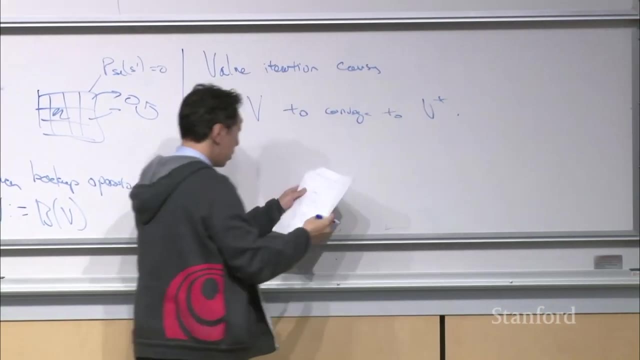 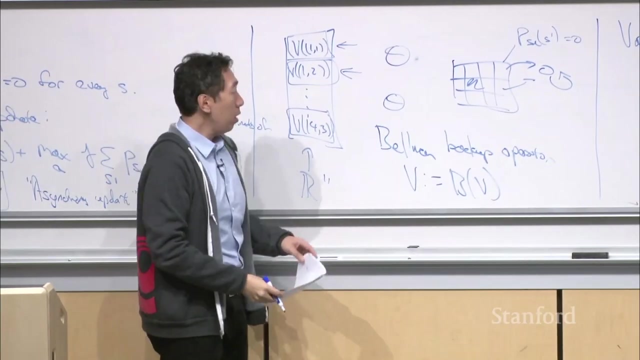 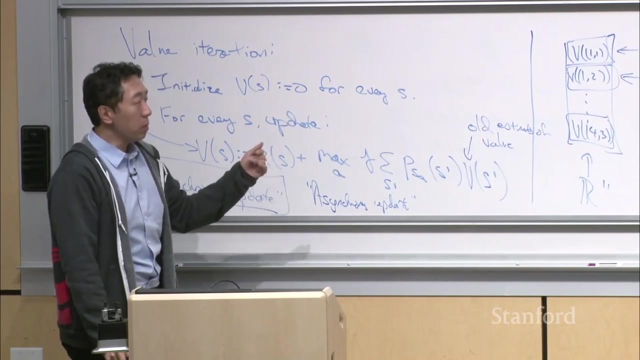 Okay, So it turns out that, um, uh, you can prove- and you see more details of this in the problem set- that by repeatedly enforcing Bellman's uh equations, that this equi- this- this algorithm will cause your vector of 11 values. 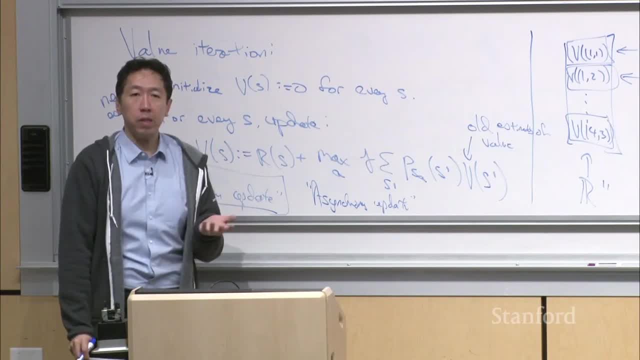 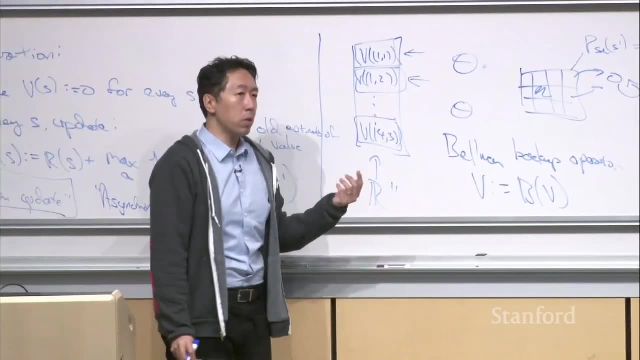 so it'll cause v to converge to the optimal value. function v star. Okay, Um and more details you- you see in the homework, a little bit in the lecture notes, And it turns out this algorithm actually converges quite quickly, right? 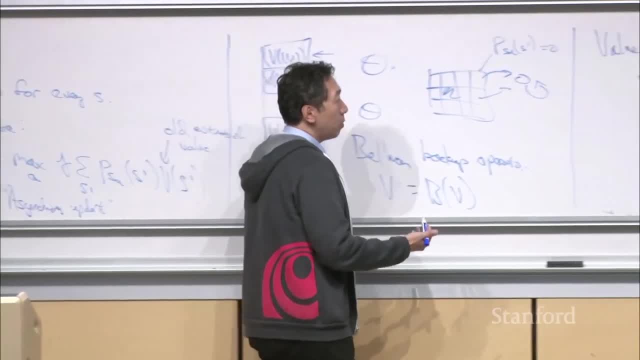 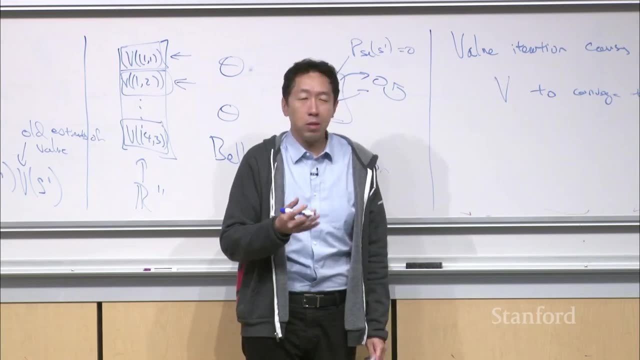 Um, to- to-, to give you a flavor, I think that, uh, with the discount factor, if the discount factor is 0.99, it turns out that you can show that the error uh reduces, you know. 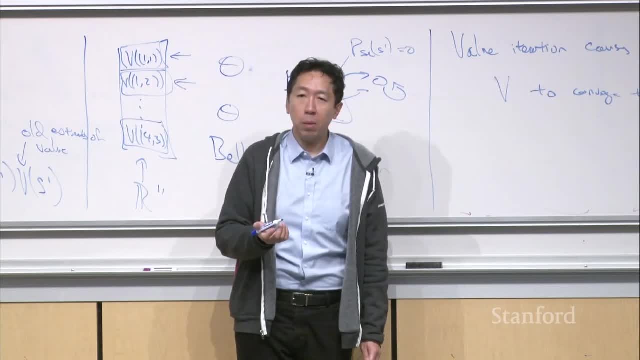 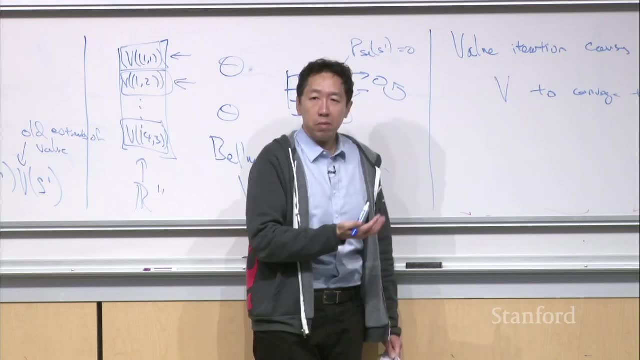 by a factor of 0.99 on every iteration Um and so v, actually converges quite quickly, geometrically quickly or exponentially quickly um to the optimal value function v star, And so this: you know, the discount factor is 0.99,. 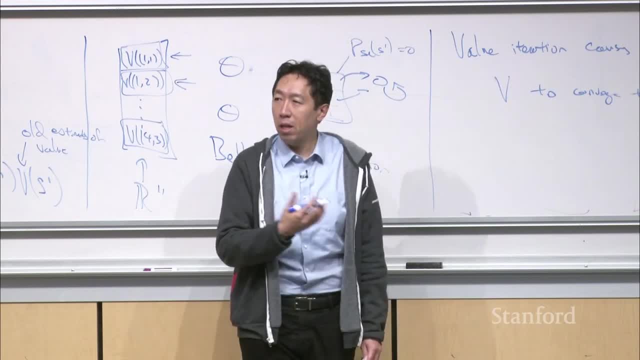 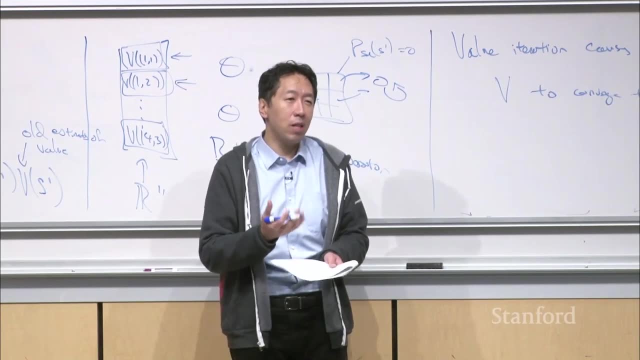 then with, like a few- with a hundred iterations or a few hundred iterations, v would be very close to v star- Okay, And- and the discount factor is 0.9, then with, just you know, 10 or a few dozens of iterations. 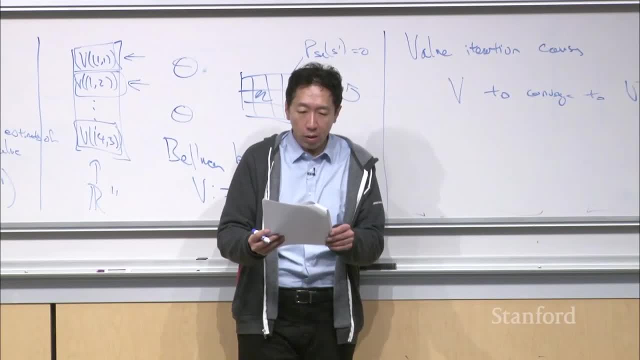 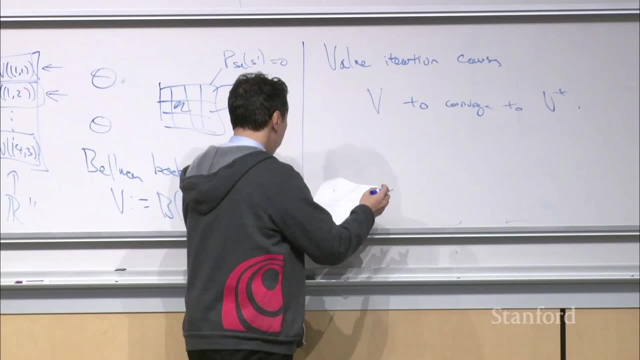 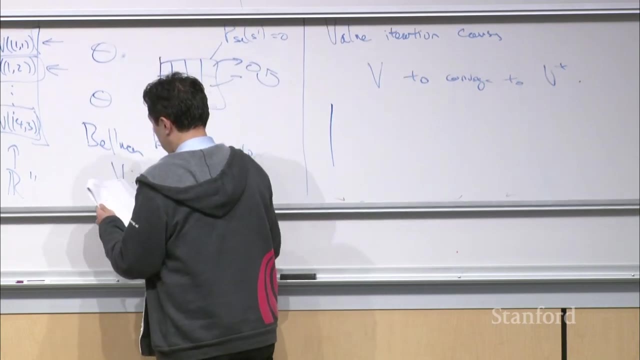 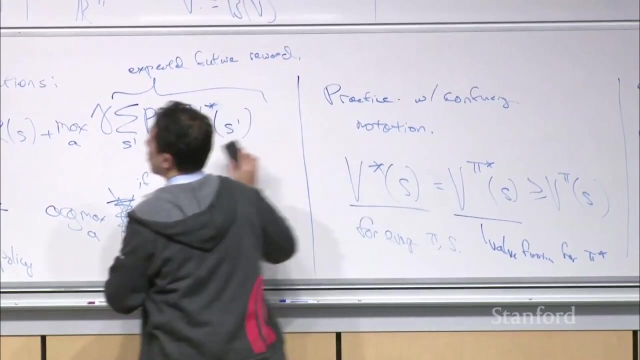 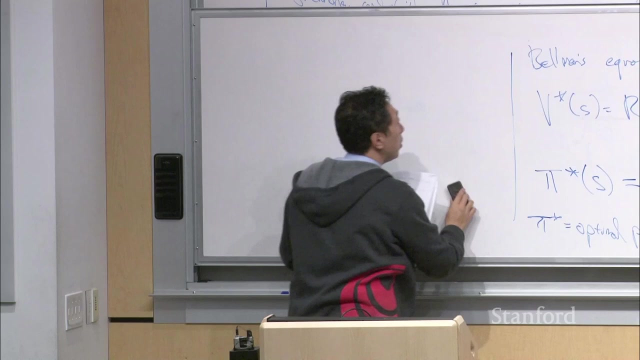 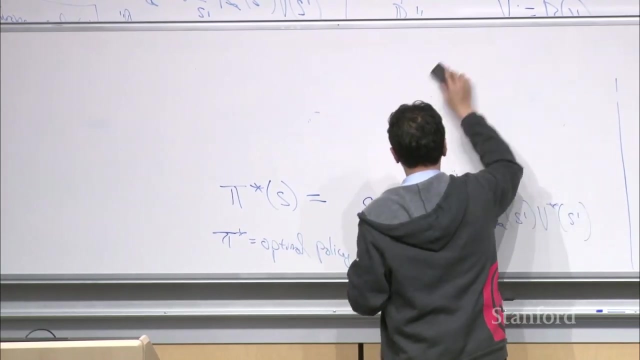 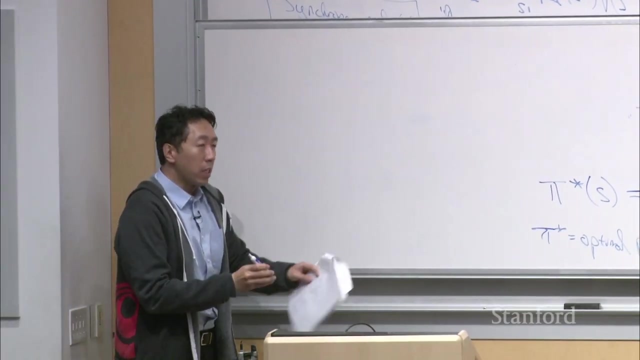 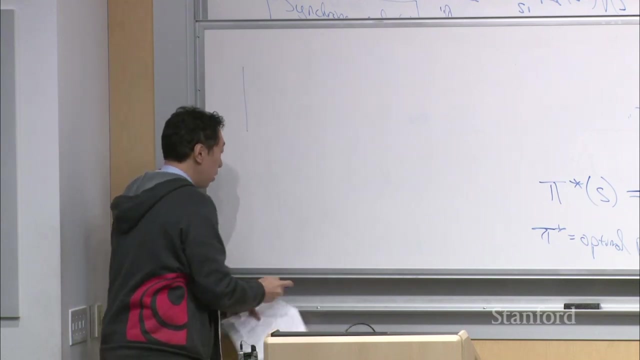 it'll be very close to v star, So this algorithm actually converges quite quickly to v star. Okay, Um so let's see All right. Um so, just to put everything together: Um, if you- Uh, if you run value iteration on that MDP. 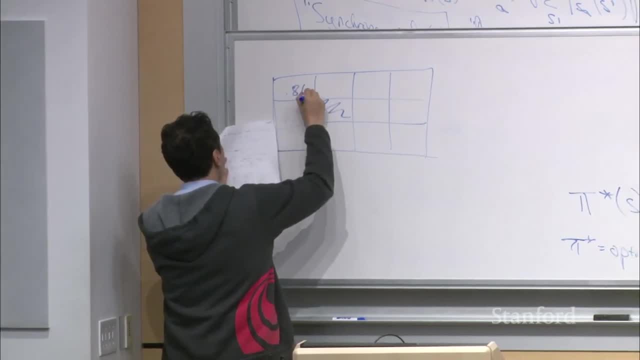 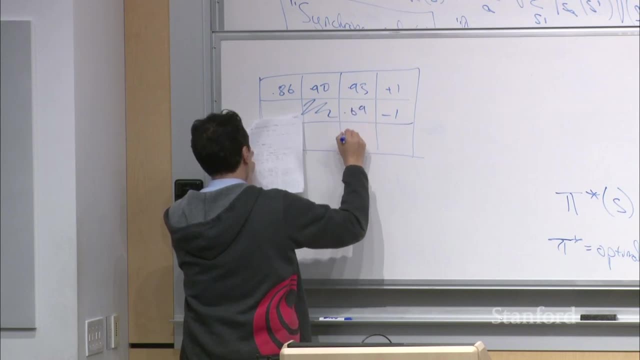 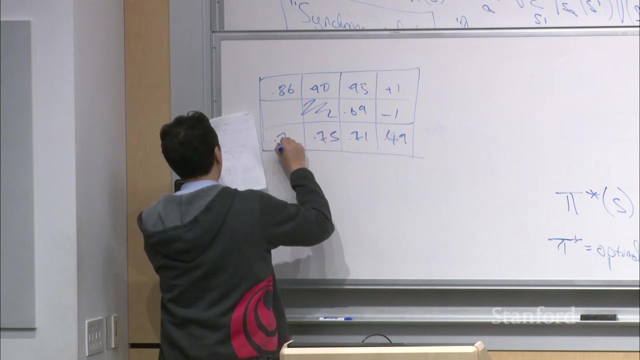 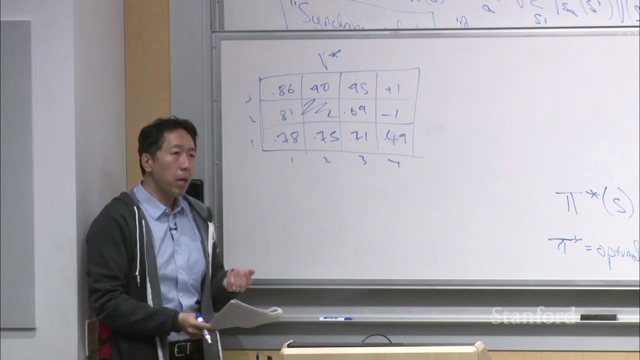 you end up with this: um Uh, so this is V star. okay, So it's a list of 11 numbers telling you what is the optimal um expected payoff for starting off in each of the 11. 11 possible states. 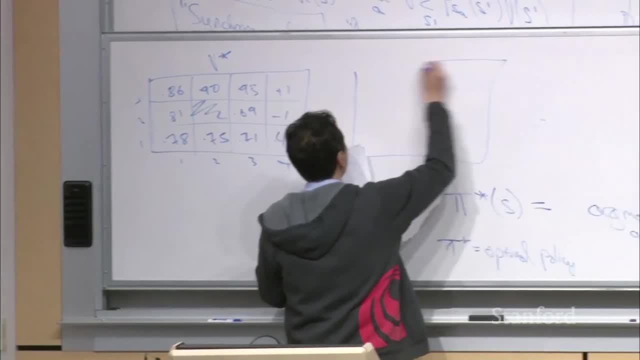 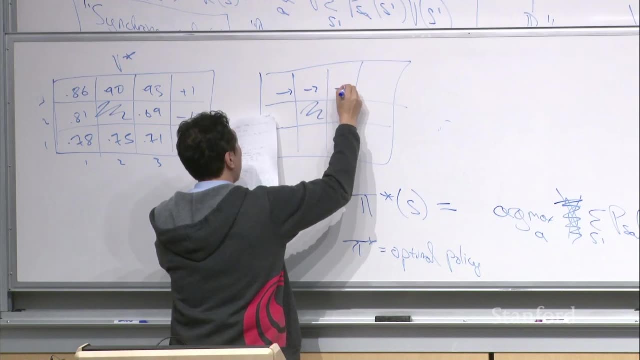 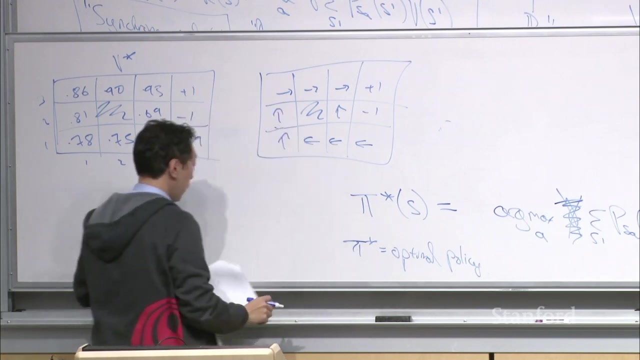 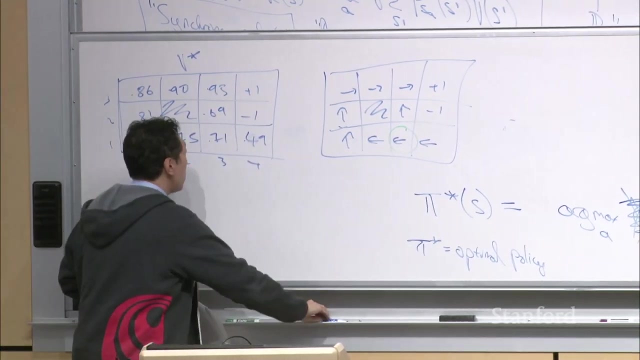 And so, um, I had previously said- I think I said last week, uh, of the week before Thanksgiving- that this is the optimal policy, right? So you know, let's just use as a case study how you compute the optimal action for that state um. 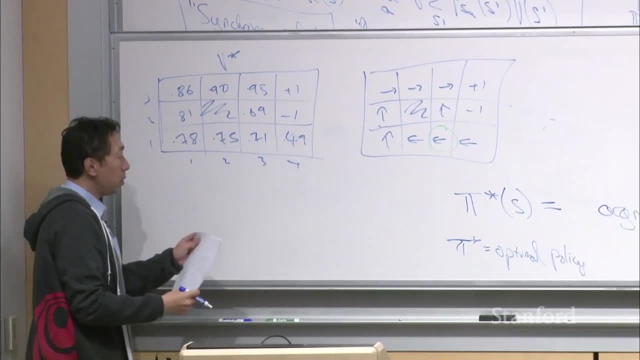 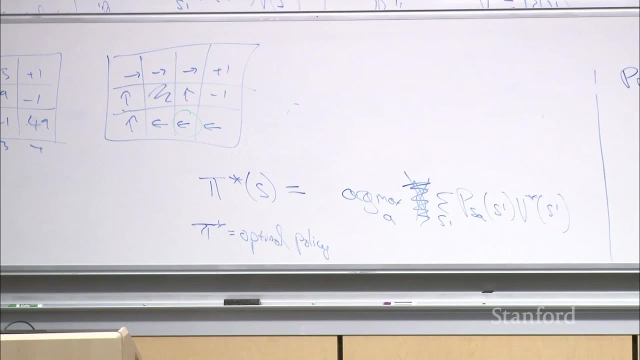 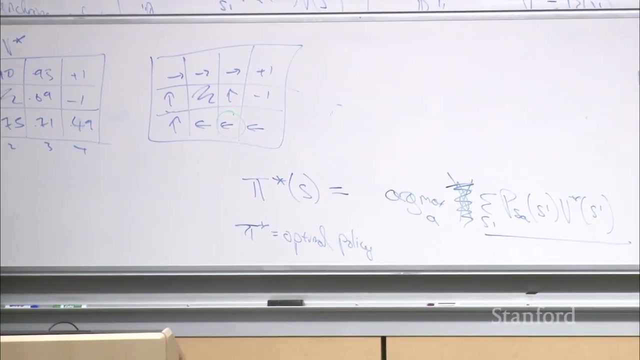 given this, this V star right, Well, what you do is you'd actually just use this equation And so, um, if you were to go west, then if you were to compute, I guess this term um sum of S prime uh. 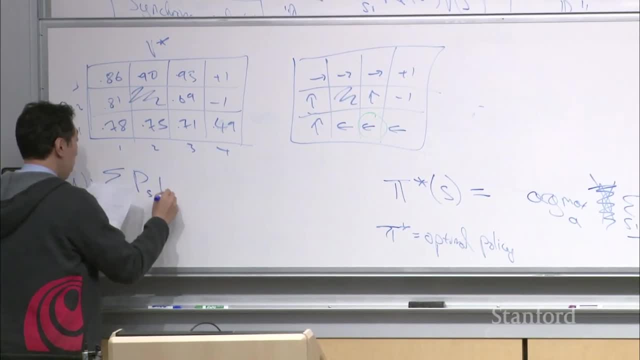 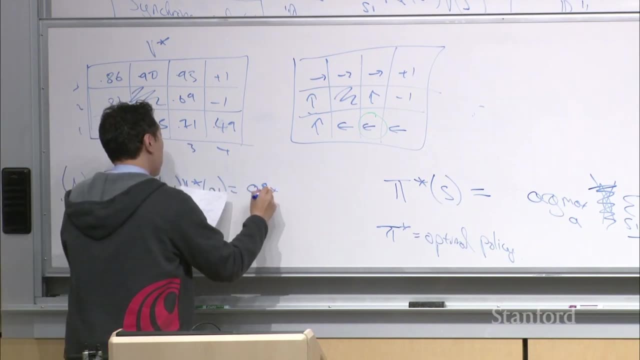 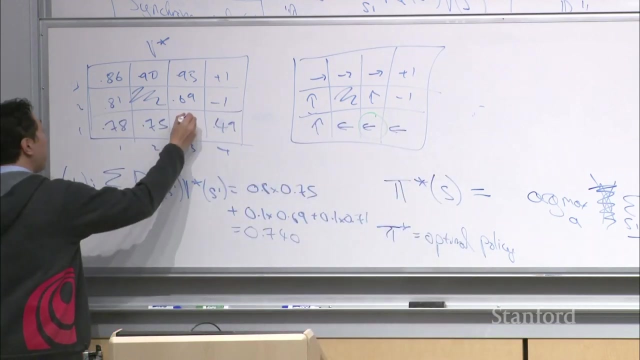 west or left? I guess right P of S A, S prime, V, star of S prime is equal to um. if you were to go west, you have a um right, um right. So if you're in this state and if you attempt to go left, 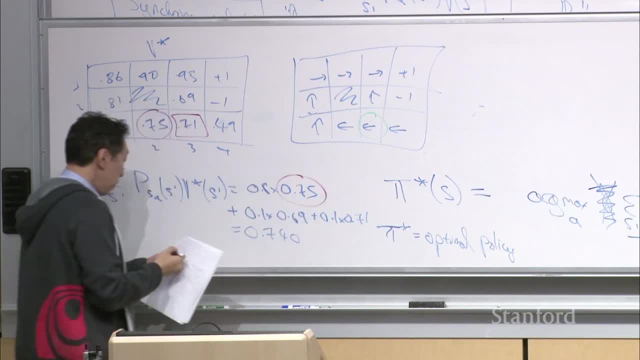 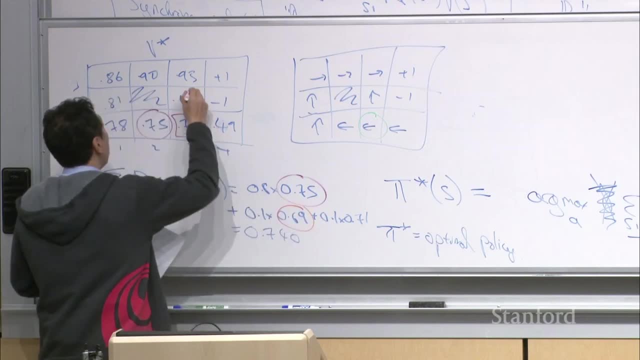 then there's a 0.8 chance you end up there with uh uh V star of 0.6.. 0.75, there's a 0.1 chance, you know, if you try to go left. 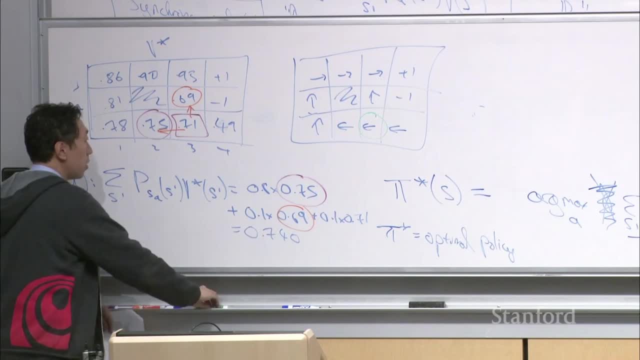 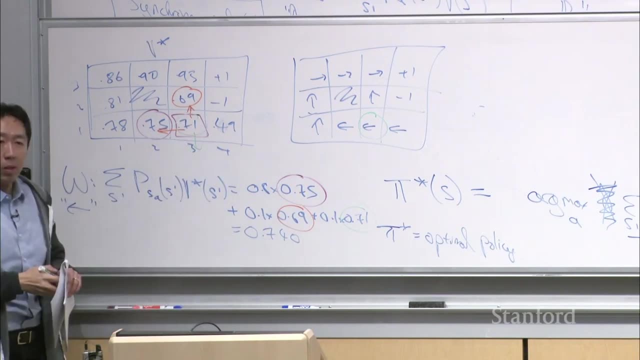 there's a 0.1 chance you veer off to the north and have a 0.69.. And then there's a 0.1 chance that you actually go south and bounce off the wall and end up with a 0.71.. 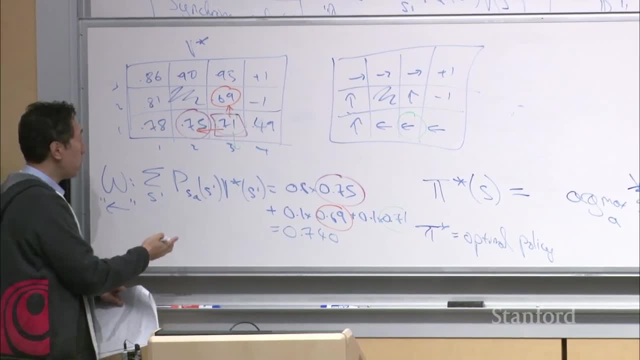 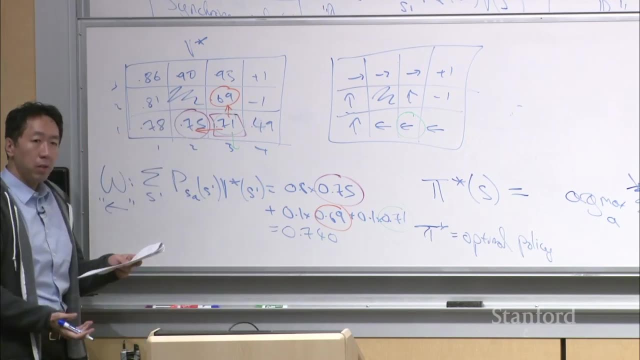 And so the expected uh future rewards, expected future payoff. given this equation is that if you attempt to go west, you end up with uh 0.740 as expected future rewards, Whereas if you were to go north, if you do a similar computation, 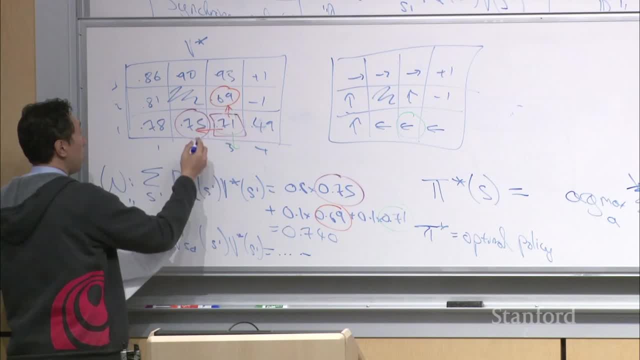 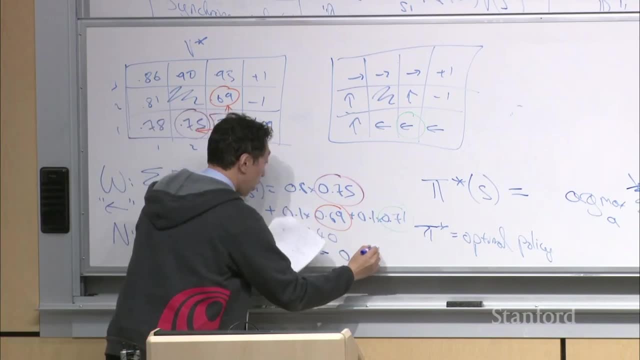 you know. so, uh, 0.8 times 0.69 plus 0.1 times 0.75, plus 0.1 times 0.49, the appropriate weighted average. you find that it's equal to 0.676,. 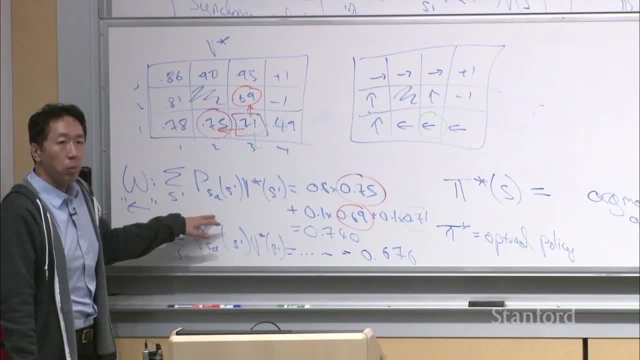 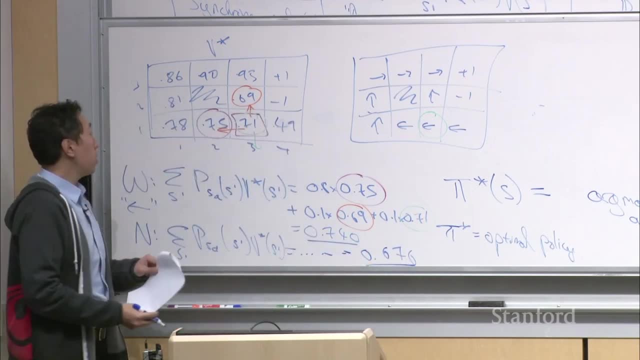 um, which is why the expected future rewards if you go west, if you go um left, is 0.740, which is quite a bit higher than if you go north, Which is why we can conclude, based on this little calculation, 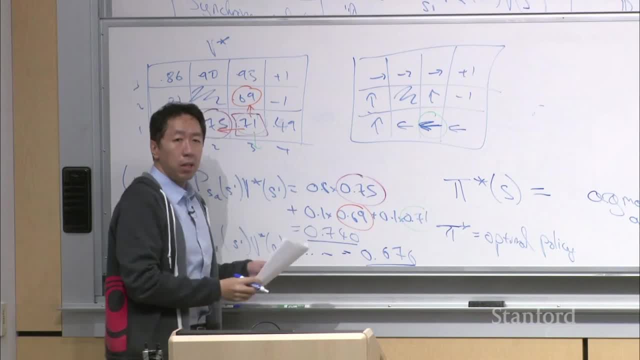 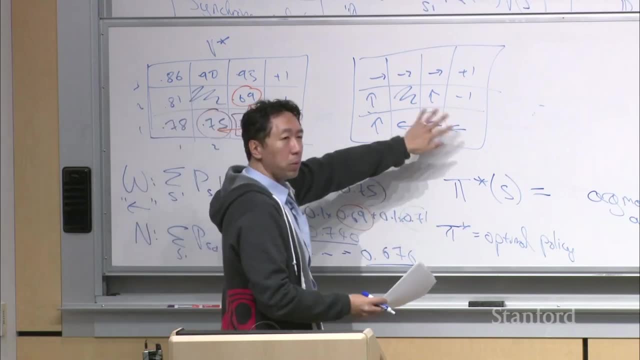 um, that the optimal policy is to go left at that state. okay, And- and really- and technically, you check north, south, east and west and make sure that going west gives a higher reward, And that's how you can conclude that going west is actually the better action at this state. 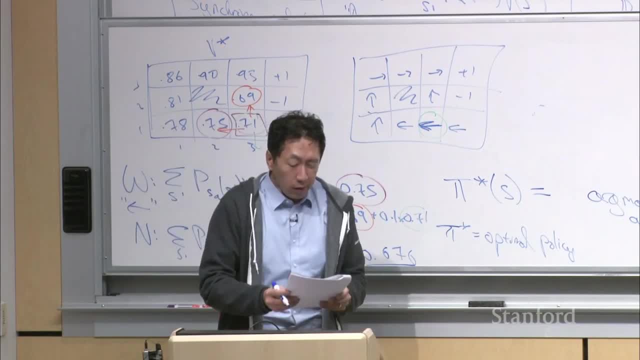 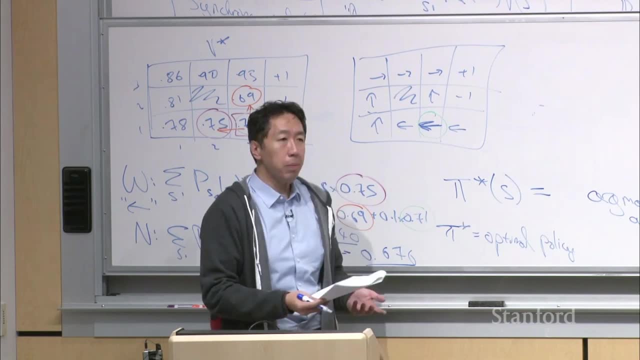 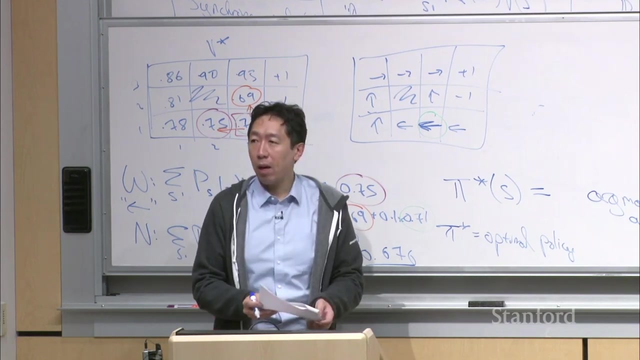 Okay, So that's value iteration And um. based on this, if you um uh are given an MDP, you can implement this, uh solve for V star and uh uh be able to uh compute Pi star. okay. 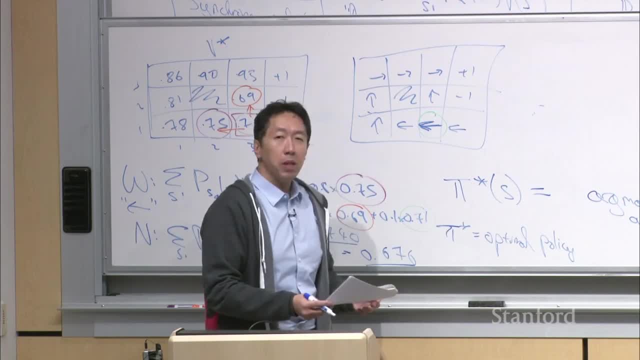 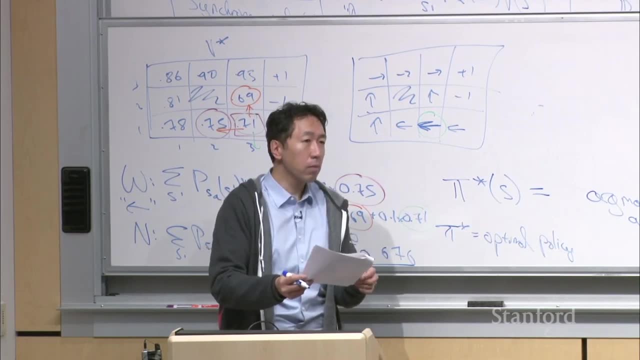 All right, Um, a few more things I want to go over, but before I move on, uh, let me check if there are any questions. Yeah, Oh sure, Yep, Uh. is the number of states always finite? 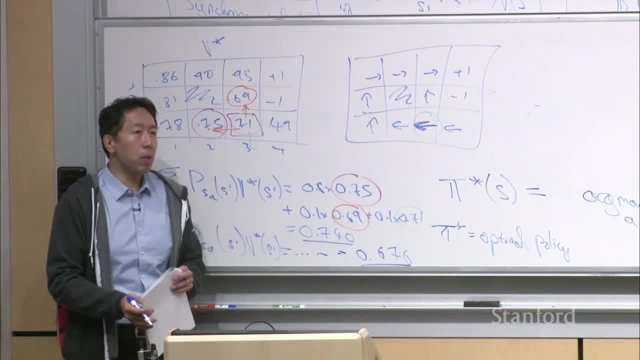 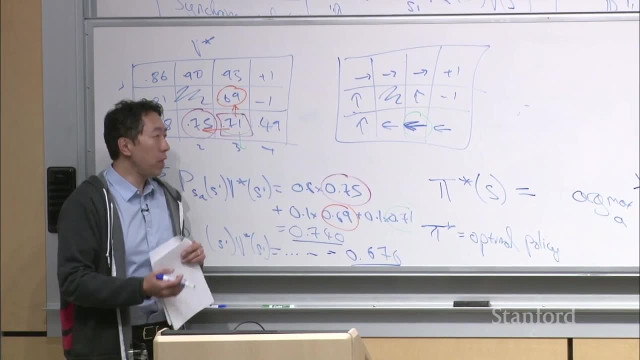 So, in what we're discussing so far, yes, Uh, but what we'll see on Wednesday is how to generalize this framework. I'll- I'll allude to this a little bit later, but, uh, it turns out, if you have a continuous state, MDP. 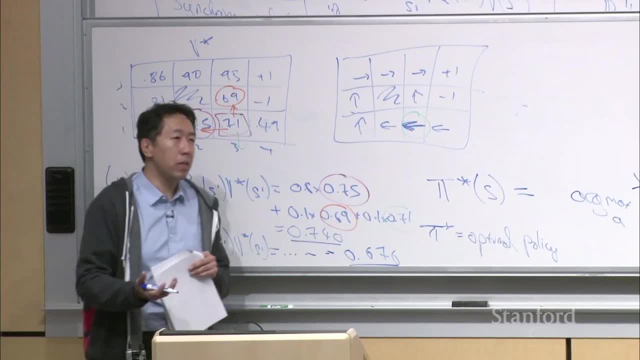 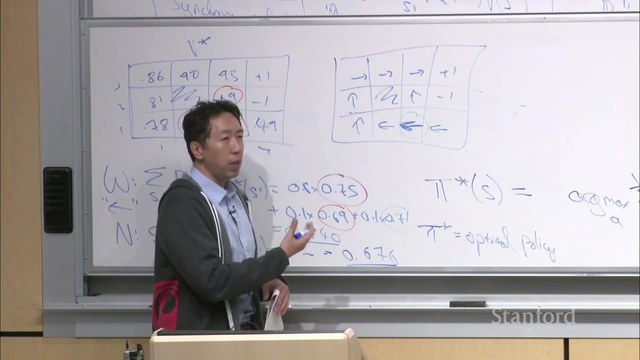 uh, one of the things that's often done, I guess, is to discretize into finite number of states. Uh, but then there are also some other versions of um, uh, you know value iteration. that applies directly to continuous states as well. 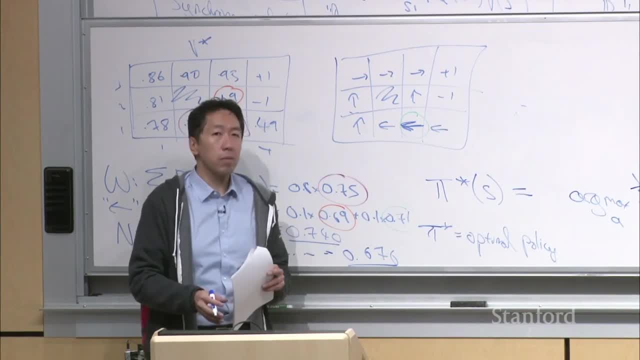 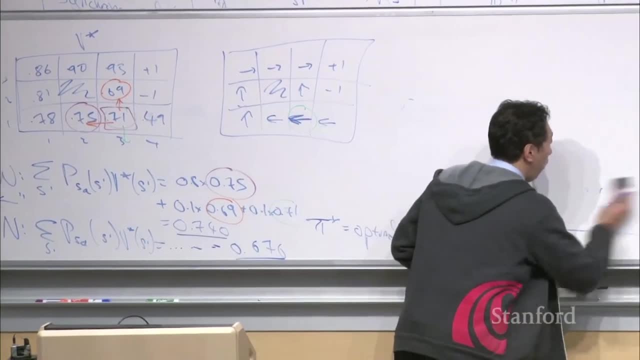 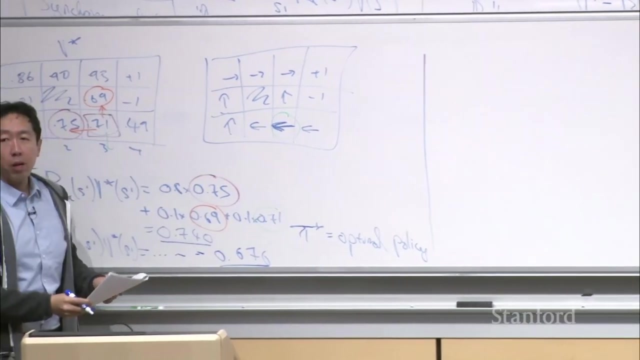 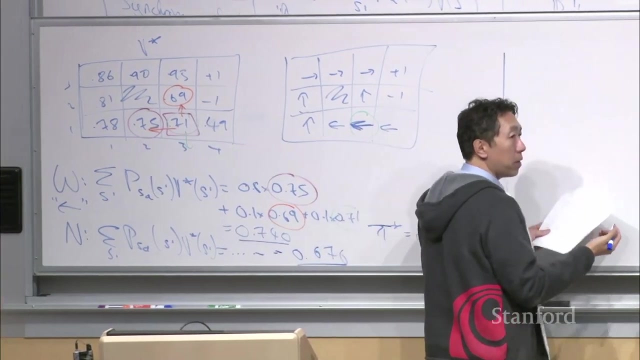 Anything else? Okay, cool, All right. So, um, what I described is an algorithm called Value Iteration. The other, um, I don't know, common, uh sort of textbook algorithm for solving for MDPs is called Policy Iteration. 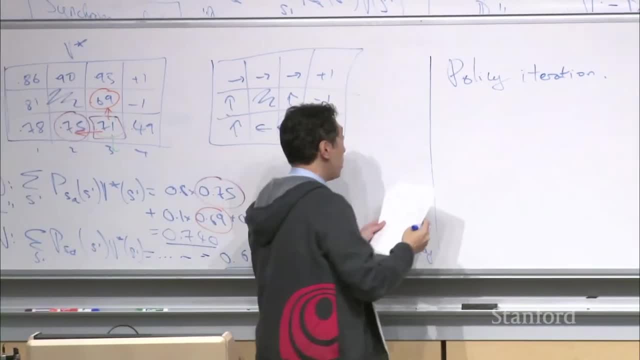 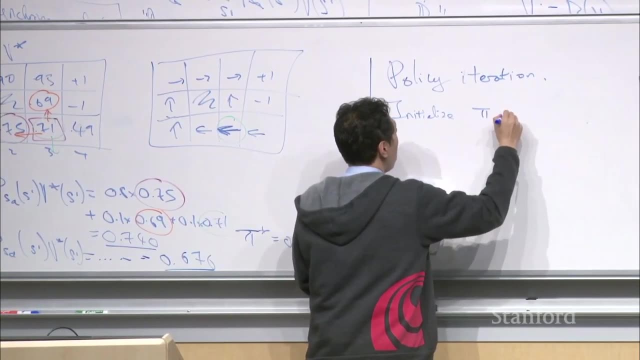 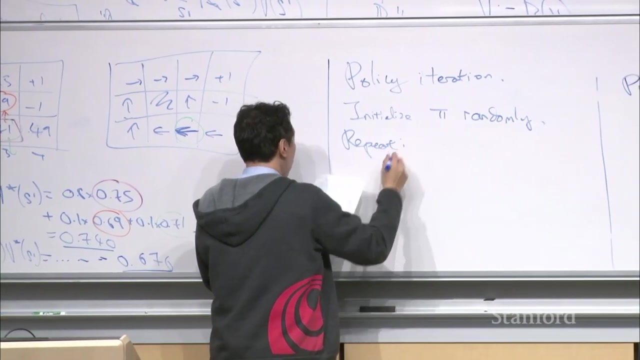 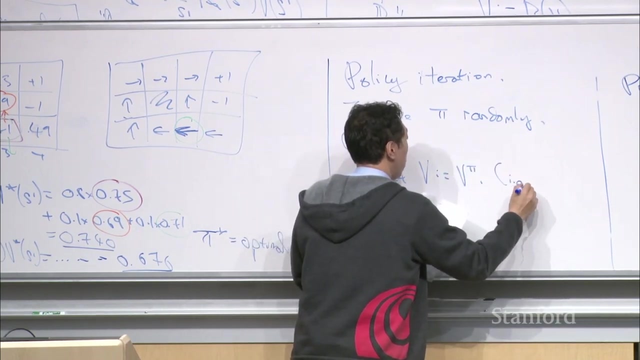 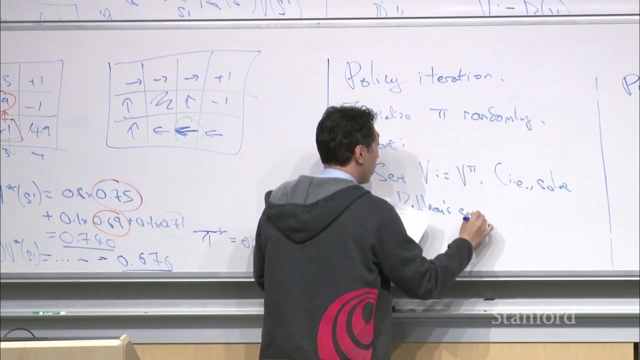 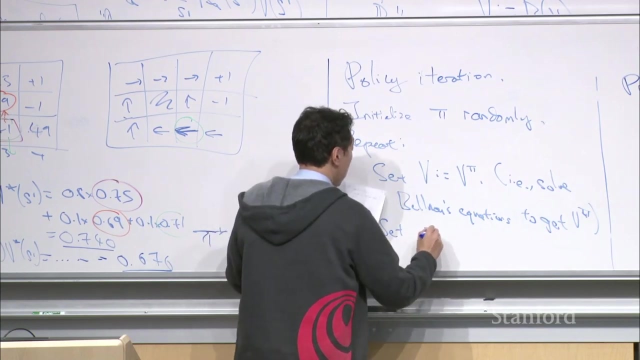 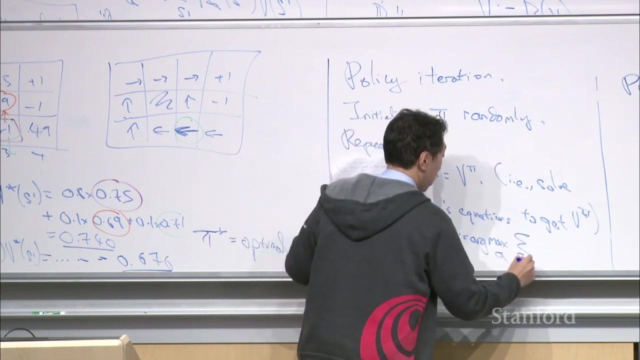 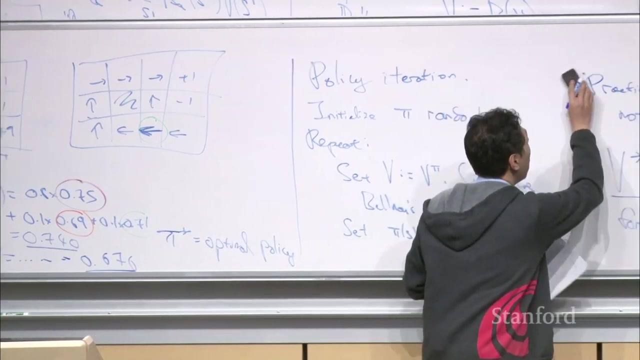 And, um, let me just- I'll just write out what the algorithm is. So here's the algorithm, which is, um you know, initialize Pi randomly, right? Uh uh, uh, uh, uh, uh uh. 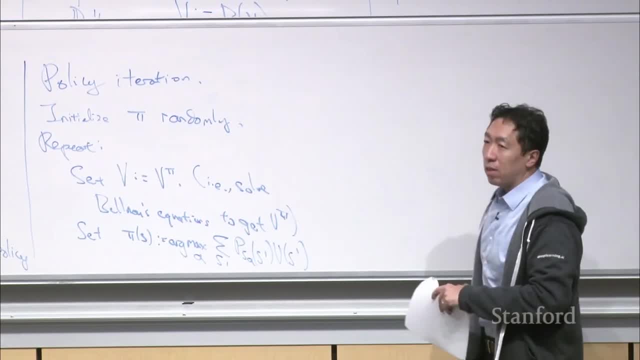 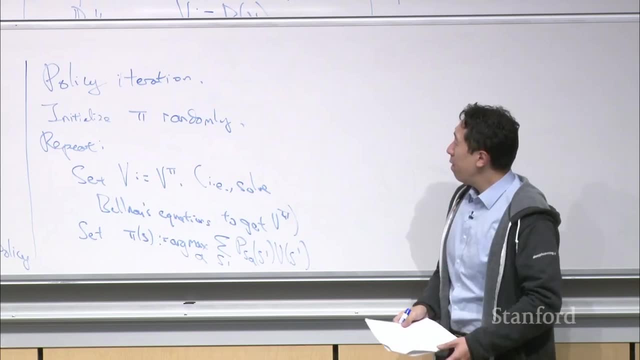 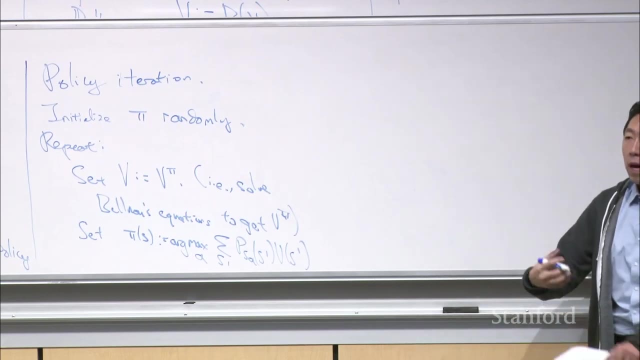 Okay, So let's see what this algorithm does. We'll talk about pros and cons of valuation versus policy iteration. a little bit Um in policy iteration, uh, instead of solving for the optimal policy v-star, so in- in value iteration. 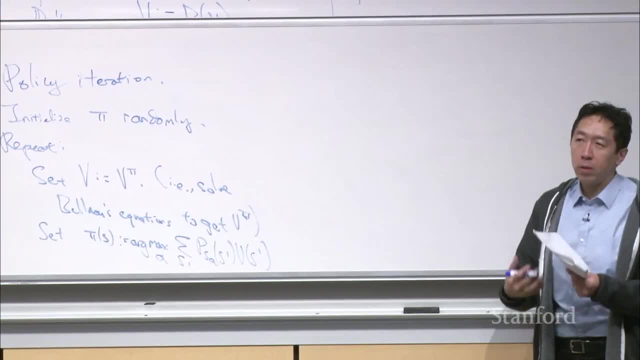 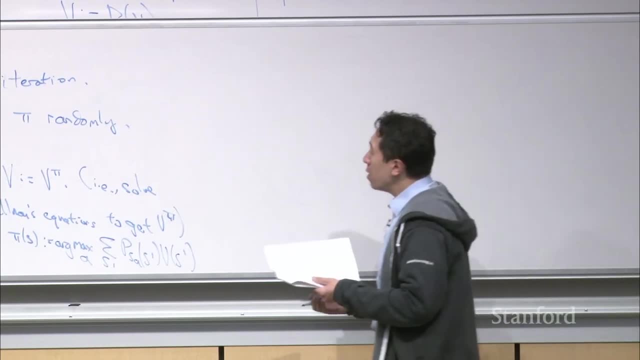 our focus of attention was v-star right Where, um you know, you do a lot of work to try to find the value function and then, once you solve for v-star, you then figure out the best policy. In policy iteration, the focus of attention is on the policy pi rather than the value function. 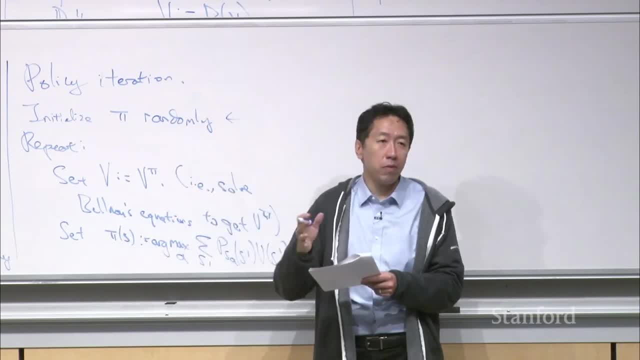 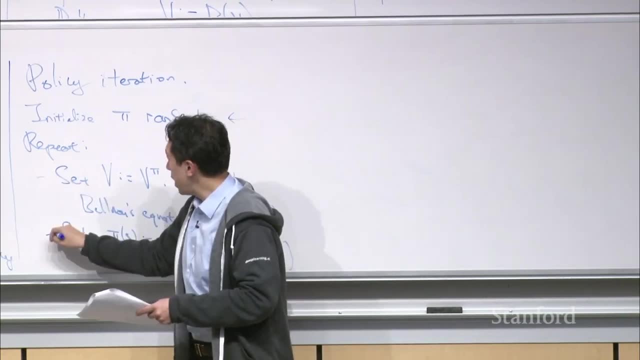 And so initialize pi randomly. So that means for- for each of the 11 states. pick a random action, right? So a random initial pi, And then we're going to repeatedly carry out these two steps, Um, the first step is: 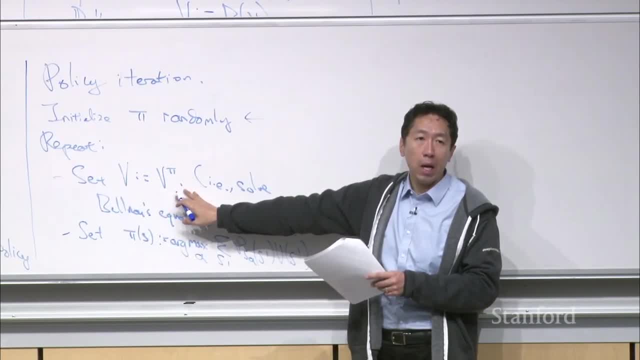 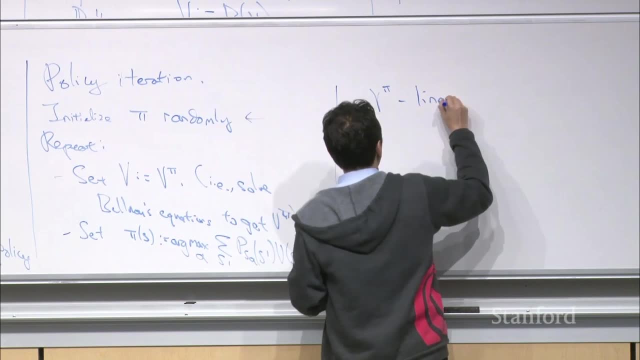 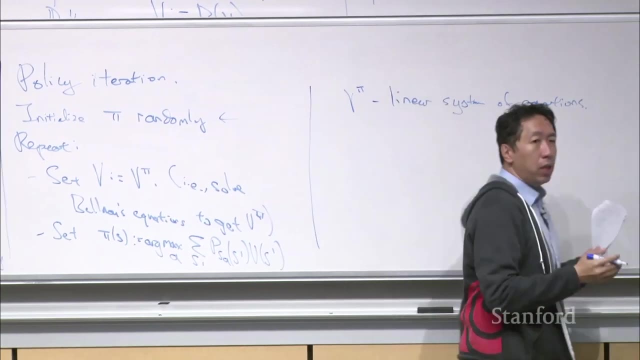 um solve for the value function for the policy pi right, And remember um for v pi. this was a linear system of equations, Right, With uh, 11 variables, with 11 unknowns, And then there's a linear system of 11 equations with 11 unknowns. 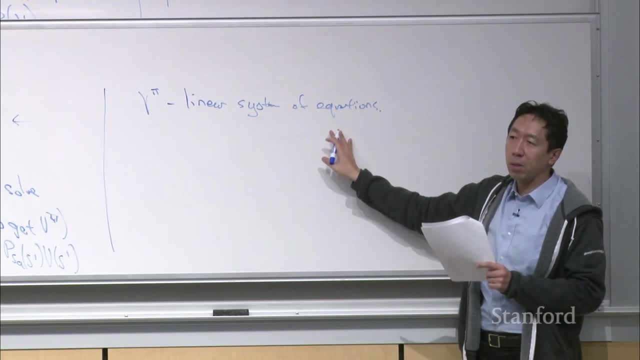 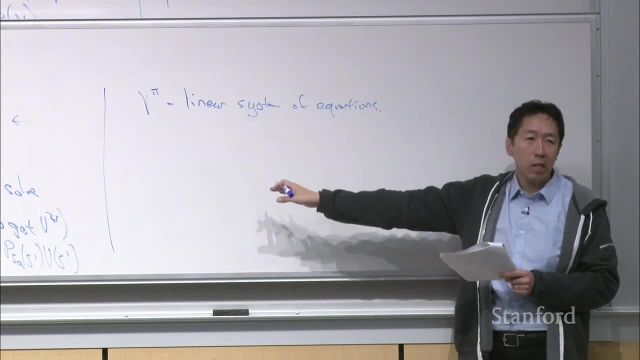 And so, using a sort of linear algebra solver or linear equation solver, given a fixed policy pi, you could just, you know, at the cost of inverting a matrix, roughly right, You could solve for- you could solve for all of these 11 values. 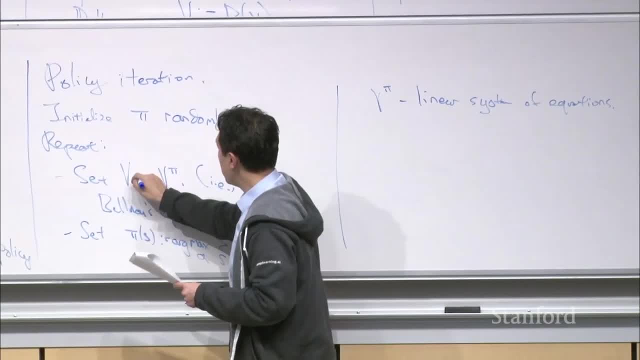 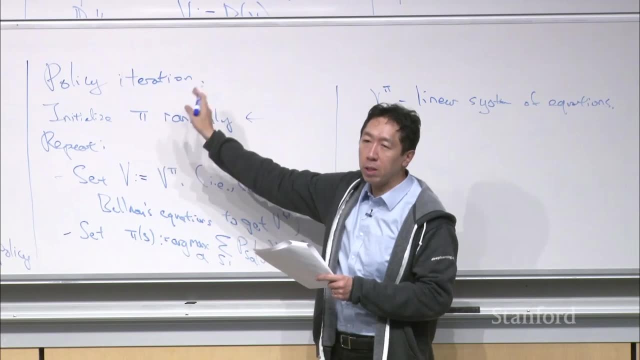 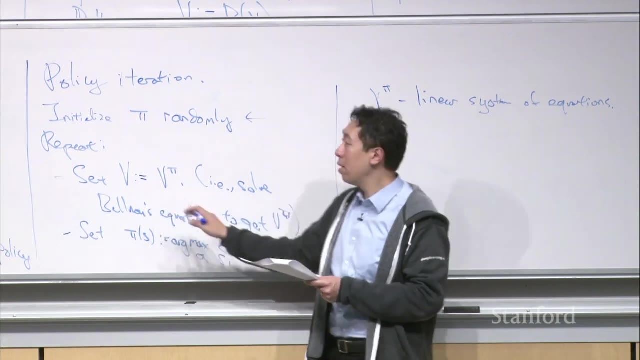 And so in policy iteration, um, you would you know, use a linear solver to solve for the optimal value function for this policy, pi that we just randomly initialize And then set v to be the value function for that policy. Okay, Um, and so this is done quite efficiently with a linear solver. 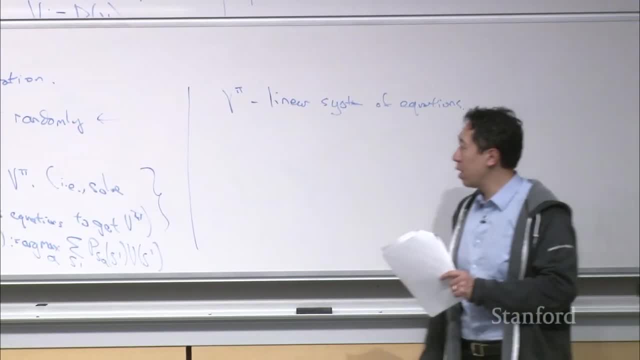 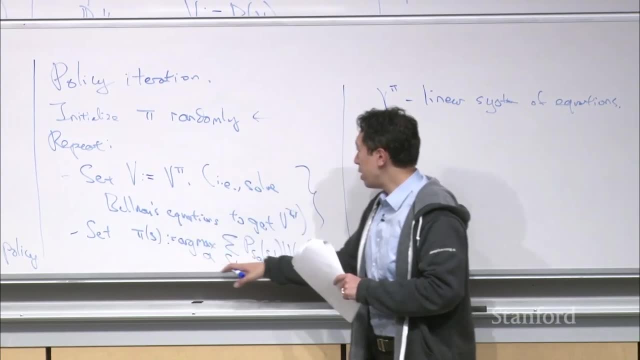 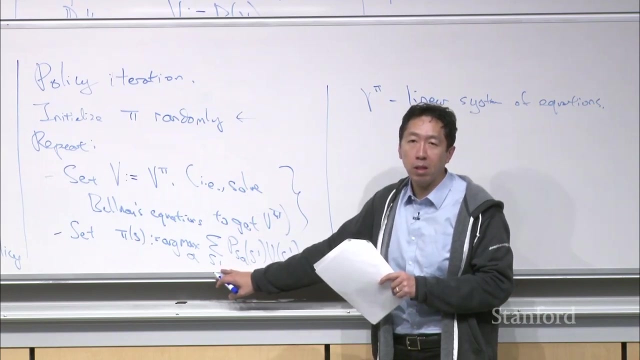 And then the second step of policy iteration is um, pretend that v is the optimal value function And uh, update, uh, update, pi of s, you know, using the um, uh, Bellman's equations for the optimal value function, right, 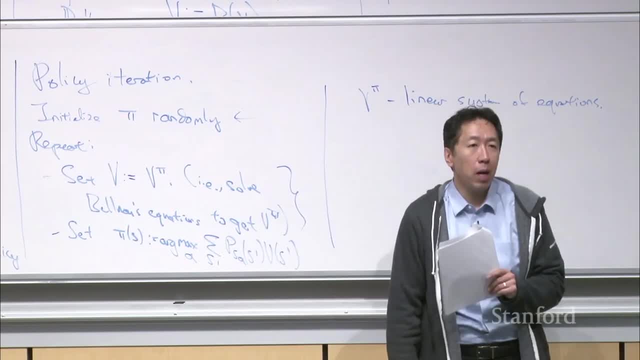 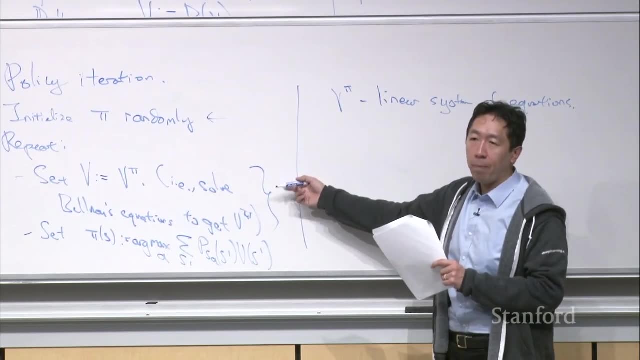 Or update it. um, as you saw right How you update pi of s And then you iterate, And then, given a new policy, you then solve that linear system of equations for your new policy, pi. So you get a new v, pi. 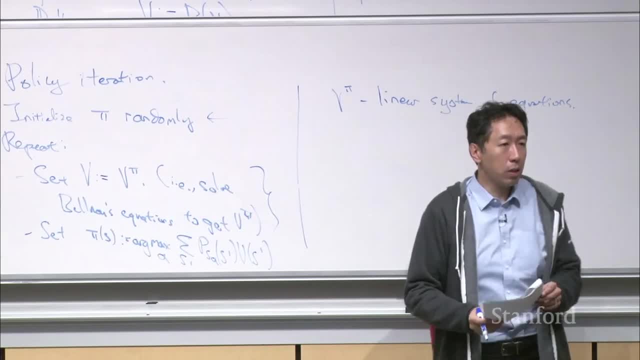 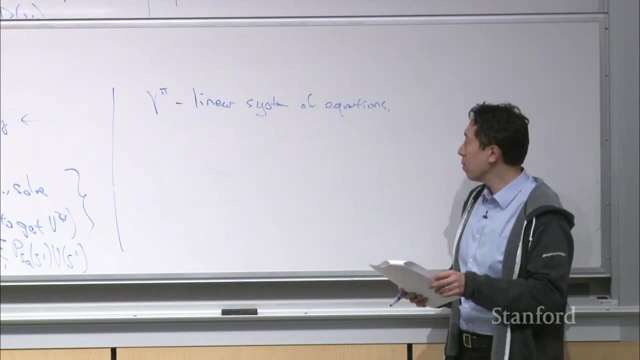 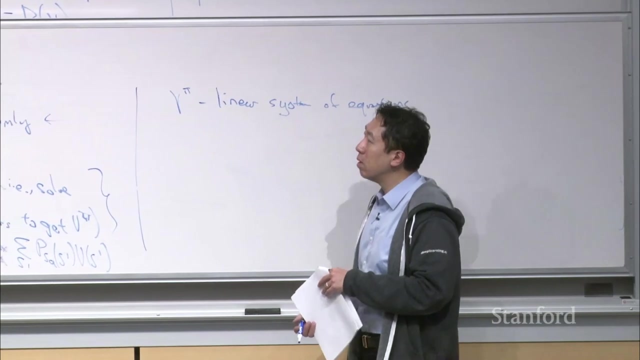 and then you keep on iterating these two steps um until it converges. Okay, Yeah, Yeah, Yep. Yes, that's right. So in in in value, uh, yeah, yeah, yeah, yeah. So in in value iteration. 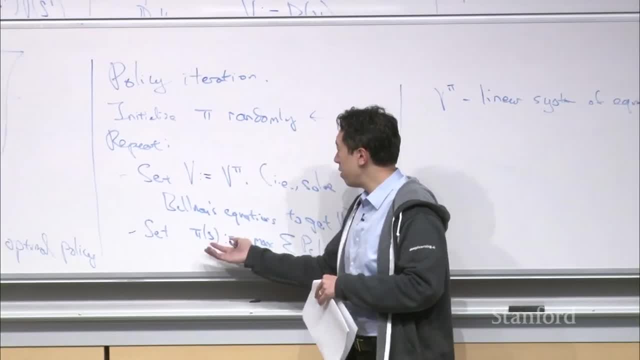 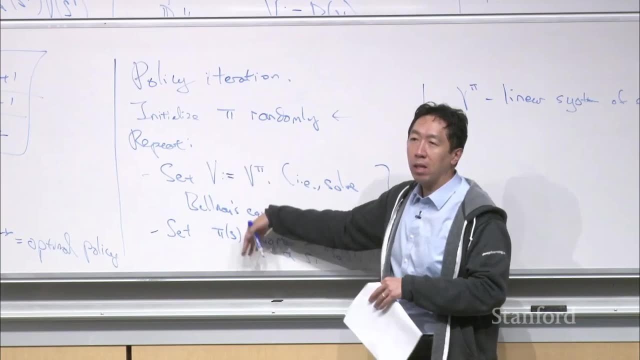 um, uh, actually in value iteration. you think of value iteration as waiting to the end to compute pi of s right, Solve for v stop first, then compute pi of s, Whereas in policy iteration, we're coming up with a new policy on every single iteration right. 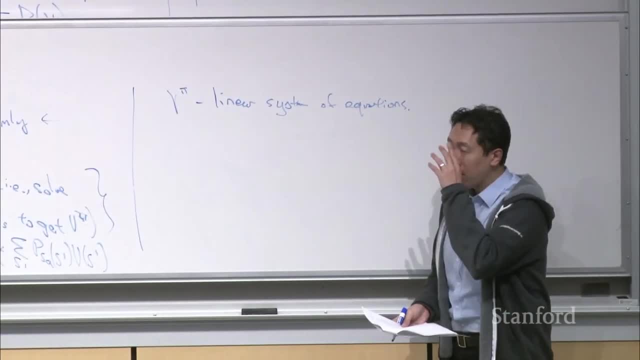 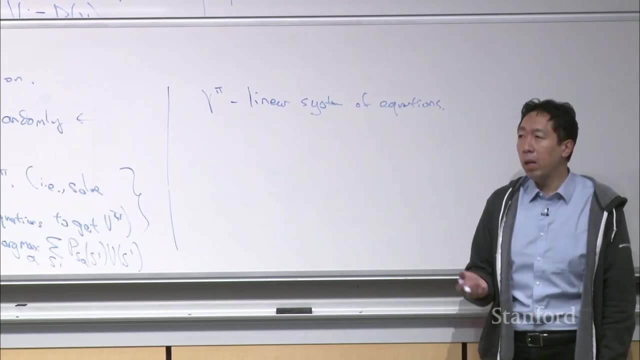 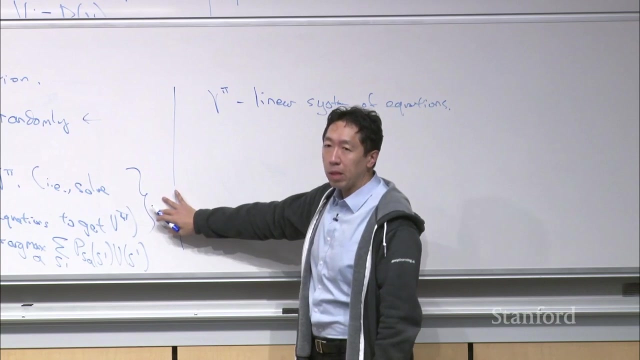 Okay, So um pros and cons of uh, poli- and. and it turns out that this algorithm will also converge to the optimal policy. Um pros and cons of policy iteration versus value iteration. Policy iteration requires solving this linear system of equations in order to 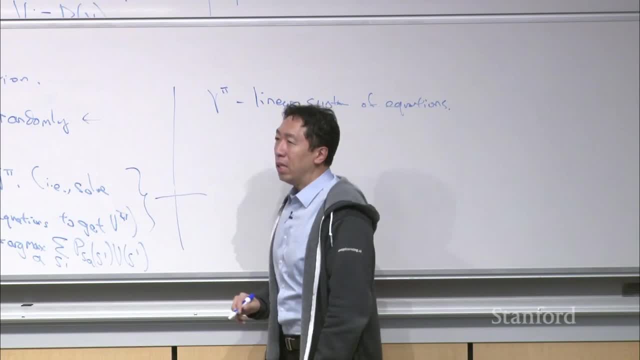 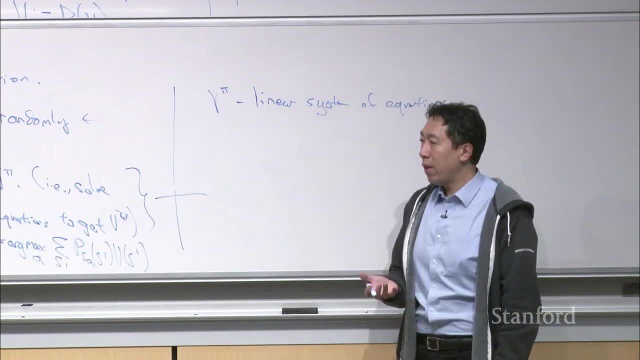 um get v pi. And so it turns out that if you have a relatively small state space, um like if you have 11 states, it's really easy to solve a linear system of equations- uh, you know, of 11 equations- in order to get v pi. 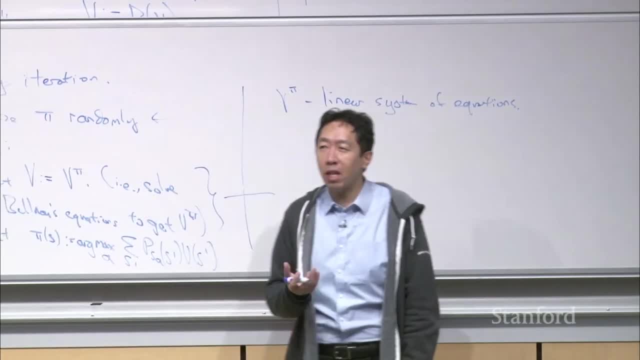 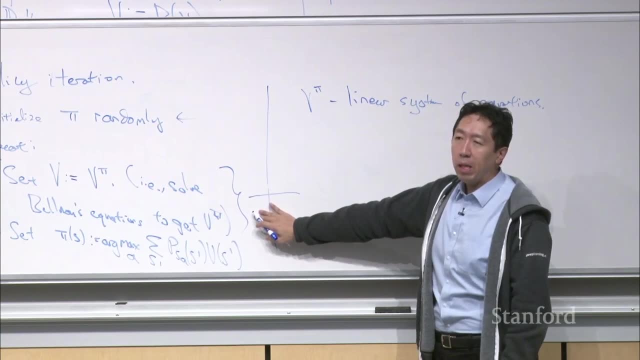 And so if you have a relatively small set of states, like 11 states or really anything you know, like a few hundred states, um, policy iteration would work quite quickly. Uh, but if you have a relatively large set of states, 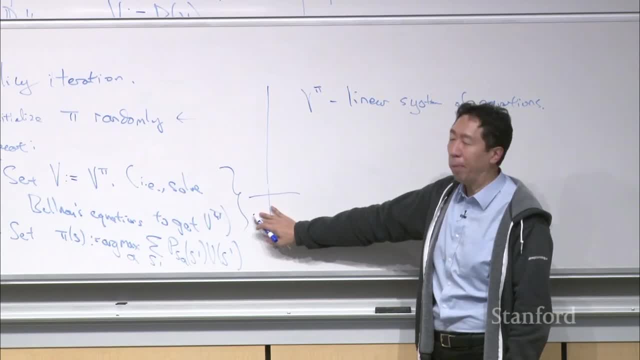 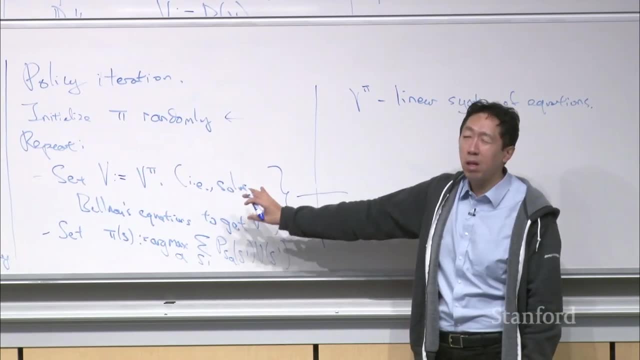 you know, like 10,000 states, or or or a million states. um then this step would be much slower, at least if we do it right by solving linear system of equations, and then I would favor value iteration over policy iteration. 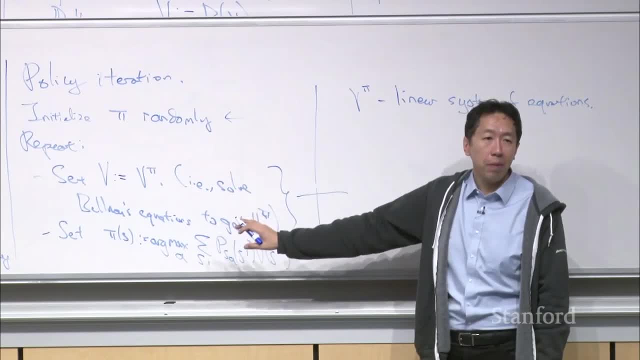 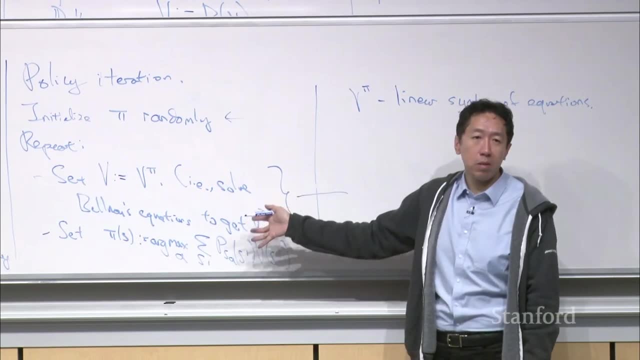 So for. so for larger problems, usually value iteration will um, uh, uh. usually I would use value iteration because solving this linear system of equations- you know is- is pretty expensive. if it was a is a million by is a million equations. 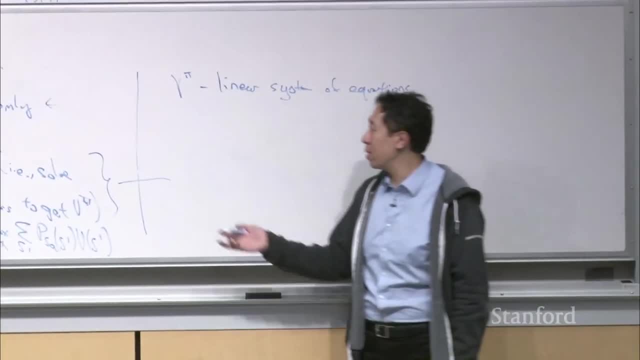 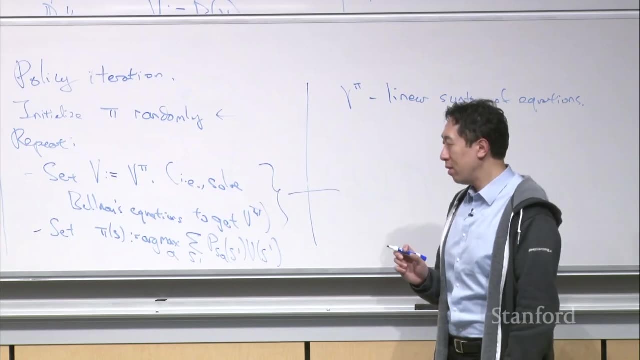 a million unknowns, that's quite expensive. But if 11 states and 11 unknowns, this is a very small system of equations, Um, and then one- one other pros and cons, one other, uh uh difference. that- that's maybe- maybe more academic than practical. 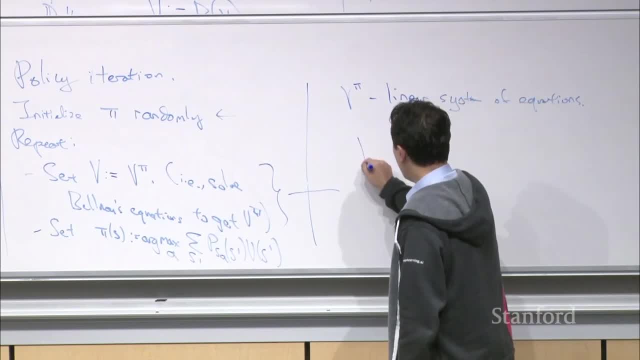 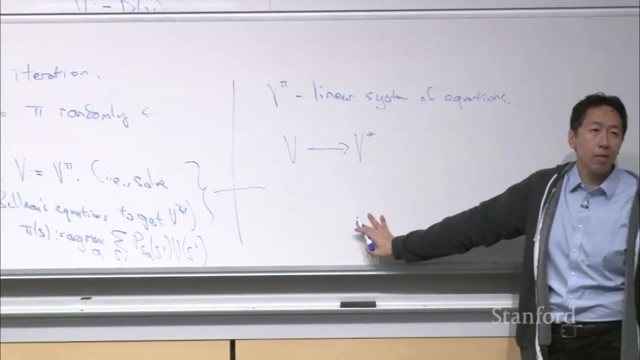 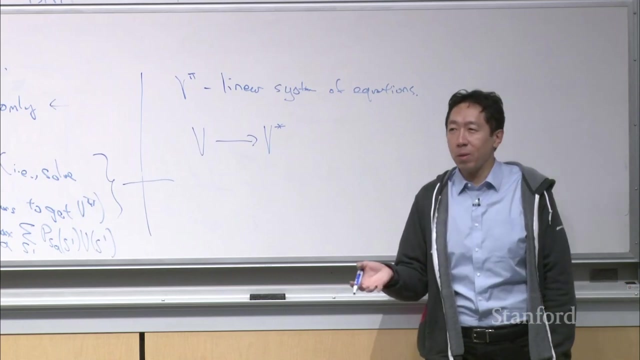 but it turns out that if you use value iteration, um v will converge toward v star, but it won't ever get to exactly v star right. So just as if you apply gradient descent for linear regression, um gradient descent gets closer and closer and closer to the global optimum. 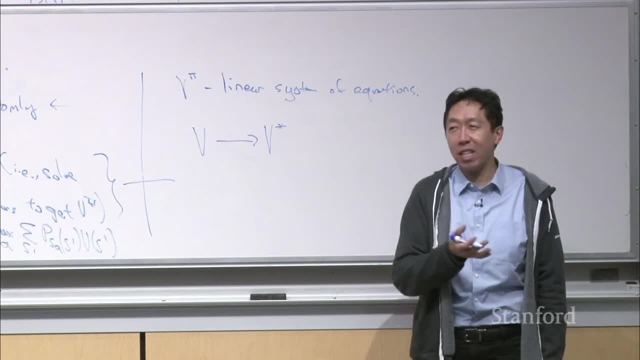 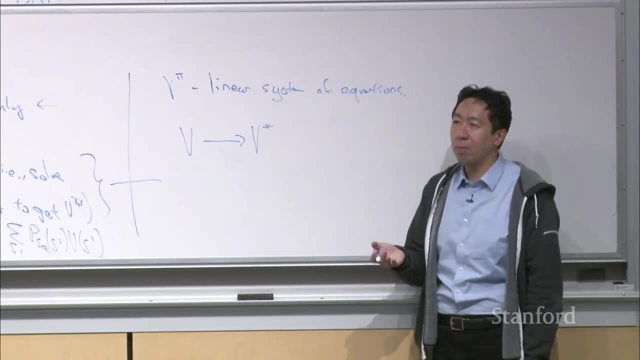 but it never, you know, gets exactly the global optimum. It just gets really really close, really really fast. Actually, gradient descent actually turns out asymptotically, converges geometrically quickly or exponentially quickly, right, But it never quite gets, you know. 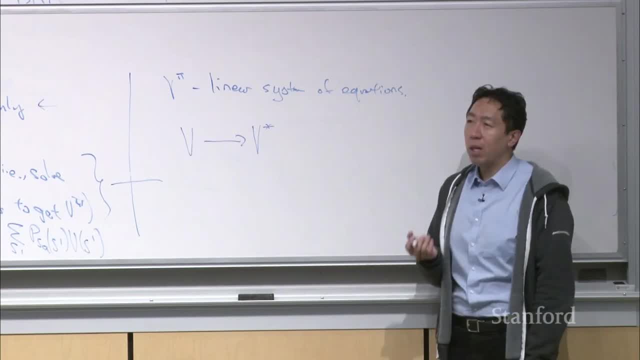 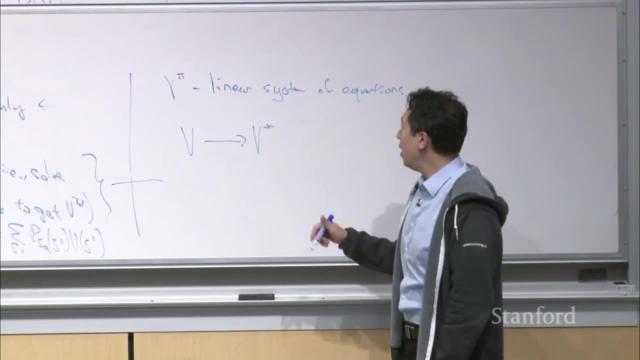 definitively to the optimal- to the one optimal value, Whereas you- you saw, using normal equations it just jumps straight to the optimal value and there's no you know converging slowly, And so value iteration converges toward v star. 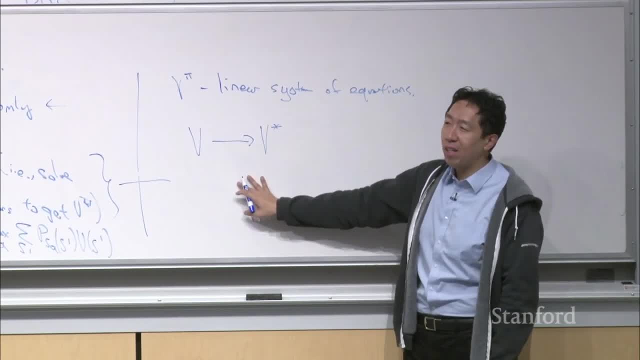 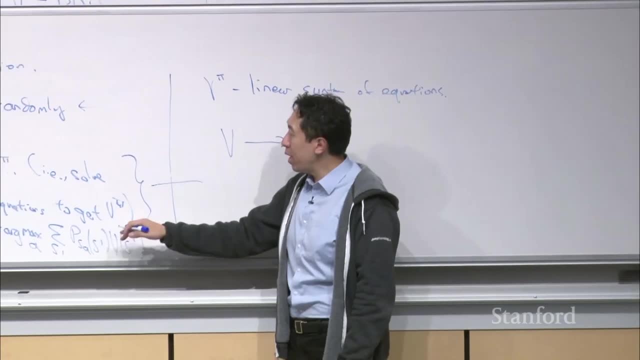 but it doesn't ever end up at exactly the value v star. Uh, this difference maybe a bit academic, because in practice it doesn't matter, right, Um? but in policy, iteration, um, if you iterate this algorithm, then after a finite number of iterations. 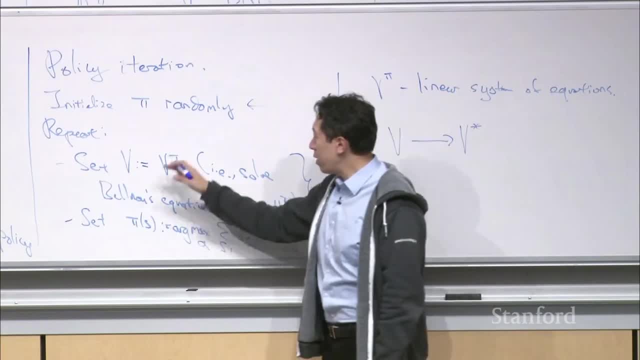 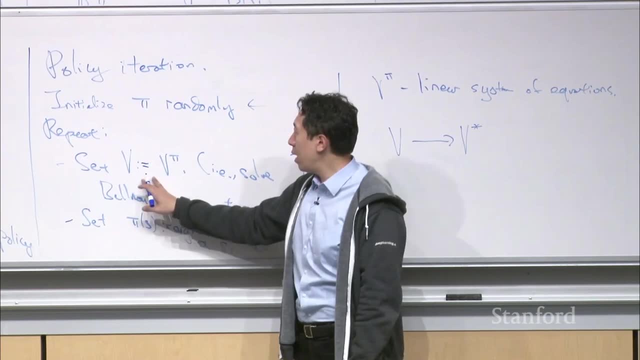 uh, this algorithm will stop changing, meaning that after certain number of iterations pi of s will just not change anymore, right? So you find pi of s, update the value function and then, after another iteration, when you take these arg maxes. 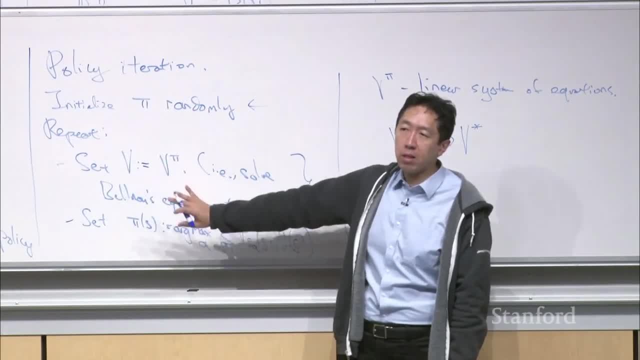 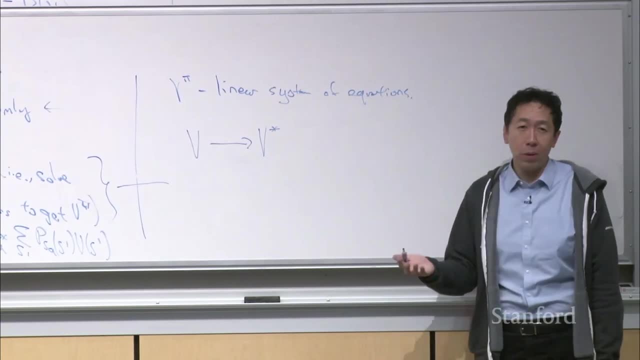 you end up with exactly the same policy, And so this just solves for the optimal value and the optimal policy, And it just, you know, uh, it doesn't converge-. it doesn't just converge toward the optimal value, it just get the optimal value when it. 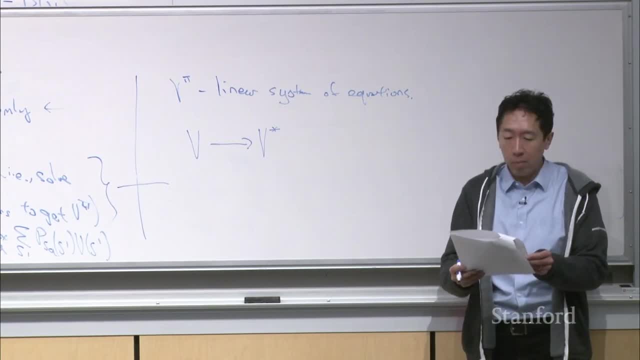 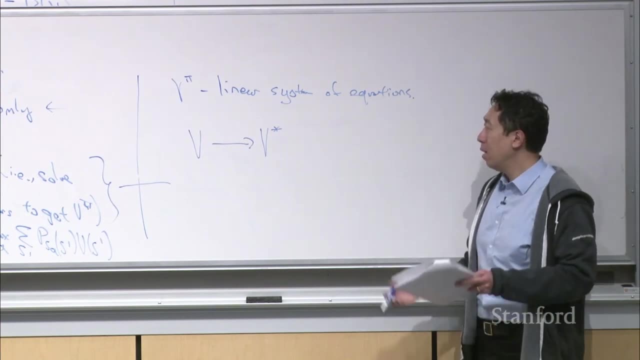 when it converges, okay, Um. so I think in practice I actually see value iteration used much more. uh, because um solving the Hello Stvre equations gets expensive, you know, if you have a larger state space, but um value iteration, uh. 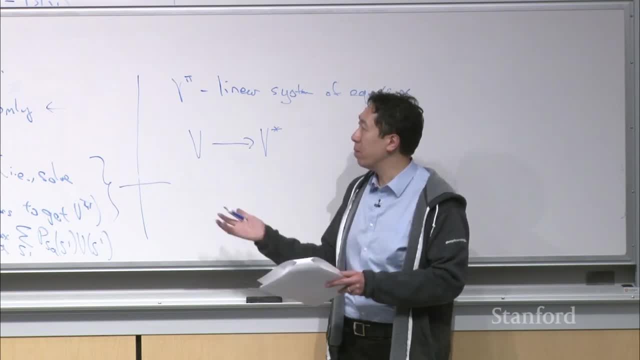 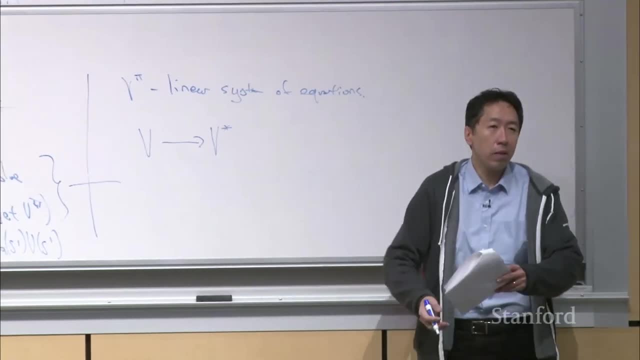 like in the same way. Uh, but that's a differentê, excuse me, po- see, I see valuation used much more. But if you have a small problem, you know, I think you could also use policy iteration, which might converge a little bit faster if. 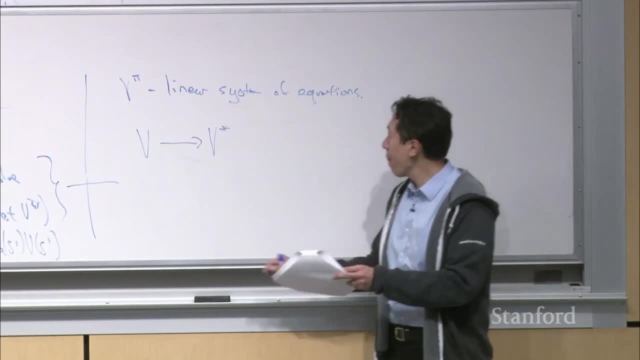 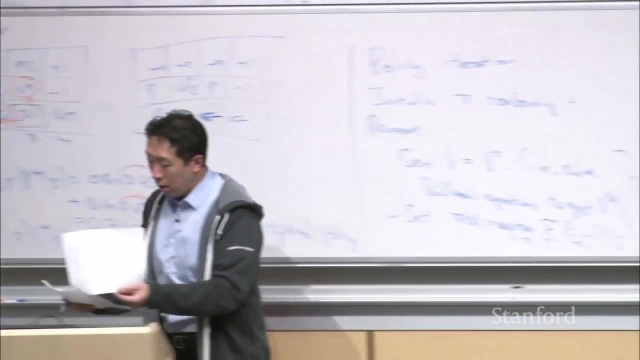 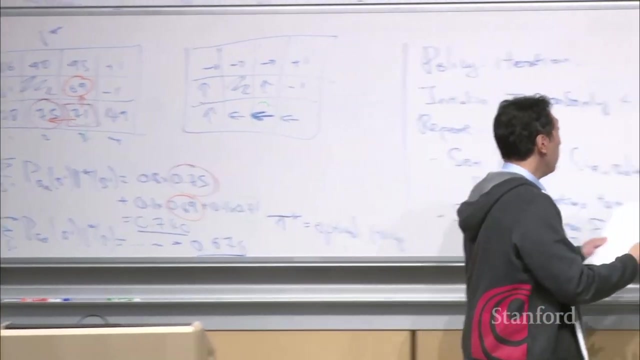 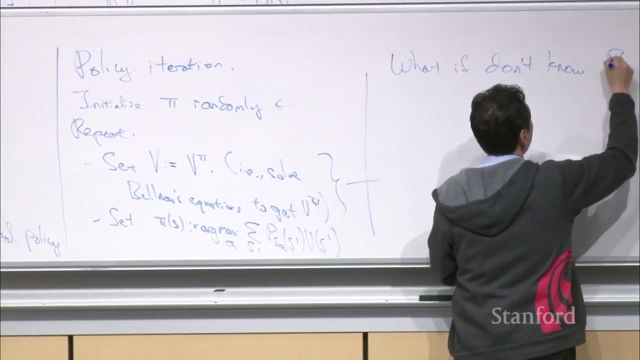 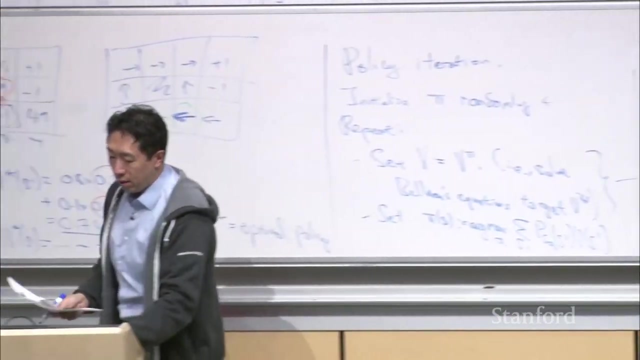 if you have a small problem, okay, All right. good, So the last thing is, um, kind of putting it together, right, And what if you don't know, right? Um, so it turns out that, uh, when you apply this to a practical problem, 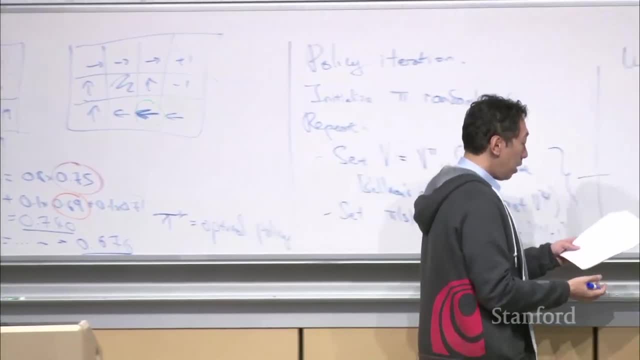 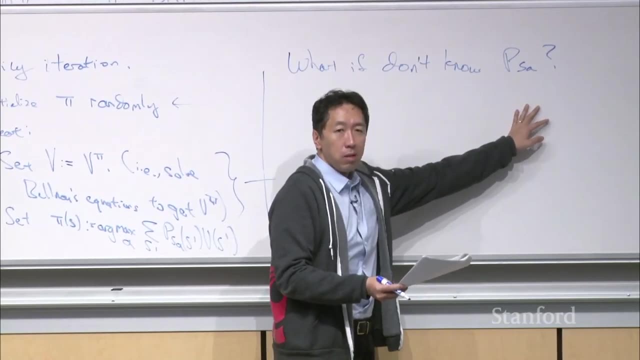 you know in, in, in, in in robotics, right? Um, one common scenario you run into is: uh, if you do not know what is P of S A, If you don't know the state transition probabilities, right. 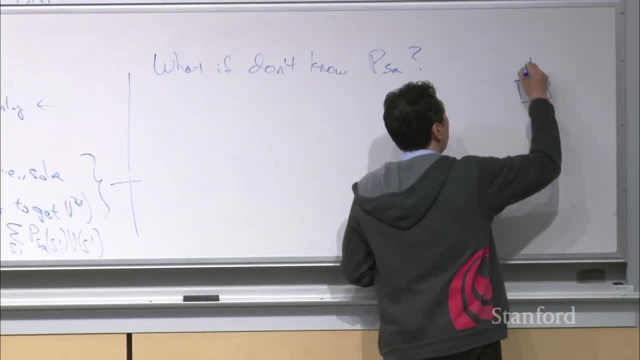 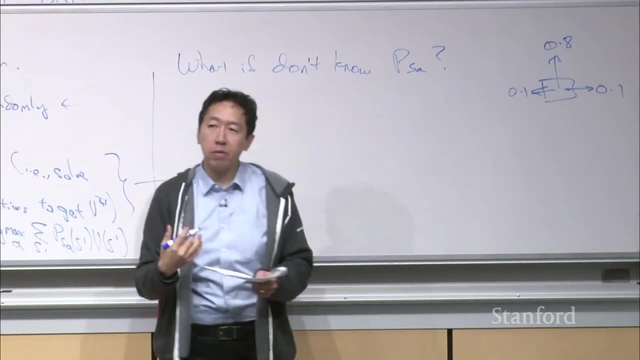 So when we built the MDP, we said, well, let's say the robots, if you go north, you know, has a 0.8 chance of going north and a 0.1 chance of veering off to the left or right. 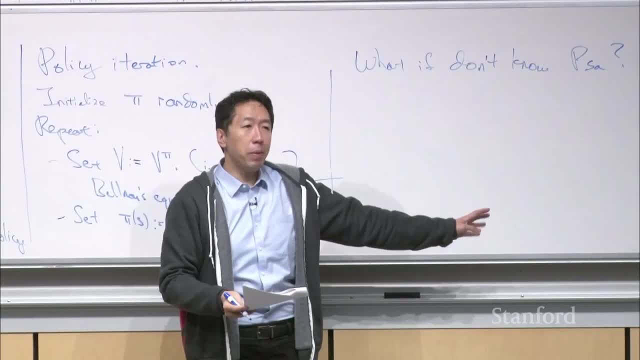 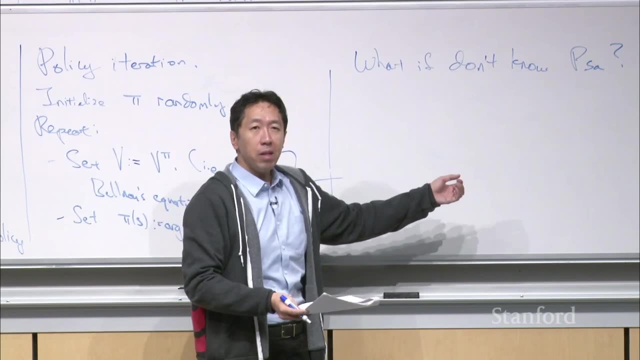 So if you actually- again, this is a very simplified robot- But, uh, if you build a, uh, actual robot, or build a, you know, helicopter or whatever, play, play, play chess against an opponent um the state transition probabilities are often not known in advance. 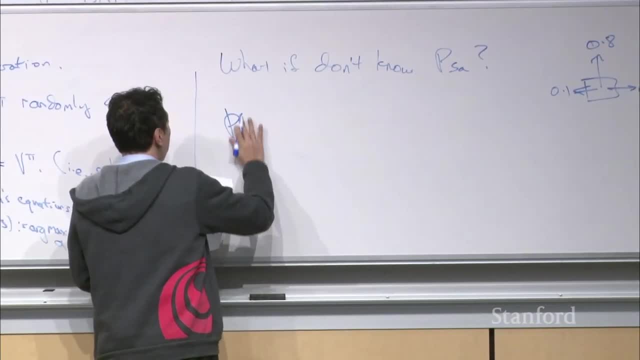 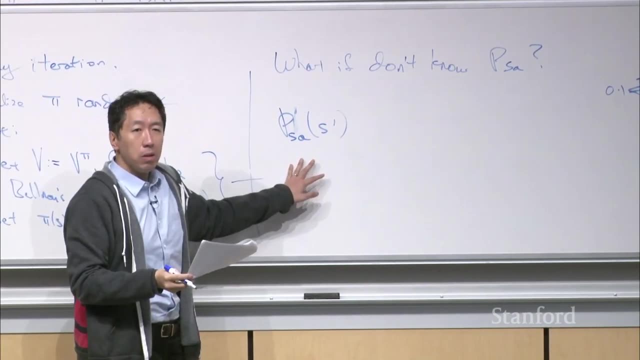 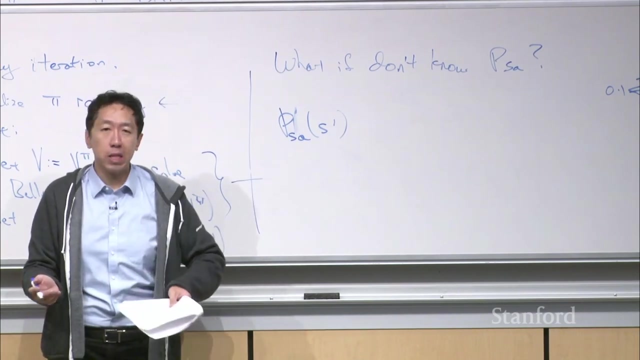 And so, um, in many MDP implementations, you need to estimate this from data, And so, uh, the workflow of many reinforcement learning projects will be that you will, um, have some policy and have the robot run around. You know, just have a robot run around the maze and count up. 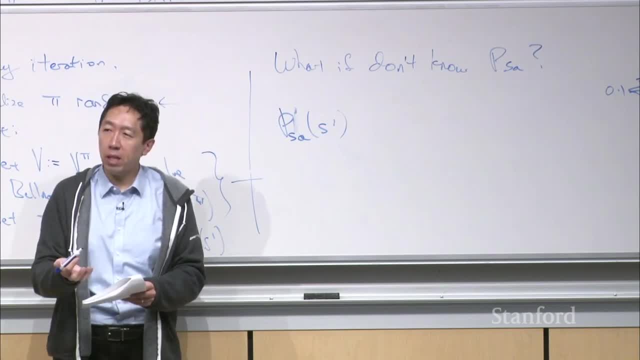 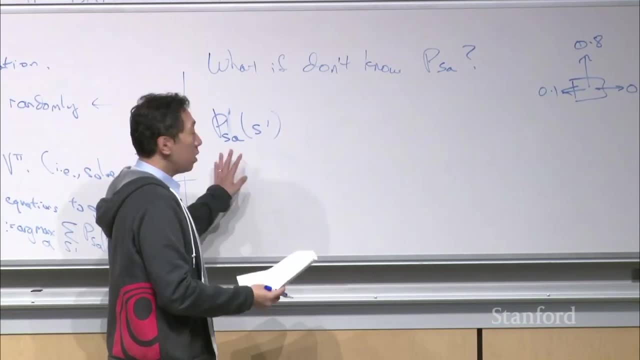 of all the times you had it take the action north, how often did it actually go north and how often did it veer off to the left or right, right? And so you use those statistics to estimate the state transition probabilities. So let me just write this out. 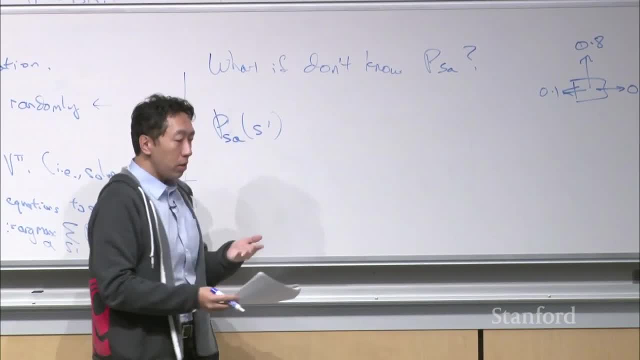 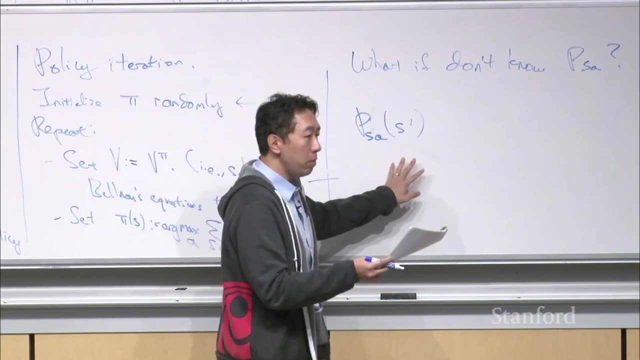 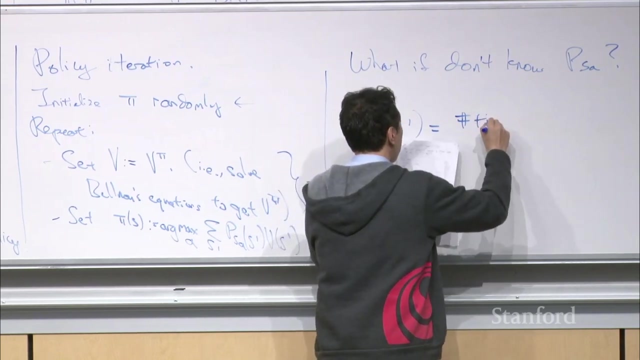 So you estimate um so, after you know taking maybe a random policy, or take some policy, execute some policy in the MDP for a while, and then you would estimate this from data, And so the obvious formula would be: estimate P of S A S prime to be number of times. 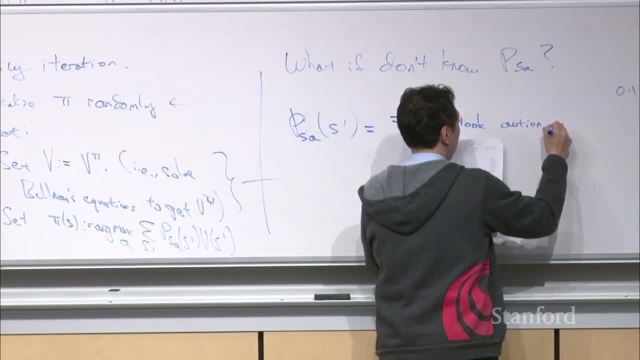 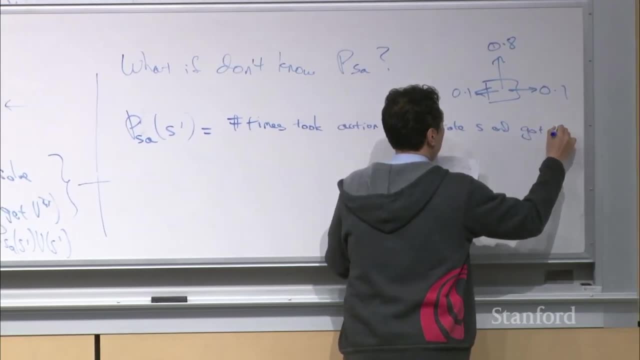 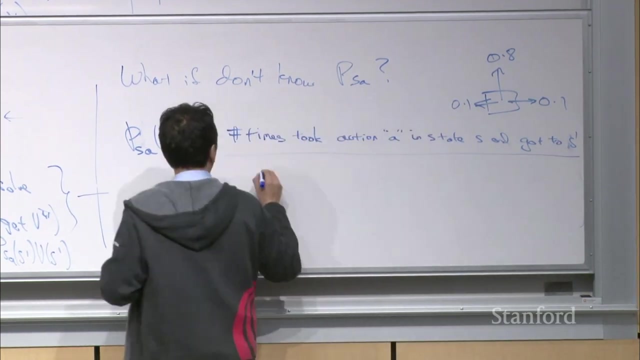 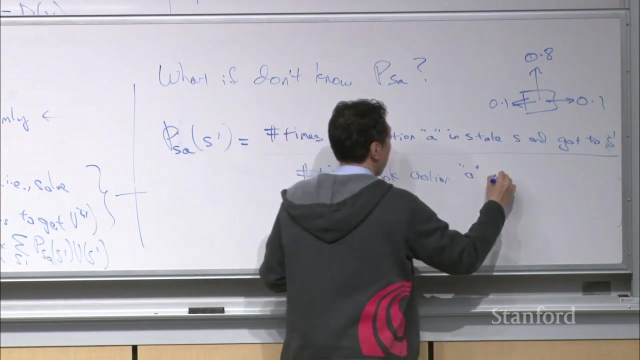 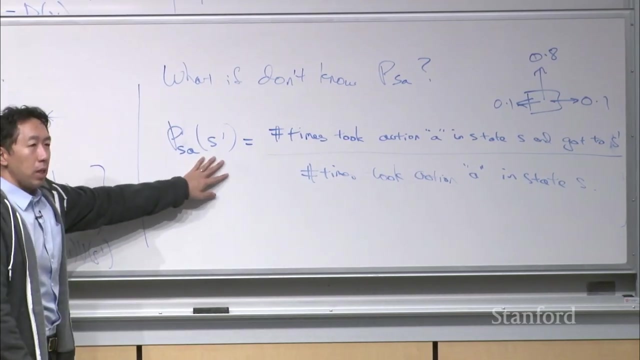 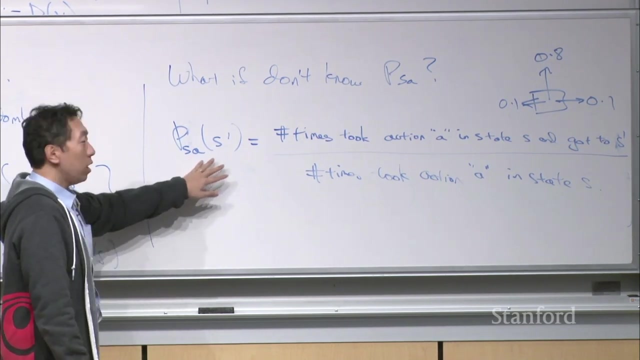 um took action A in state S and got to S prime and divide that by the number of times you took action A in state S, right, So P of S A S prime estimate- this is actually a maximum likelihood estimate. Uh, when you look at the number of times you took action A in state S and of that, what's the? 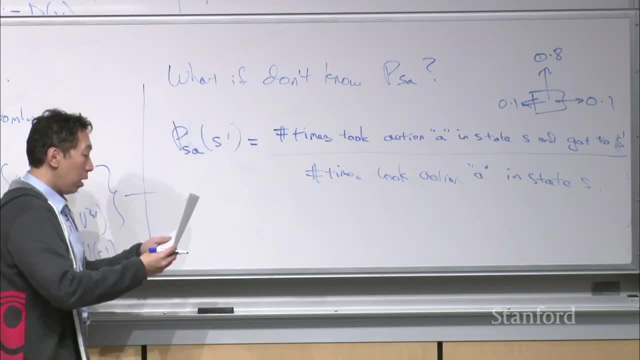 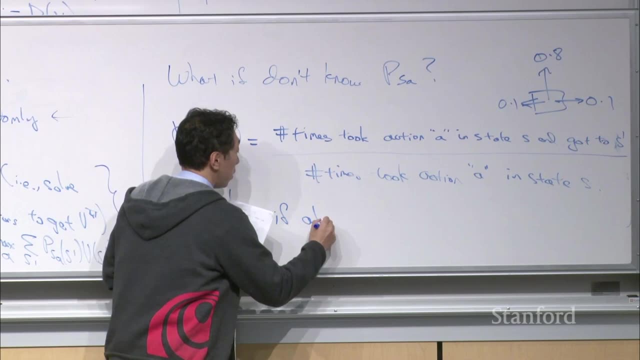 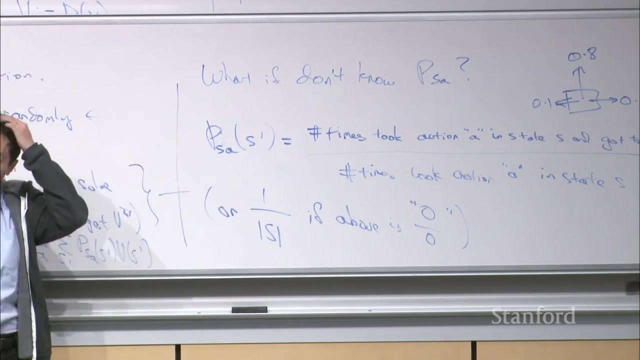 fraction of times you got to the state S prime right Um or 1 over S at the above is 0 over 0, right And a common you know heuristic is: uh, if you've never taken this action in this state before. 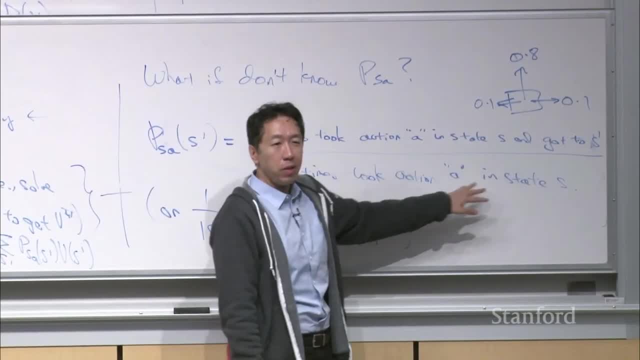 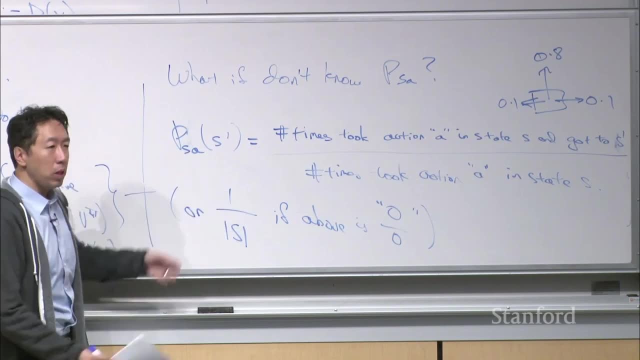 if you- if the number of times you try action A in state S is 0, so you've never tried this action in this state, so you have no idea what it's gonna do, then just assume that um the state transition probability is 1 over 11, right. 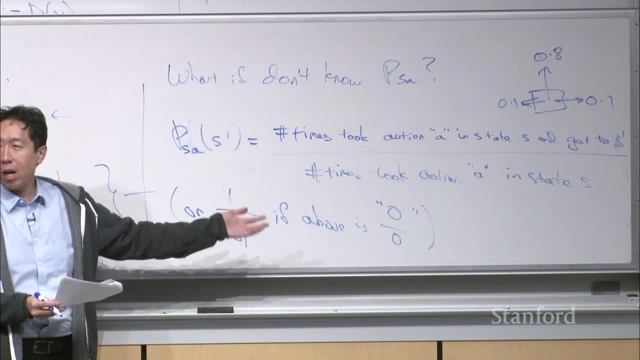 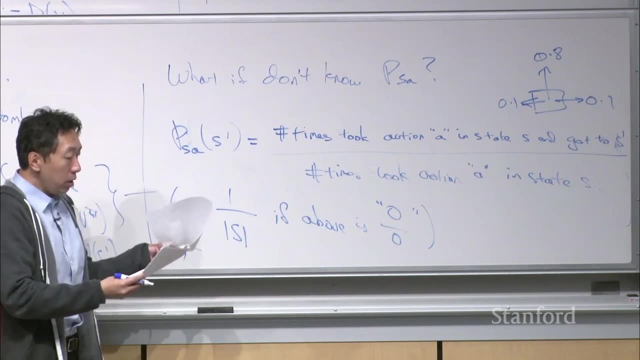 That you know randomly takes you to other states. So this would be ran- common heuristics that people use when implementing reinforcement learning algorithms. okay, Um and uh. it turns out that, um, you can use Laplace smoothing for this if you wish. 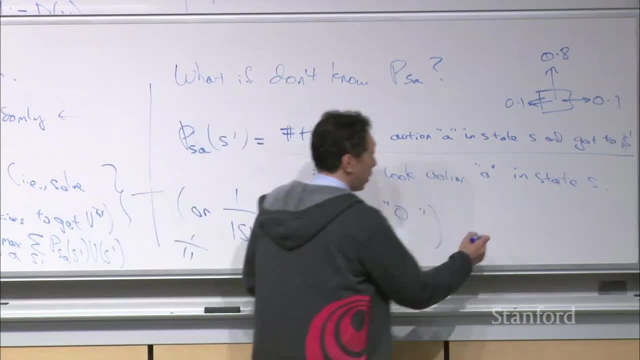 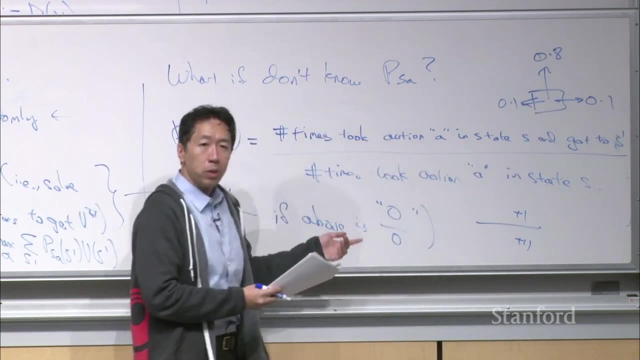 but you don't have to because, uh, so you're at Laplace smoothing, right? So it'd be, um, uh, you know, add 1 to the numerator and add 11 to the denominator would be if you were to use Laplace smoothing. 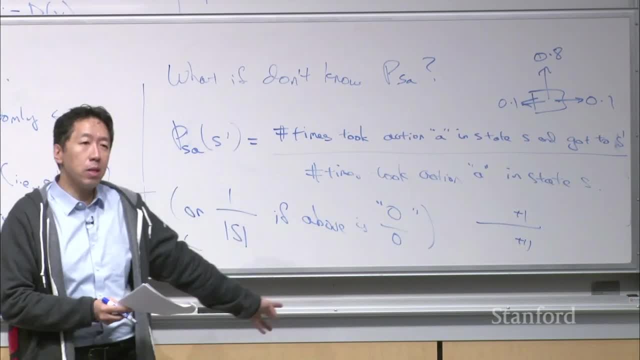 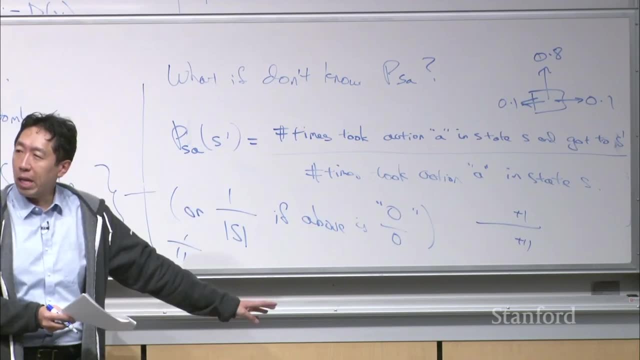 um, which avoids the problems of 0 over 0s as well. But it turns out that, unlike the Naive Bayes algorithm, um, uh, these solvers, the MDPs, are not that sensitive to 0 values. So if- if one of your estimates of probability is 0,. 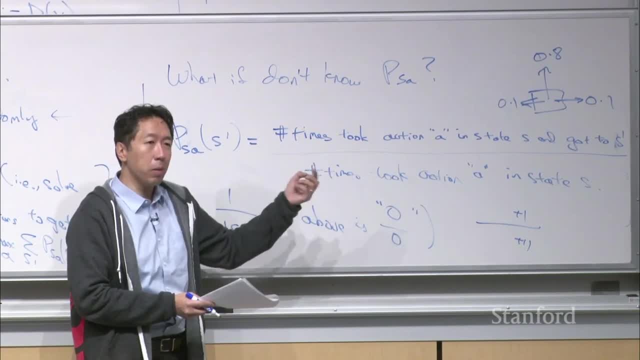 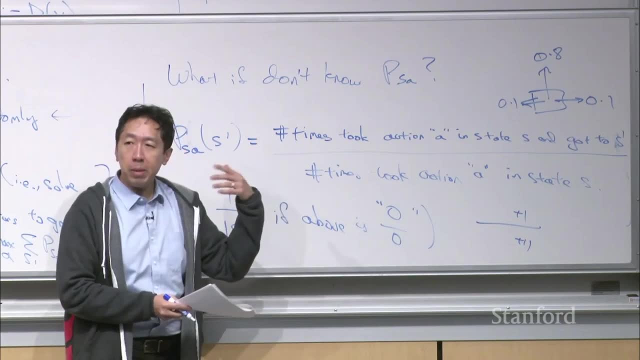 um, you know, unlike Naive Bayes, where having a 0 probability was very problematic for, uh, the classifications made by Naive Bayes, it turns out that um MDP solvers, including valuation policy iteration, they do not give sort of nonsensical slash, horrible results. 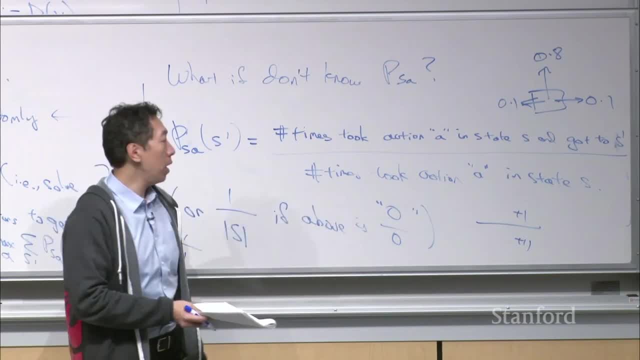 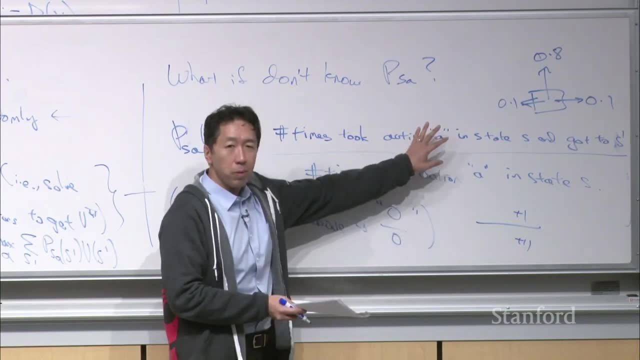 just because of the few probabilities that are exactly 0.. And so, um, in practice, you know you can use Laplace smoothing if you wish, uh, but because, um, the reinforcement learning algorithms don't- don't perform that badly. 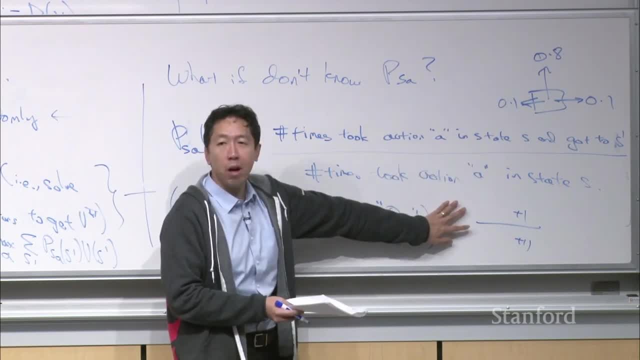 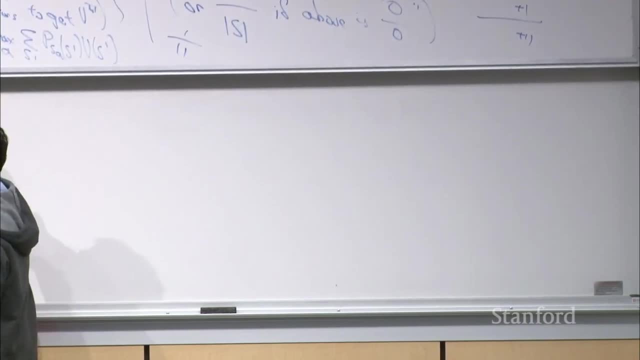 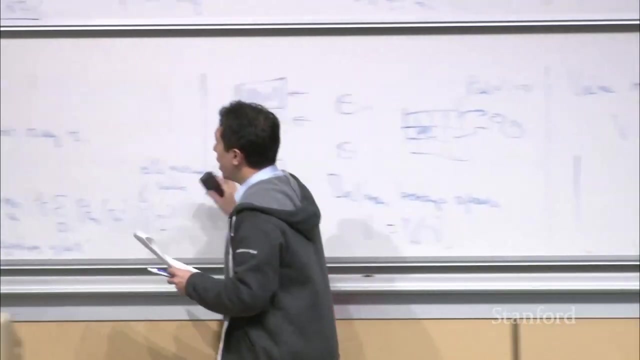 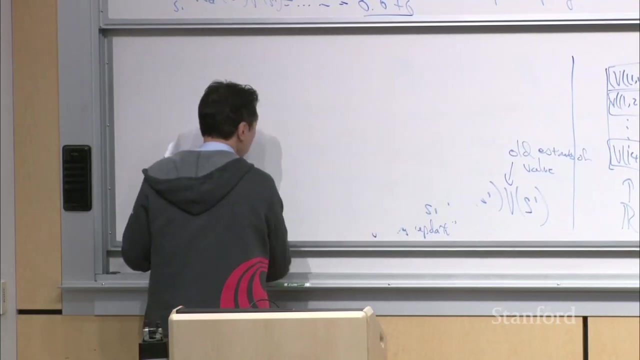 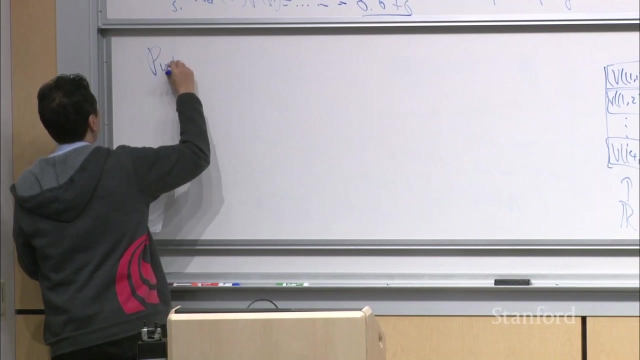 if these estimates are often more than or equal to 0,. in practice, Laplace smoothing is not commonly used and what I just wrote is- is more common. Okay, So, um, to put it together, all right, um. 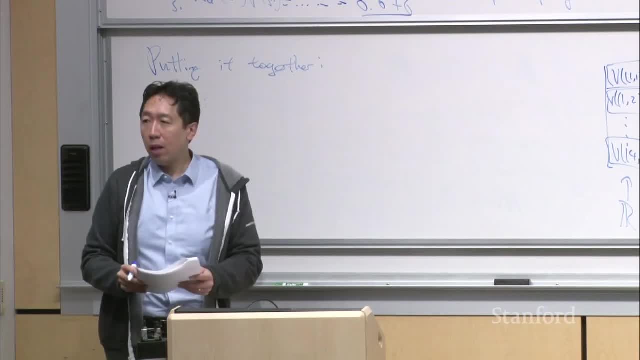 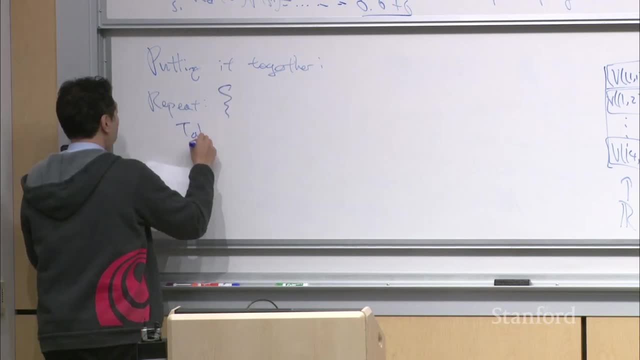 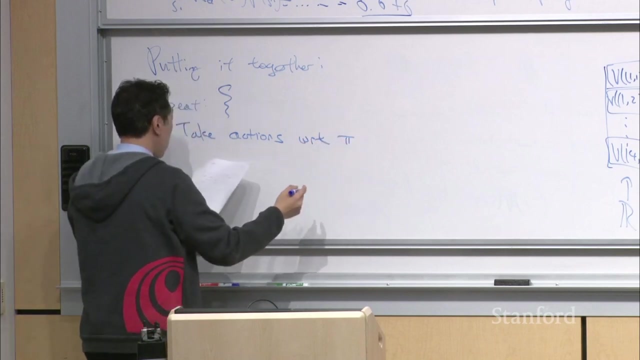 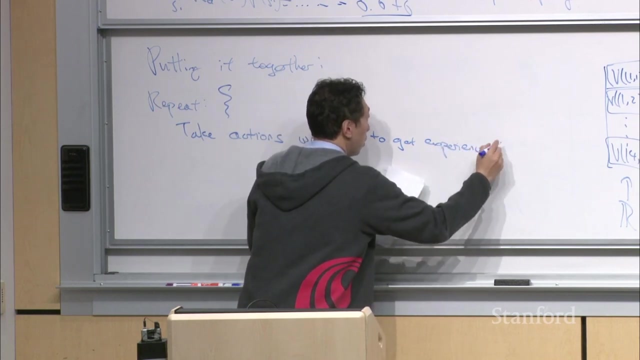 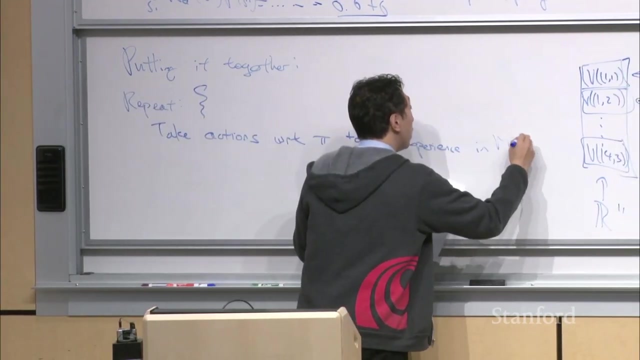 if I give you a robot and ask you to implement a um MDP solver to find a good policy for this robot, what you would do is the following: Take actions with respect to some policy pi So you get experience in the MDP right. 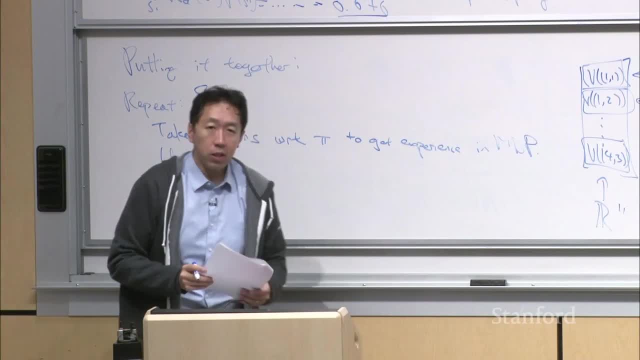 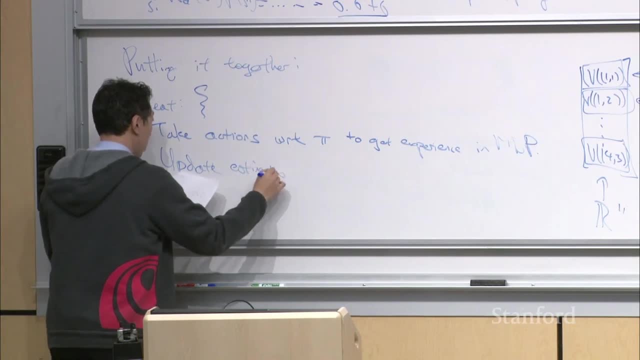 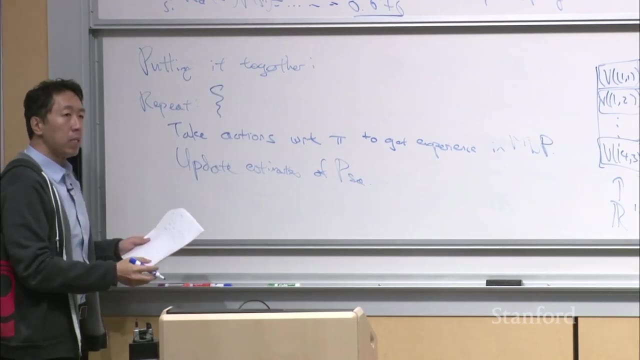 Um, so go ahead and let your robot loose and have it execute some policy for a while And then update estimates of PFSA, Right, Um, based on the observations of where the robot goes when it takes different states. uh, update- get updated estimates of PFSA. 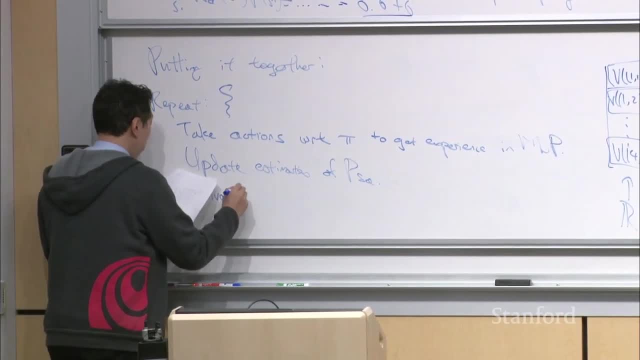 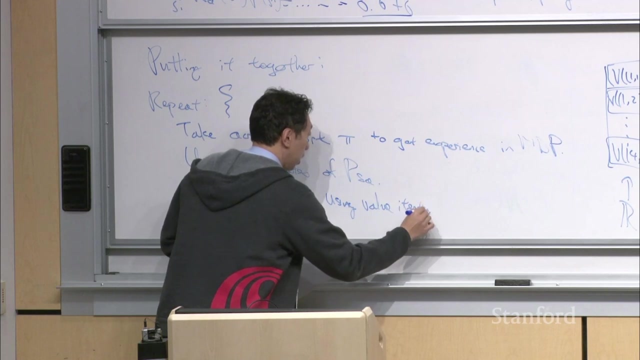 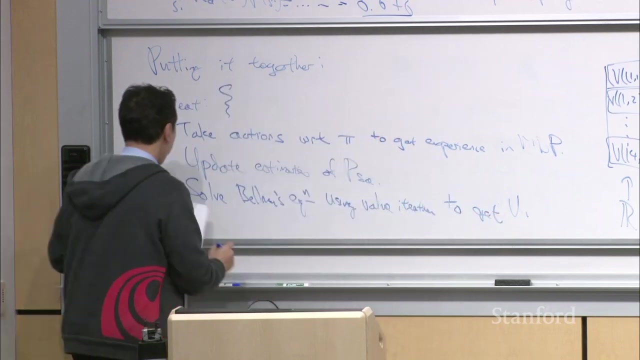 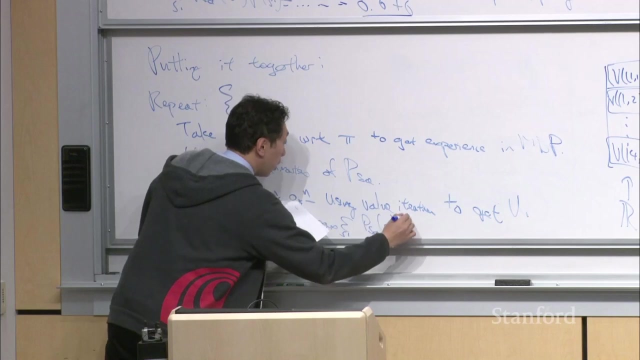 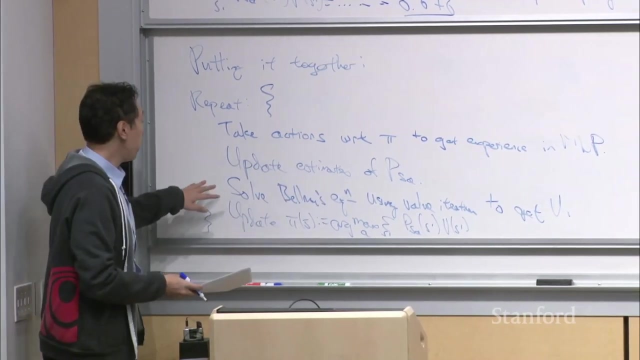 Um solve um Bellman's equation using value iteration To get V And then uh update. So this is the um value iteration way of putting it together. Uh, if you want to plug in policy iteration instead in this step, that's also okay. 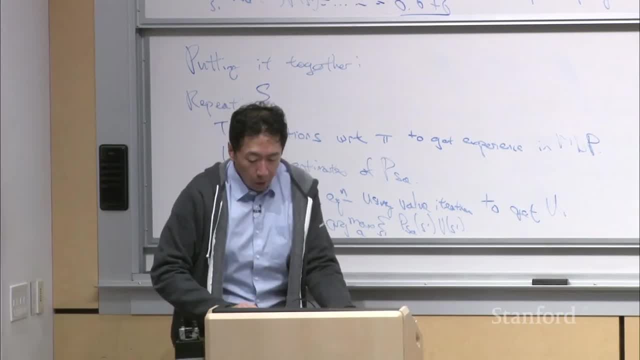 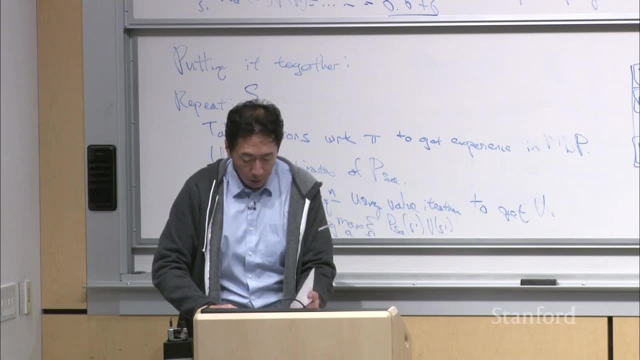 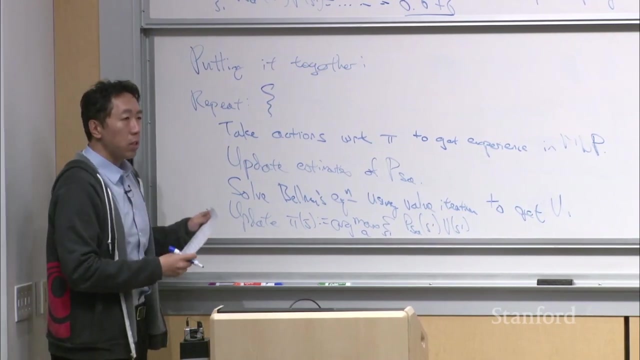 Um, But so if you actually get a robot, um, uh, you know, um, yeah, right, Right, If you actually get a robot, uh, where you do not know in advance the state transition probabilities, then this is what you would do in order to. 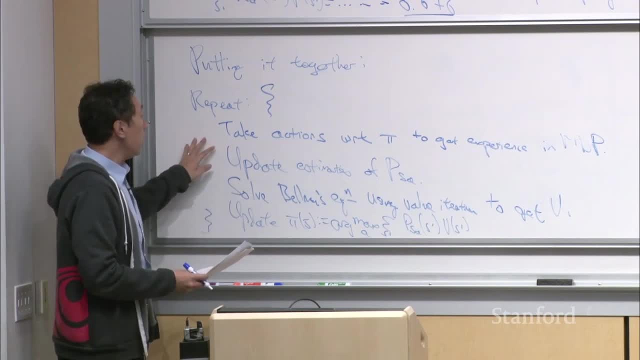 um, iterate a few times, I guess right. Repeatedly, uh, find a-, find a-, find a policy, given your current estimates of state transition probabilities. Get some experience, update your estimates, find new policy and kind of repeat. 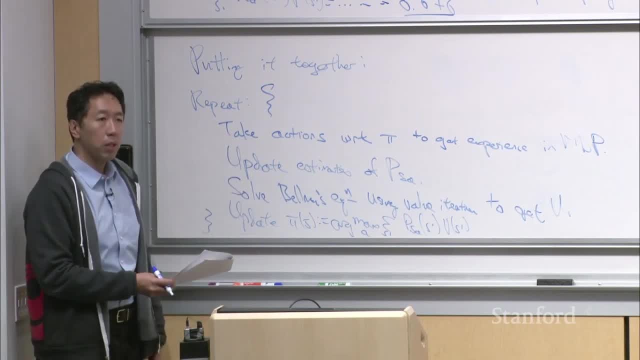 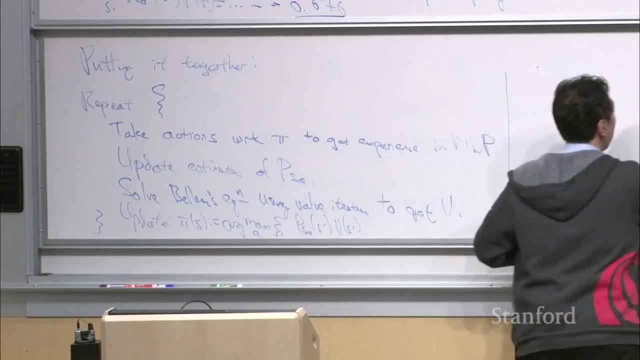 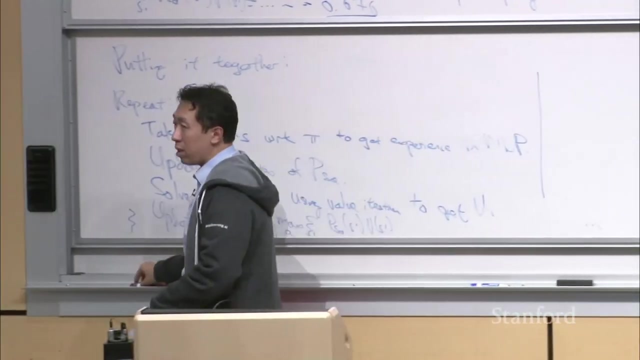 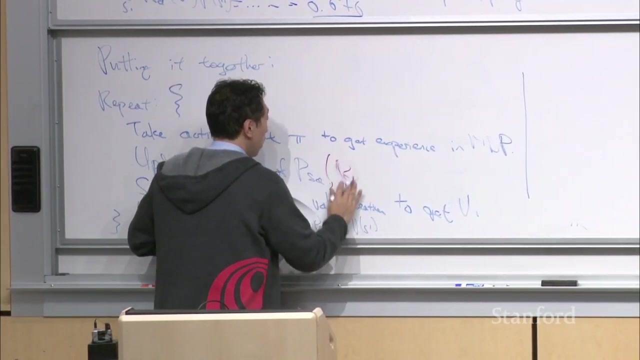 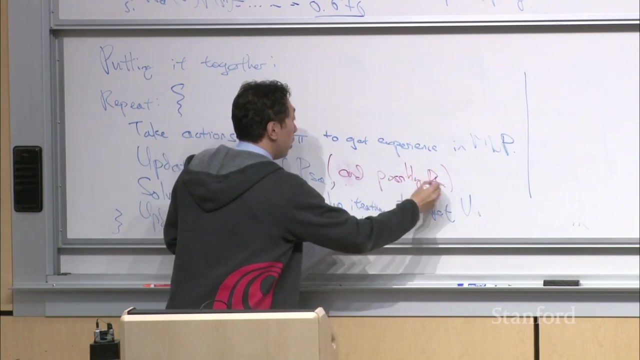 this process until, hopefully, it converges to good policy. okay, Now just to add more color or more richness to this um. we usually think of, we usually think of the uh reward function as being given right as part of the problem specification. 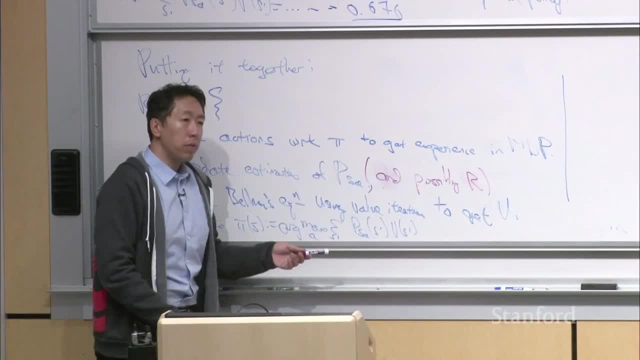 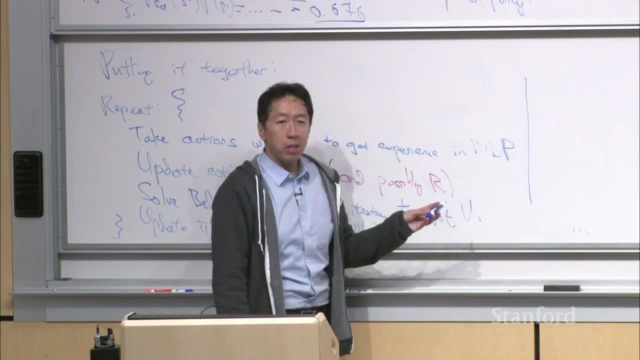 But sometimes you see that, um, uh, the reward function may be unknown. And so, for example, if you're building a stock trading application, um, and the reward is the returns on a certain day, it may not be a function of the state. 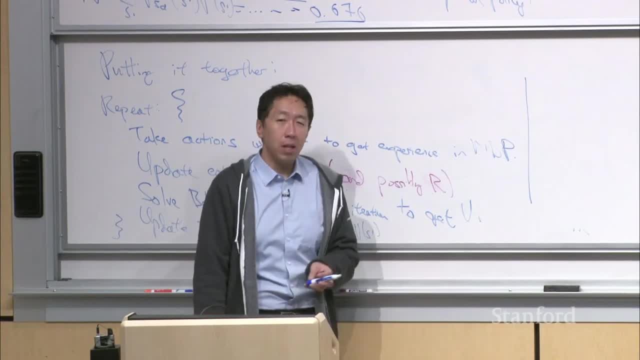 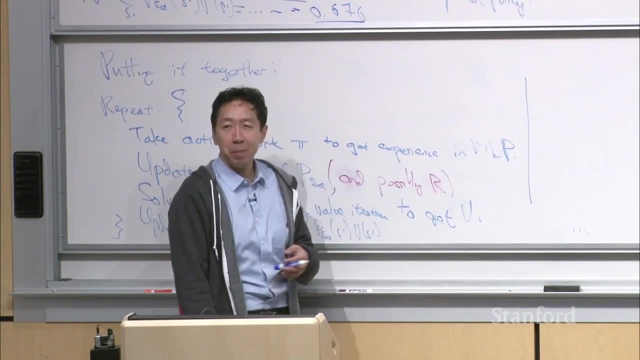 it may be a little bit random, Um, or if your robot is, you know, running around but depending on where it goes, it may hit different bumps in the road right, And you want to give it a penalty every time it hits a bump. 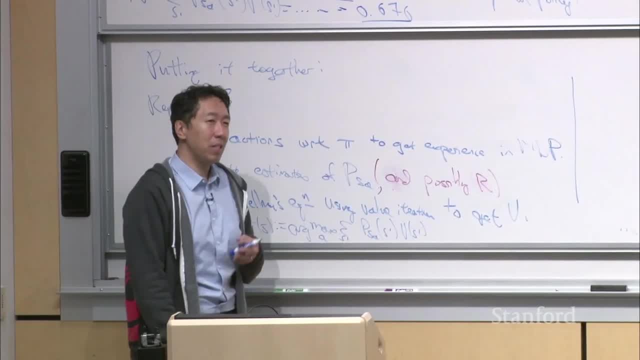 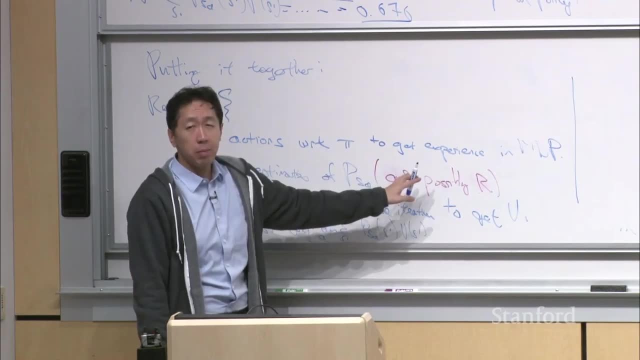 We're gonna build a self-driving car right, And every time it hits a bump- uh, hits a pothole- you give it a negative reward. Then sometimes the rewards are a random function of the environment, And so sometimes you can also estimate the expected value of a reward. 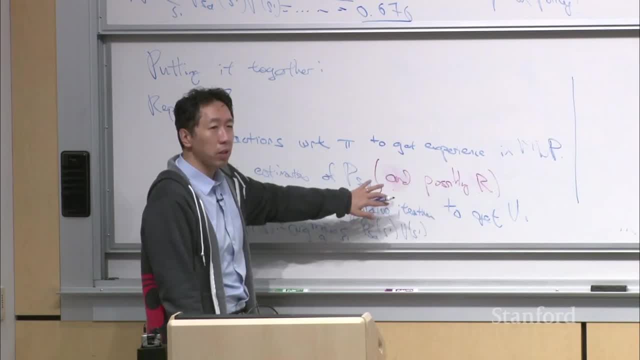 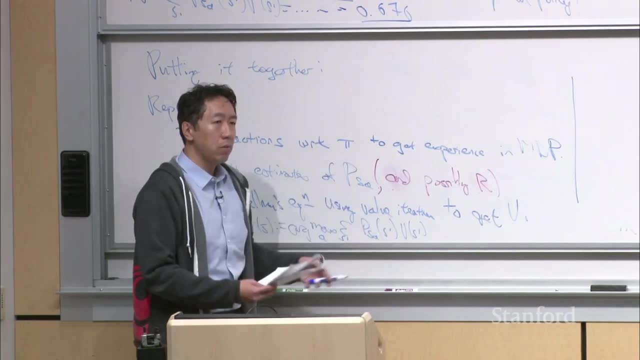 But- but uh in- in- in some applications, if the reward is a random function of the state, then this process allows you to also um estimate the expected value of the reward from every state, And then running this will help you to converge okay. 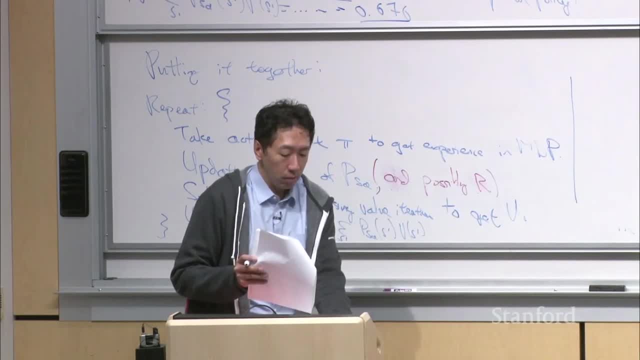 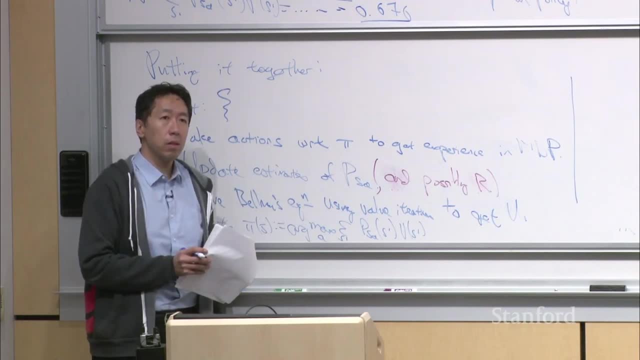 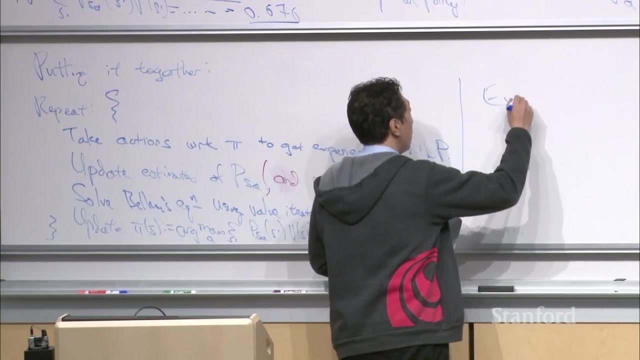 Um, yeah, Yeah, Yep, Cool, Yep Cool, Great question. So let me- let me talk about exploration, right? So it turns out that, um this one- so it turns out this algorithm will work okay for some problems. 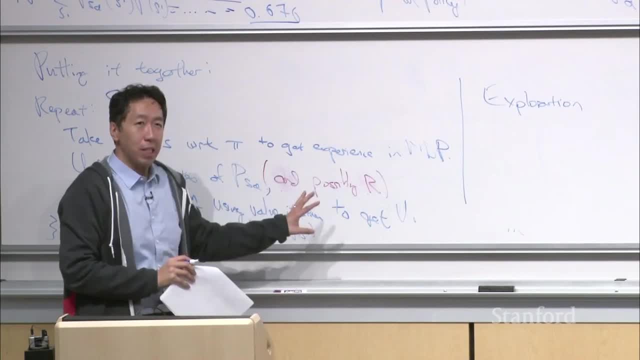 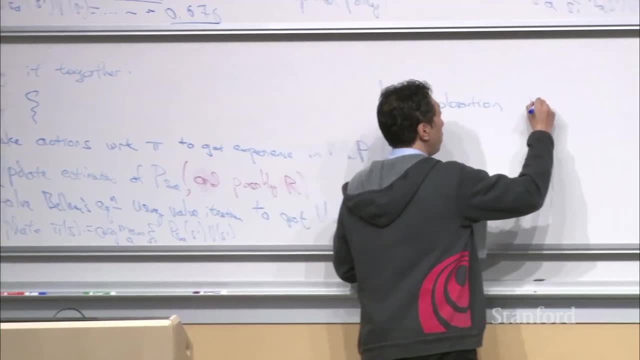 but th- th- there's one other uh again, to add richness to this, there's one other um issue that this is not solving, which is the exploration problem, And in- in reinforcement learning, sometimes you hear the term exploration versus exploitation. right, 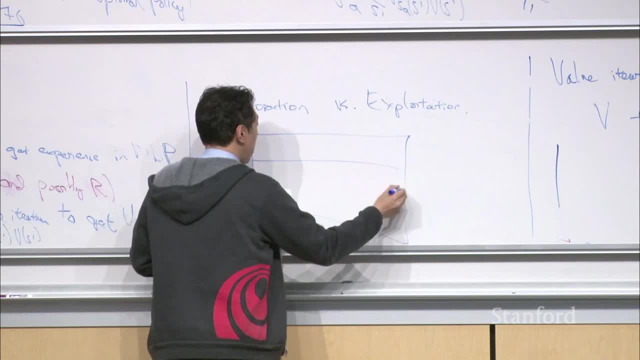 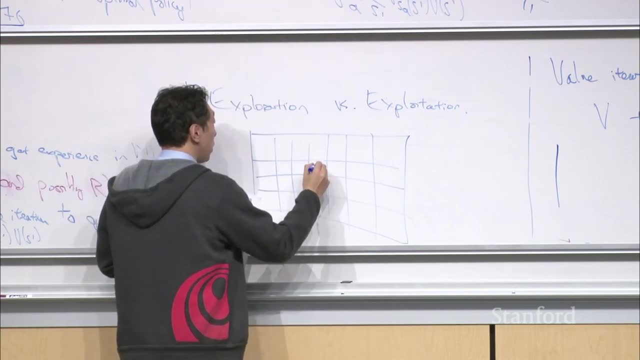 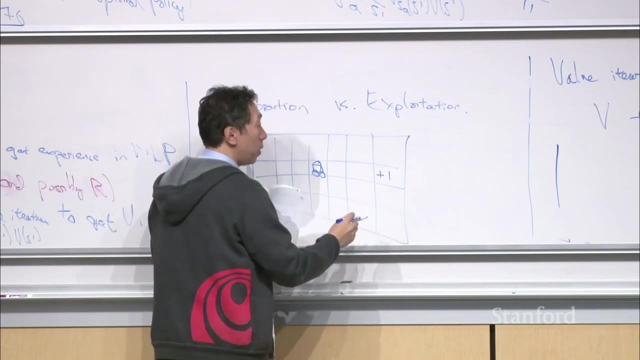 Which is um. let me use a different MDP example: right, Which is um. if your robot, you know, starts off here, and if there is a um plus 1 reward here, right, And maybe a plus 10 reward here. 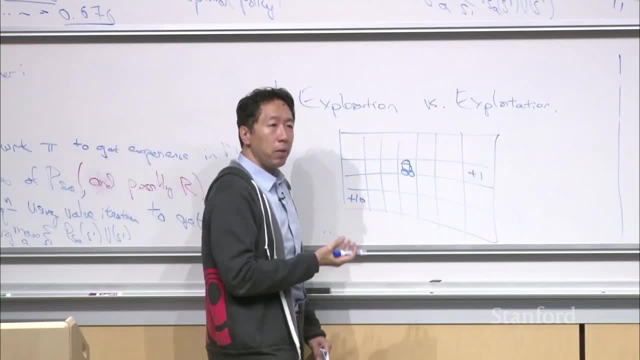 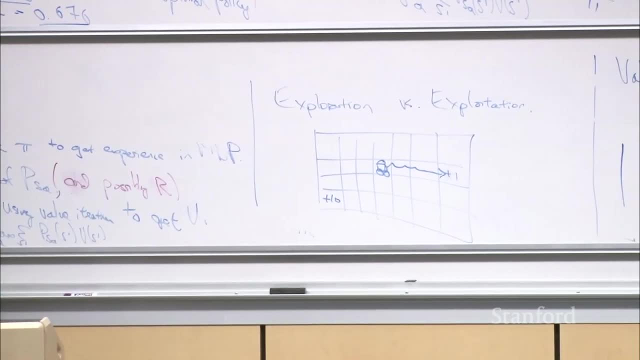 If just by chance, during the first time you run the robot, it happens to find its way to the plus 1, then if you run this algorithm, it may figure out that going to the plus 1 is a good way, right? 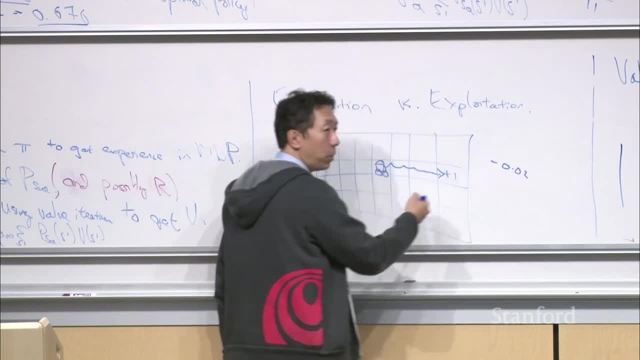 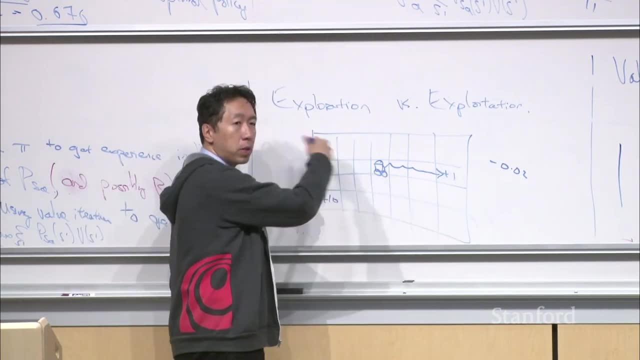 Or we- we're giving a discount factor. there's a field search charge of minus 0.02, on every step. So if just by chance your robot happens to find its way to the plus 1, the first few times you run this algorithm. 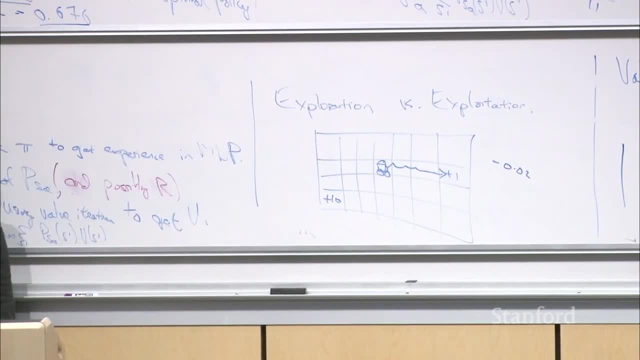 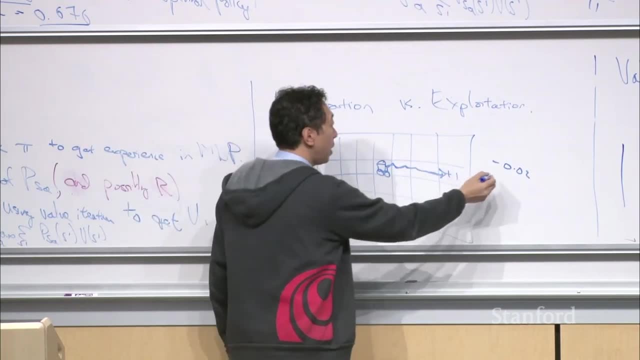 then this algorithm is, um is sort of locally greedy, right? Uh, it may figure out that this is a great way to get to a plus 1 reward, and then the world ends. It stops getting these minus 0.02 surcharges for fuel. 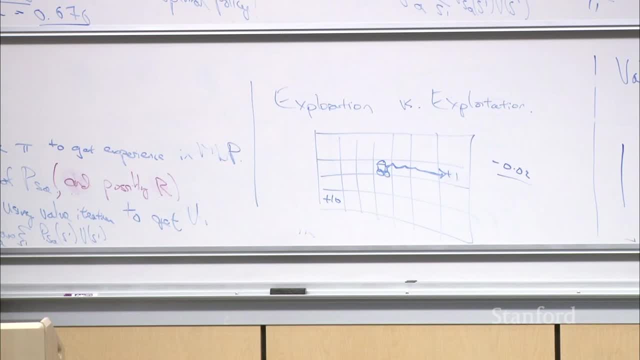 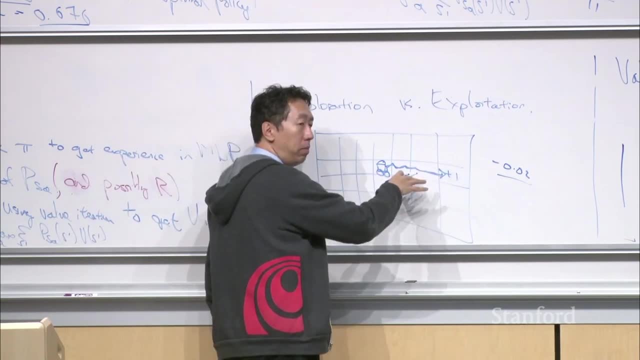 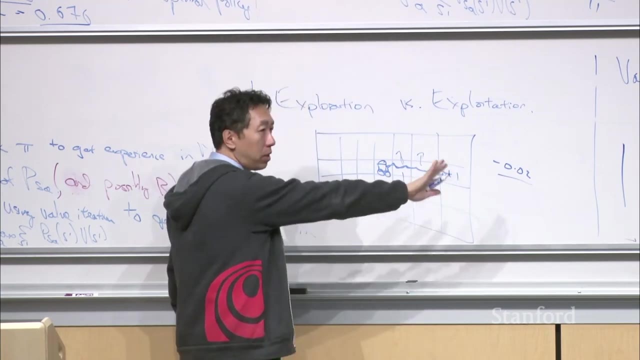 And so this particular algorithm may converge to a bad you know kind of local optima. where it's, it's always heading to the plus 1.. And as it hits the plus 1, sometimes it'll VR randomly right And get a little- little bit more experience in the right half of the state space. 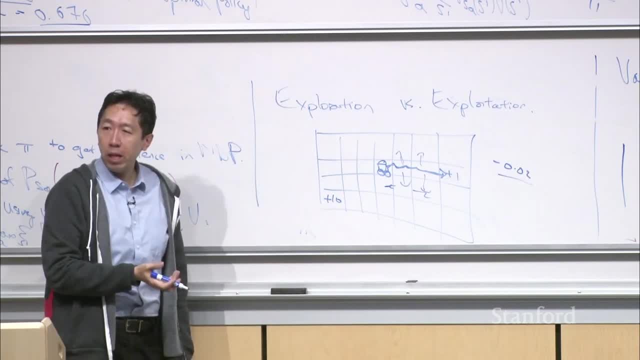 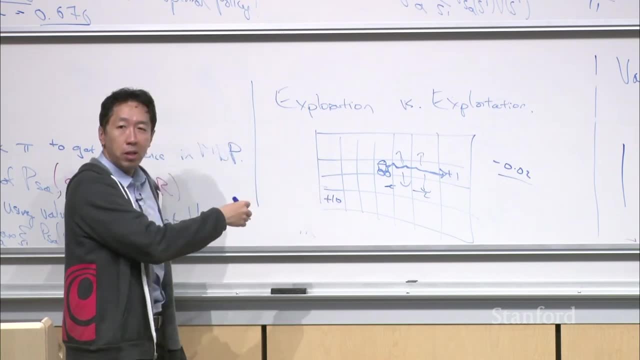 and end up with pretty good estimates of, uh, what happens in the right half of the state space And, um- and it may never find this hard to define- plus 10 polyp gold over on the lower left. Okay, So this problem is sometimes called- actually. 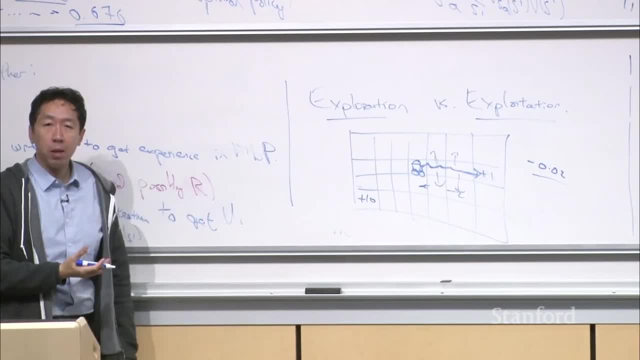 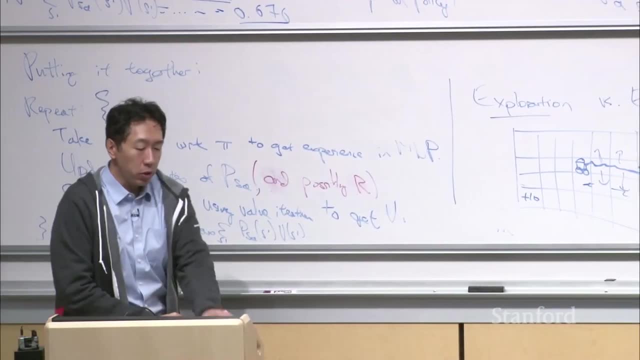 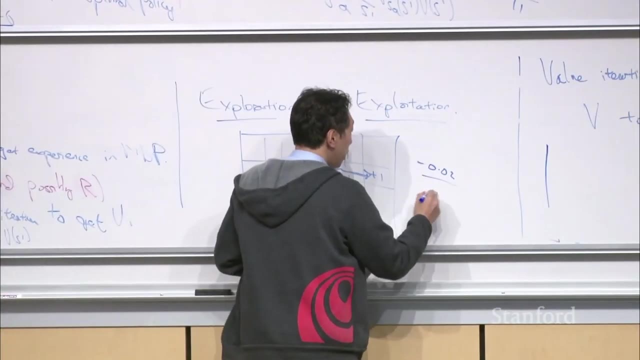 well, it is called the exploration versus exploitation problem, which is um when you're acting on an MDP, you know how aggressively or how greedy should you be at just taking actions to maximize your rewards, And so the algorithm we described is relatively greedy, right. 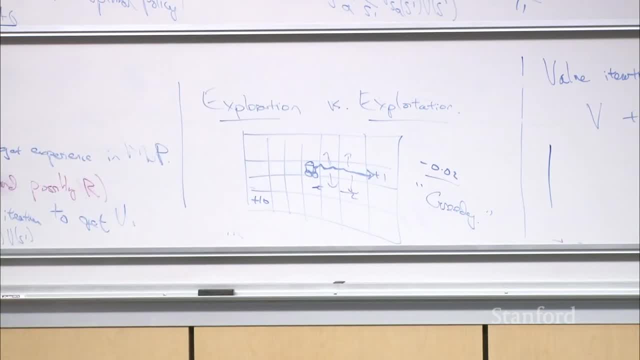 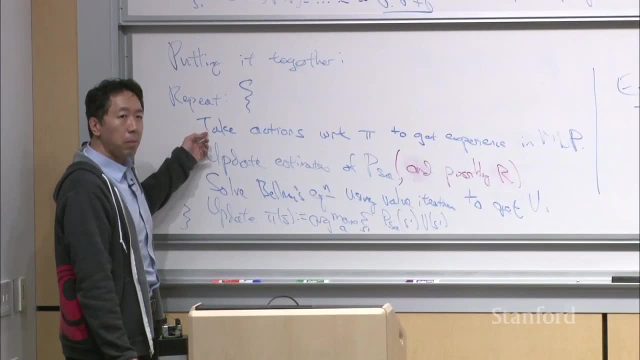 Meaning that, um, it's taking your best estimate of the state, transient probabilities and rewards and it's just taking whatever actions. And this is really saying: you know, pick the policy that maximizes your current estimate of the expected rewards, and it's just acting greedily. 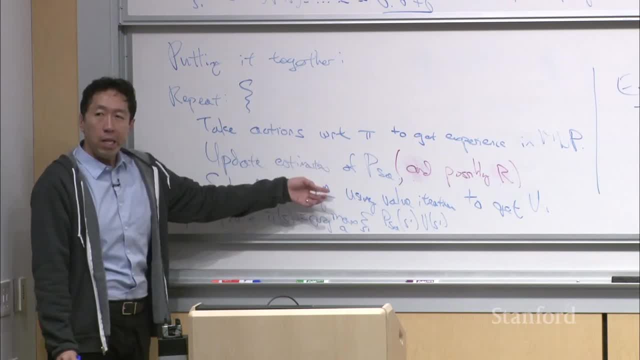 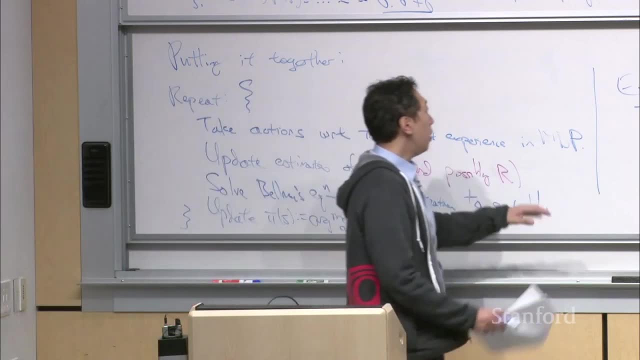 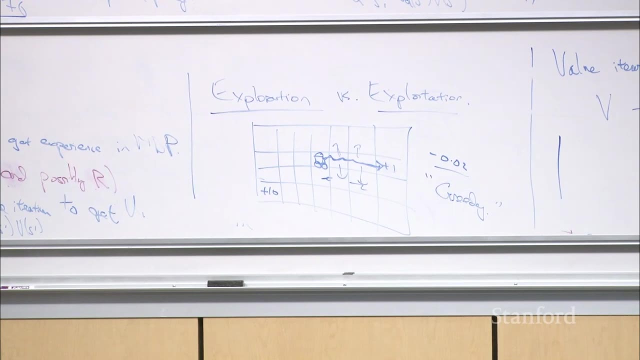 meaning on every step, it's just executing the policy that it thinks allows it to maximize the expected payoff right. And what this algorithm does not do at all is explore, which is the process of taking actions that may appear less optimal at the outset. 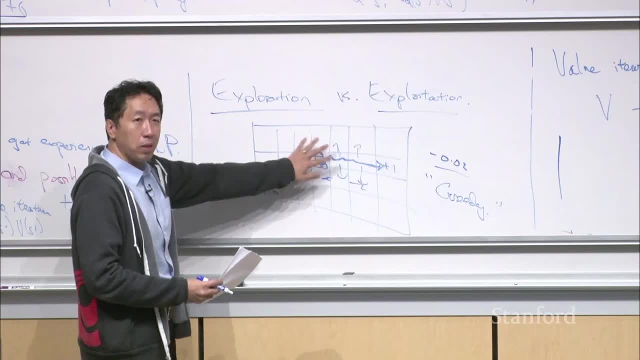 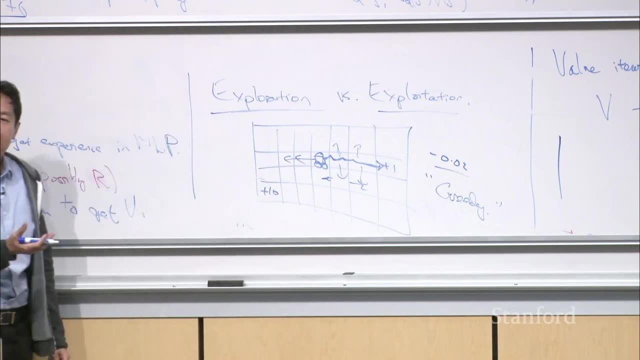 um, such as if the robot hasn't seen this plus 10 reward, doesn't know how to get there. maybe it should. you know, just try going left a couple of times, just for the heck of it, right To see what happens. uh. 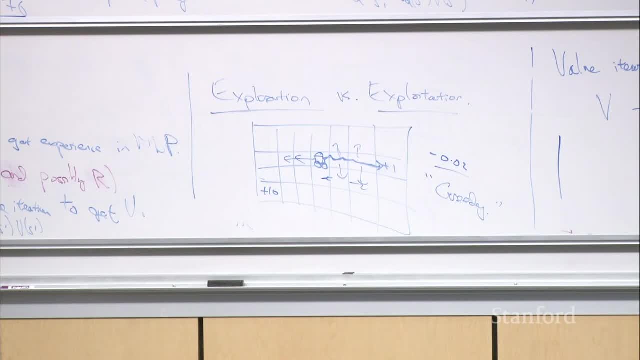 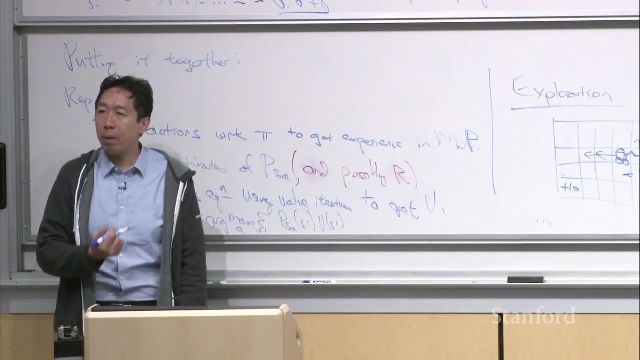 because, even if it seems less-, even if going left from the perspective of the current state of the knowledge of the robot, um, maybe if it tries some new things it's never tried before, maybe you'll find a new pot of gold okay. 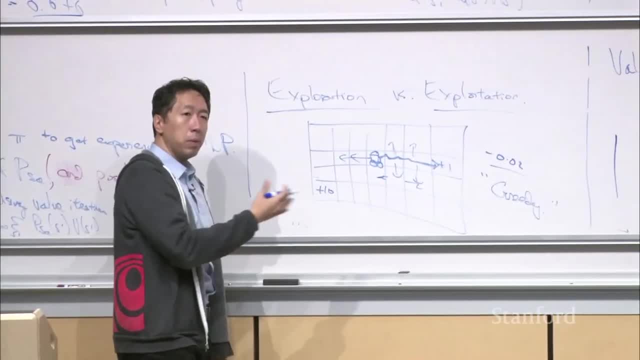 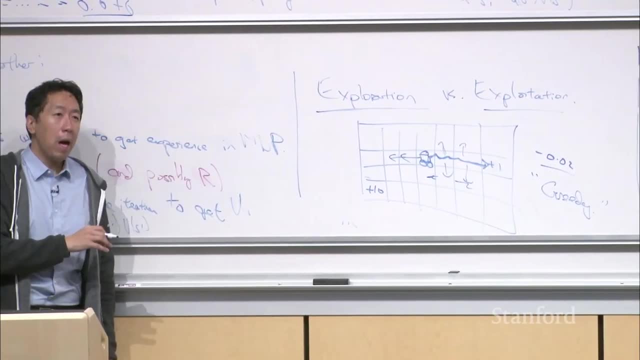 So this is called the exploration versus exploitation trade-off- Um, oh and- and this is actually not just an academic problem. It turns out that some of the large online web advertising platforms, uh uh, have the same problem as well. 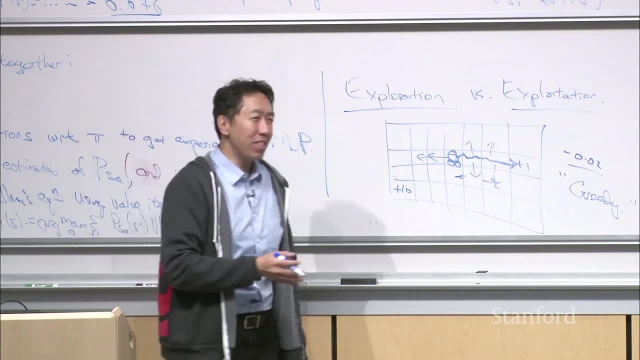 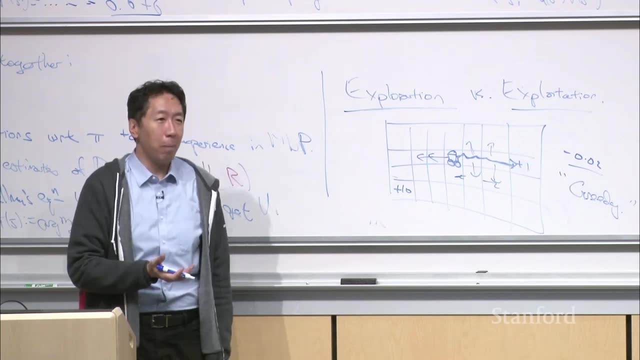 Again, I-, I-, I- I have mixed feelings about the advertising business. It's very lucrative, but it causes other problems. um, as well, But-. but it turns out that for some of the large online ad platforms, um, uh, you know, when, a- when an advertiser 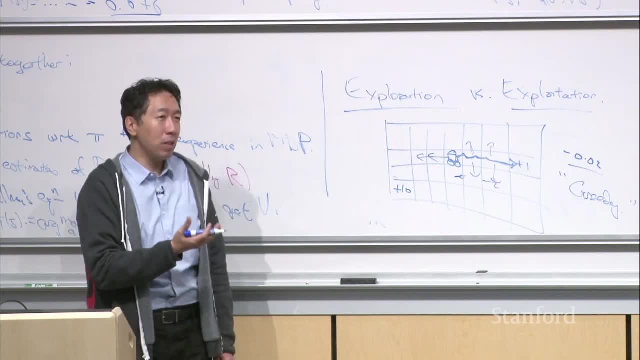 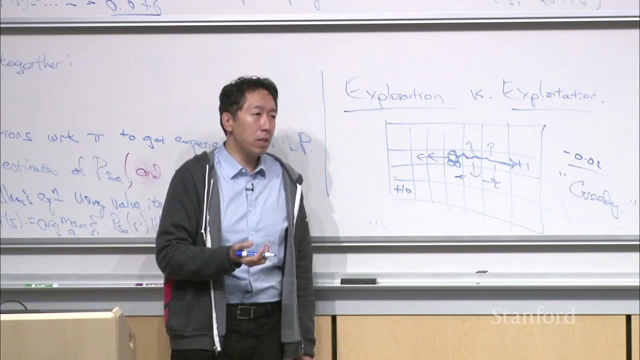 um, uh, starts selling a new ad or, you know, posts a new ad on one of the large online ad platforms. the ad platform does not know who is most likely to click on this ad, right And so pure explore-, pure exploitation. 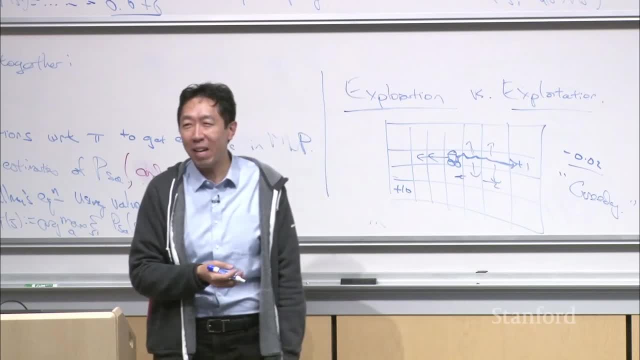 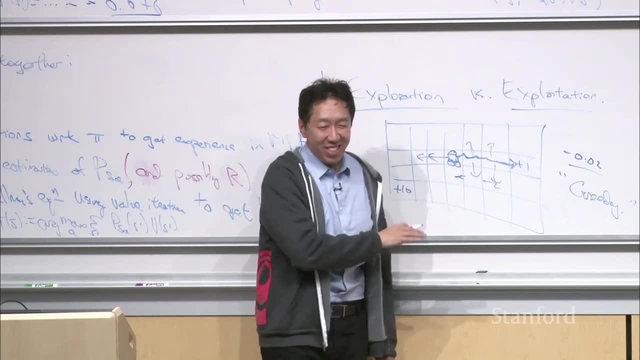 boy. exploitation is such horrible connotation, especially when you talk about online ad platforms. Uh, it's a technical term, not a-, not a social term when used in this context, But a pure- you know, reinforcement learning sense exploitation policy. 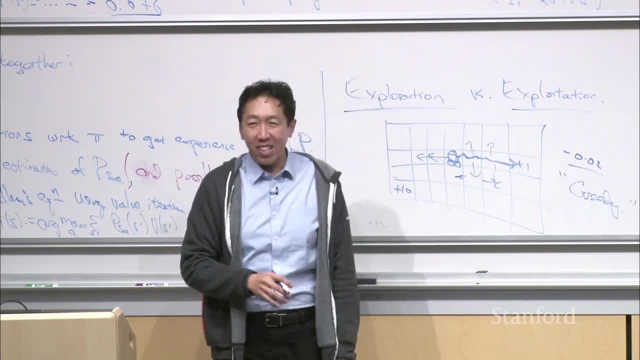 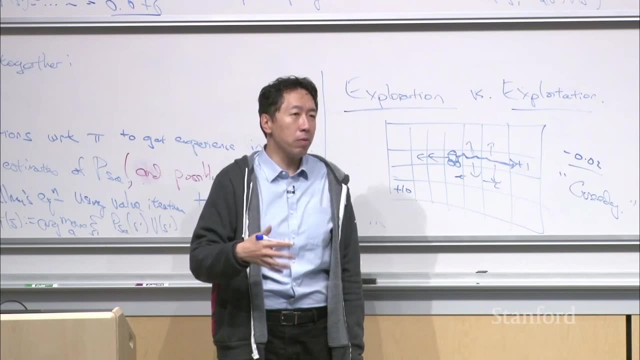 not- not the other. even more horrible sense of exploitation, um would be to always just show you- show- show- users the ads that you know they are most likely to click on to drive short-term revenues, Because we want to just show people the ad they're most likely to click on to drive short-term revenue. 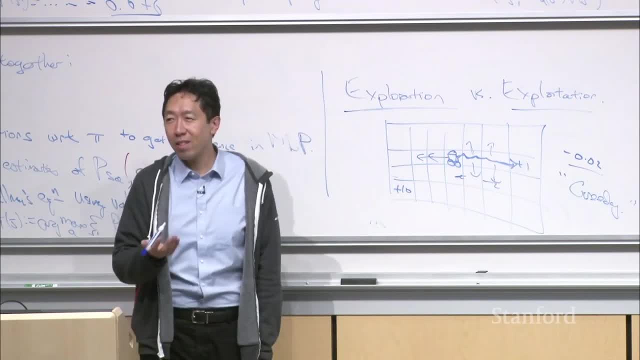 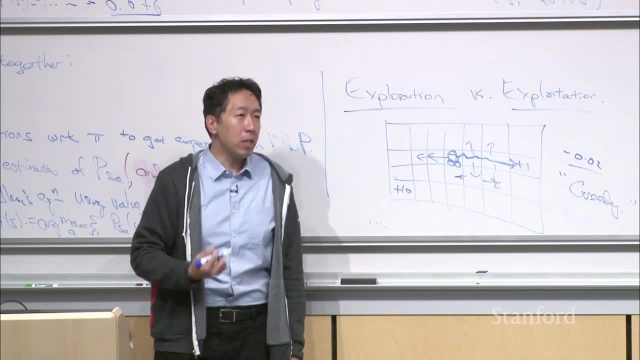 Whereas an exploration policy for a large- you know some of the large online ad platforms- is to show people some ads that may not be what we think you're most likely to click on in this moment in time, But by showing you that ad, or by showing a pool of users an ad that you might be less likely to click on, 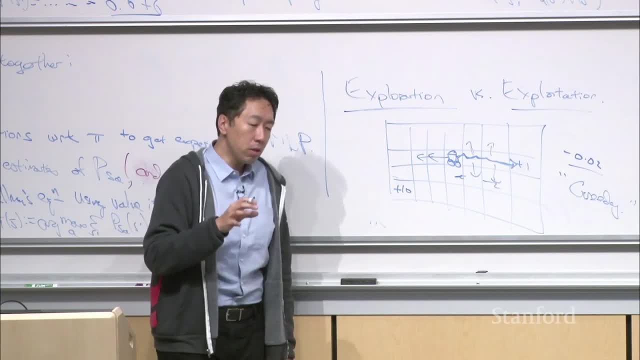 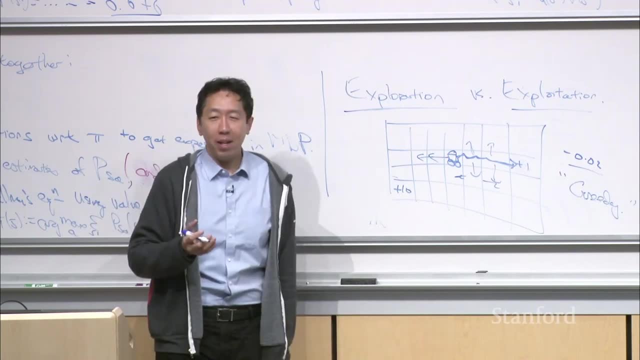 maybe you'll learn more about your interests, And that um increases the effectiveness of these large- of these ad platforms at finding more relevant ads, right? I mean, for example, I don't know, um, probably not-. I- I guess, uh. 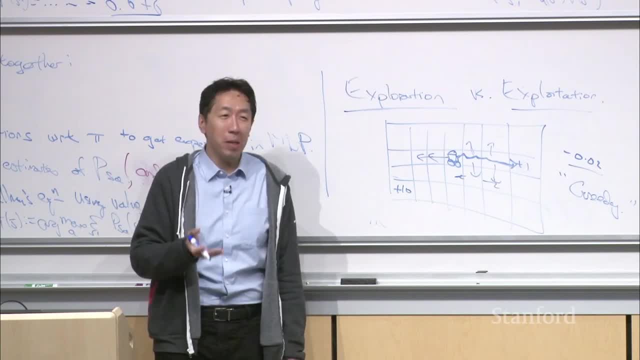 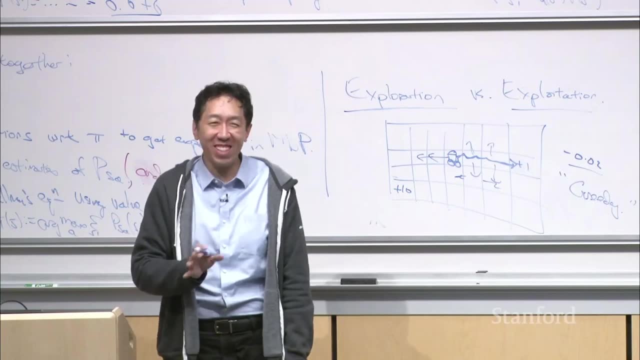 there are probably no advertisements for, uh, Mars landers, as I know. But if the large online ad platforms don't know that I'm actually pretty interested in Mars landers, if it shows me an ad for Mars lander, which I don't think such a thing exists right. 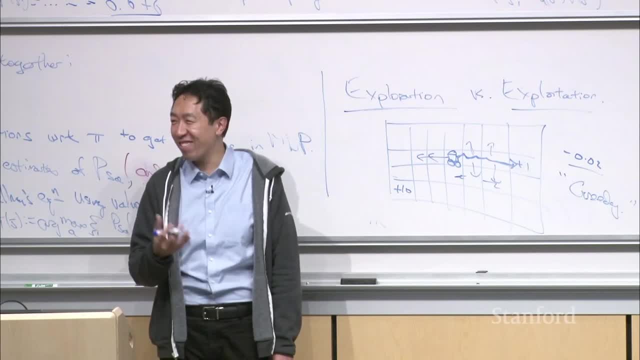 And finds that I click on it, then they may learn that showing me ads for Mars landers is a great thing, right Or- or some other thing that it may not know you're interested in. So this is actually a real problem. 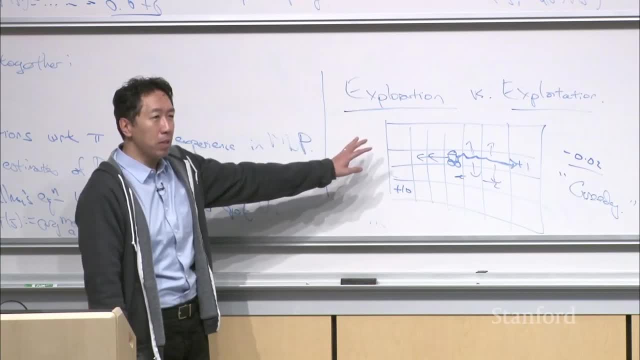 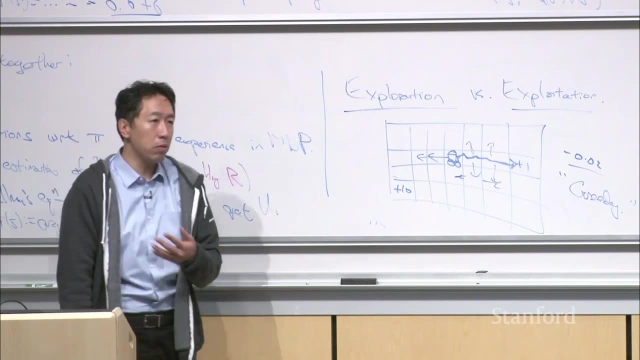 There are, um, uh, some of the large online ad platforms. uh, um, actually do explicitly consider exploration versus exploitation and make sure that sometimes it shows ads that may not be the most likely you click on, but you know. 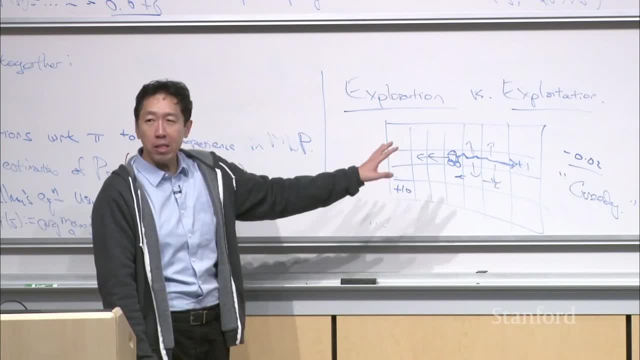 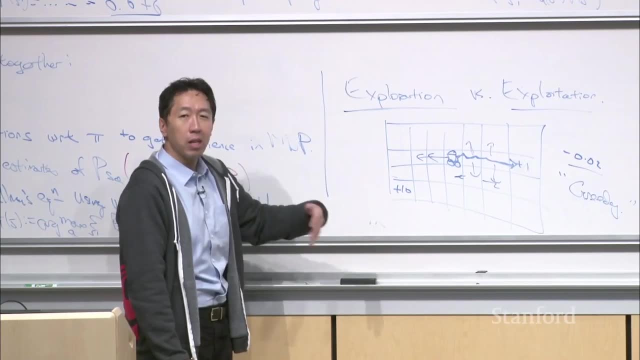 allows you to gather information, to then be better situated to figure out where the future rewards to- to be better positioned to, uh uh, learn how to match ads, not just to you, but to other users like you, right. 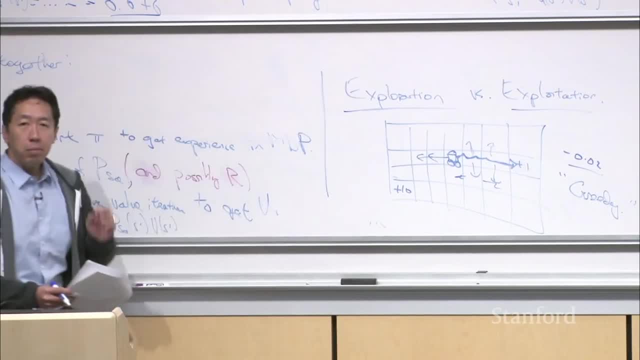 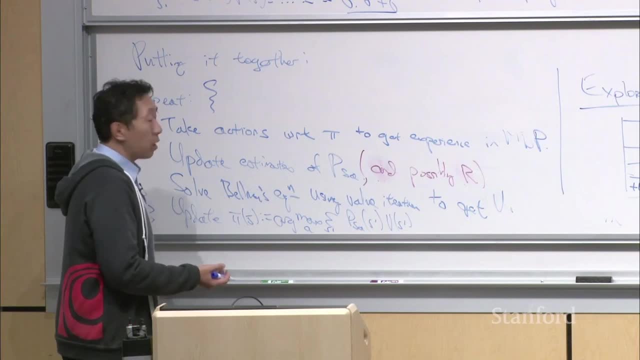 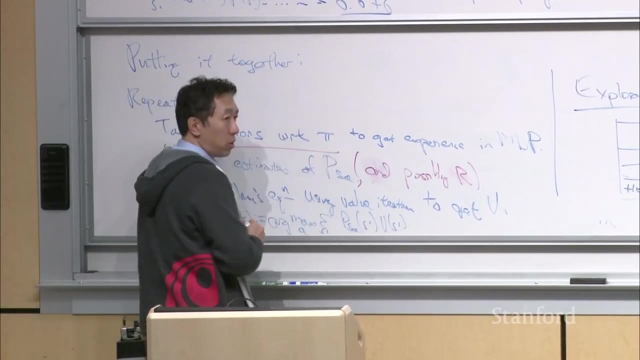 Um, sorry, Okay, But so in order to make sure the reinforcement learning algorithm um uh, explores as well as exploits a, um, a common uh uh modification to this would be take- instead of taking actions with respect to Pi. 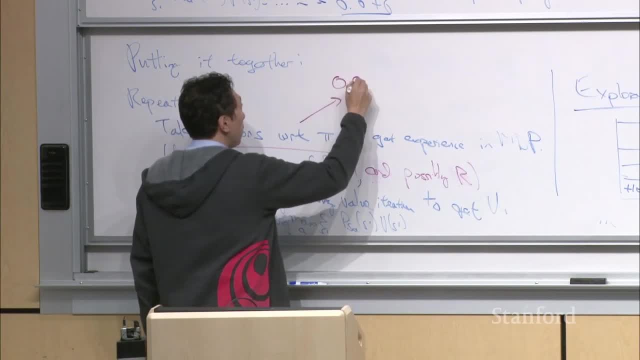 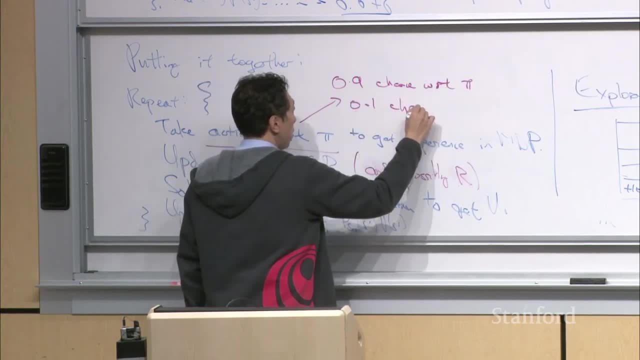 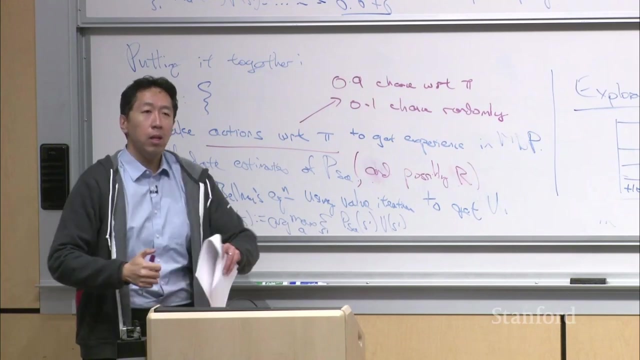 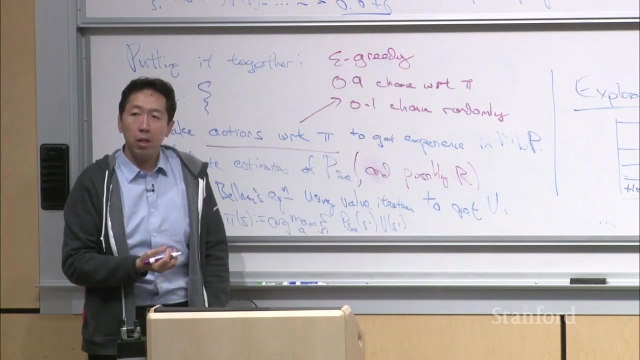 you may have a um uh 0.9 chance with respect to Pi and 0.1 chance. take an action randomly, okay, And so um. this particular exploration policy is called Epsilon greedy, where on every time step. 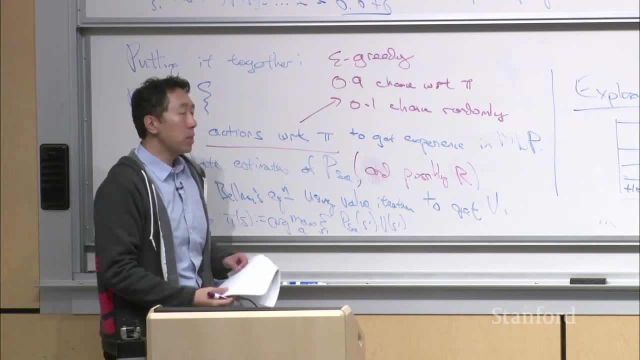 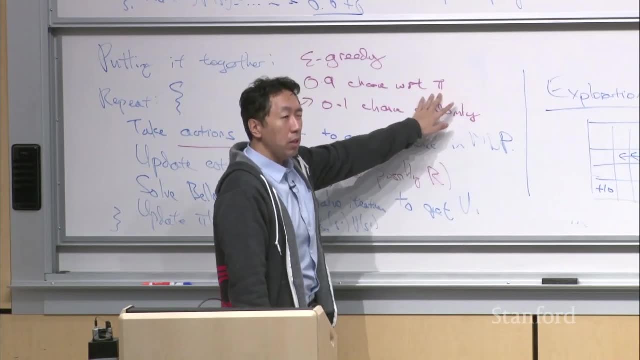 and on every time step you toss a biased coin. But on every time step- let's say, 90% of the chance, you execute whatever you think is the current best policy and with 10% chance you just take a random action. 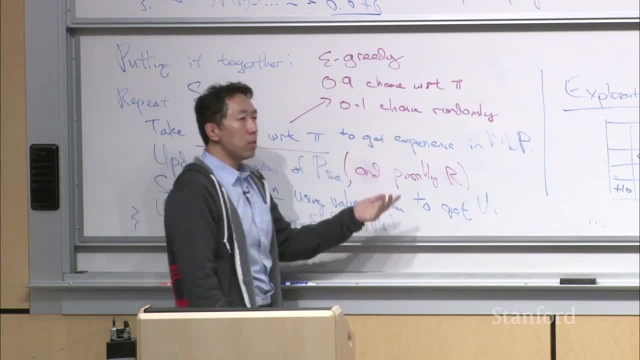 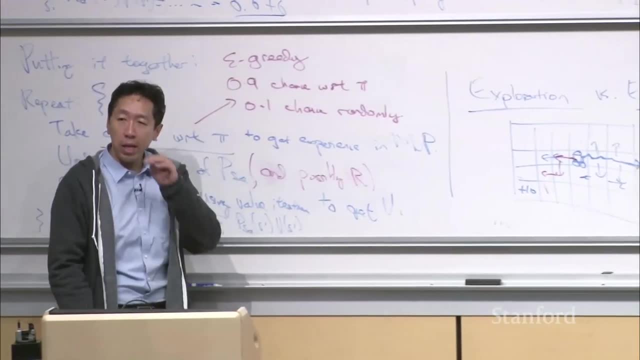 And this type of exploration policy, um increases the odds that you know every now and then maybe just by chance, right, It'll find its way to the plus 10 pot of gold and learn state transition probabilities, and-, and- and then eventually, 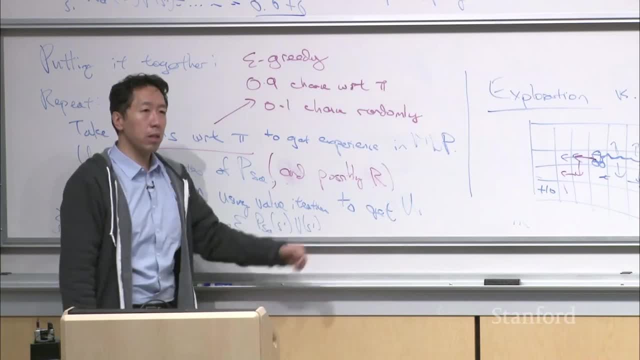 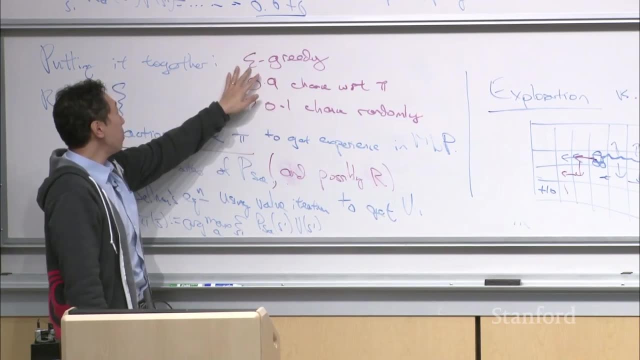 um, end up exploring the state space more thoroughly. okay, Um, this is called Epsilon greedy exploration, and, um, it's a little bit of a misnomer, I think. Uh, so in- in- in the way we think of Epsilon greedy. 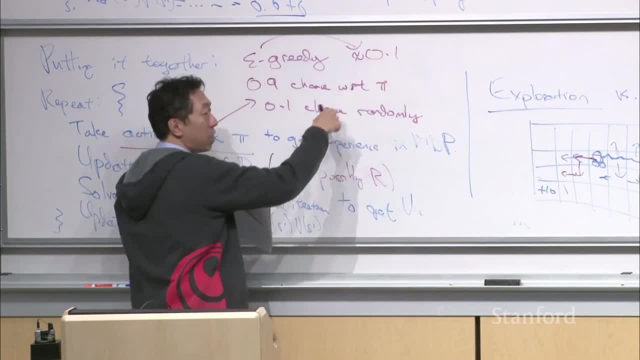 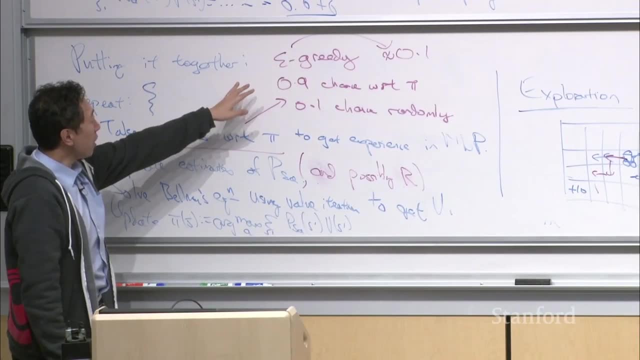 Epsilon is, um say, 0.1, is the chance of taking a random action instead of the greedy action. Um, this algorithm is- is always been- a little bit strangely named because, uh, if 0.1 is actually the chance of you acting randomly, right? 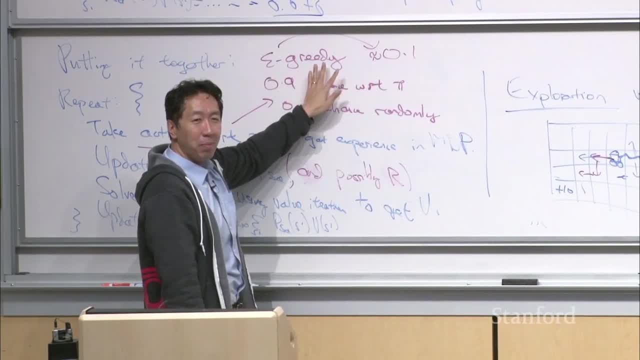 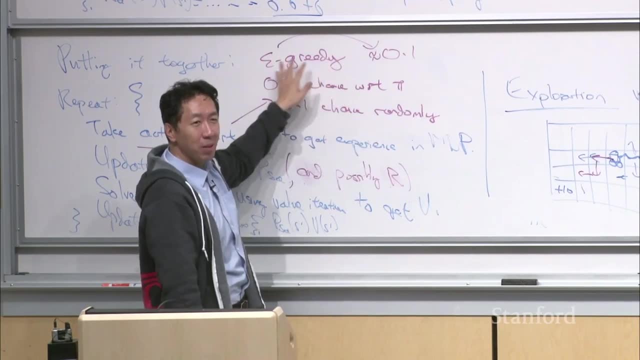 So Epsilon greedy sounds like you're being greedy 0.1 of the time but- but you're actually taking actions randomly 0.1 of the time. So Epsilon greedy is actually maybe 1 minus Epsilon greedy. So this- this name has always been a little bit um off. 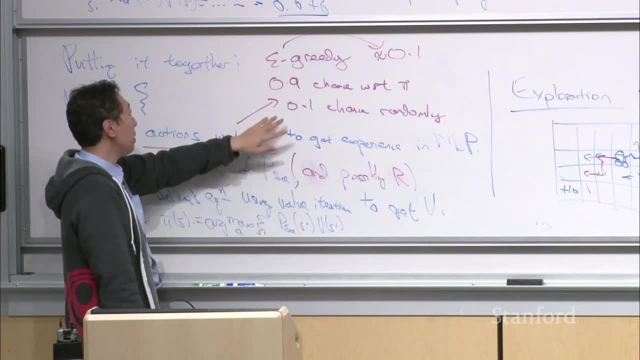 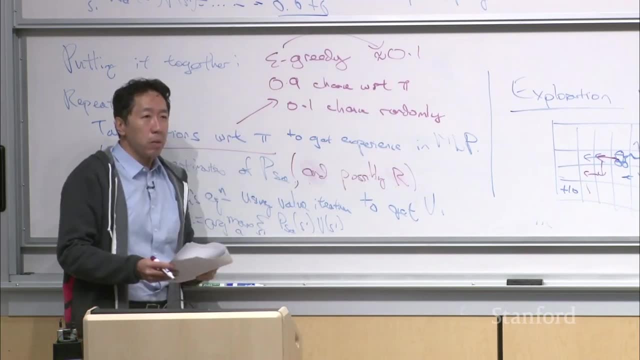 but- but that's what- that's- that's- that's how people use this term. Epsilon greedy exploration means Epsilon of the time, which is a hyperparameter, which is a parameter of the algorithm you act randomly into- instead of going to what you think is the best policy. okay. 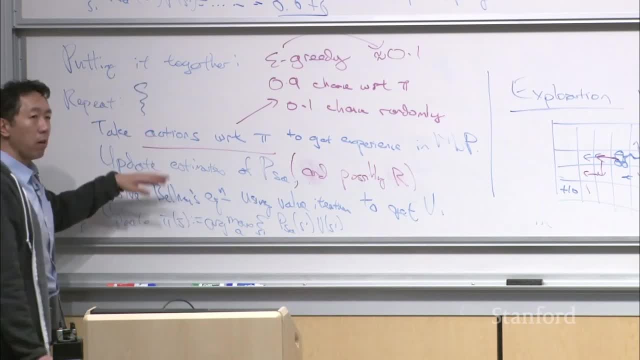 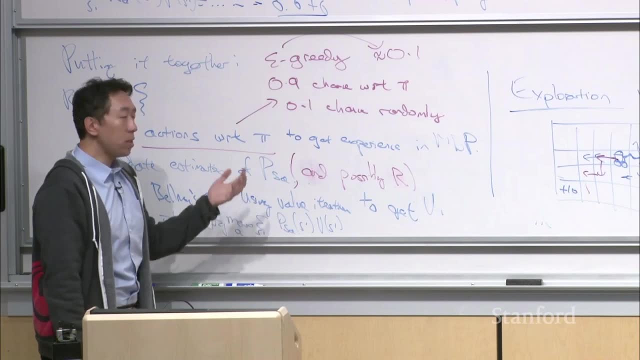 And it turns out that, um, if you, um, if you implement this algorithm with um Epsilon greedy exploration, then this, uh, uh, this algorithm, um, will converge to the optimal policy for any discrete state: MDP right. 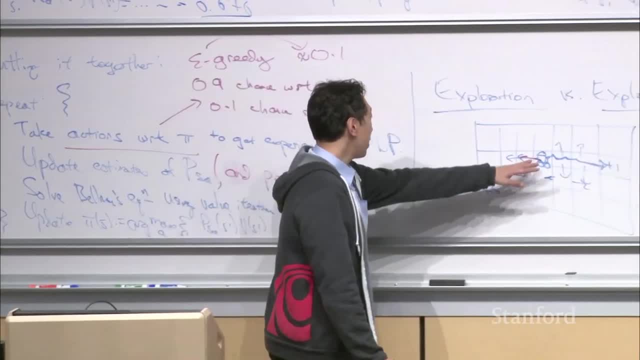 Uh, sometimes they take a long time because you know, if there's a- if it takes a long time to randomly find plus 10, it could take a long time before it randomly stumbles upon the plus 10 part of goals. 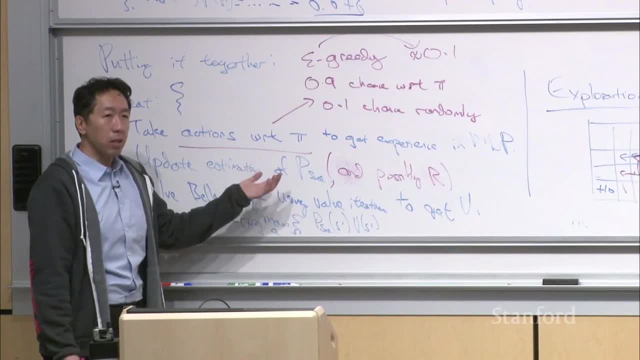 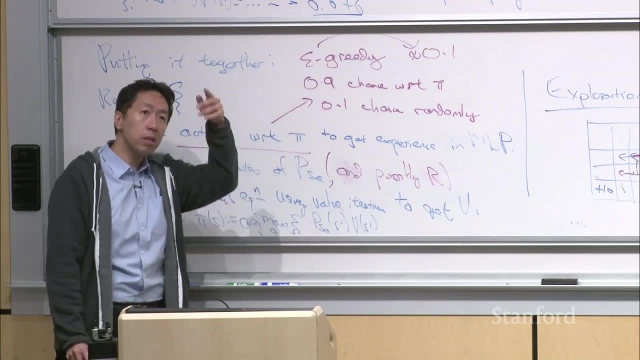 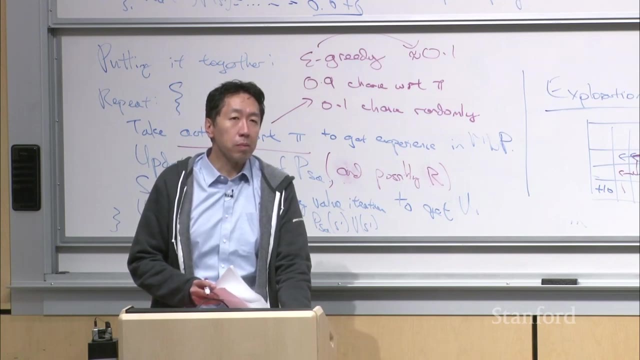 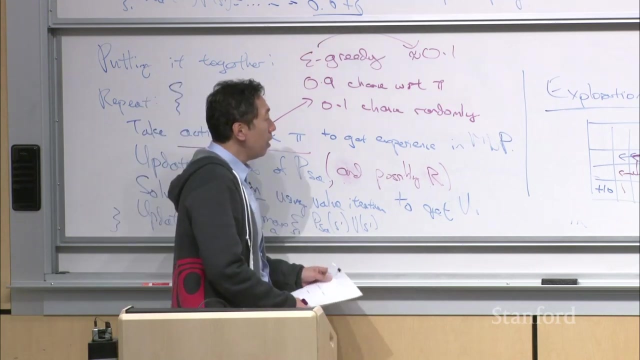 But um, this algorithm with an- with an exploration policy, will converge to the optimal. um will converge the optimal policy for any MDP. Is there a question? Oh yeah, Yes, So right, Should you always keep Epsilon constant or should you do dynamic string Epsilon? 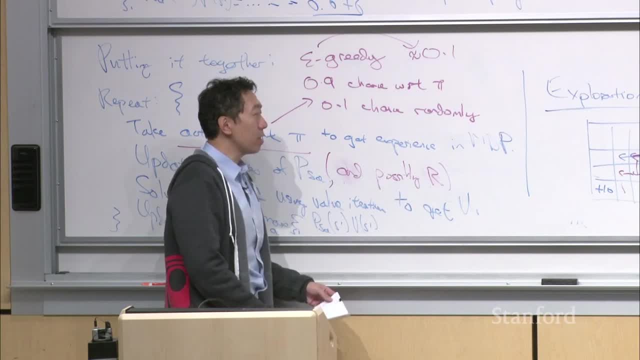 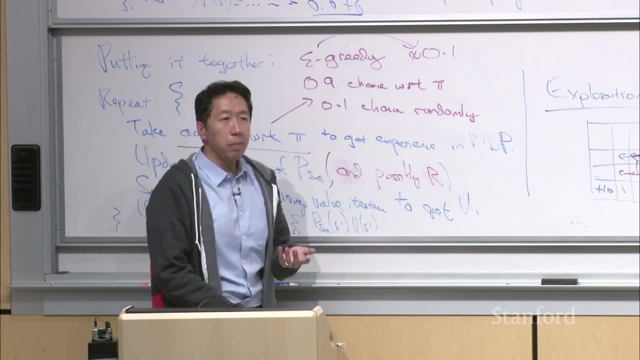 So, yes, uh, there are- there- there- there are many heuristics for how to explore. Uh, one reasonable thing to do would be start with a large value of Epsilon and then slowly shrink it. Um, another common heuristic would be: 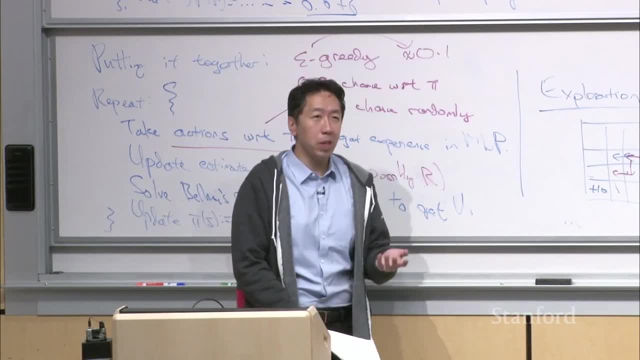 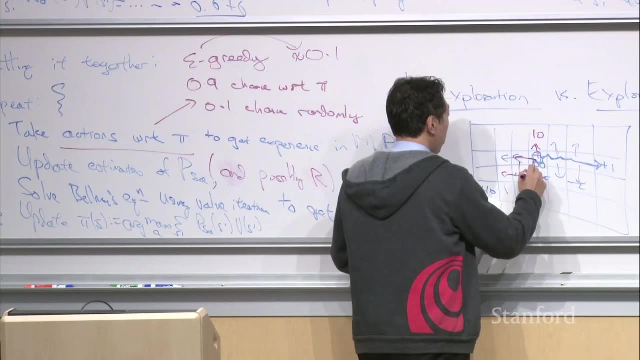 um, uh, there's a different, uh, uh type of exploration called Boltzmann exploration that you can look up if you want, which is, uh, if you think that the value of going off is, um, you know, 10 and the value of going south is 1,. 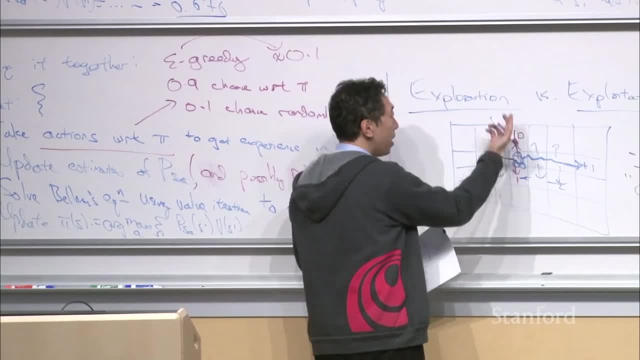 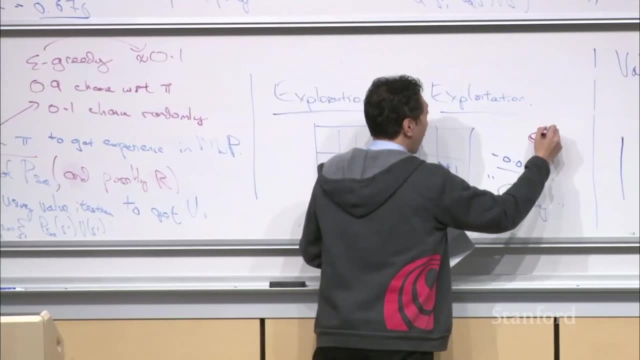 then there's such a huge difference that you should bias your action to what going to. the bigger result, the- the bigger reward and uh, you could have the probability be E to the value. basically, right Time, uh, divide it uh. 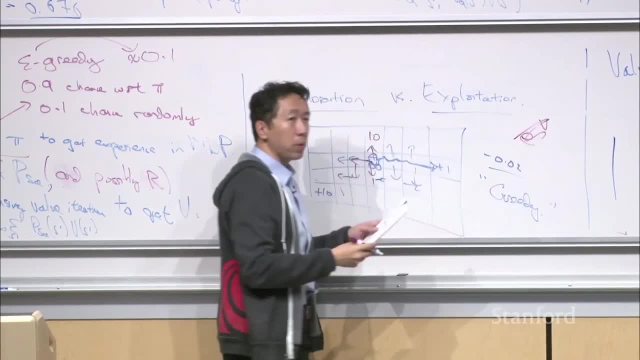 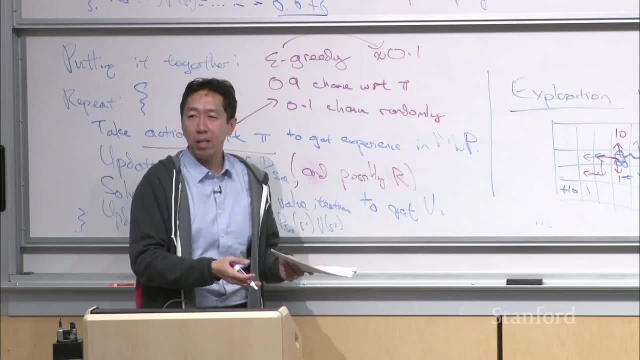 times the- times the scaling factor right. So that's called Boltzmann exploration, where, instead of having a 10% chance of taking action completely at random- uh, you could, just you know, have a very strong bias to heading toward the higher values. 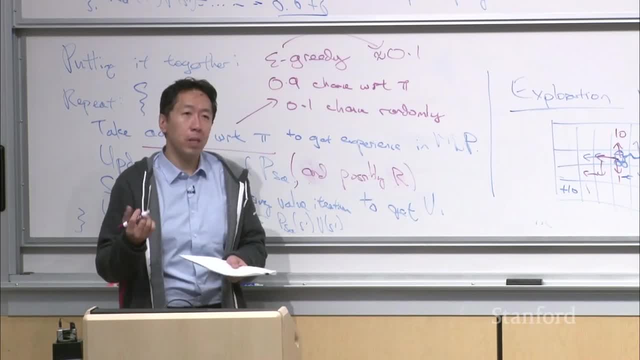 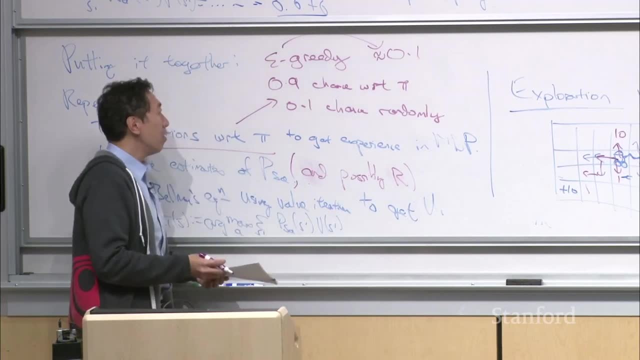 but also have some probability to going to lower values, but where the exact probability depends on the difference in the actual values. This- so another- probably the- I think Epsilon- greedy- I feel like I see this used the most often for these types of MDPs. 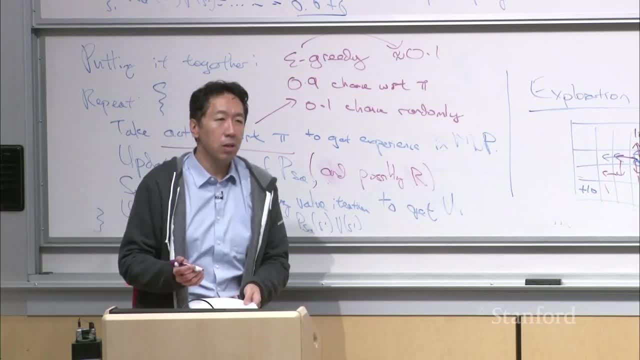 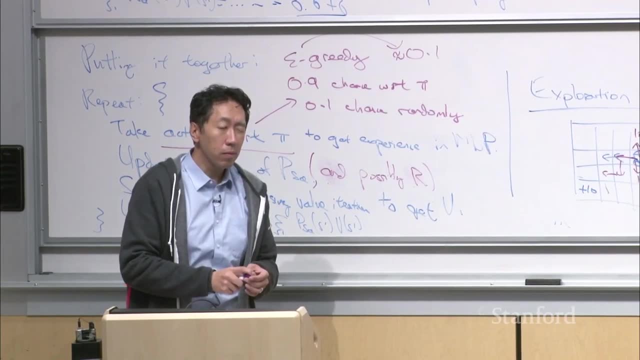 and then Boltzmann exploration, which- which is why I just tried this- also use. Well, I'll use two more questions. One more question as we wrap up. Go ahead. Uh, can you also give a reward for reaching states you've never seen before?